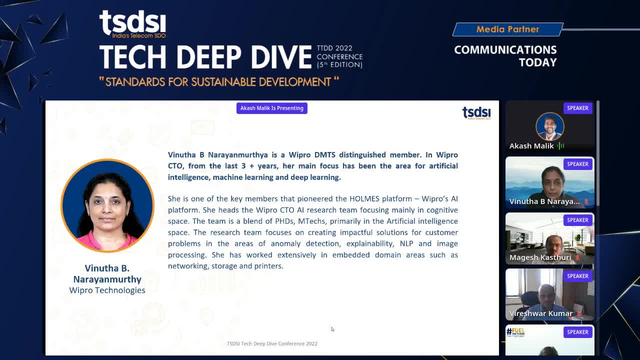 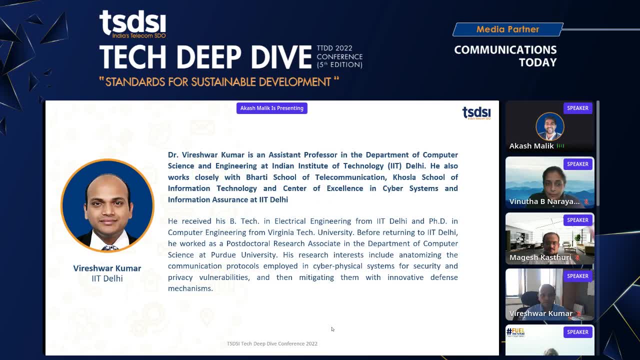 Her main focus has been the area for artificial intelligence, machine learning and deep learning. Introducing Dr Veereshwar Kumar. he is an Assistant Professor in the Department of Computer Science and Engineering at the Indian Institute of Technology, Delhi. He also works closely with the Bhartik School of Telecommunication. 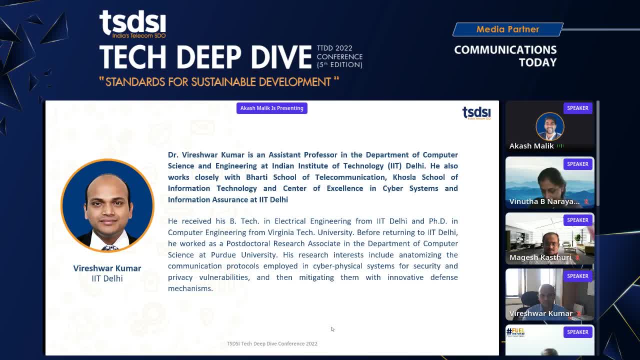 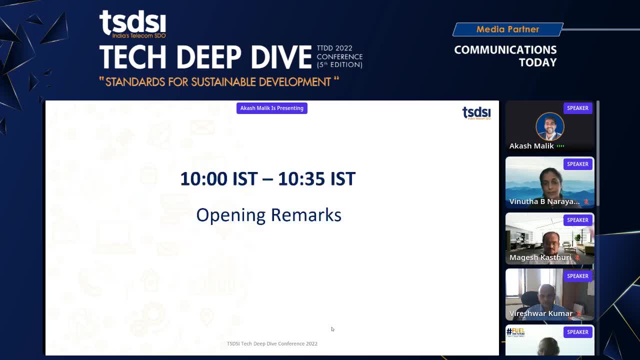 Khosla School of Information Technology and Centre of Excellence in Cyber Systems and Information Assurance at IIT Delhi. Welcome co-chairs. We would like to give opening remarks Over to you. Thank you, Thanks, Akash. So good morning everybody. 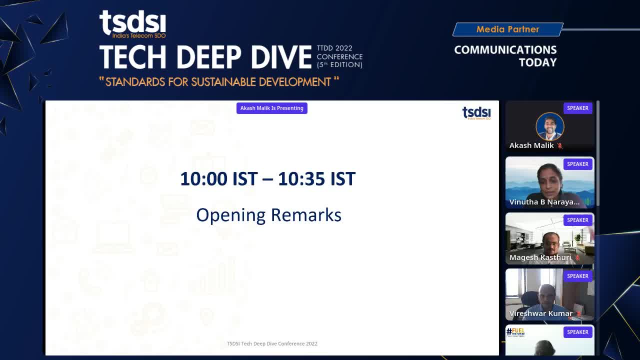 I'm Vinuta Vinuta. we'll just give a brief on what we can expect as part of this session. As we all know, we know that 5G Connections- GSMA states that 5G Connections surpassed 1 billion in 2022 and 2 billion by 2025.. 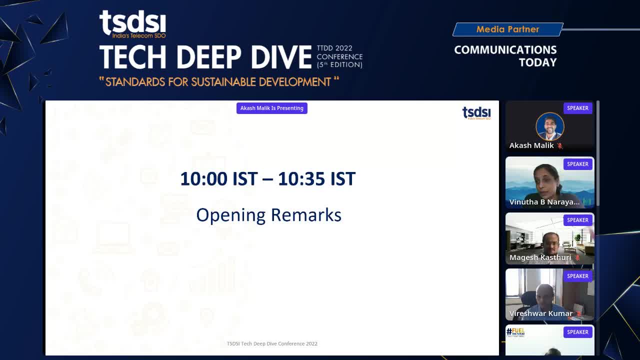 With its rapid strides in technology. we have a 5G-enabled IoT world that can help one monitor their own homes, provide healthcare services even to remote places, feed data at ultra-low latency for autonomous vehicles to take rapid decisions. We also have quantum computers that have come in. 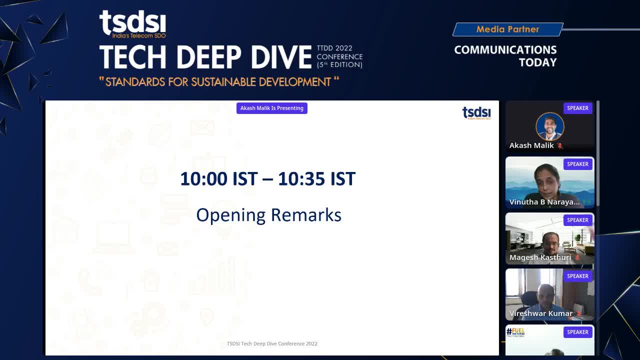 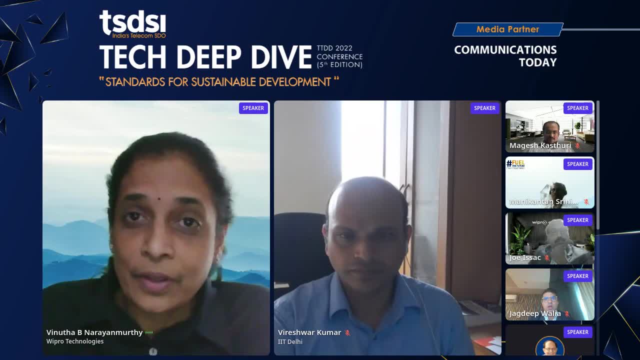 to help you solve complex problems in real-time. But how secure is this 5G-enabled IoT world in the presence of quantum computers? Today, in the world of IoT, there's a possibility. we've also seen instances where malware can attack home networks. 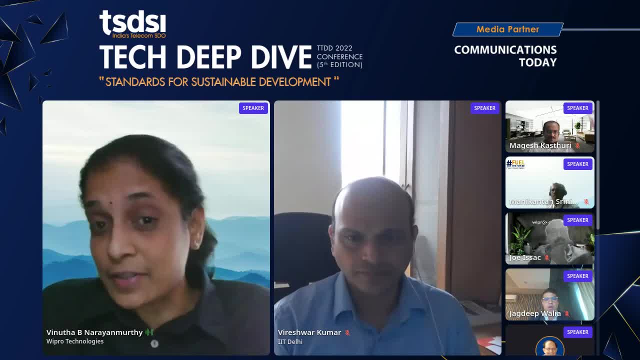 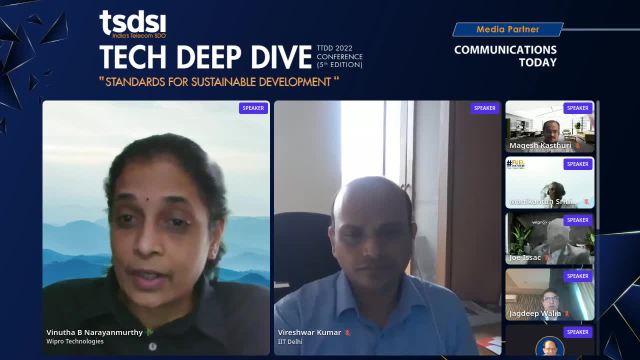 There's also a possibility that you know you can have: a sabotage of healthcare systems. 5G, with its rapid strides in technology, has come in which can, with a lot of taken up, try to take care of constraints there in the 3G and 4G issues. 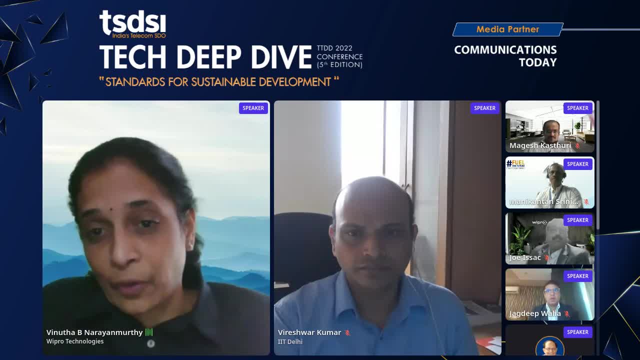 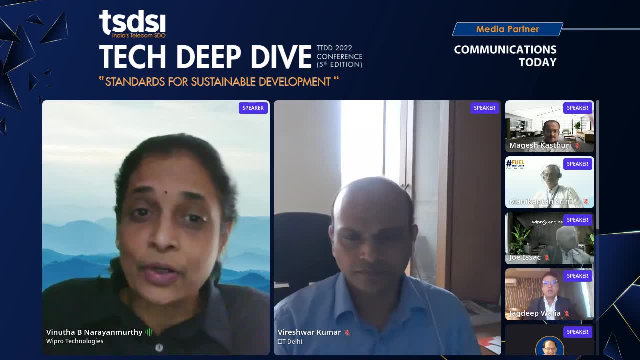 like you know, encryption, better encryption, ensuring you cannot track people, and things like that. A lot of security things have been taken care of in 5G, But it also has brought in all this with concepts like network virtualization, network slicing, new technologies. 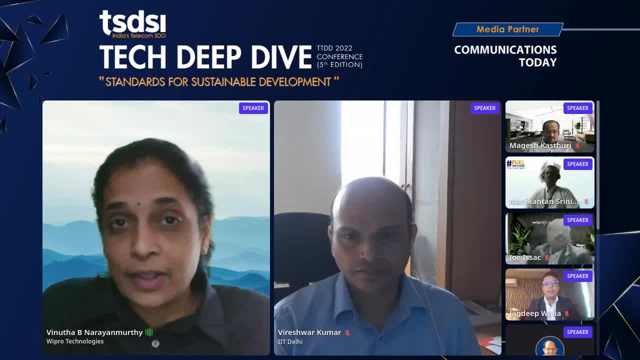 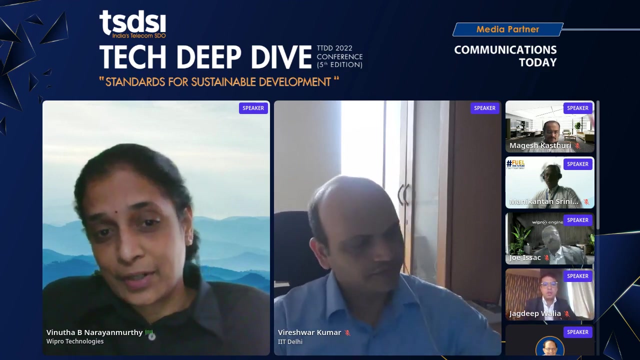 which come with their own security challenges. Further, the existing cryptography technologies can be easily broken by quantum, So security is a key aspect so that to ensure inheritance to be handled by these technologies, so that we can all live comfortably in this world in a secure way and enjoy the technology trends. 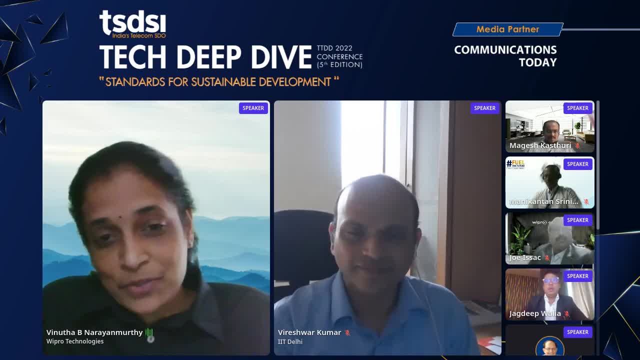 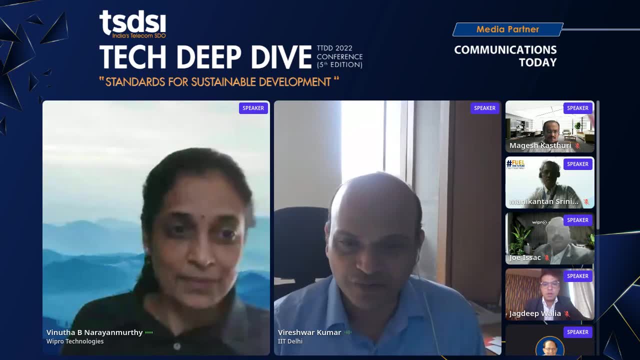 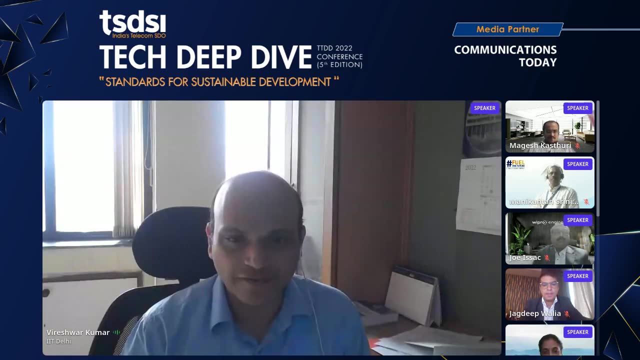 I would also hand over to Professor Veeresh for his thoughts. Yeah, thanks, Vinita, for that introductory remarks. Good morning everyone. I welcome all the speakers and all the attendees here. So I think we have three keynote speakers. 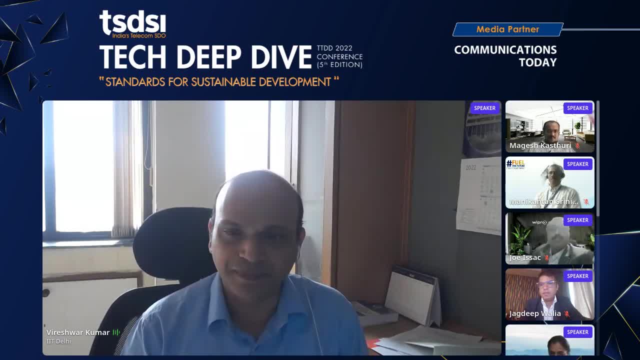 who will talk about the different aspects of 5G security, IoT security and quantum computing-related issues. And then we have a nice panel there, an excellent set of speakers there, who will discuss the impact of quantum computing on 5G-enabled IoT. 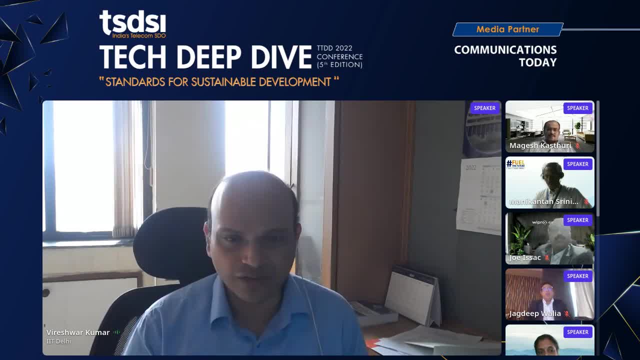 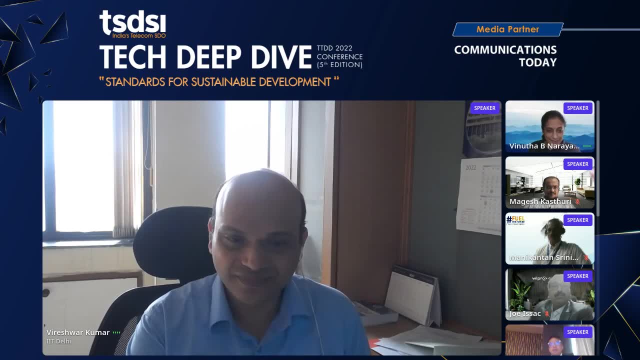 So I look forward to a nice session Without any further ado, we should go to the first keynote address. So back to you, Vinita, Thank you. Thank you, Professor Veeresh. The first keynote session is by Joe Isaac. 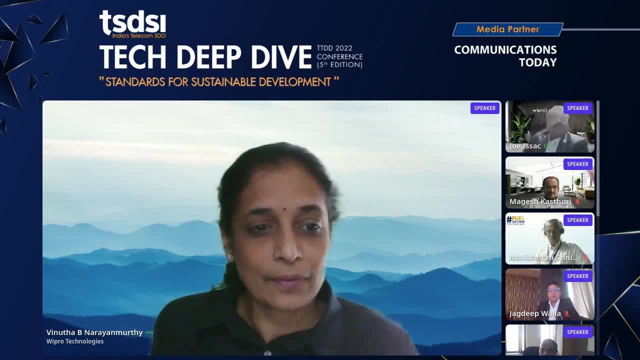 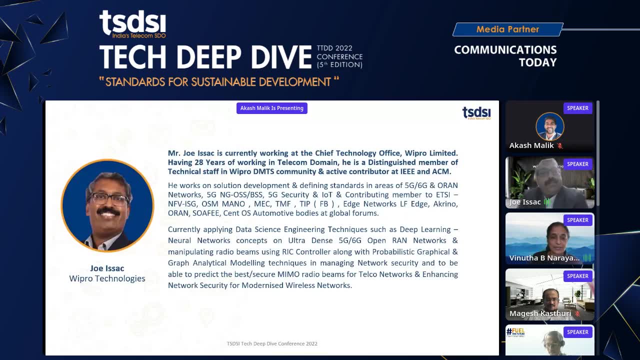 a nuclear technologist. Hello Vinita, Hello all Yeah. So I'll just give a brief introduction. I'll just talk quickly about Joe Isaac. He's currently working with the CTO division in Wipro. He has over 28 years of experience in telecom domain. 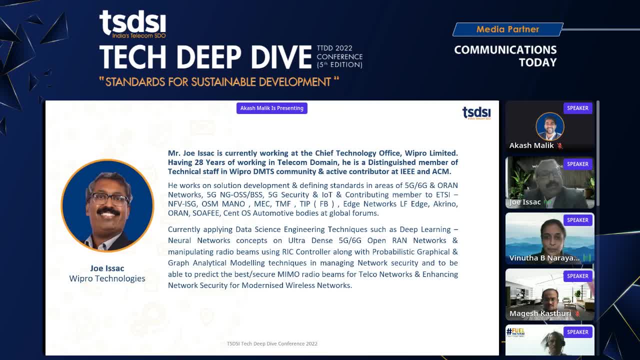 The list is endless. He's a distinguished member of technical staff in Wipro, contributes actively to various standards in IEEE and ACM. He also implements solutions, which actually helps him define the standards better. And also, not the least, he's also taken care of getting data science into the 5G world. 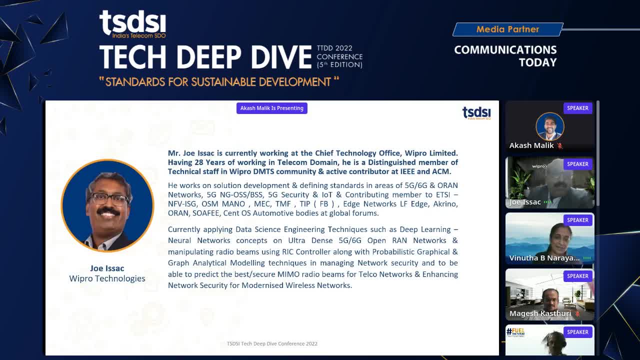 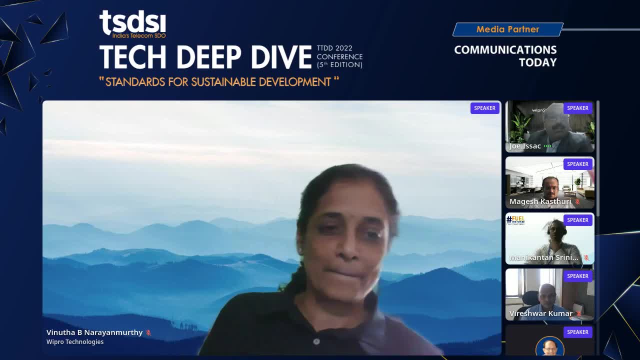 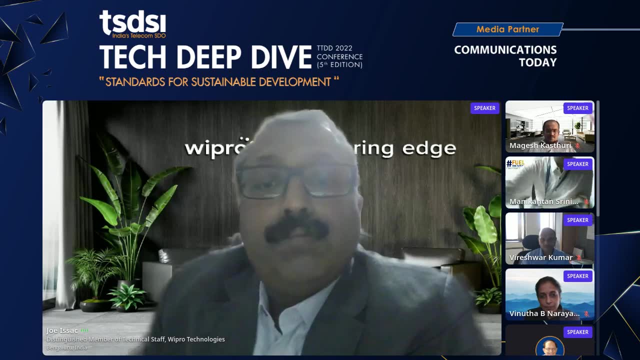 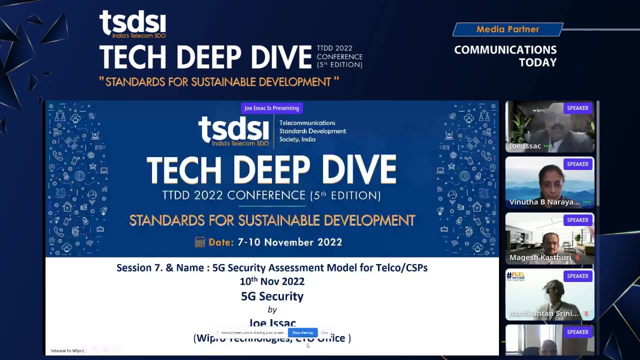 which is wonderful to see Over to you, Joe, for your session. Thank you, Vinita. I'm just sharing my slide. Sure, I hope my slide is visible. Yeah, Okay, So the thing. very good morning to you all. 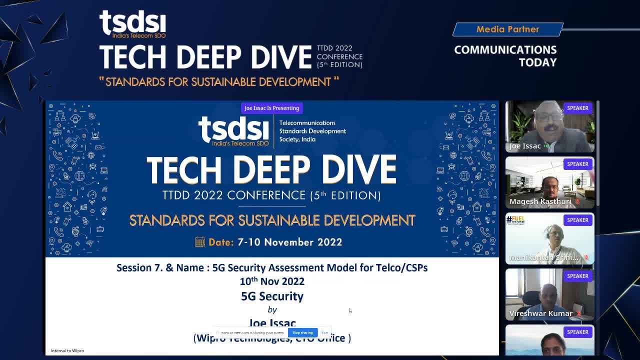 The theme I took up today for 5G secure- 5G security side was, instead of looking at the whole standards as the perspective, how can 5G security assessment be a model for implementation of a known or unknown security methodologies within a network? 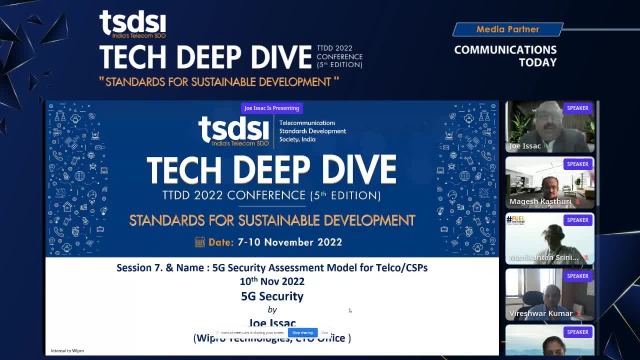 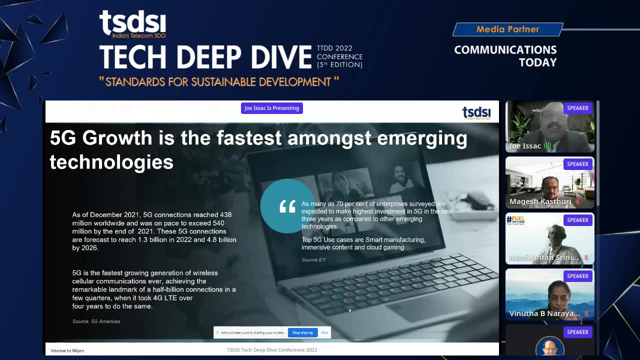 or within a telco core network or for a service provider. That's the area I took up today to have for a small discussion And that's the basis of my whole of this conversation. So we know that 5G growth is something which we're seeing is the most fastest or emerging technologies. 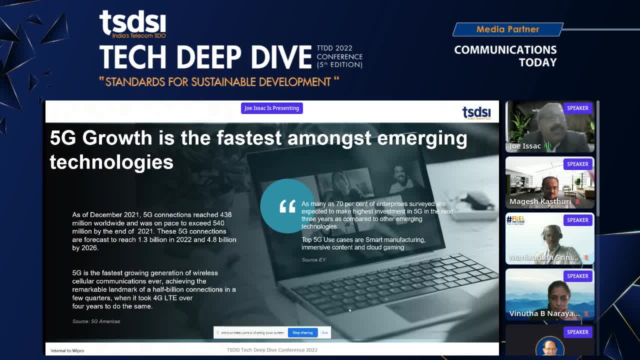 for the last three or four years We've seen a lot of implementations of 5G going live in places very far, like the AT&T networks or the telephonic networks, or even in India, as much that it has gone live today with 5G trial networks running on. 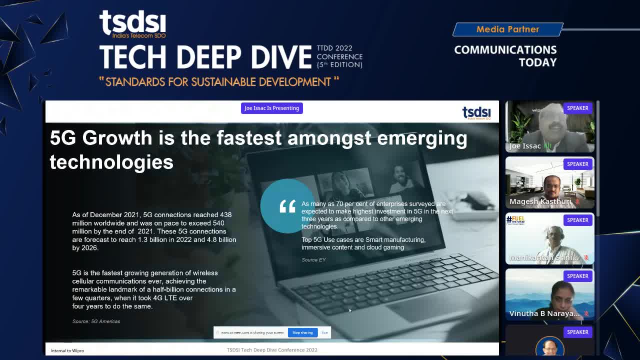 And there's been a lot, lot of importance of data to be one of the most adamant seen acumen around the whole mobile computing industry. We're seeing data- the voice video data- converging on the same plane, while mobile broadband gets even more popular. 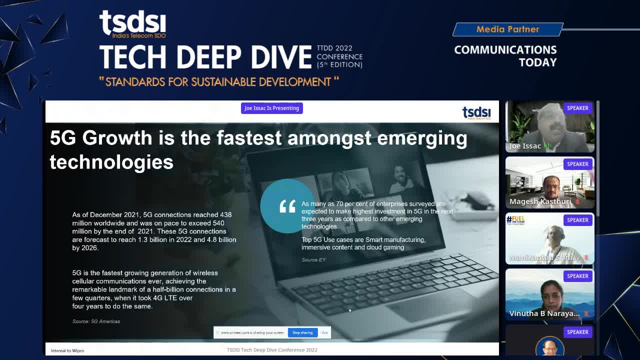 So there's, there is a huge outflow and we have something reached about 500 million worldwide space, So 540 million around the 5G connections will up with the with the middle of, I think, the July to the to about 550 million. 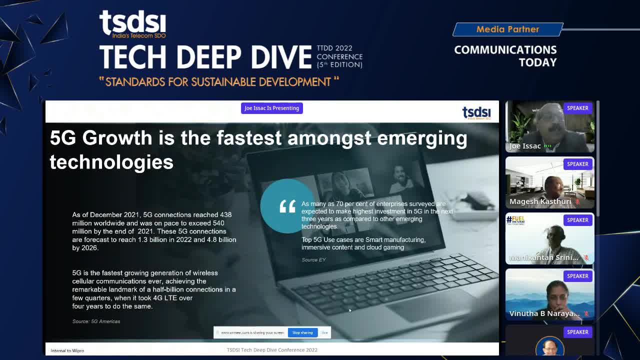 So I'm right around. that was the connection stand only on 5G. We're seeing faster growth in India as well. We're seeing 5G making its importance into every domain we think of, Be it the banking, be it the security. 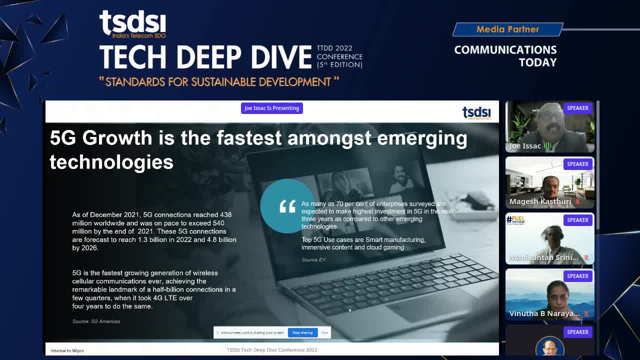 be it the retail, transportation and everywhere. I think 5G is the name which has been placed ahead, but this brings in a lot more of you know, a lot more of criticality from an application perspective, And when we know that 70% of enterprises want to move towards private 5G networks, 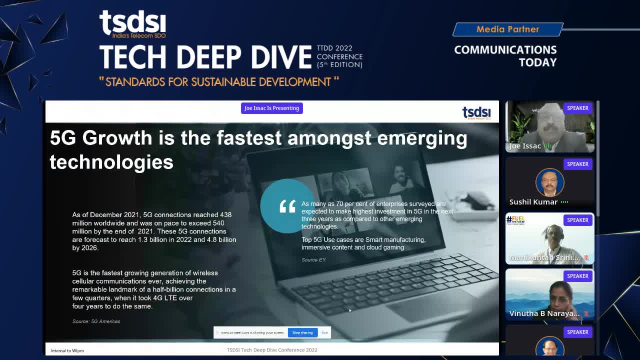 while there's a big investment being planned, how can we ensure that these can be secure? How can we ensure that the use cases, of the smart use cases, can be still manageable when it comes to when it comes to the whole ecosystem to sustain into one plane? 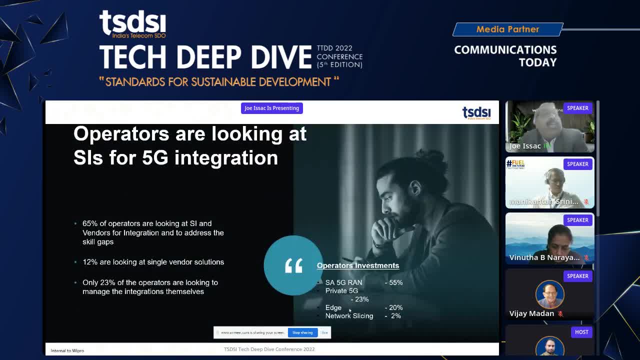 to a common plane. Operators, while are looking, you know, are looking to upgrade the networks from from 4G LTE to 5G, NSA and to SA. Some people want to do a direct SA but I've seen, I think, people doing NSA and initially 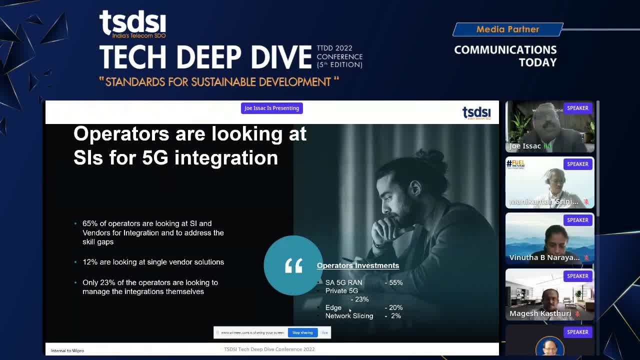 and then moving to SA. 65% of people, of the operators- are looking to move very fast and they're looking at to have people to come and integrate the whole thing for them, because there are a lot of skill gaps when it comes to you know. 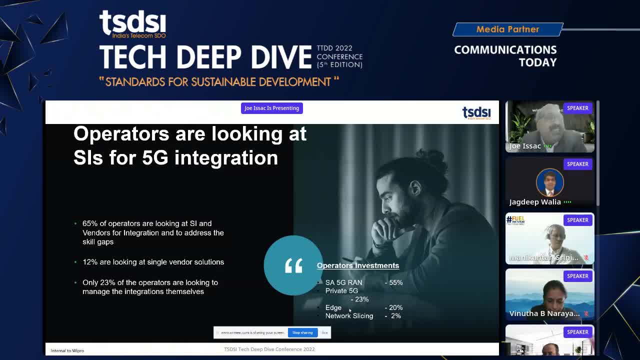 newer technologies, especially when it comes to 5G or another 5G, say a packet code implementation. or how will security play its role when it comes to package code implementations? How will the front door, middle door and back door have its play to ensure that they're not susceptible to attacks? 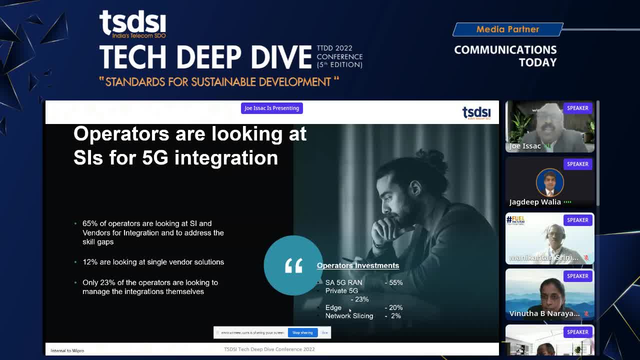 While there are about a few in the last, I think, three, two years or four years, with the open RAN concept coming into the picture I think about people are looking at. there are some few companies who- few of the operators who want to run a single stack or monolithic stack kind of environment where they have a common vendor. 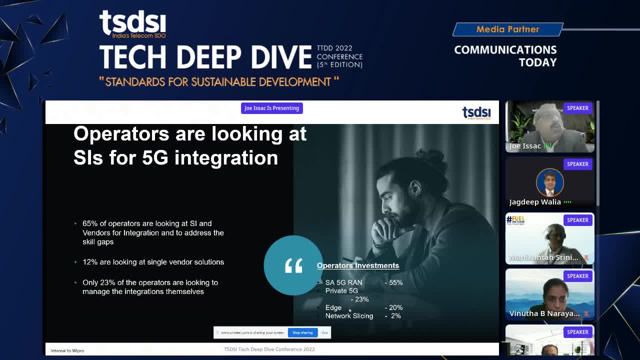 But the larger, larger perspective is to have a open architecture or open technology where they have various different hardware components coming into the same plane, because standardization was standardization. I think about 23% of operators are looking to manage the whole thing themselves, while there is criticality in that of how they are able to manage the whole security. 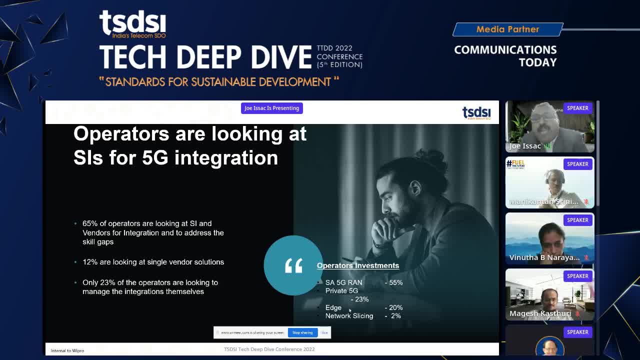 I think, from a 5G RAN perspective, I think a 25% of investments already operators are putting in today worldwide. globally Private 5G has been 23% last year. It's short to 36% as of July list this year. 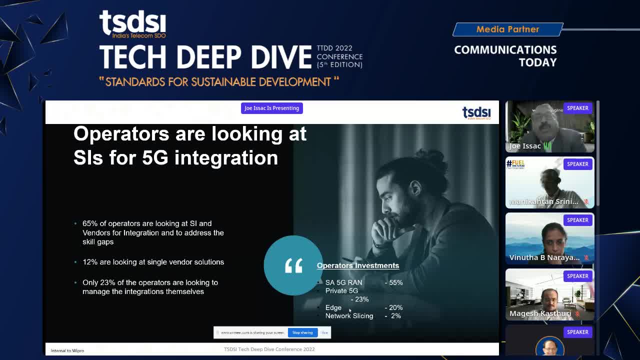 We're seeing edge becoming very prominent and edge growing beyond just the 5G edge. It's also the 5G edge cars, for example, the cars going cloud car, And so each of these car systems are like an edge system. So the network slicing plays a key role from a 5G perspective. 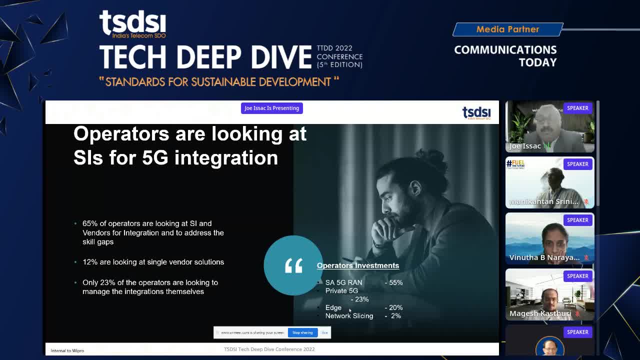 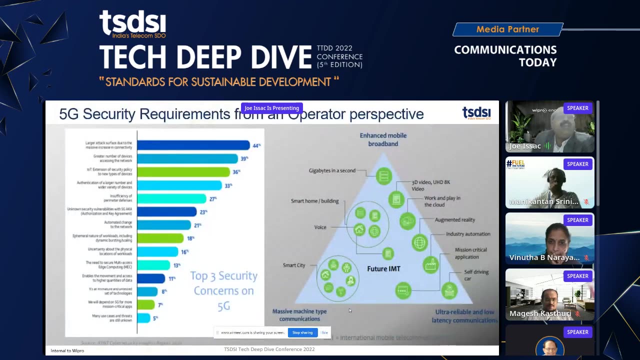 I'm able to secure the whole protocol using instantiated individual UPF, SMF and AMF, for an instance, while there is a proper control and security. as such, If there is one slice being hacked, I can still bring it down and still have the other slices running as normal. 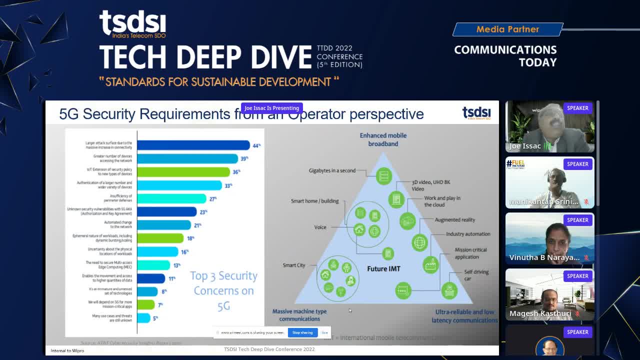 From a from a list of the security requirements or the larger spectrum from operator perspective. the last, the top three requirements, I think, which are concerning operators, are that larger attacks on the surface due to massive increase of connectivity. Basically the 5G radios accommodate more users. 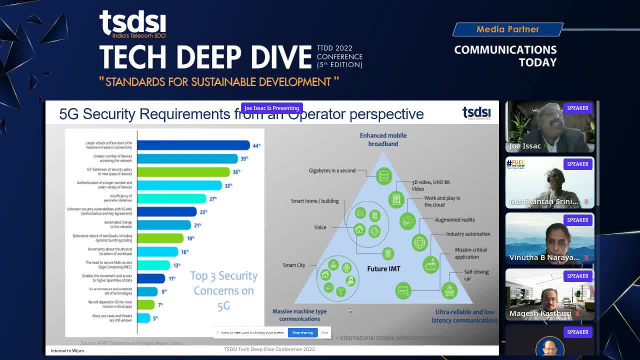 more dense. they're more susceptible to carry more dense connections and hence a larger, larger amount of connections, leading to more unsafe environments. Second, that the number of non-passive, or the passive or active devices on the network, as it has gone triple four to five fold. 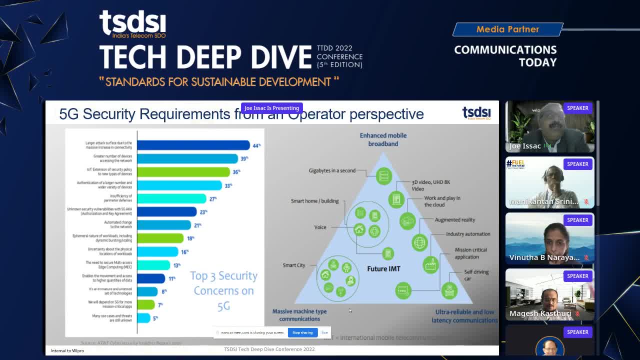 they've gone with that, with your MTC protocol in place, with the sensor networks going live, with the items, going live with most of the wider networks on Azure and IoT- the free free platform example, where there are a lot of integrations with associates on board for cloud car environment or even for sensors for manufacturing. 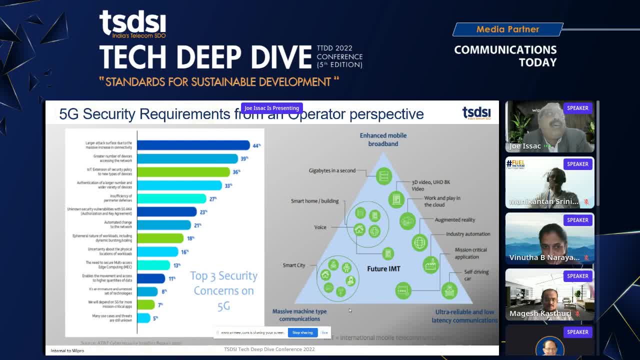 I think there's a huge amount of of scale up happening there on the, on the devices, from a manufacturing perspective, transportation, logistics perspective. I think that that I think is forms of who bulk of traffic beyond that to carry the whole thing across. the third: 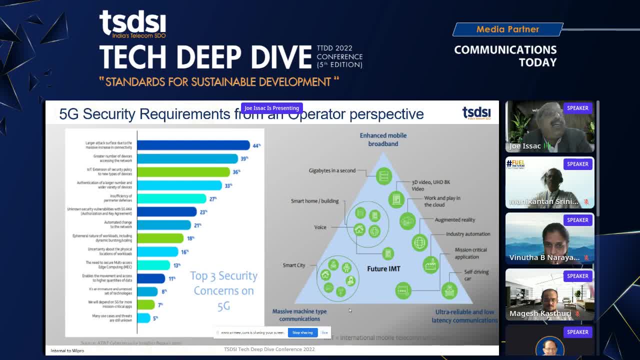 I think the most. one of one of the top three concerns are the: how do you manage the entire IoT extension security when it comes to newer devices? You have new protocols on IoT is going to take place, and most of these are pushing them to go to the cloud and making their aspirant to it. 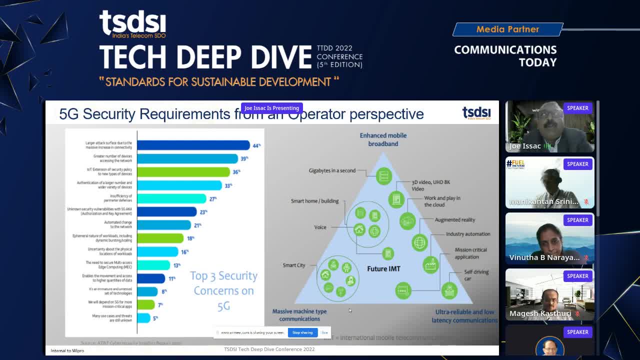 Right, Right, Right Right. I have not covered much in the cloud here, but just keeping my focus only on five G security as such. There are a few more like example. There are so many unknown security on vulnerable when it comes to why, Jacob example, when it comes to authorization, manual attacks. 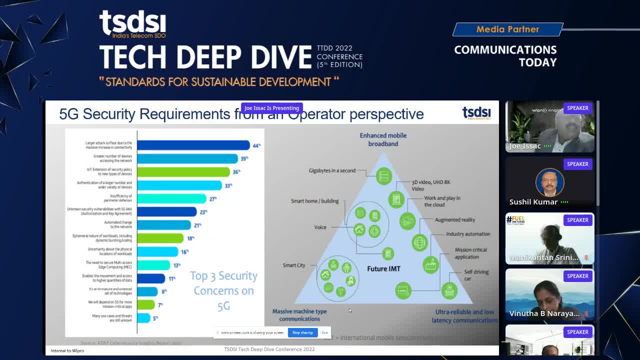 How does DDoS play, How anti DDoS plays an effect here? There are so much of it, I think. when it comes in, I think I took the top three only, but you see the whole percentage I think between that itself comprises something about 60% of the whole of this. 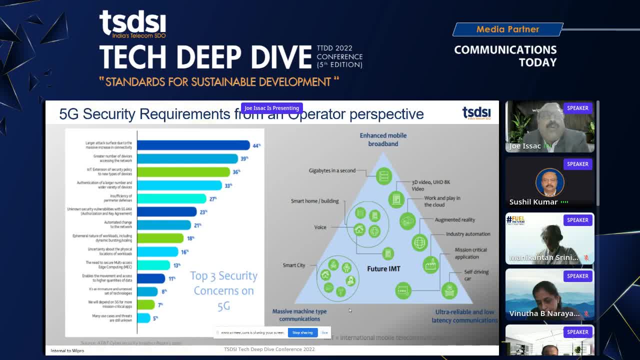 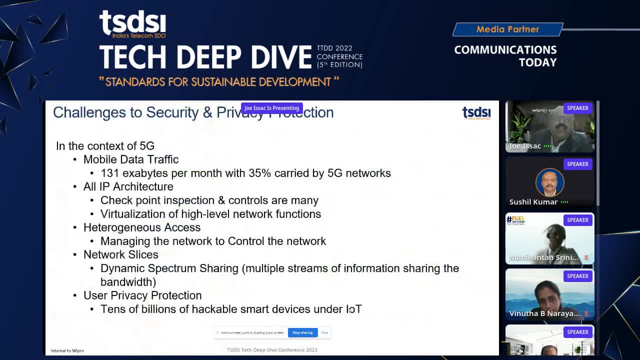 I think that's and that's the area I think we're looking at. How can this be? How can these service be made as simple as possible to address from my perspective or your perspective or perspective? So some challenges I think what we see are in the context of five G data is that the mobile data traffic patterns have been pretty high and most of the of the networks today care are carried of the data networks carried out by the five G networks. 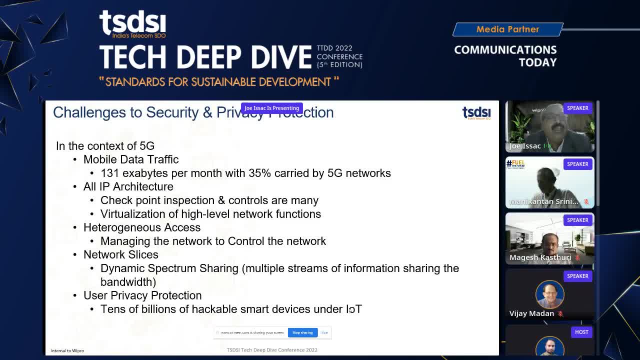 All in all, that there's a huge transformation: The one, the virtualization on the, on the softwareization and continuation of the networks, which brings in a lot more complexity from a checkpoint perspective. The control points are many and virtualization of high network functions make it even more tedious. 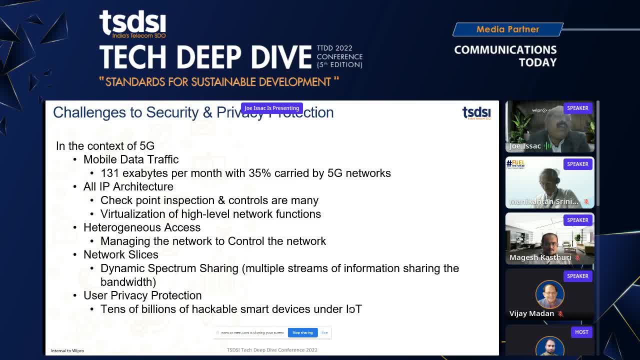 There is a lot of homogeneity and heterogeneity within the whole network. managing, trying to manage it to the networks is not easy, especially when you have, when you have, multi vendor environment within the whole of this ecosystem with the, with the EMPB 5G slices or the MMTG slice, or you are just slices and 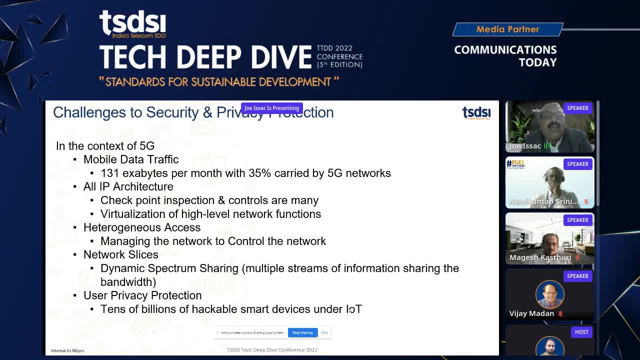 you have multiple networks. So all in all, in this kind of context we are able to actually make use of dynamic spectrum sharing, DSO kind of environments where multiple streams of sharing- I can actually share the radio spectrum itself on a five G and which actually throws out even more problems when it comes to security and try to manage the front hall becomes really difficult. 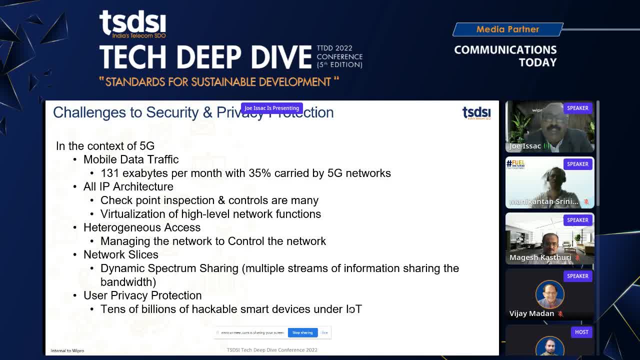 And how can we make sure that these standards can be addressed? Your privacy protection is another big area which I think, which I think is playing a bigger role, even more complex, when it comes to European places like Europe, where your GDPR restrictions as well. 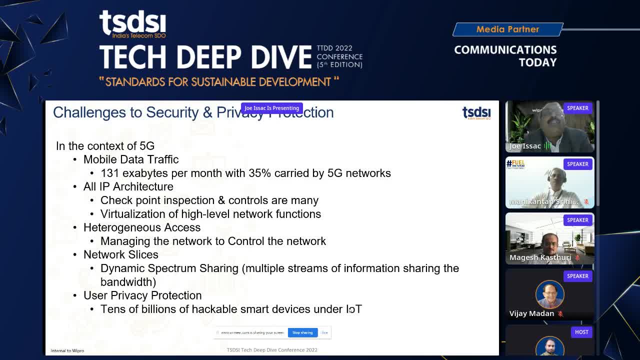 right. well, how are you going to make it context sensitive? how are you going to become sensitive? right, these, they make it even more uh. you know outreaches, i think, when it comes to uh challenges there a lot more packets, a lot more, not billions of hackable devices. you've got your smart classes. 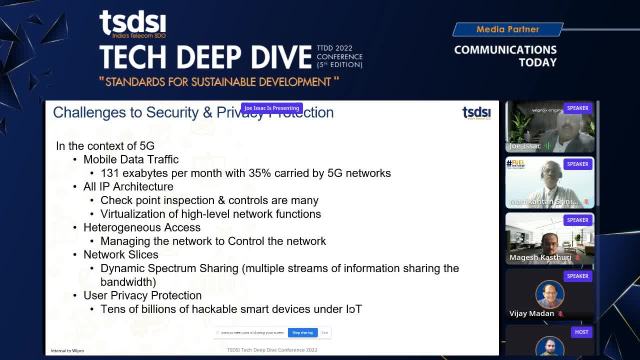 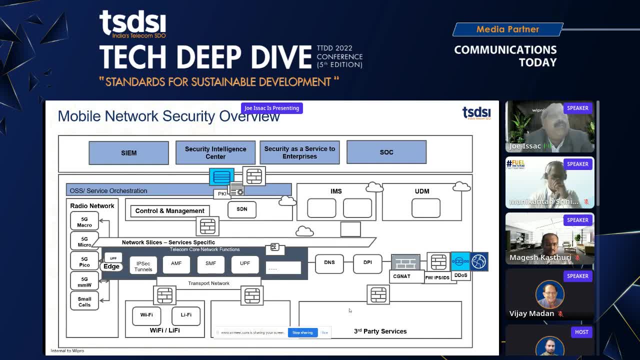 you know name, name it and everything is on the world is actually enabled on this whole platform which runs on this 5g network. from a whole life perspective. when i look at the security, information and even management right, there's a lot on the on the top most layer that how will? 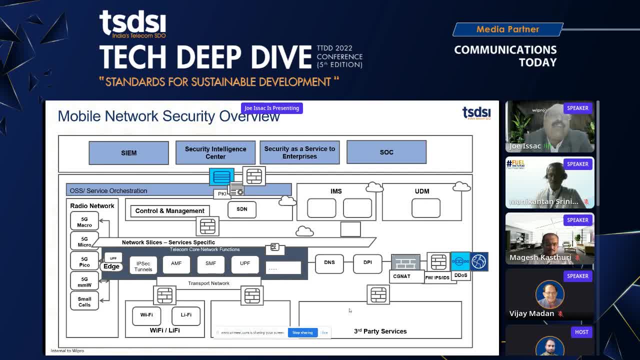 the security pattern, uh get, i get itself identified on the whole confidence. how can these components get integrated in a part of each of these um, in the orchestration layers? how can the rig controllers ensure that the the respective protocols, the respective underlay tunnelings are in place? how can we ensure that these tunnelings, while in place? 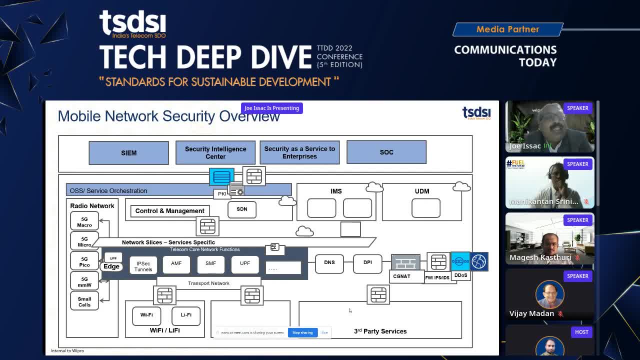 uh, do not still load the network right. these are some big time questions left there. there is no other means other than going with an ipsec kind of tunneling environment. um, which is which is what 5g standards also drive towards when the the bd, the ts35, 501 or 3333.310. 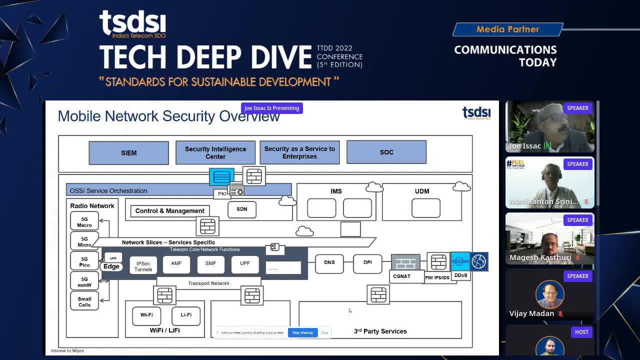 or the ts 33.210, all of these driving the whole 3gpp towards the 5g security uh perspective, i think, with more of these being virtualized softwares and containerized the subs, the it's, it's, um, it's, uh, it's throwing itself to be more susceptible to the whole world, while there are a lot of good. 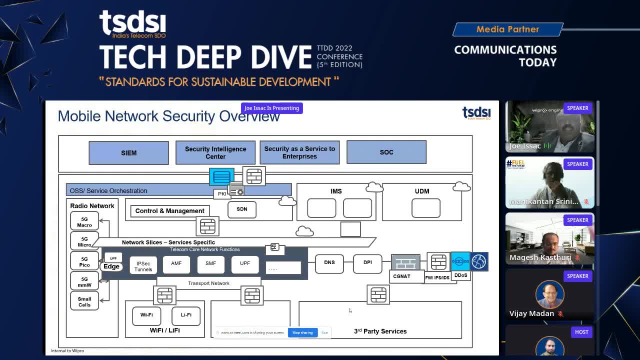 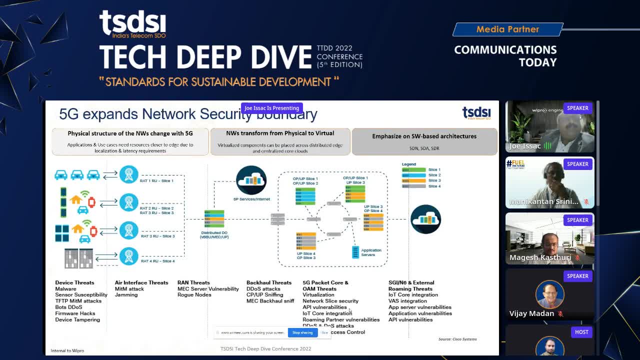 and bad elements on the network which needs to be controlled in some form or another to ensure that we have a seamless way of integration from the whole enterprise when we expand this whole uh, the whole security of these uh, of this 5g network security across boundaries. i would like to cover them in three areas. one has the physical structure of the 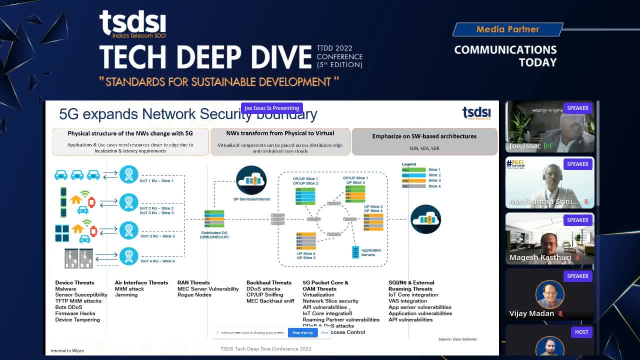 network change within the 5g, 5g specs, mandate for virtualized, virtualized software and contrast kind of workloads. uh, while earlier do not continue, but now i think the whole whole thing is going towards the virtualized environments, even more complicated, that most of these are moved from private data. 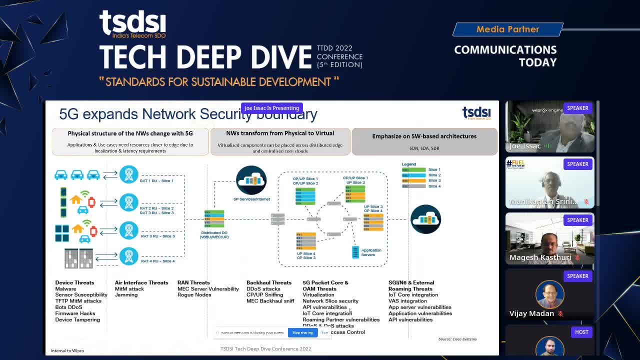 centers into the public cloud- uh, either hosted on azure networks or or an AWS network- any of these, which was even more challenges within um. so it makes it even more easier to easier to actually adapt. so i'm able to actually connect from anywhere, so i don't really don't have to have 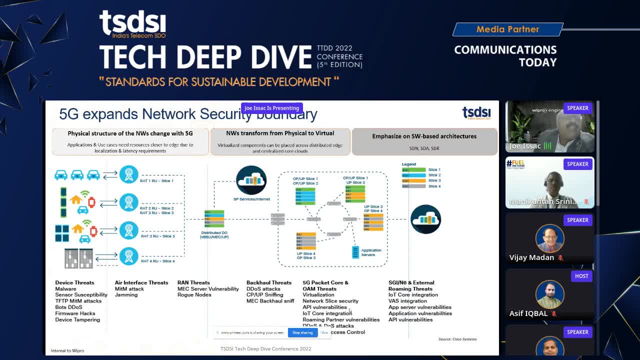 most of these components in my premises i'm having a sas based availability, with slicing being very um service perspective, uh it. it throws up a lot more that, in terms of device threats, malware like malware, for example, sensors, for example, tftp based manual attacks, how do you stop bot based ddos? 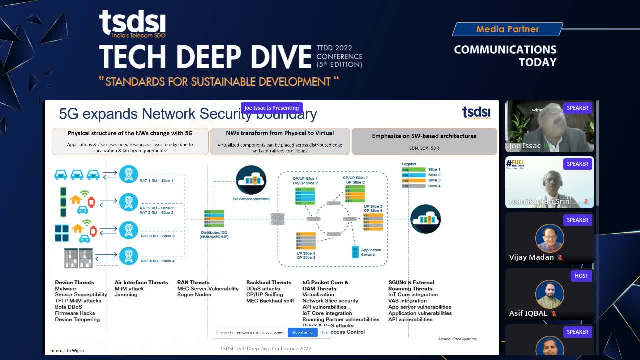 attacks on the device, um, firmware hacks, because mostly software defined radios are- are upgraded online, and then um, there will be areas where cert notifications, i mean they're pretty pretty, pretty much the same, but there's a lot of things that can be done to make sure that the device can be. 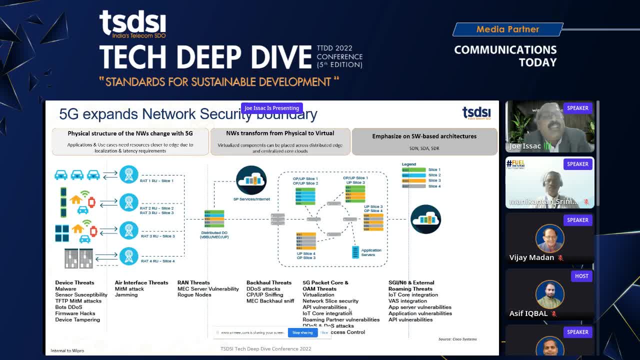 tampered or even 5g device can be tampered. how do you ensure that the whole, the air interface attacks um can be stopped? i mean you can have jamming on the network itself. this jam, this jams can, can come from a simple iot sensor networks, mesh sensor networks. right, it's very difficult to 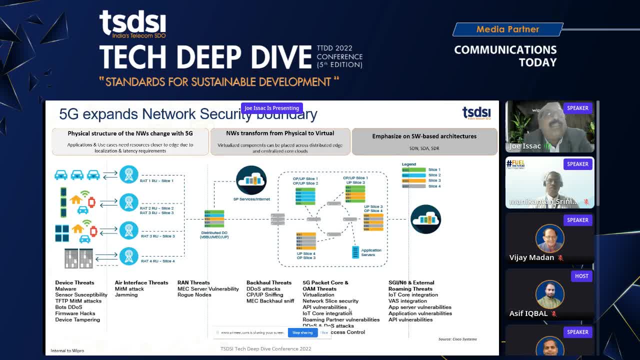 predict from where this would have come out. uh, one way of actually managing that is you have iot slices and each of these slices- uh, for each, each customer can be sub-sliced. so then you have a pfsm of an amf with a, with an nef part allocation to it, and you can, you can just softwareize it and 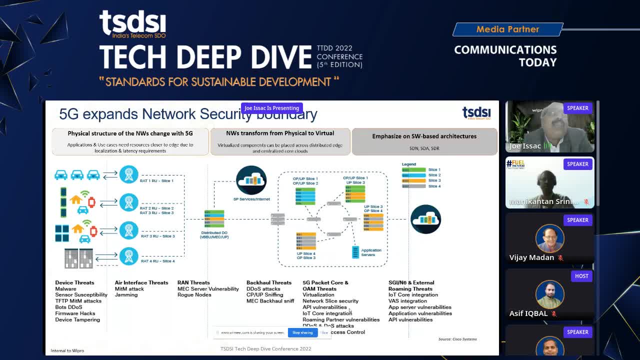 then uh, instantiate it and give it to that. so if there is, if you see some kind of um spurious activity, you're actually no, you don't actually uh down, hold the whole network down, but uh, only that slice, the sub slice, can be brought down and re-looked into it, or or the mall can be always. 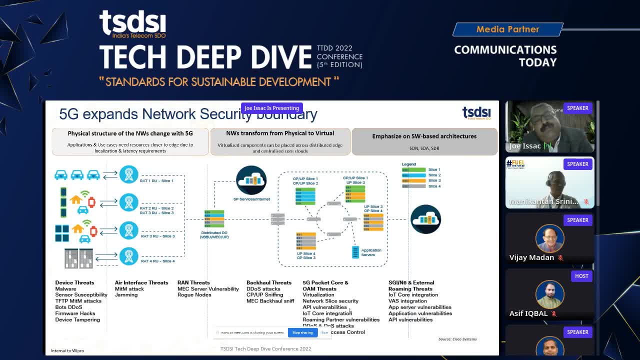 can be attacked through. second part, is that the whole part of that, um, the ramp threat which comes um, uh, giving that, given that latency is the core of the applications today. when it comes to 5g, we'd be a, we'd be a, um, a smart, um, a smart v2x communication perspective, or we'd be um. 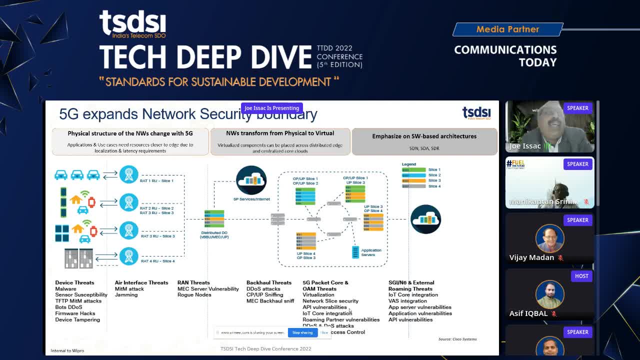 an application perspective where you have really low latency networks, like associates uh in the entertainment space or associates in the gaming, in the game space or in the car space, where they want most of these vehicles to be monitored. governments want most of these vehicles to be monitored. governments want most of these vehicles to be monitored and hence makes its way uh to have. 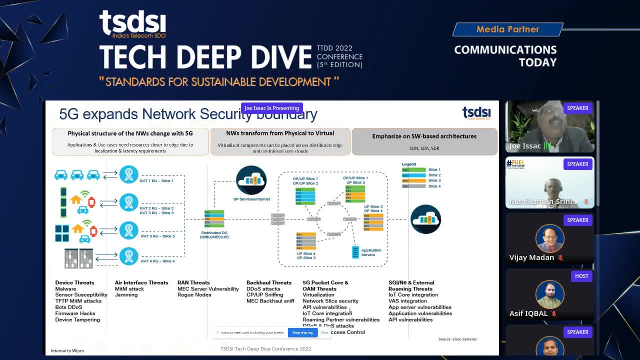 much more. uh. you know much more that the rogue rogue node elements will be persisting the network. how do you stop these kind of uh rant threats? there are a lot of black hole threats like distributed door ddos is quite common in the networks from 4glt. we've been seeing this to. 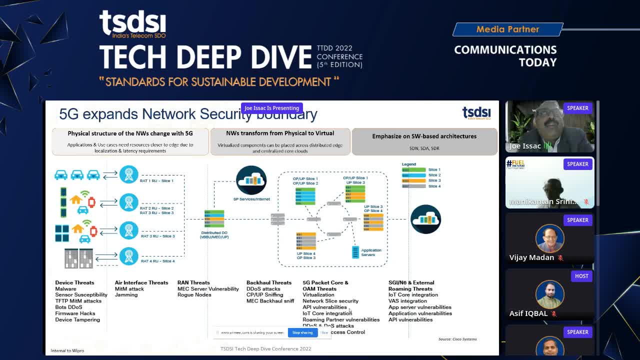 some good extent, i think, identifying as far as traffic has been uh, you know, uh, proactively stopped. how do you? you have no weight other than since, with, with the, with the uh, with the, with the, the control plane and the user plane being open, it is susceptible. 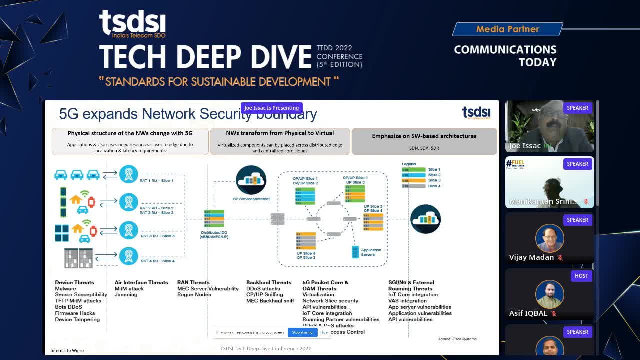 to sniffing And then how do you stop the sniffing? How can you do a backhaul sniffing? How can you stop that? actually, These are some of the backhaul threats On the packet core. I think you'll see, because of virtualization and 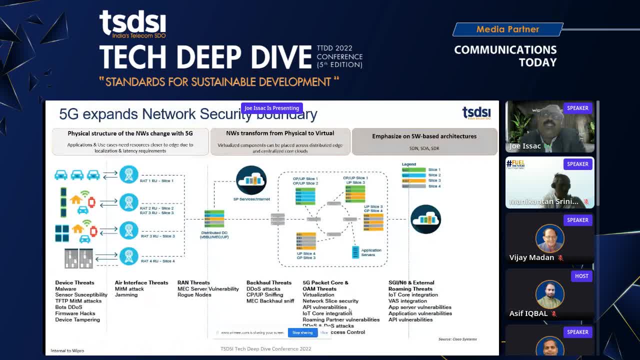 slice security being implemented. with APIs exposed, you will see a lot more APIs getting smurfed through the network. IoT core integrations with the cloud networks will open further more issues. While we may still claim that it's neat, I think within the protocol we need to have some kind of 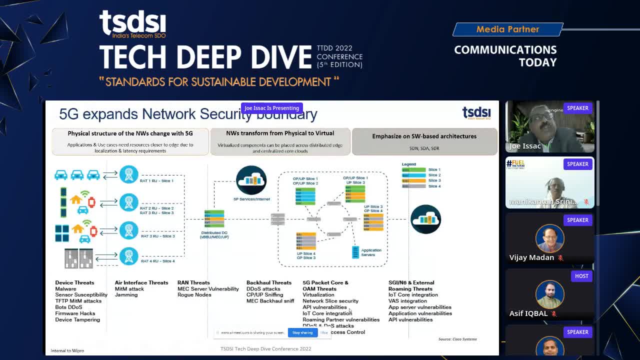 ubiquitous computing security plane to be implemented. How do you control the roaming partner, especially in the switch networks across countries? Just that you cannot stop at the HLA or the VLA, but within the protocols, with the SB architecture. how can I actually have? 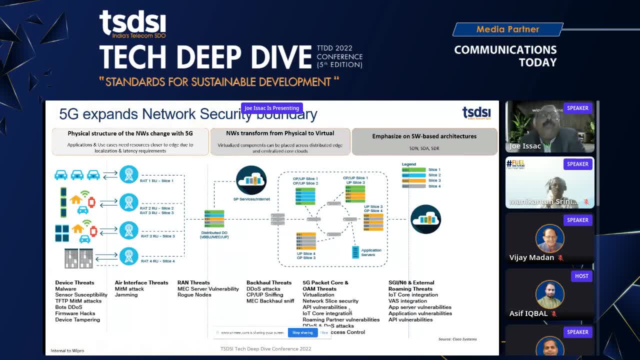 a security component implemented Well. not all may be on the 5G SD networks, but they may still be in SD networks, So you will still find SD interfaces. you'll find vast integrations from legacy still available, So this brings out a lot more. 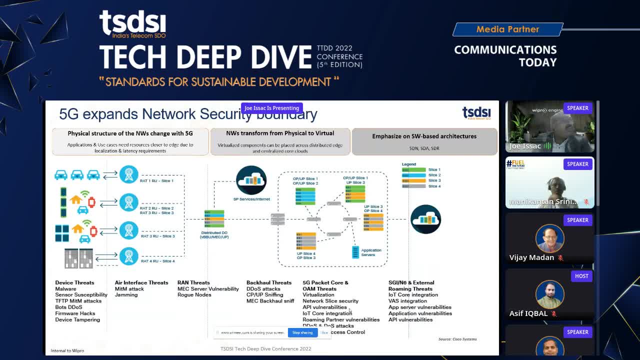 that the apps vulnerability or the APIs vulnerability will be much more actually stuff on it And more that you have software-defined networks running the whole networks. you have things like strategy deployment agendas for your software-defined radio networks, With the radio networks being software-defined, which means that 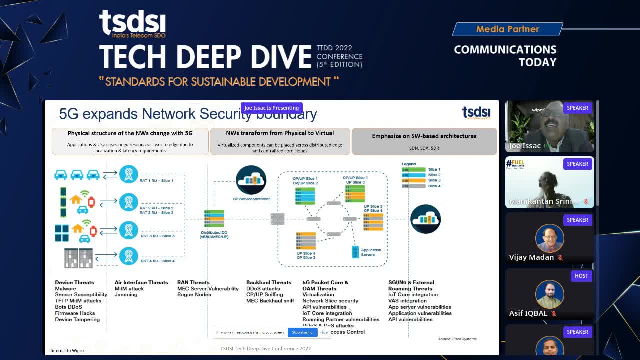 all the changes will get as they make a beta release every three months, six months. you'll see SD platforms. they'll want to upgrade and check how things work And these form the whole base for the whole security networks to be threatened off And how. 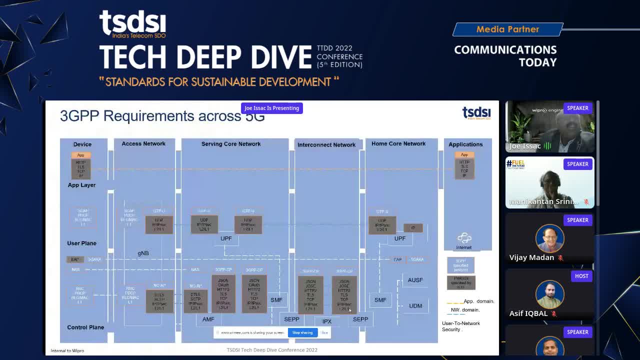 do you ensure that somewhere you can actually form some layer for this Across? you'll find 3GPP requirements. you'll find IEEE requirements, for example, requirements like your datagram transport level securities or your stream control transfer protocols or your you know. 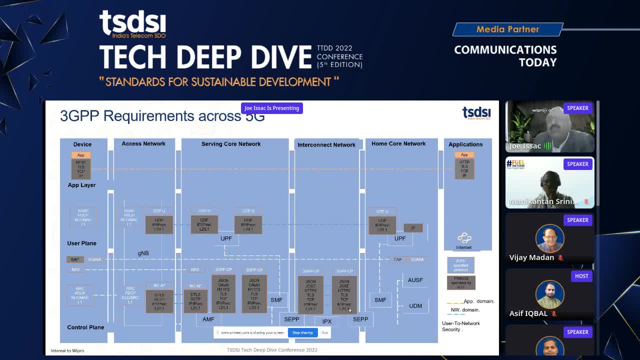 the Java object, data encryption systems, geosystems, for example. All of these form a layer of dependency, form a layer of overhead. when it comes to this tunneling, I mean you're trying to ensure tunneling between the user plane. 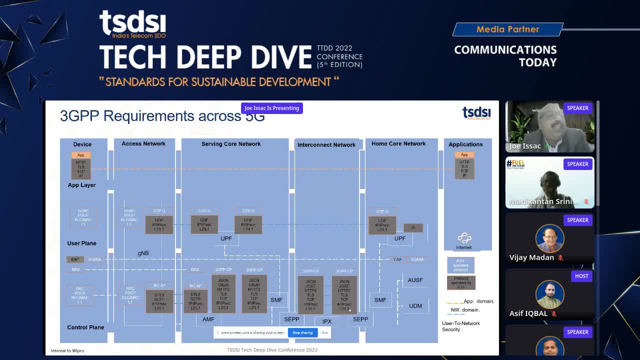 or the control plane? How do you ensure that you still have efficient communication between the radio networks from the front hall to the back hall? How do you ensure that you are still able to virtualize the whole of the packet core and still have them to be served to the whole network domain? 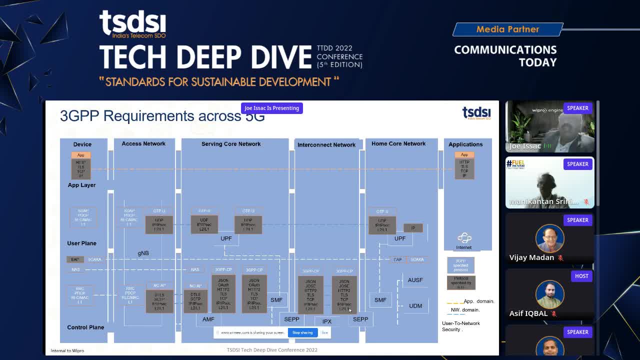 In a manner that the user to use the network security is still safe, while network to network have still have the flexibility to cooperate within the secure networks. there You may still have some kind of secure mechanism, but most of the secure mechanisms should not be an over it to the whole. 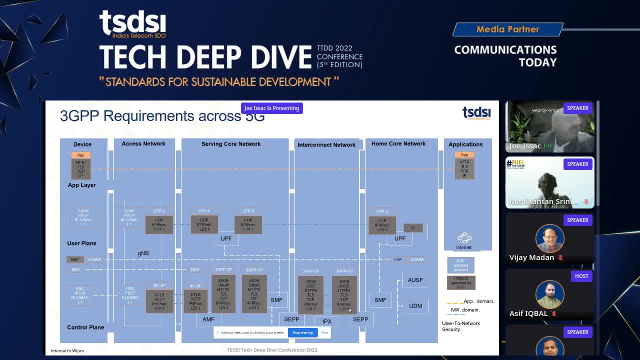 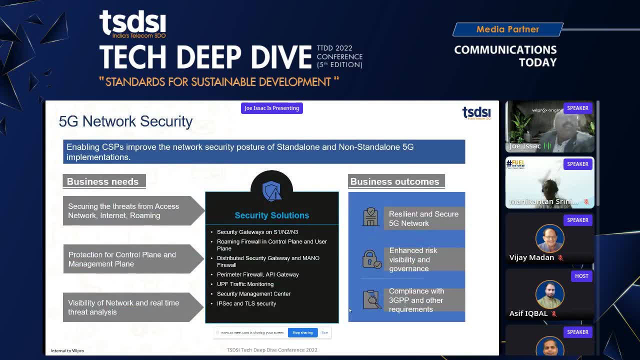 network And that I think from engineering standpoint that needs to be ensured to make sure that we don't lose much on this From. I think I covered three. I will try to cover three or four slides on from a security side. What is the business need? I think the whole need. 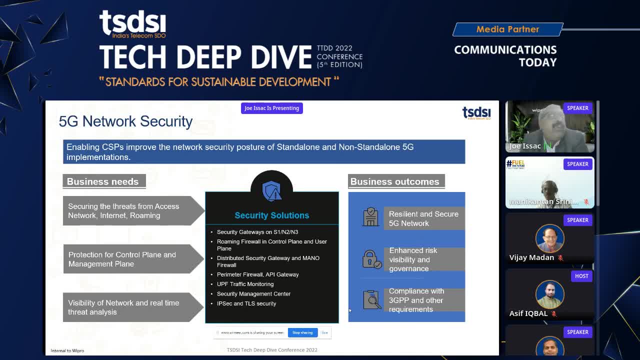 is to ensure that we don't have threats from access network, especially the, the two, towards the radius of access, the, the access segment, especially the radio networks, to the macro radio or the or the micro radio cells. How do I stop that? How do we enable, how to ensure that the roaming 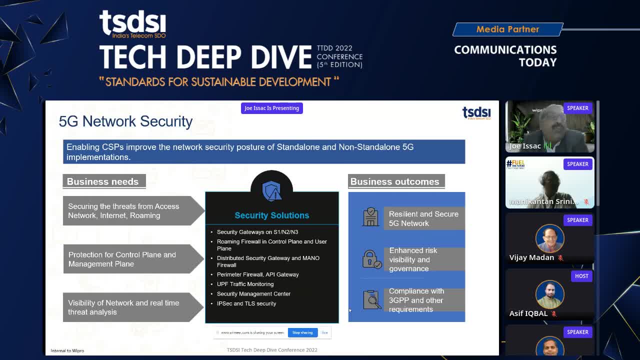 between big cells, There's no issue. when I have a switchover from network network, There is no much issue. I think that's one of the critical needs today, as our own date: How do we ensure that there is the control plane and a management? 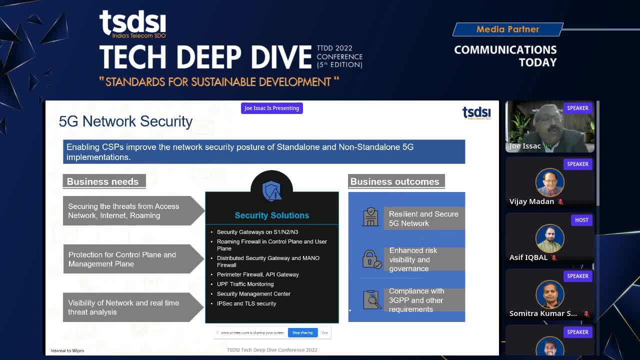 plane Security being being coexisting to ensure that there is development across the whole ecosystem. How to ensure that the visibility network and real time threat analysis comes to play. Why we want to ensure a resilient system. We want to ensure risk free visibility and governance. 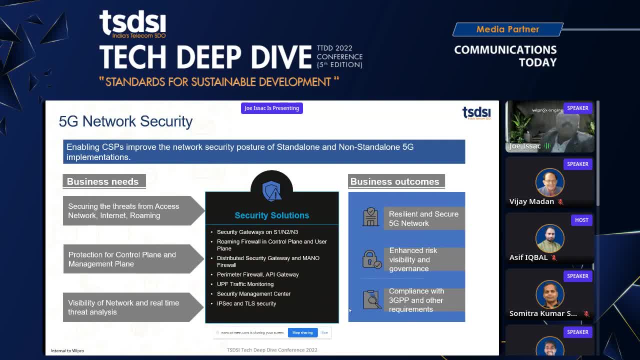 We want to have three to five standards to play their role there. Some things like, for example, having a security gateway on your, in your FIG NSA on the S one plane, or end to end through, or or N nine planes. for example, implementing 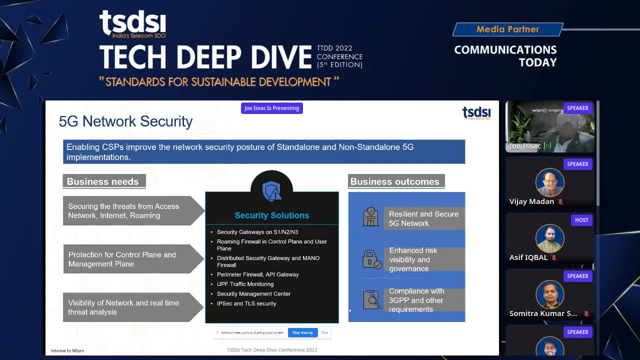 off virtual firewalls on, say, a parallel to firewall or something One of these which you can have, a virtual plan, virtual on the virtual in the control plane. orchestrating your needs through the firewall instead of actually directly orchestrating gives you more control. 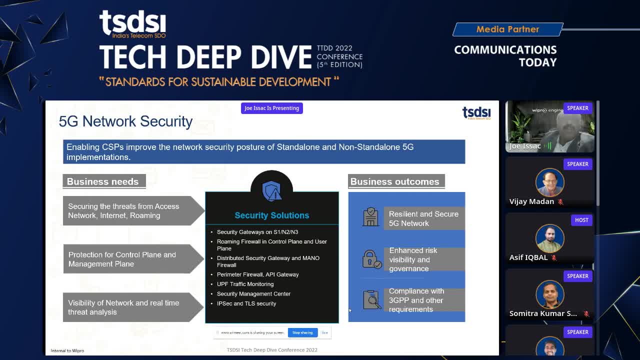 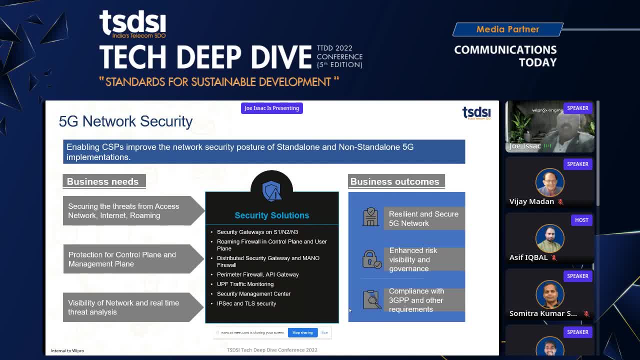 There are many, many different types of policies which should derive in an orchestration layer. Make sure it's. it is much more regularized. Why do you have layered orchestration in FIG use? use a time that we look at choreography based implementations, where you have even 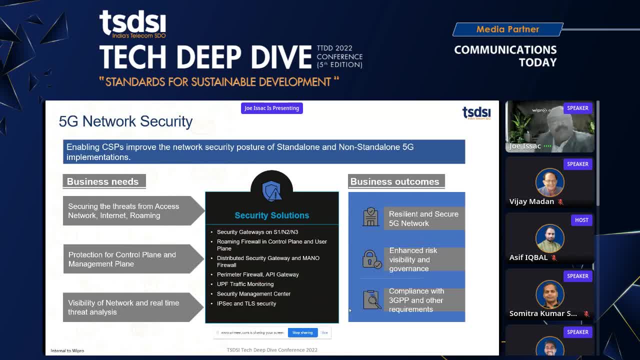 more control beyond, beyond the or the Person. I purple, How can I look at that thing? I people, six is looking IP, The, the 16 network is looking partly at that, Given that we have a certain type of integrated Parliament. Yes, yeah, So the different types of quality that the network network can be looking at. 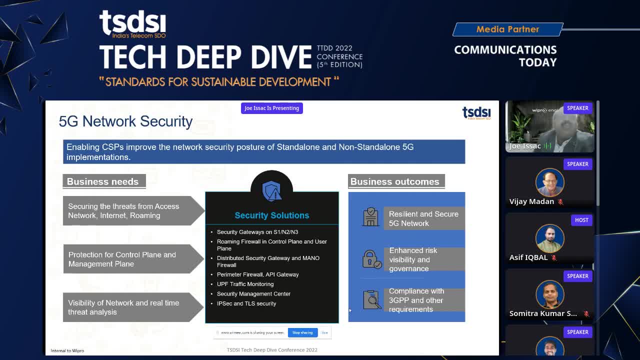 the different types of quality that the network is looking at, The different types of quality that civilization have, no other means other than TLS and IP security as one of the forms to ensure that you have security placed within the whole of the packet core or the radio infrastructure within. 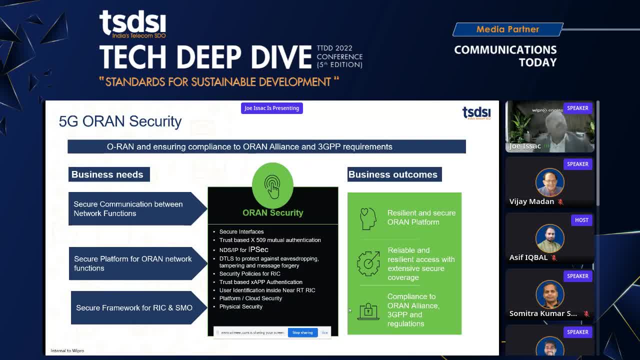 the network. Second, I think the next susceptible part is the overrun part. I think You'll find that you need to ensure that each interface- the E1 interface or the F1 interface or the E2 interface- needs to be secure when they communicate. 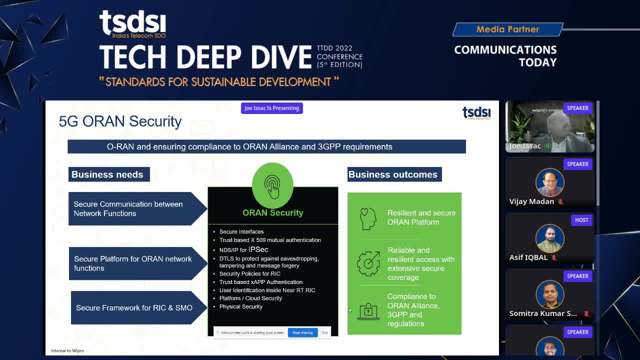 with the packet core protocols: ensuring that there are mutual authentications between your certificate-based authentication between the networks. ensuring that you have datagram protection at all levels. ensuring that you don't have manual attack. ensuring you have trust-based protocol within the exact thing. 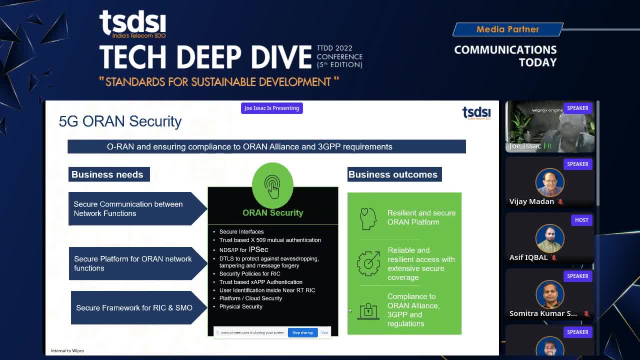 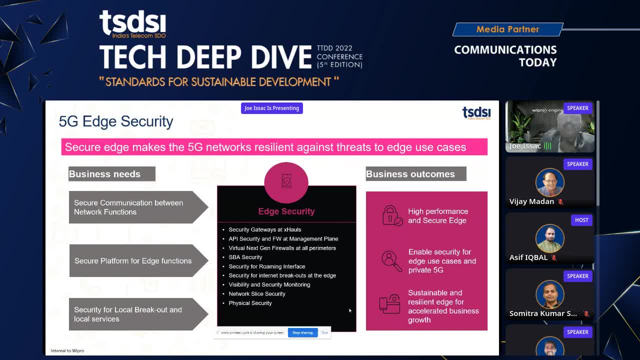 and trying to get the security of the whole cloud and land Overrun systems. half of the systems today are running the cloud and remaining on-premises of the network. Edge plays another big role in 5G and I would ensure that most of the 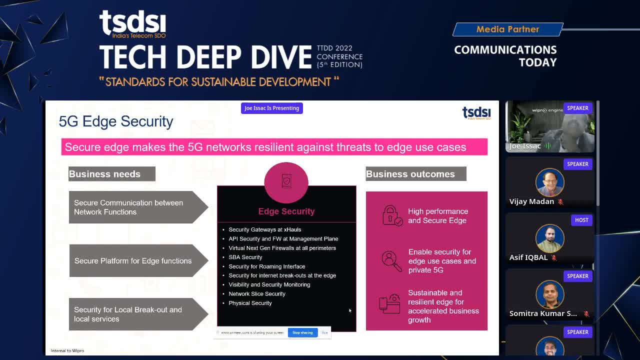 dynamic orchestration is going towards edge, like the movies, for example, wherever you see, things like, say, T20, Imagine played people watching streams and then they are able to push this entire stream to the Mac and then stream it from there to the nearest user. I think it opens more. 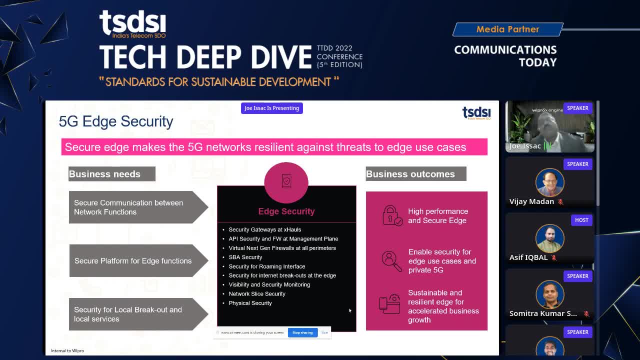 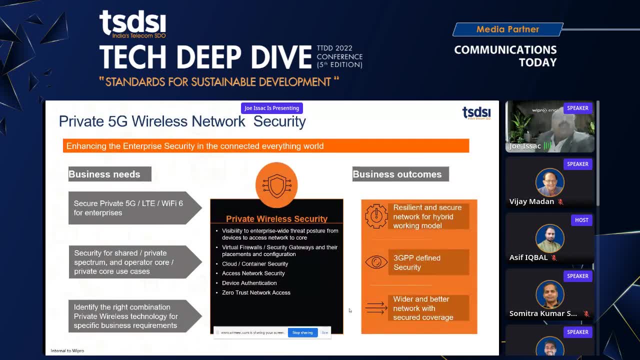 for the roaming interfaces. it opens more for breakouts, F3, big codes or how do you ensure that security? these are the areas I think roughly you can see that. how can you manage out something around? the private 5G network is getting even more critical, I think, with mass adoption. 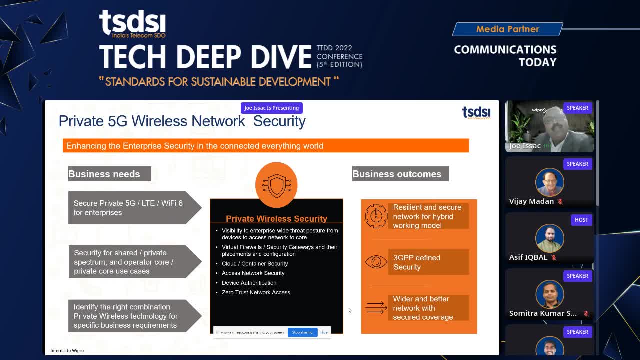 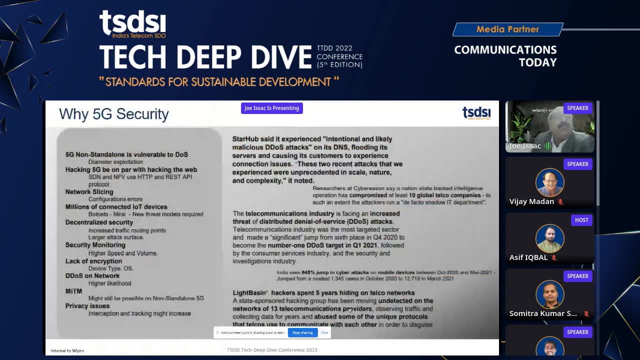 of private networks from operators. I think there is some amount of trust on that. This is gaining its importance. I think. more than India, I think Europe is actually going big way on private wireless because of your factories getting automated big time and it's causing a bigger challenge. 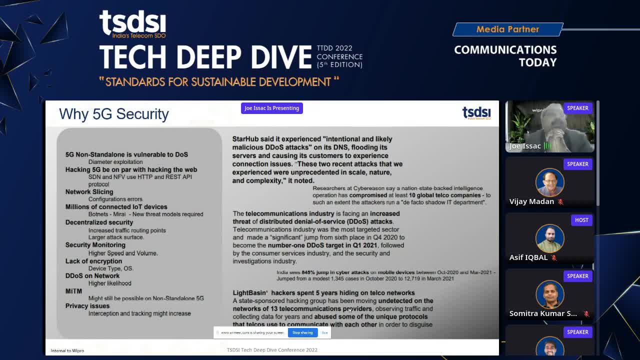 there Some things like, for example, how do you ensure that the NSA is not susceptible to, or not vulnerable to, DDoS, for example? Hacking is going to be as far as much as the net today, I think with more of. 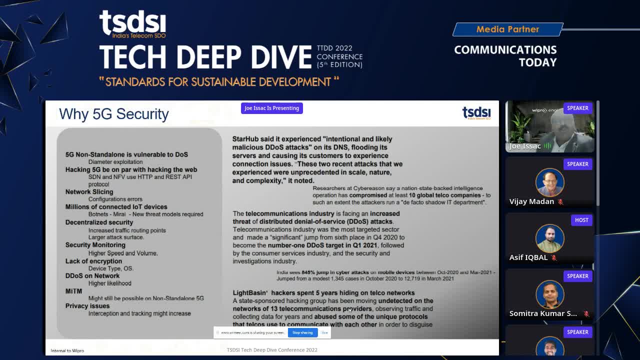 TLS or HTTP to secure protocol communications. I think you're able to control to an extent. Slicing configuration errors can throw much more of connectivity problems, of attacks where these slices can actually give up by DDoS attacks. Millions of IoT devices have been connected and rebuffering back. 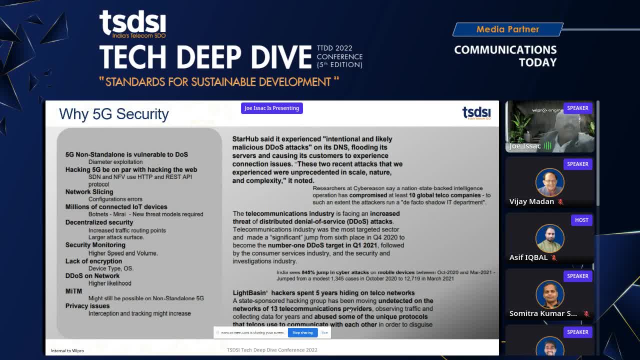 onto the protocol leading to traffic on the routing points. I think today, with some amount of networks in, you can actually drop the packet. but then, from a third party perspective, how much will users be okay for it? There are some of these areas. I think we'll look at it. 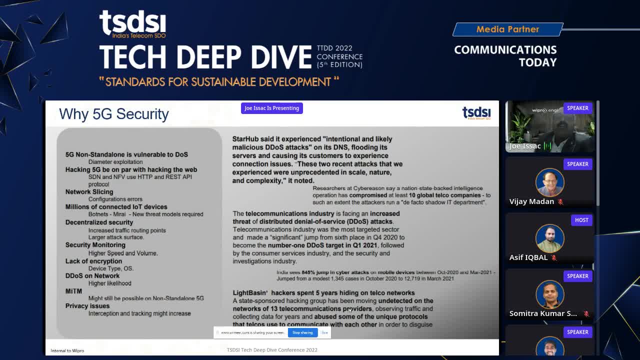 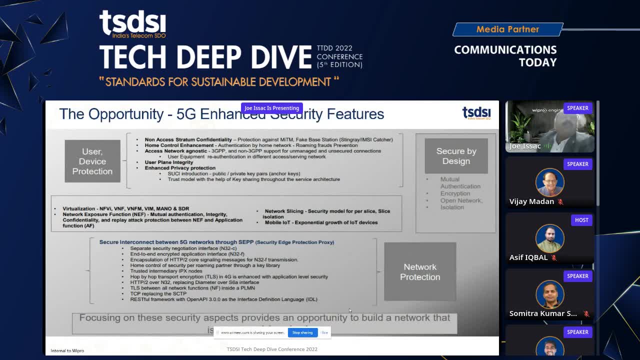 in deeper. There are a lot of people like startup who made comments about how they should look at all this and what are the kind of areas they bumped into. This is all throwing up a big, big security feature list for us from a non-access stratum confidentiality perspective. 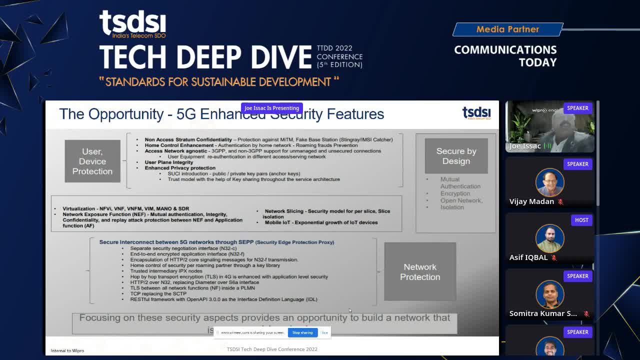 from a home control enhancement perspective, from an access agnostic network. If I have to have 3GPP and not 3GPP support from unmanaged or unsecured connections, how do you manage it? How do you ensure that the user plane protection versus the control? 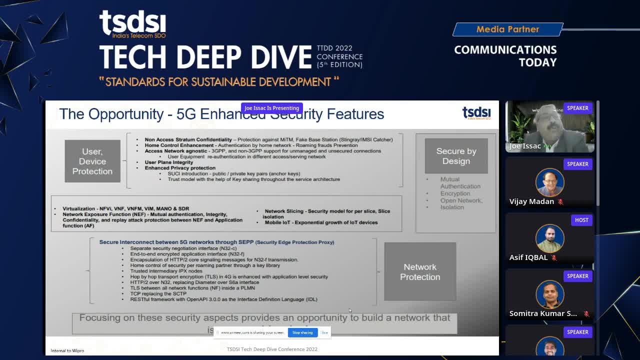 and production integrity is enhanced. How can I ensure that the private protection from a public-private key anchors or a trust model anchors the whole thing out? There are a lot more, I think from a secure, I think from a perspective that how to ensure that the security? 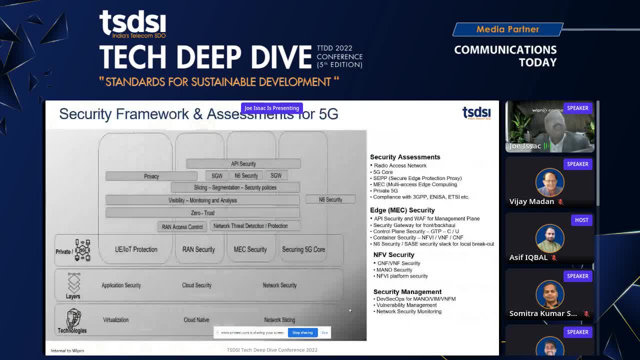 protection proxy can ensure that a lot more things are placed and we can extort. There are some kind of assessments like the radio. there are these mandatory assessments which we do typically for operators from a deployment perspective. We try to do the radio access network. 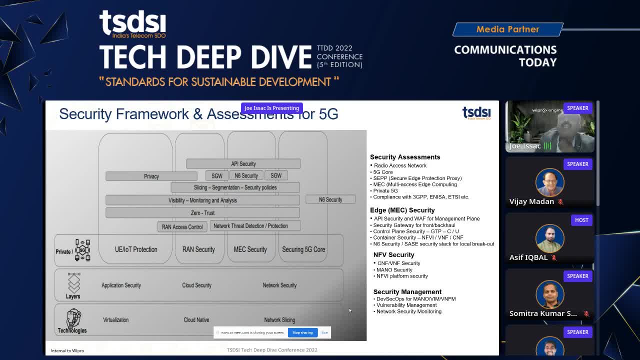 assessments- and these are continuous assessments of 5G packet co-assessments. on the protocol itself, We flash that, we strip the packet and see what happens at the MEX side, the APS security side, The WAF planes are even more complicated, I think, when it comes to. 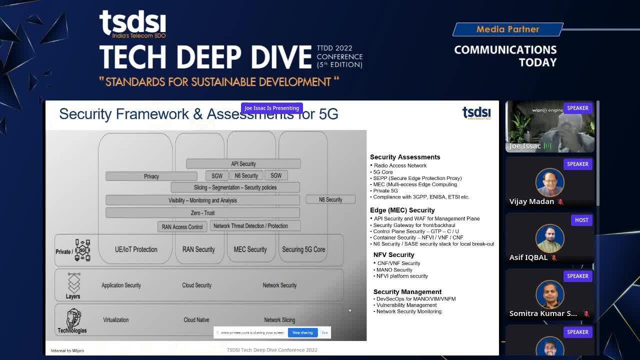 apps because of proxying, but you still have control on it. You have some control plane. the tunneling protocols and the control on the user plane gives even more some amount of padding. but I think the firewalls will be very, very important. They have to be. 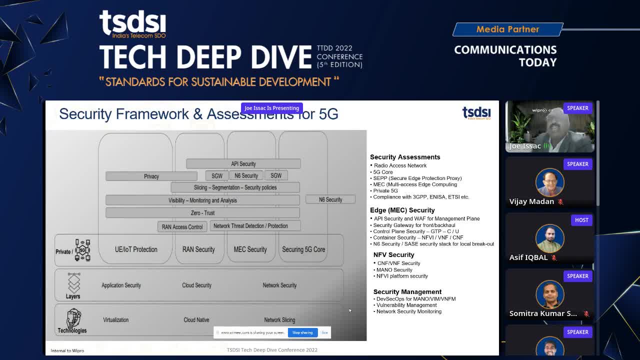 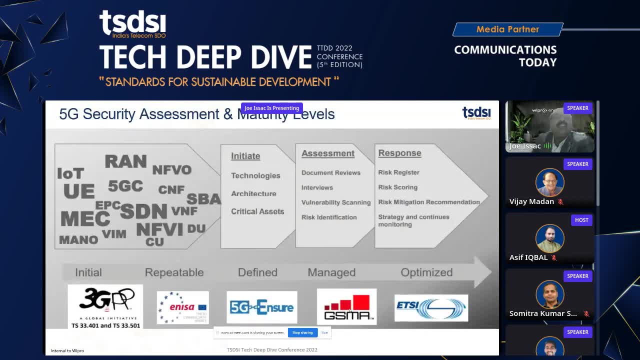 particular about viewing this. The N6 security, for example, as it breaks, gives out some old breakout features, but then it's still susceptible. I think you need to have an ID system to manage the whole of this thing. So we have a maturity. 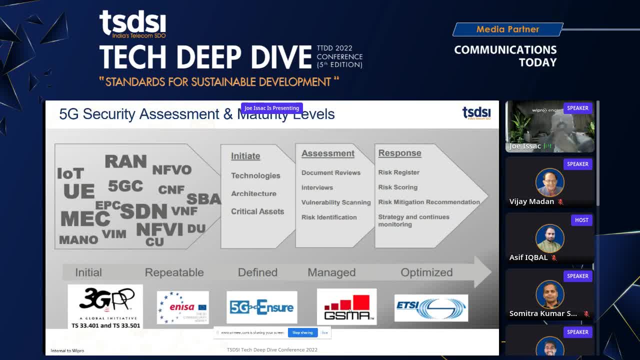 framework where you have which is repeatable, defined, managed and optimized. You initiate the assessment on the technology, the architecture and the deployment and the rollout You from documentation to interviews to one of the scanning, regular scanning at odd intervals risk. 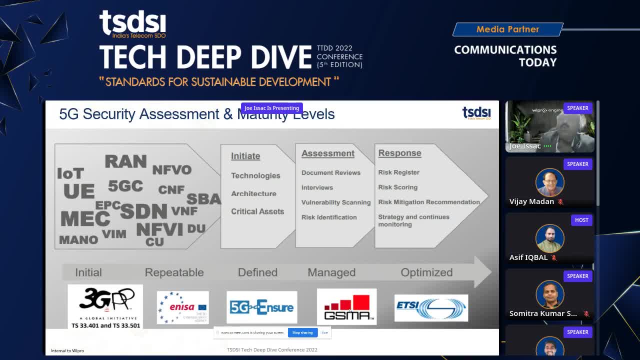 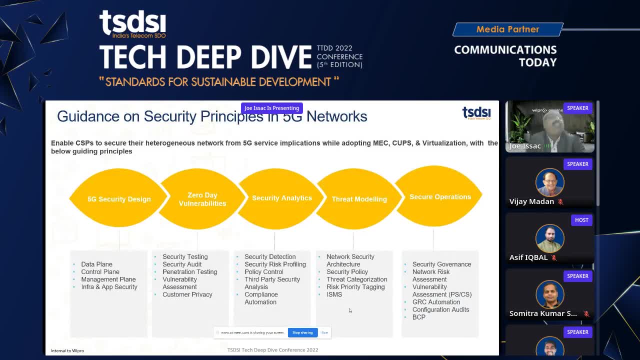 identification, moving the risk levels up on the register, scoring it and kind of managing the recommendation, and day by day this changes. So some of the guidelines there are: how do you ensure that you have a 5G security design on the data plane control plane? 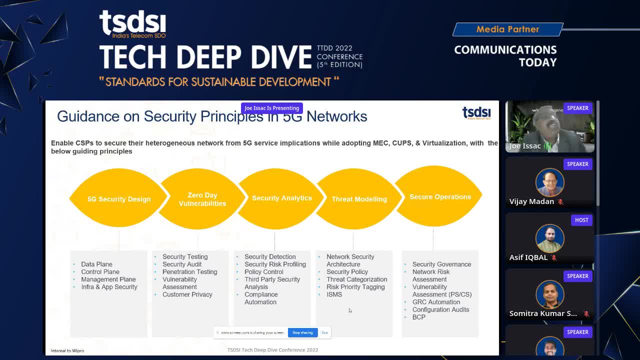 management plane and these three becomes very critical when it comes to managing 5G rollouts. Testing the whole security is again it's a round the clock basis. It has to be done in a factory as manner where you have an orchestration. 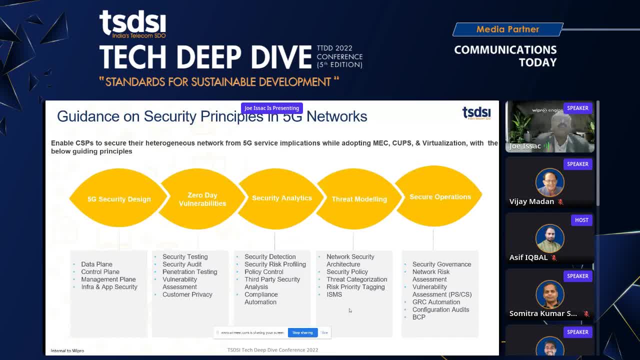 layer to manage the entire security audit, for example, or the VA assessments and probably checking it. I think these things are all moving to AI models and ends at much more precise. we can test out How do you do analytics and how do you re-thread this back to data science to see how the 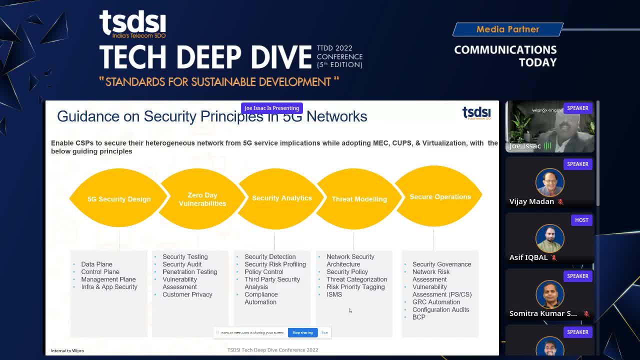 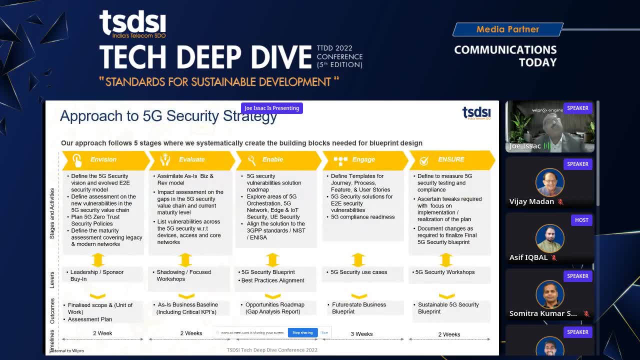 repeatability of these threats can be. How do threat modeling- on-the-fly dynamic threat modeling- and risk tagging it and then ensuring dropping packets there are due to secure operations around it? One of the approaches we use is to envision it, envisage it, evaluate it, envisage it. 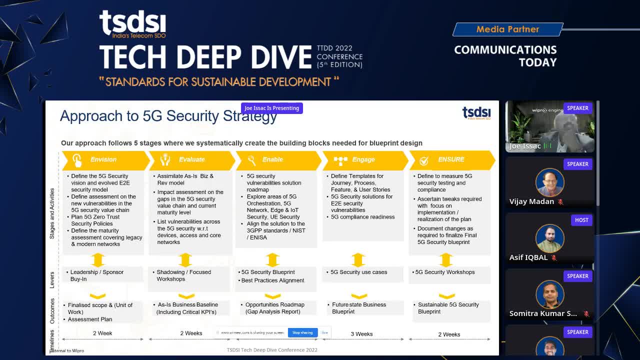 and ensure it. So this is the 5E model we defined, where we said that we're able to actually do some amount of visioning, some amount of evolved day-to-day controlling the whole thing, assimilating the whole access to rev model, ensuring that we are able. 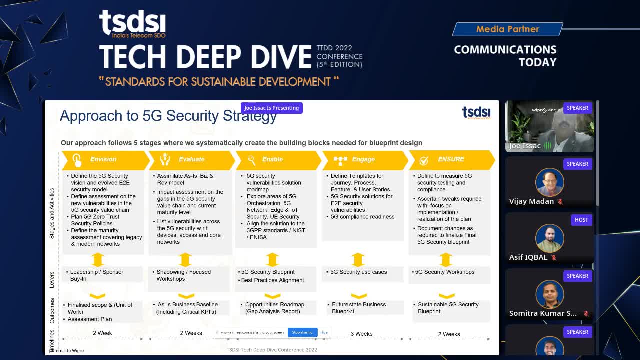 to explore areas within the 5G core, the 5G ORA and the 5G network steps within the whole thing and endangering with the standards- Aligned with standards- gives some amount of comfort because protocols are much fixed And then you're able to do it. So you need it needs completely. 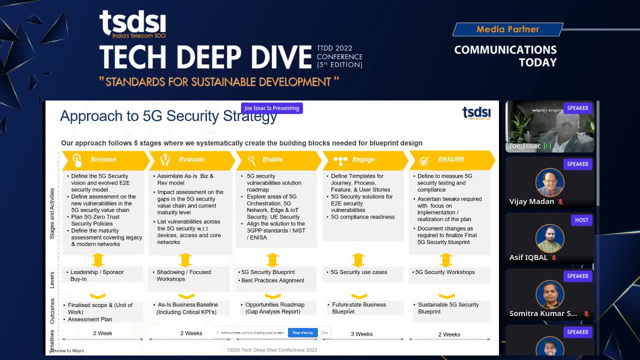 a sponsorship buy-in from the CIO office, the CTO office, which drive most of these. The 5G blueprints have to be updated every day or every week, given the risk assessments you go through within the whole thing. Some of the use cases which make its importance. 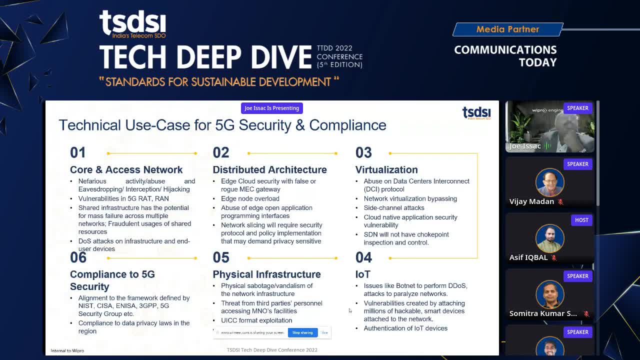 here are on the core and the access networks. You have a lot of these abuse happening on the network where you have eavesdropping, intersection, interjection, for example, hacking, for example, one of the 5G blueprints, the RAT or the RAN, the terminal or the RAN site Shared. 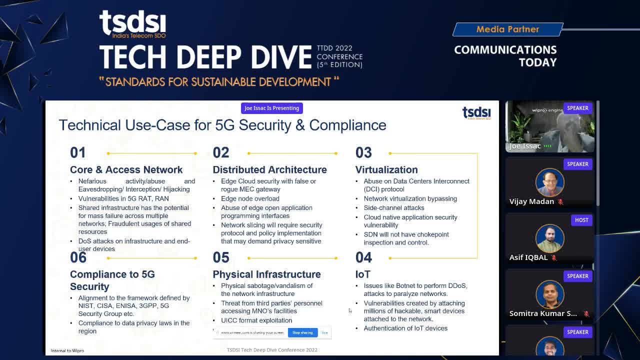 infrastructures have even more potential. especially when you try to do sharing of spectrum, you'll have even more issues at the access region, And then that's one of the issues. Second is: I think when you used to do distributed edge environment, especially after the view, then you need to be. 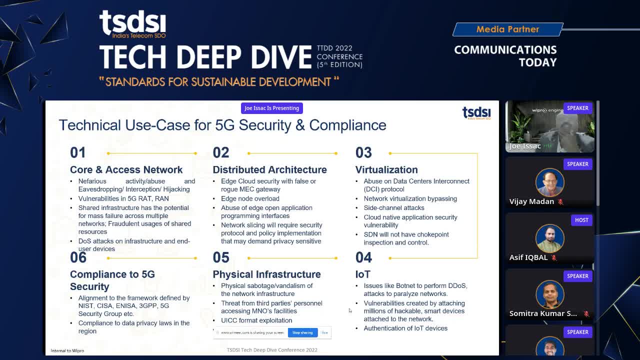 extremely careful of how the edge nodes overlap and how do you ensure the slicing is in place. How do you ensure that you don't have data centers being abused using virtualized? These are all cases. to make sure that you have a. you have a 24 cross 7 rollover on 5G. 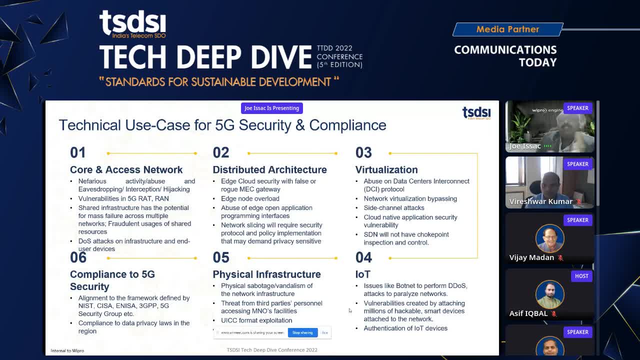 And then you have to be very careful about how you use security in compliance, And these things have to be a living model. This can't stop in a day or two. Each day is a learning, And that's why I said implementing of statistics and 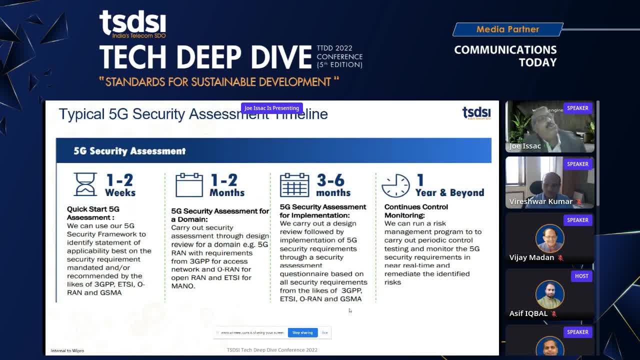 algorithms is the best way to take this forward. Typical assessments take the way we wrote. is what that you are one to weeks of a blue stick at a dipstick based assessment where you it's a question of assessment and a snap view of the entire network. You're able to say what is the kind of environment you're at, and a two months assessment on each domain of the top. 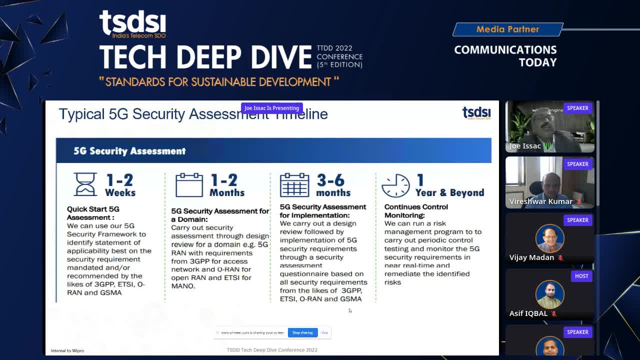 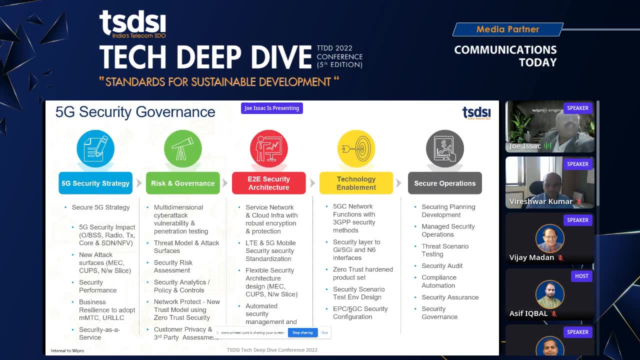 And then then this, inevitably, and this you baking component before the technical component, and three to 6, they have done, And then once the report is in place, the that's kind of as an identifier Identified, every interval that across every year to six months. 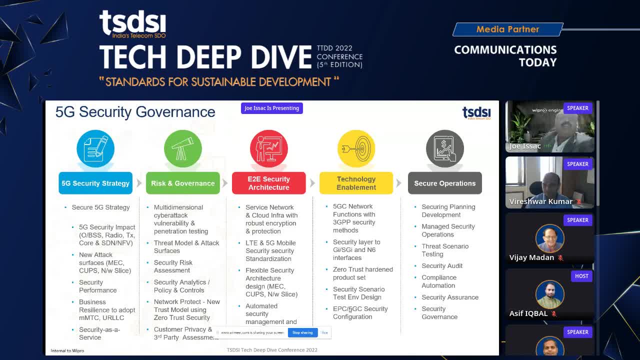 There is a repeatable desk hunting going on which makes it based some, some things, I think, our governance, to ensure that know there is a secure way of managing the whole of the rest, the governance, the security architecture from an infrastructure perspective, from from security standard perspective, from a from a CEO dutyards, worldisher. 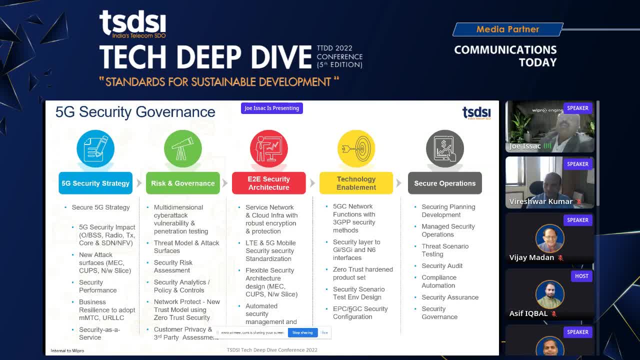 design, the CUPS, the slicing, for example, enabling automated security platform using. I would still think that data science algorithms are better than AML here, because you have a trained data and the training makes it even more intelligent and better in functionality, And that's one area. 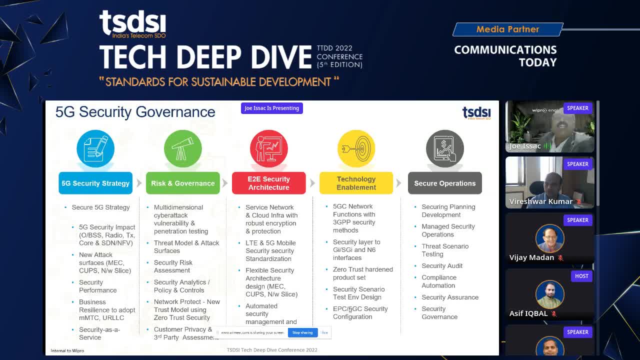 where we are also looking much into it. How do I ensure that the SG interface or GN interface are much more hardened? How can I ensure that zero-trust hardening product can be in from a service perspective? How can I ensure that I have a secure planning from the 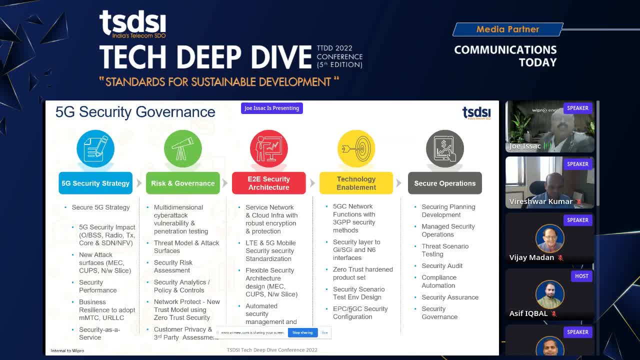 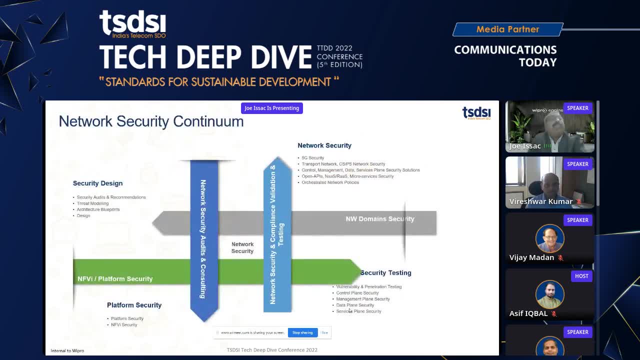 security to the risk, to a security architecture from end-to-end perspective and updating your technology at regular intervals and secure operation. I think that's the thing To end up the slide. I think I just put up into four things. that one is: the design of security has to be. 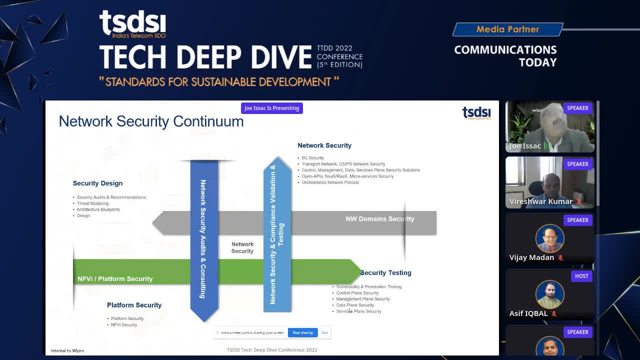 around. It cannot be just that: the protocols. it has to be from the learning of networks, the networks lane hackers learn day by day, So the pattern of how your network behaves becomes very critical. hence calls for audits. There are threat modeling, which happens on a daily basis. 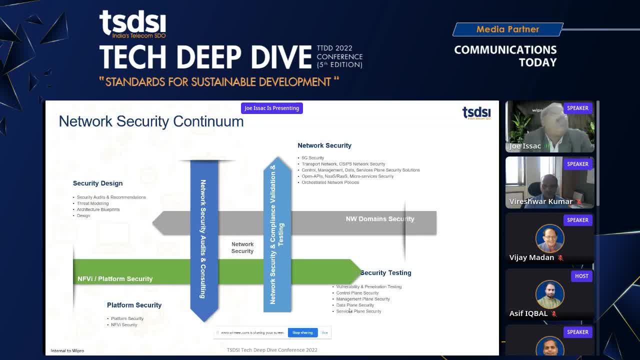 though the threat. what you see on a web is not the same what you see on a radio interface, for example. You should be able to model each of these and bring it forward. These architecture inputs give you a lot more insight and be able to manage better From a platform security especially. 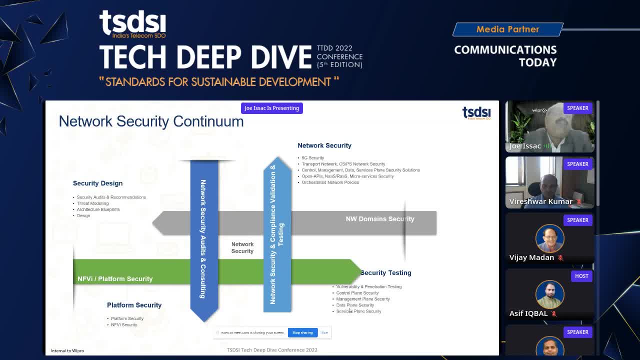 when it comes to NFVI or the cloud infrastructure, I didn't address cloud from a public cloud perspective, but that's even more that because they will cover that part of it and the remaining they will not cover. So how do you holistically cover? 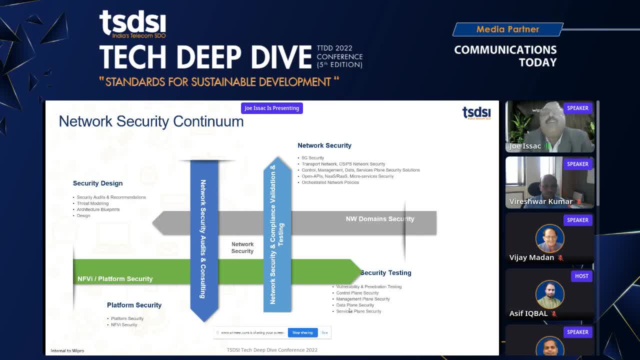 that part of it. How do you ensure that you have a complete network security, from your transport to your applications, managed through the controller or the orchestrated network plans? How do you ensure the entire security testing is in place? I think with all of these four together, I think you'll be able to achieve. 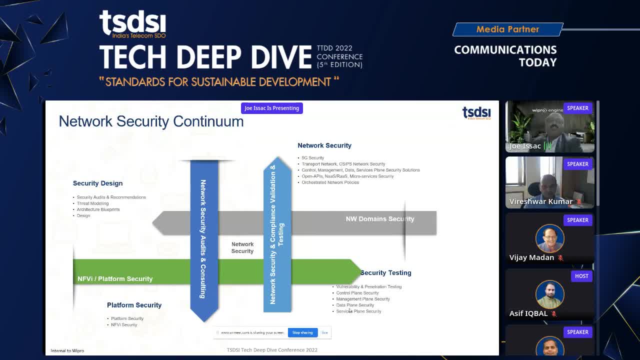 some amount of sensitivity in the whole of this and manage this through. I'd like to conclude saying that security is a daily affair. Network security, especially in 5G, 6G networks, will be a daily affair going forward And if you are able to model, 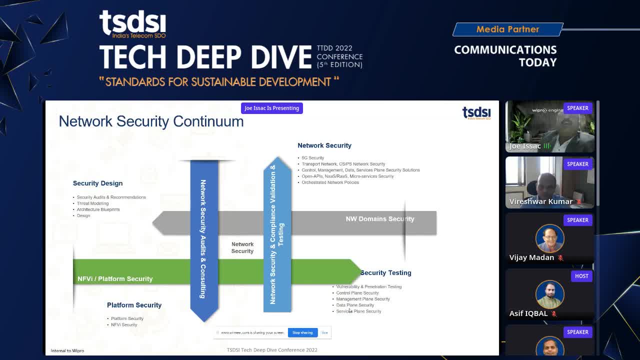 the whole of this using data science algorithms. this is the best way to go forward, and you're able to predictively figure out the faults without human interventions. I think that's the message I'd like to leave to the team. Thanks a lot, Joe, for the wonderful. 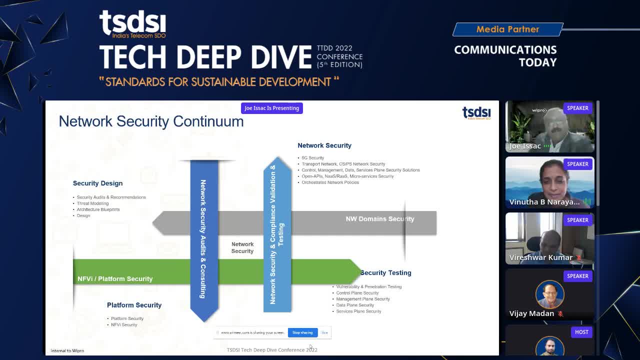 information. Thank you very much for your insights into the challenges and not just the challenges- how they can also be addressed. Everything is not lost Definitely. with audits, with assessments and using data science, things can also be controlled. So thanks a lot, Joe, for taking time for this session. 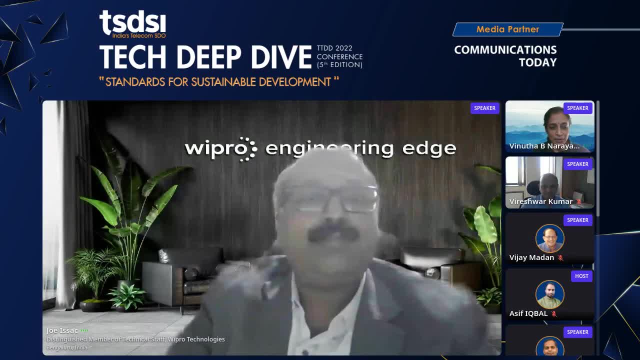 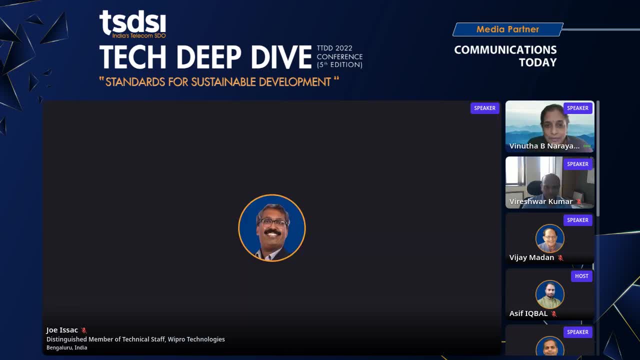 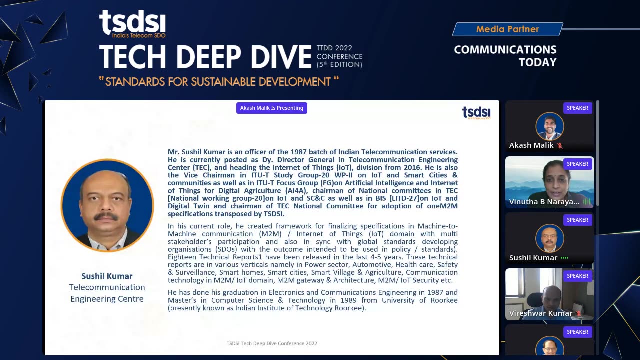 Thank you. Thank you, So we'll move on to the next session by Mr Sushil Kumar. Hello, Mr Sushil Kumar, Thank you for joining this session on the security. A brief introduction about Mr Sushil Kumar. He's an officer of the 1987 badge of Indian Telecommunication. 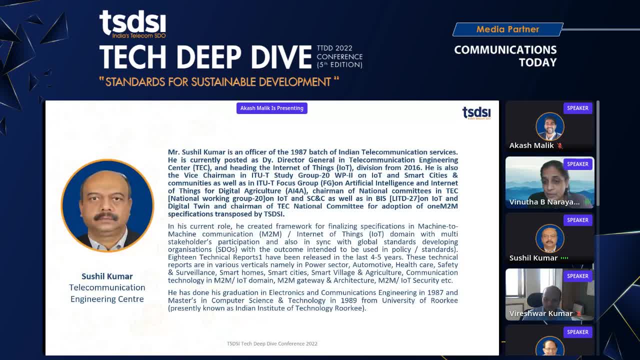 Services. He's currently posted the deputy director of general in Telecommunication Engineering Center, TEC, and he heads the Internet of Things division from 2016.. He's also the vice chairman in ITU study group 20 on IoT and smart cities and communities, as well as ITU. 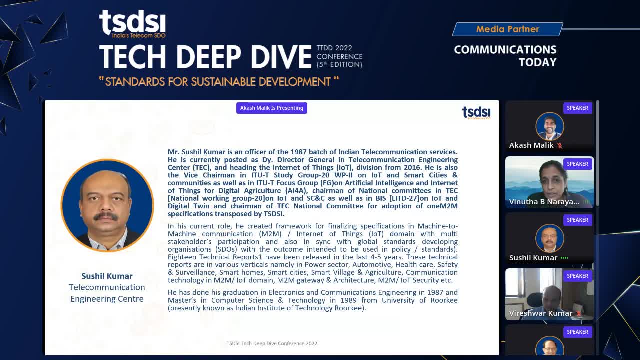 focus groups on artificial intelligence, Internet of Things for digital agriculture. Mr Sushil Kumar is the chairman of national committee in TEC on IoT and NC and as well in the BIS on IoT and digital twin. He's also the chairman of TEC national committee for adoption of. 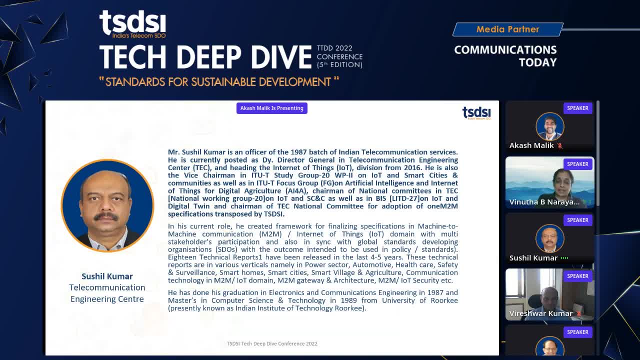 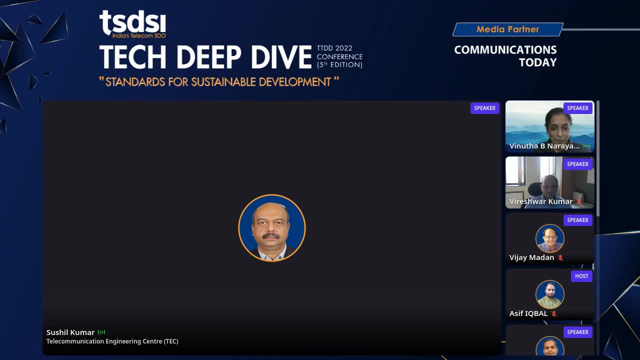 one M2M specifications transposed by TSDSI Over to you. Mr Sushil Kumar, Thank you for taking this session. Yeah, thank you very much. This. please give me the sharing right for the presentation. Okay. 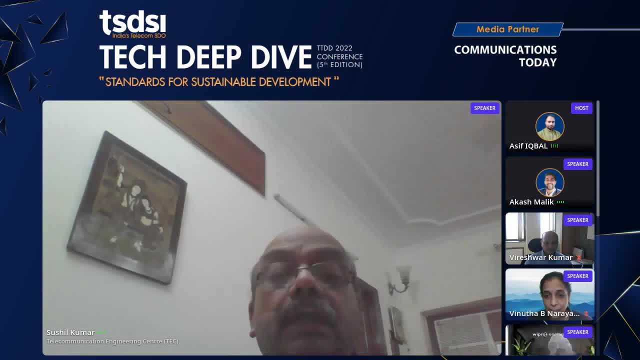 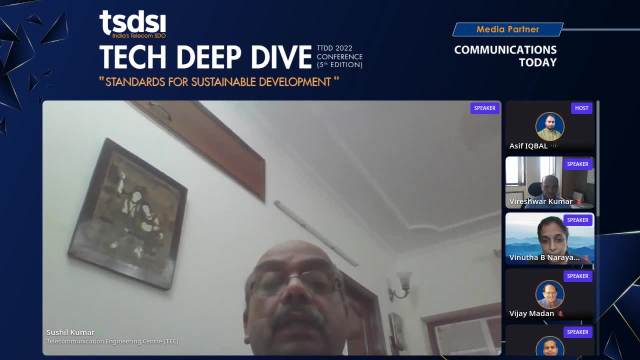 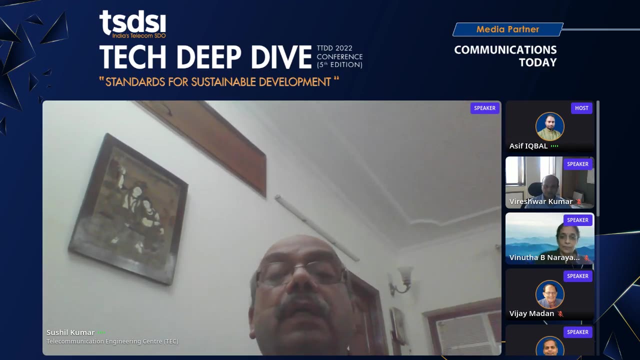 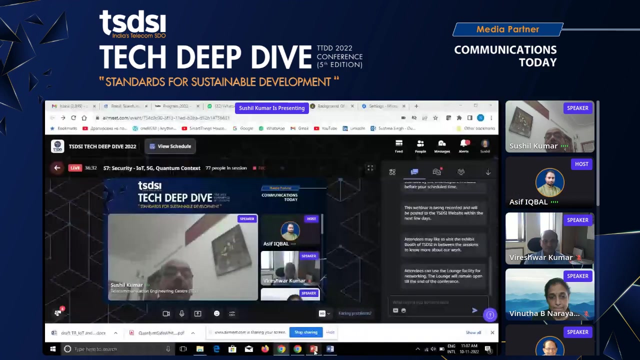 You can share, sir, In the bottom third, present to audience, Then select entire screen or it's nearby your mic. Yeah, yeah, I got. Yeah, we can see your screen now. Yeah, Okay, thank you very much. 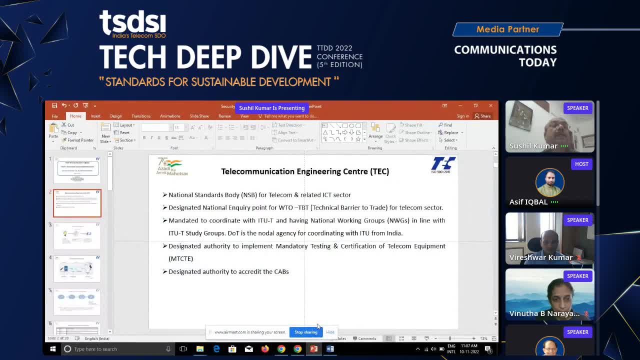 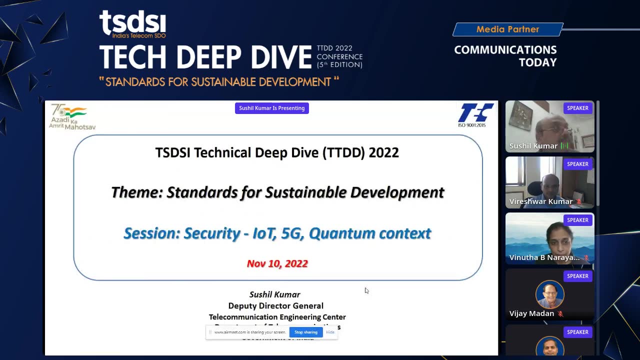 And thanks a lot to TSDSI to give me this opportunity. Sir, can you make it slideshow mode? Yeah, yeah, sure, sure, Thank you, sir. Okay, it's a wonderful presentation by the previous speaker on 5G security And I'm really 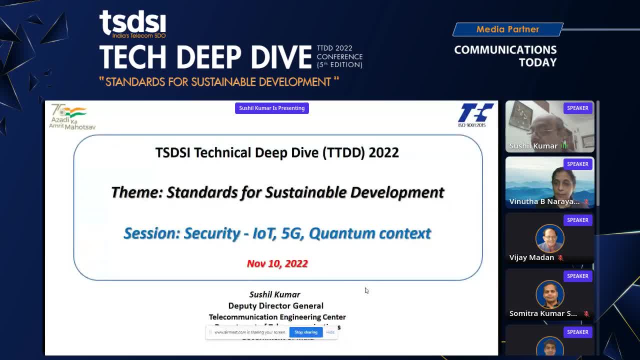 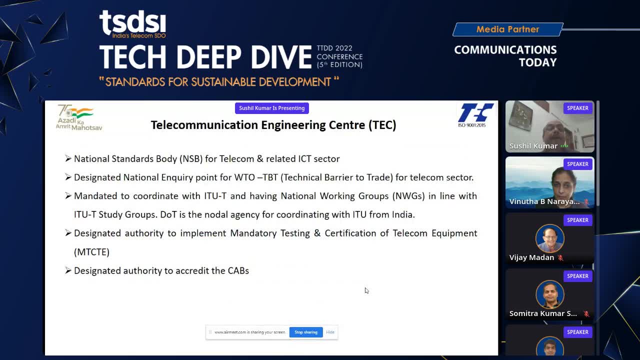 thankful to TSDSI to give me this opportunity to express my views on IoT security And I'm really thankful to TSDSI to give me this opportunity to express my views on IoT security And I'm security. so i am from telecommunication engineering center. this tec is basically the telecom. this. 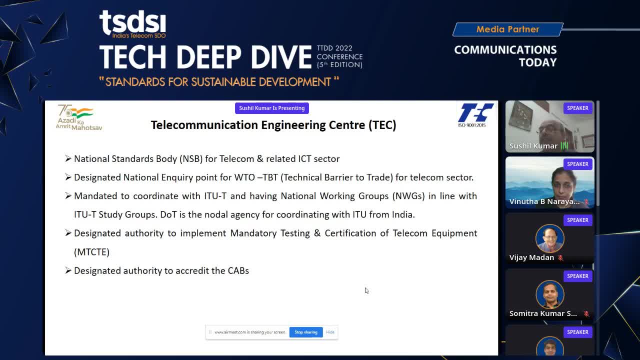 standard body for the dot on telecom and ict related activities and it is also designated as a national inquiry point for wto tvt. that is technical barrier to trade for telecom sector, mandated to coordinate with itut and having national working groups in line with itut study. 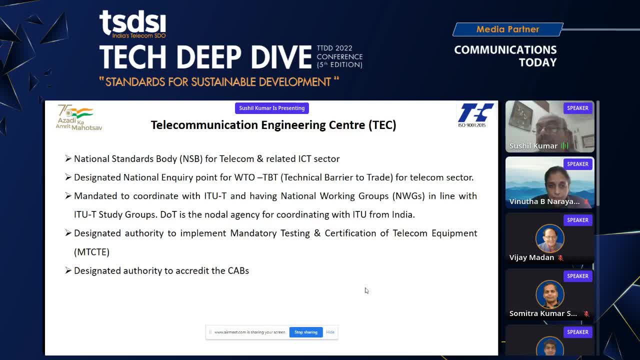 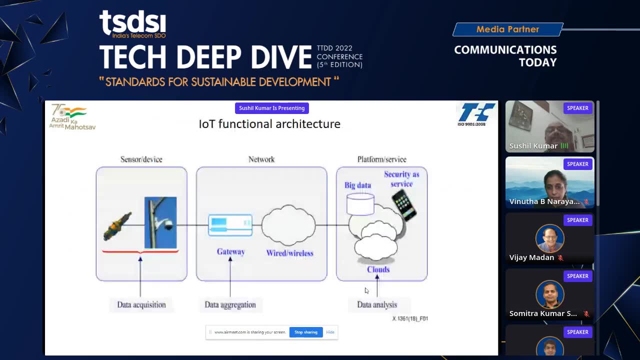 groups. it is also designated authority to implement the mandatory testing and certification of telecom equipment that is very much required to ensure the security and safety of the telecom and the iot devices, and it is also the designated authority to accredit the caps. this is one of the 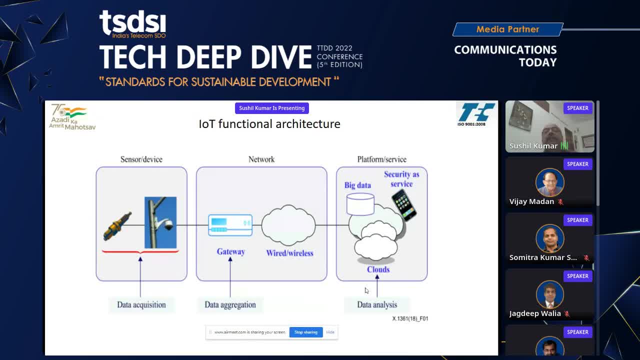 pictorial view of of the iot domain, like from the sensor and devices to network and then to platform, and the security is required in all the items of the iot domain, from starting from device to network gateways and these platforms. platforms are mainly the software entity and it will be in the cloud. 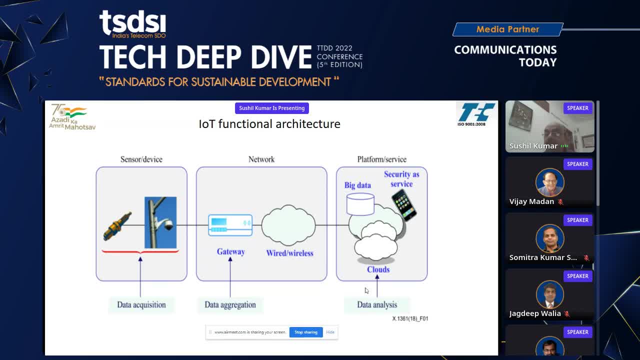 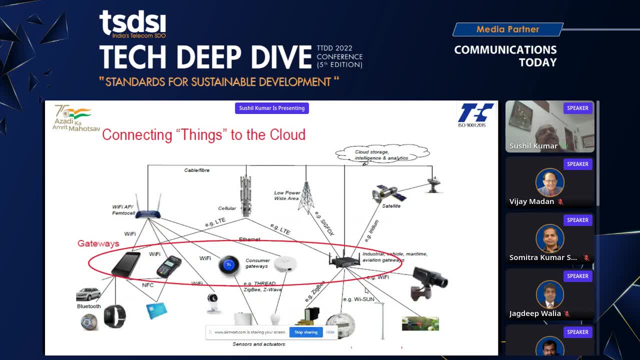 so for this the standard based solutions are required and, as we know this, in iot there may be a number of communication technologies, depending upon the use cases, starting from nfs, nfc, ble to cellular, non-cellular and even now on 5g communication technologies. so this is basically a pictorial view where the in the red circle we will be having the gateways. 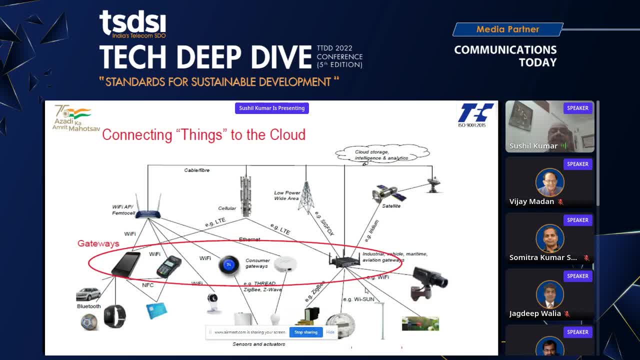 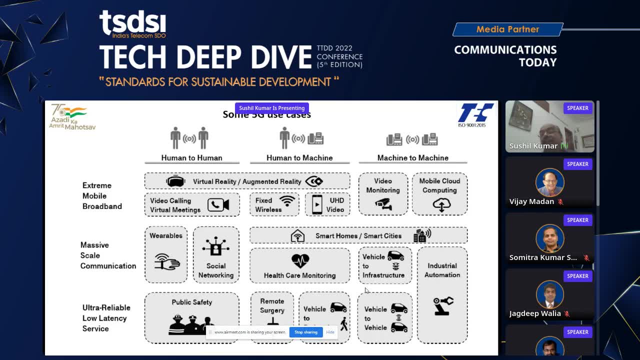 and gateways should be ip enabled and the devices behind the gateway may be ip or non-ip. then, as the 5g is being deployed across the country and across the globe now, we will be having a large number of devices to be connected on the 5g technology as it will be having the massive 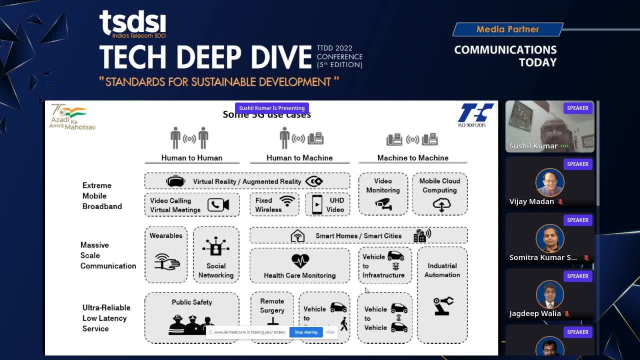 machine type communication, as well as the ultra reliable, low latency services. and 5g is mainly for the vertical industries and that is for the iot domain. so two-thirds of the 5g will be used for the iot and most of the use cases will be. 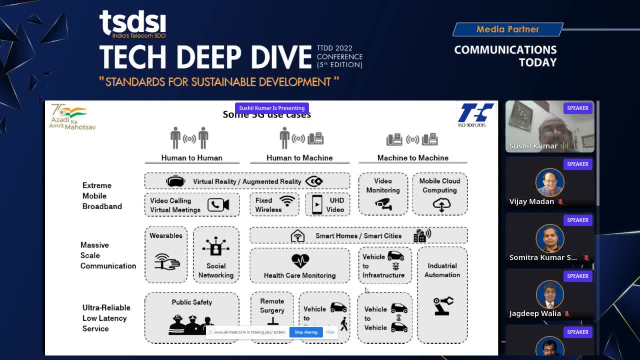 like, which are not practically possible in the previous generation technologies and will be possible in the 5g technology, like industry 4.0 and then cellular v2x, and we can have robotic surgery and so many critical use cases will be available in the 5g. but the security is required. 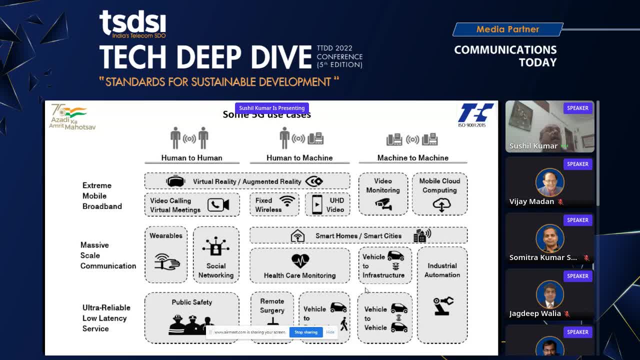 to be maintained for the 5g technology also, because a lot of elements will be accepted to the core, to the cloud. the 5g core will be in the cloud. then we will be having the ai and ml algorithms are not only in the clouds but it will be available on the roadside units or the, we can say the vts for cellular v2x. 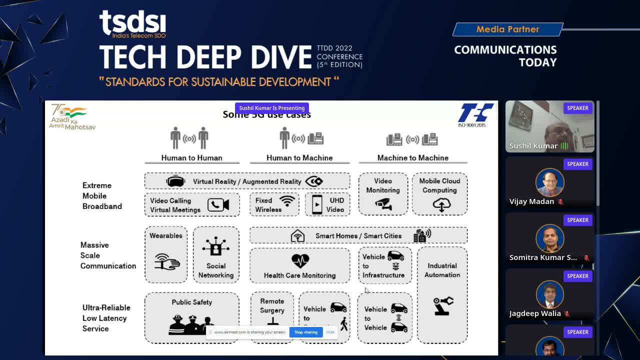 will be. we will be having the roadside units deployed across the cities and where the ai ml algorithms will be will run. so the security is required to be ensured in all parts of the communication technology, as well as the devices and also at the platform. now the dot has released. 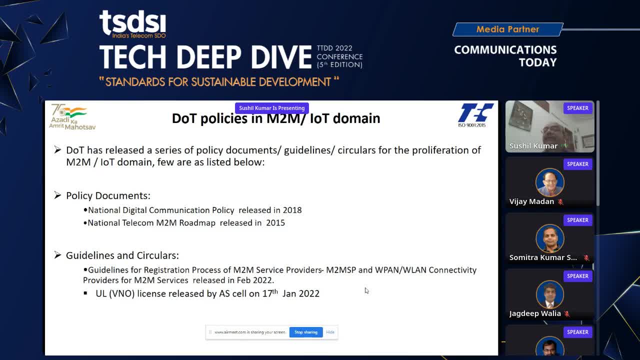 a number of policies for the proliferation of the iot domain and the national telecom m2m roadmap that was released in 2015, and this ndcp. it was released in 2018, and a number of circulars and guidelines have been released in the last five to six years. 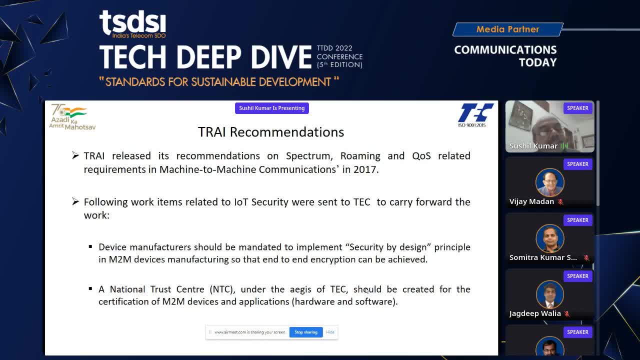 then uh try has also released uh its recommendation in 2015 and those recommendations were accepted in total by dot and two of the work items which are related with the device security. they were sent to tec to carry forward the work. these are like the device manufacturers should be. 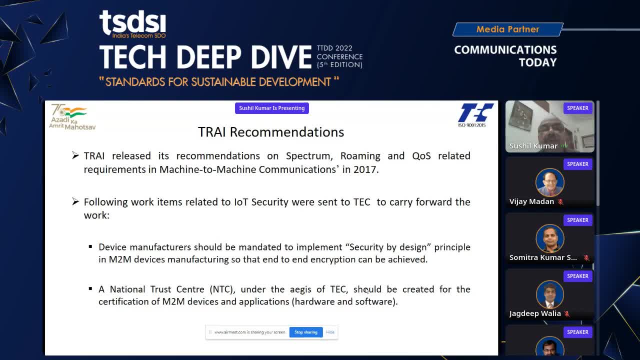 mandated to implement the security by design principles in m2m device manufacturing so that end-to-end encryption can be achieved, and the second one is in national trust center under the tec should be created for the certification of m2m devices and applications, hardware and software. 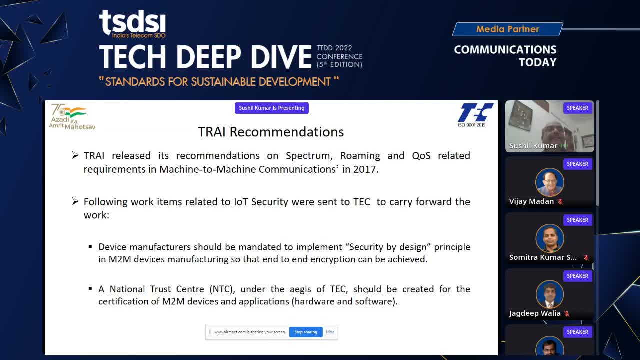 so hardware will be tested in in mtct and the software can be tested. software applications can be tested by sdqc and other software may be tested in the labs. this it's are- is being developed by the security wing of dot in bangalore. therefore, testing and certification- that is the prime requirement of 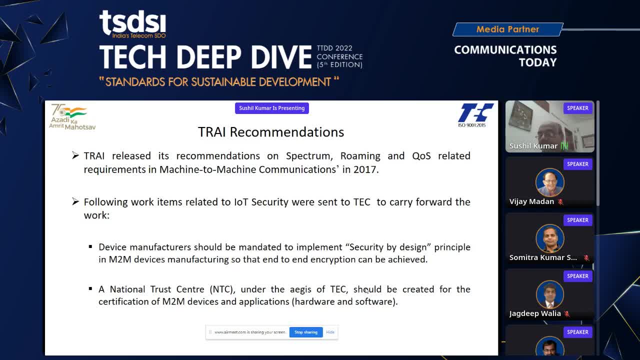 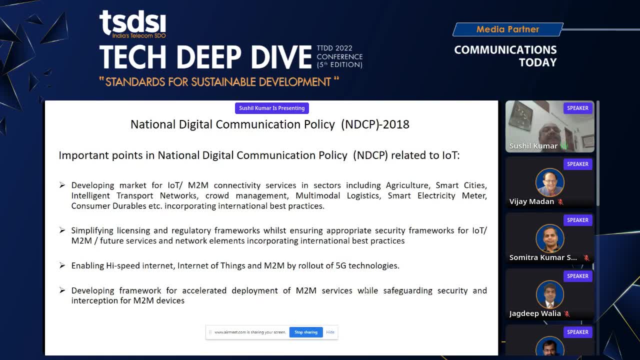 of the telecom equipment as well as the IoT devices for ensuring this security. Then, further in the NDCP, which was released in 2018, these are some of the very important items related with the IoT domain, like delivering market for IoT M2M connectivity services, like 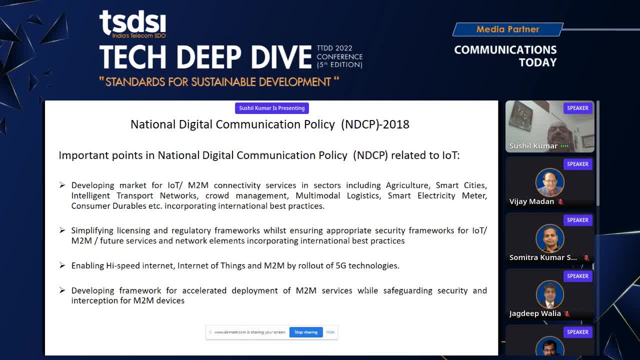 sector, including agriculture, smart city, intelligent transport system, crowd management, multi-model logistics and others. simplifying licensing and regulatory framework, enabling high-speed Internet, Internet of Things and M2M rollout for 5G technologies. developing framework and X-related deployment of M2M services, while safeguarding security and 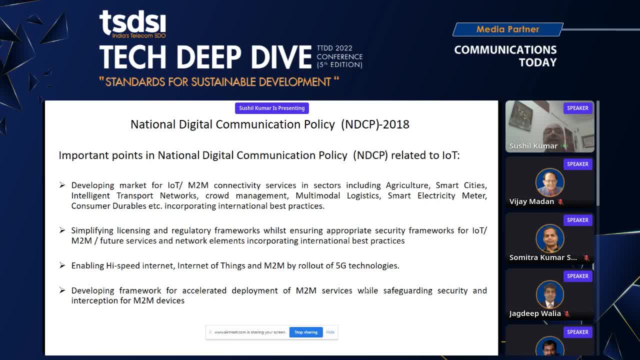 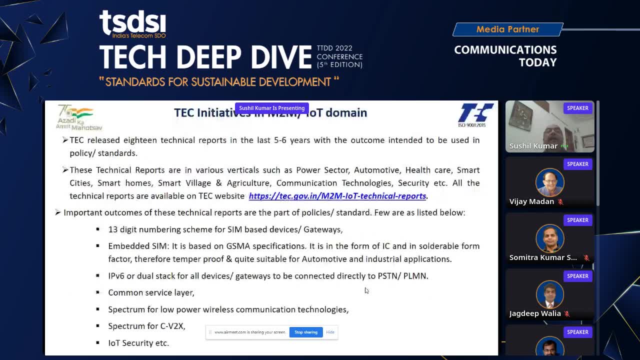 interception for M2M devices. So these are some of the points which are taken from the NDCP 2018 related to the IoT and its security. Then TEC started. TEC started working in M2M IoT domain sometime in 2013-14, and, with the association of the, 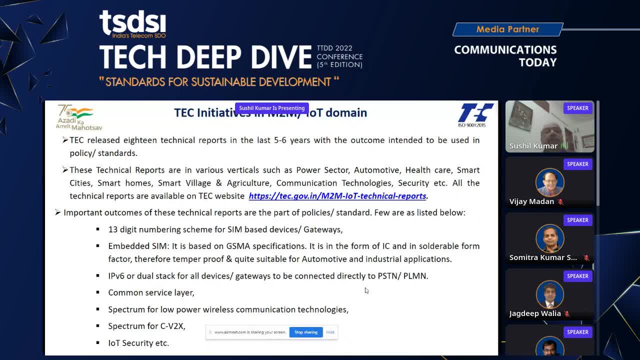 industries, academia and standardization bodies, in multi-stakeholder working groups, we can say- and released 18 technical reports so far. These reports are in power sector: automotive, healthcare, smart cities, smart homes, smart villages and agriculture, communication technology, security, et cetera. 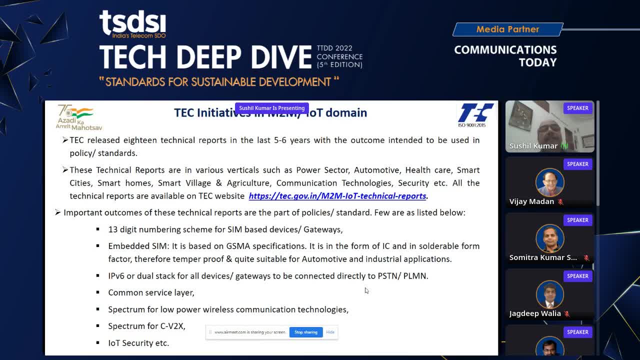 And some of the key points, like the 13-digit numbering scheme which is being used by the TSBs for SIM-based devices, that was developed in TEC-embedded SIM. IPv6, or dual-step for all devices, gateways, common service layers- large number of points which are the part. 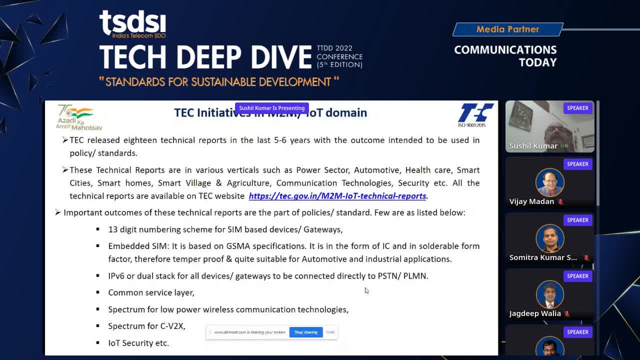 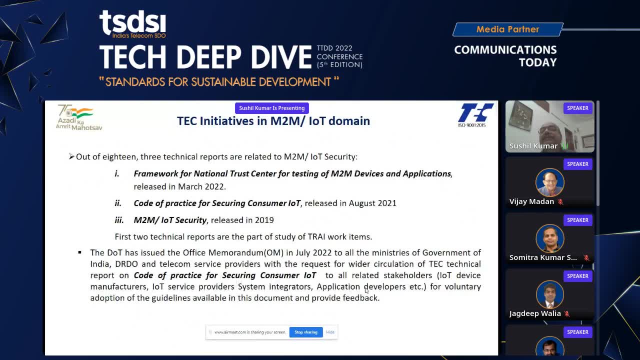 of the policies and the standards. They are the outcome of these technical reports. Three reports are related with the security. That is, the framework for National Trust Center for testing of M2M devices and applications, released in March 2022.. In fact, when we started working on the TRI work items which I mentioned in the previous, 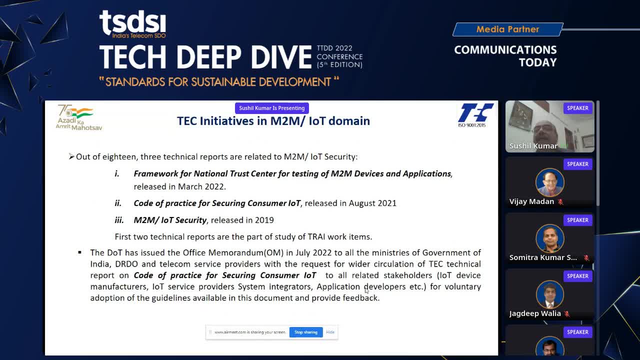 slide the first two documents. they are the part of the result of the study of the own TRI work items, That is, a framework for NTC and the Code of Practice for Securing Consumer IoT. However, the study is still in progress and we are expected to release the complete document. 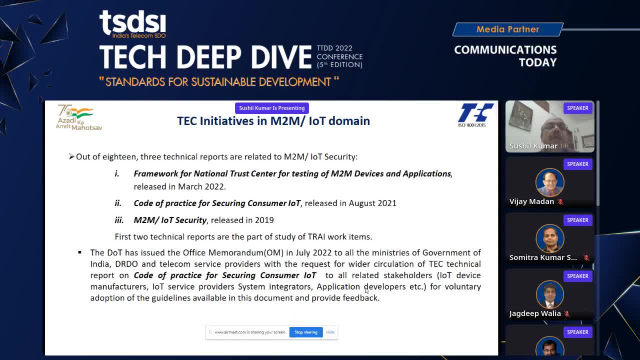 by this month, So we are expecting to release it by December 2022.. And M2M IoT Security. it was released in 2019.. So DOT has taken a further step and issued the Office Memorandum in July 2022 to all. 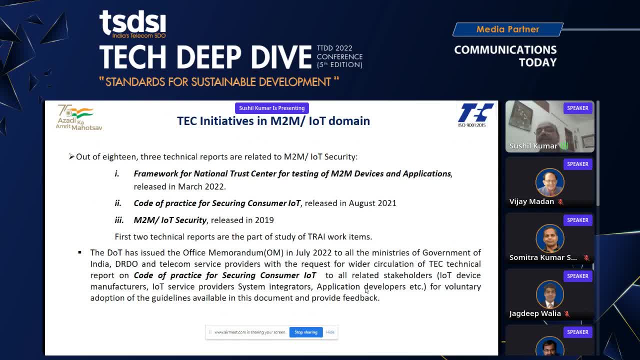 the ministries of Government of India, DRDO and Telecom Service Provider with request for wider circulation of Code of Practice for Securing Consumer IoT to all related stakeholders, like the IoT device manufacturers, service providers, system integrator, application developers, etc. for voluntary adoption of the guidelines available in this document. 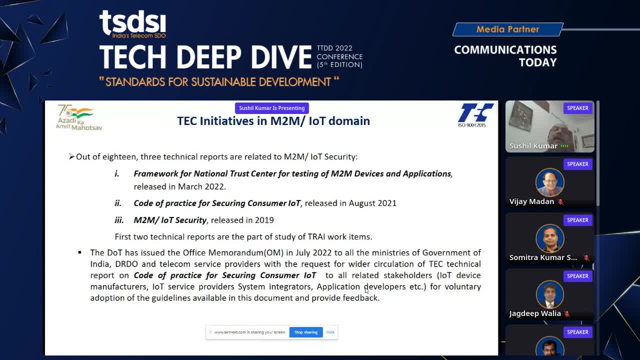 Thank you, And thank you, Puneet, for providing the feedback, Because you cannot mandate anything overnight. First, the things should be voluntarily adopted And they are very important from the security point of view up for the consumer- IoT devices- and after some time, some of these guidelines can be mandated. 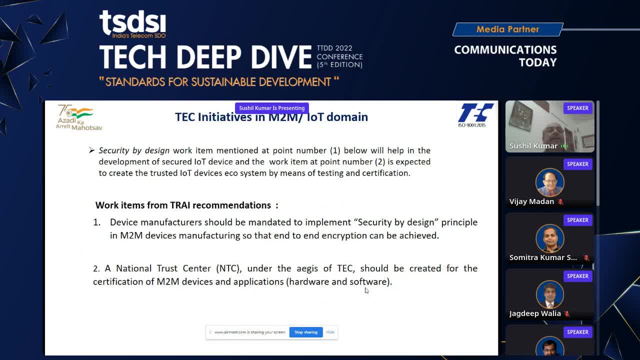 And then security by design work item. like these two work items on which we are still work- work is still in progress- and the ntc framework- national trust center framework. the document has also been released and this work has been awarded to cdot by nscs for creating a. 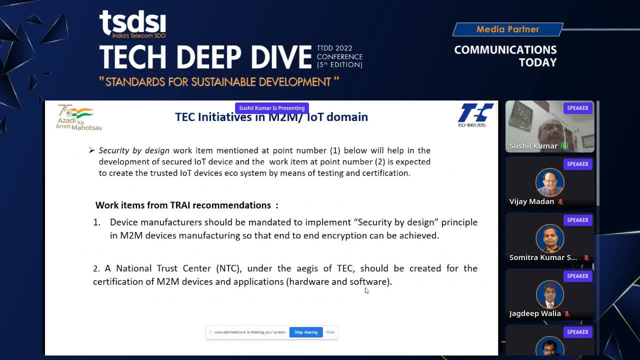 portal and for doing this pilot project for verticals as well as for the smart cities, because all the all the platforms they they are supposed to detect the vulnerabilities in the iot devices, like it may be a camera, it may be a tracking device or any other devices. 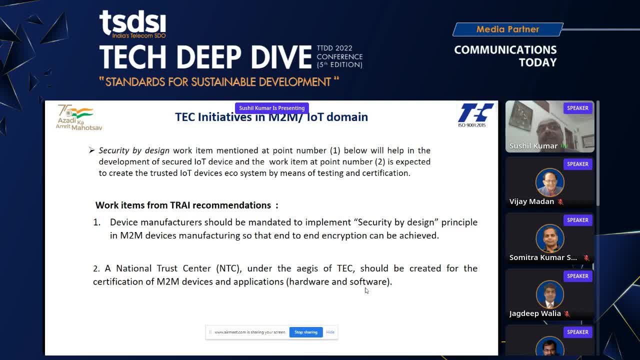 in the emblem service provider registration policy which has already been released by uh dot and more than 100 emblems provider. they have already started uh with that. so now it will be required that the if any vulnerability or security related uh issue arises in the device, then the platform uh should be able to detect uh that one and should able to manage uh. 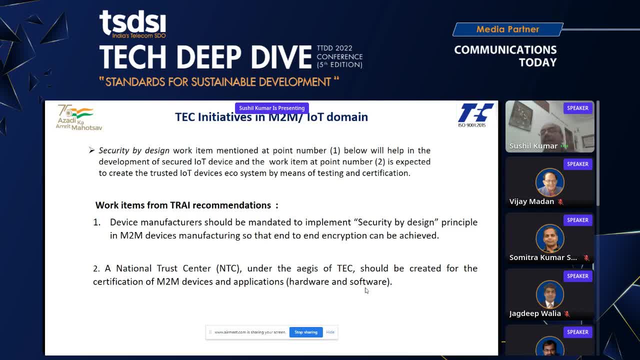 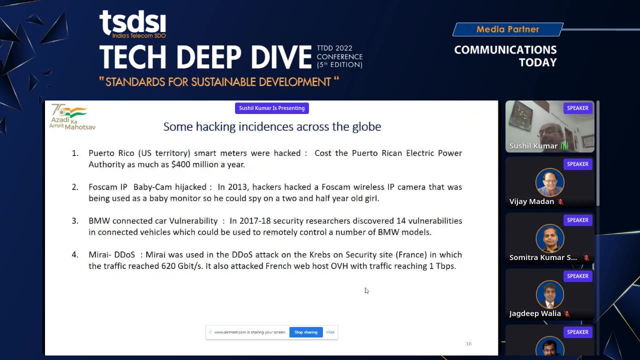 the vulnerabilities or the security related issues and uh further communicated communicate to national trust center. national trust center will uh intimate to uh the manufacturers or the researchers and uh the further uh the manufacturers should be able to uh develop the patches or the software and uh update over the air for that uh and there will be. there are uh from this study uh. 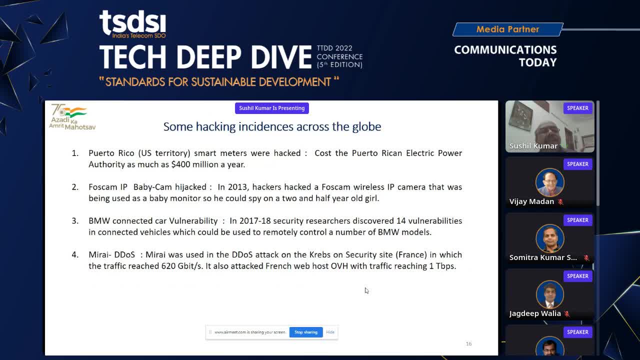 we are carrying out. uh. there are so many hacking events across the globe. for the iot devices, uh like a smart meter, then the foscam ip, baby cam, bmw, connected car vulnerabilities, ddos, man in the middle and so many uh type of vulnerabilities may arise. 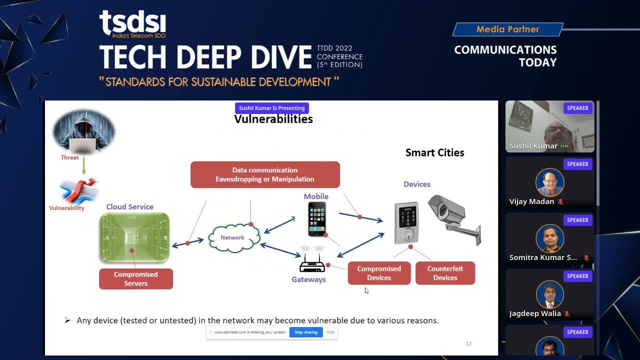 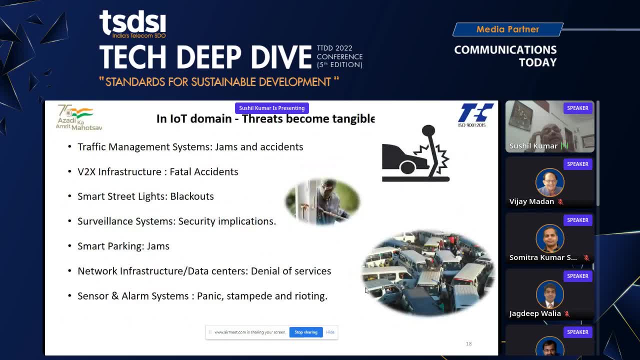 in the devices in gateways or uh in the smart cities or in any vertical industries. uh then, uh, what? maybe the consequences from uh this? there may be a traffic management systems, gems and accident v2x infrastructure, fatal accidents. maybe they are smart street light. uh may also be had that this pilot was done by welcome in some of the us. 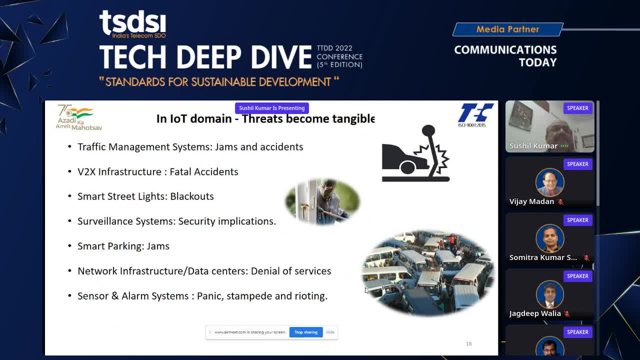 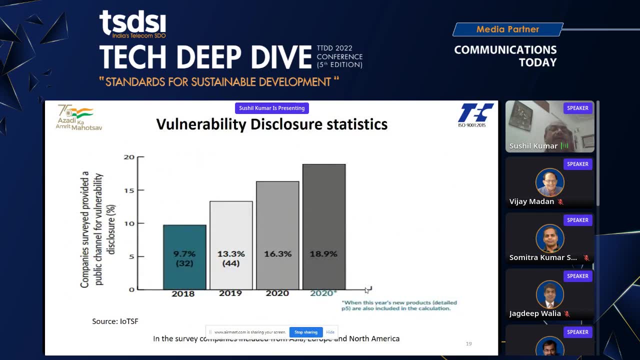 university and they presented in one of the webinars organized by tc. then smart parking gems, network infrastructure, data center, denial of service. then sensor and alarm system, panic stamper- such type of things may happen. This is a survey done by the IOTSF Internet of Things. 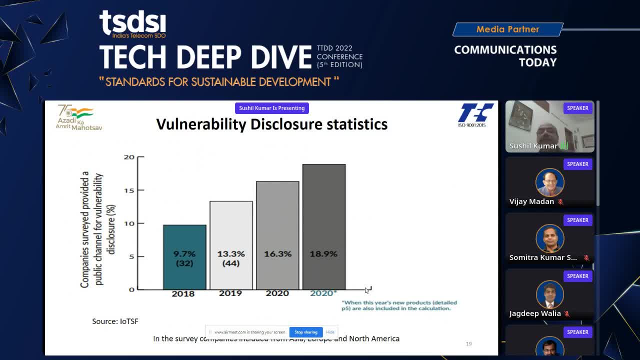 Security Foundation. They have done this survey for around 332 IOT device manufacturers and they found from 2018 to 2022, only there was very small rise of the device manufacturers who provided the vulnerability disclosure statistics and they are having the policies for vulnerability disclosure And this survey was done for the IOT manufacturers for the 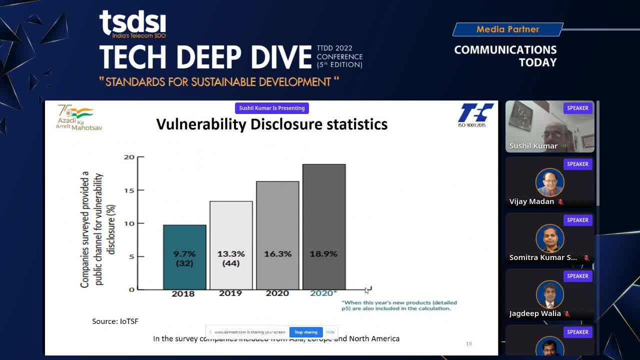 North America, Europe and Asia. This is really a very surprising situations that the device manufacturers. they feel that security may be the last option for them And Now it is required that some sort of guidelines would be mandated by the regulator or the policy makers, at least for the vulnerability disclosures. 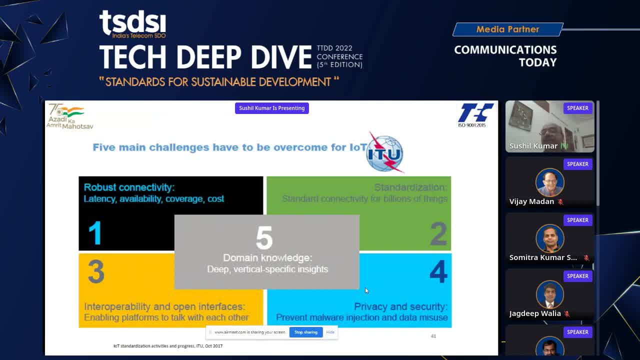 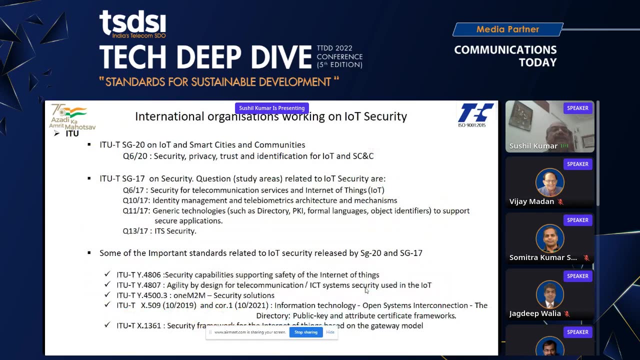 This ITU has also defined privacy and security one of the important item for the proliferation of IoT ecosystem. It's a big challenge and ITU-T study group 20 as well as study group 17,. they have released a series of standards on this. 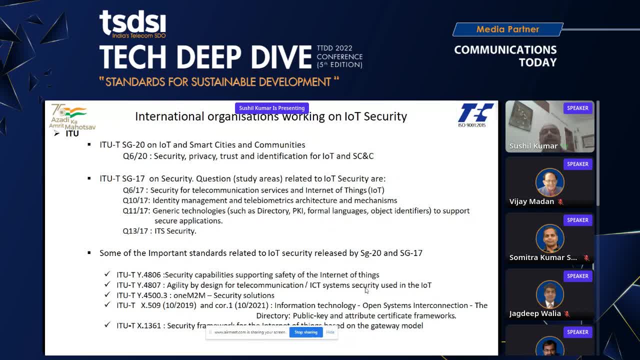 Some of these standards are mentioned here, and one of the most important standards, that is the ITU-T X.509 for creating the secure certificates It is being used. from the last more than 30 years, this standard and so many other standards have been released. 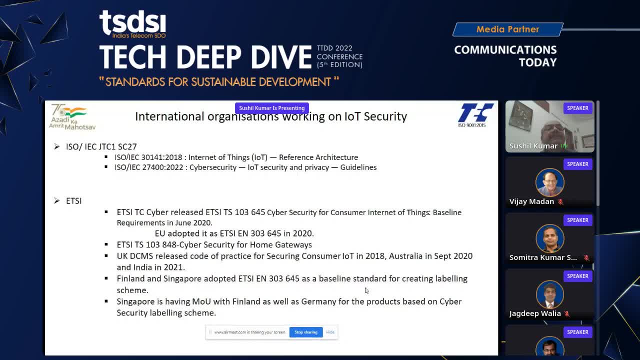 Similarly, ISO-IEC JTC-1 SC-27 has released one of the standards recently, in 2022, that is cyber security, IoT security and privacy guidelines. This is a very important standard. Then ETSI released ETSI TS-103645, that is security for consumer Internet of Things baseline requirement. 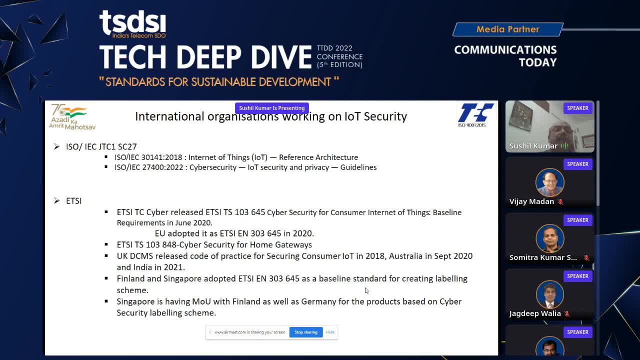 Then the same was adopted in 2022 by the European Union, Simplified Similar. based on these principles, UK is already having the consumer IoT security guidelines released in 2018, Australia in 2020 and India released in 2021.. 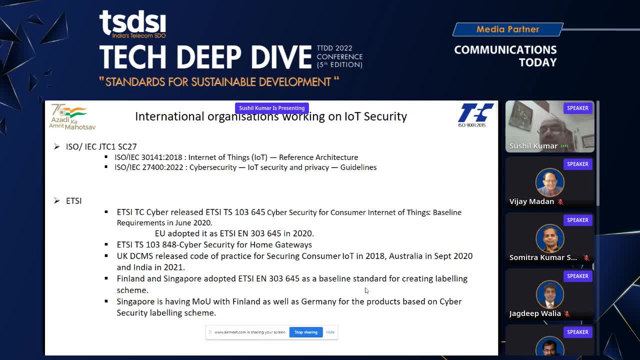 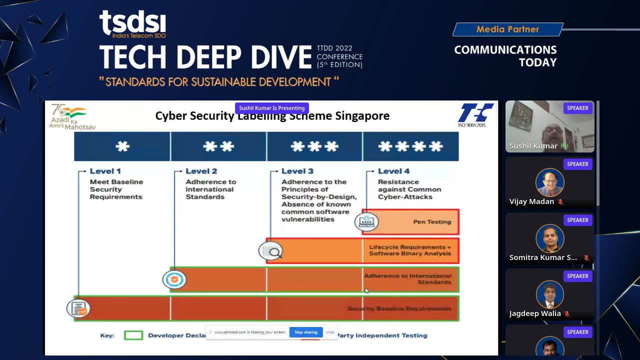 Finland and Singapore. they adopted ETSI EN 303645 as a baseline standard for creating labeling scheme. That is also very important. Singapore is also having MOU with Finland, as well as Germany, for the product based on cyber security labeling scheme. Now this is in fact, in a number of conferences, the NCSC coordinator, this national cyber security coordinator. 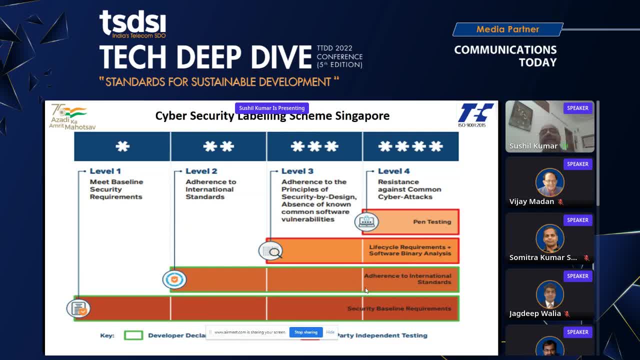 mentioned that India is not having any guidelines, as well as the labeling, which is very, very important for the cyber security. So this is one of and the code of practice was released in 2021 by TEC And after a lot of study of the standards and the best practices across the globe. 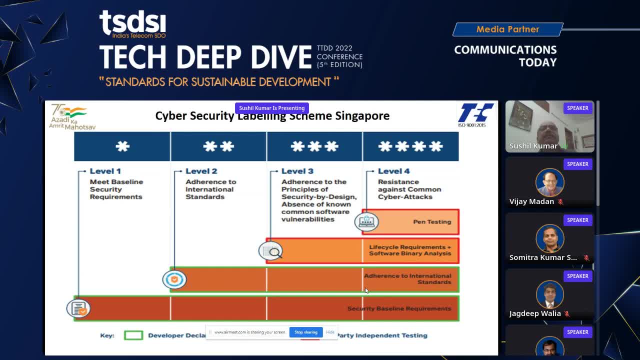 this is one of the slides I have taken from one of the documents of Singapore. This level one: meet baseline security requirement. It is based on 303645.. Then level two, adherence to international standards, And level three and level four. they have categorized the devices in level one, level two, level three. 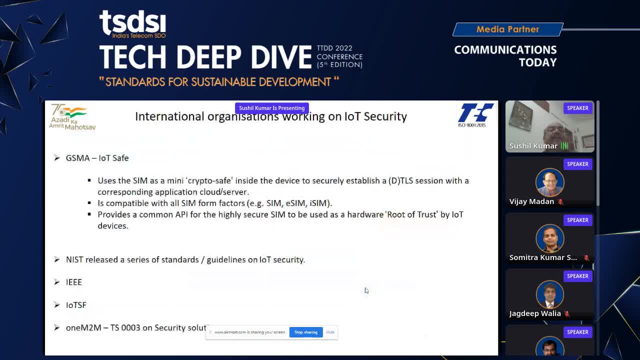 And level four. Now, similarly, the SME has released the IoT safe, which is a very, very important standards. Use the SIM as a mini crypto safe inside the device to secure. establish a DTLS session with a corresponding application. Cloud server is compatible with all SIM. 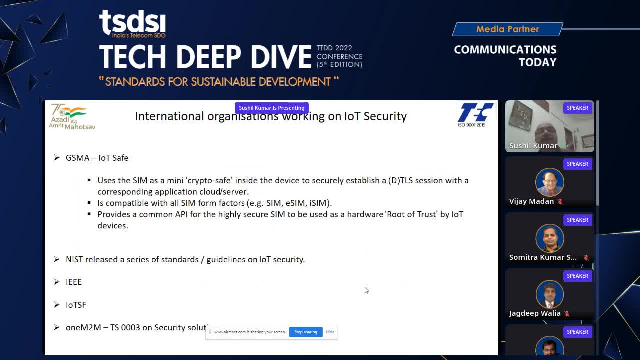 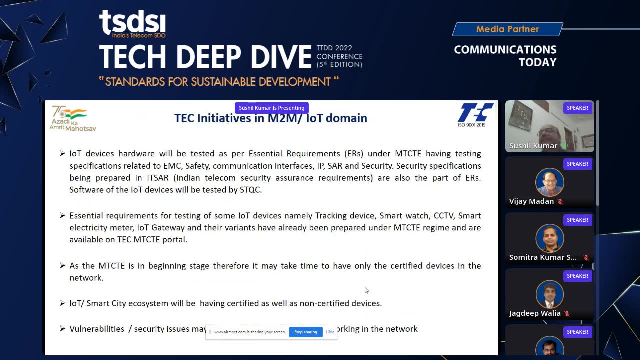 Provide a common API. Similarly, NIST has released a series of standards and guidelines on IoT security: IEEE IoT, SF, 1M2M, TS333.. That is all security solutions. We should use all these standards and guidelines for improving the security of the IoT domain. 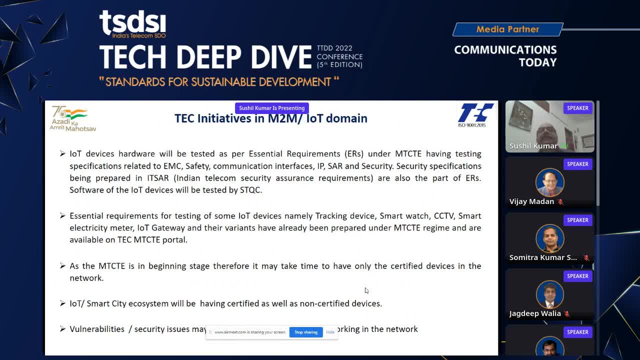 IoT device hardware, which is required to be tested under MTCT. But MTCT is being implemented in phased manner And therefore any of the device which has been deployed in the network may become vulnerable, Whether it is tested or untested. And to facilitate the IoT ecosystem- IoT network, the National Trust Center has come into the picture. 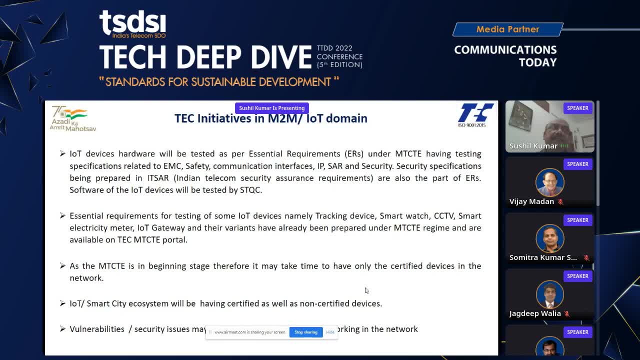 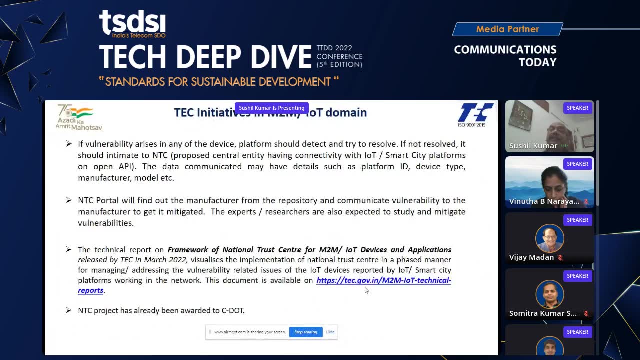 And this National Trust Center, which I mentioned, that it is being implemented. The portal is being created by the CDOT. The work has already been awarded to them And it will help in managing the vulnerability and security related issues. So all the platforms connected to the NTC. 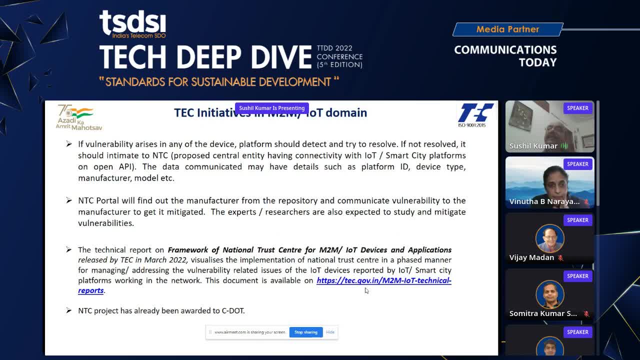 They will be transferring the details on open API And NTC portal, will find out the manufacturer from the repository And communicate vulnerability to the manufacturer to get it mitigated. The experts, researchers, are also expected to study and mitigate the vulnerabilities. In fact, the NTC should also have the repository of the vulnerabilities which are created time to time. 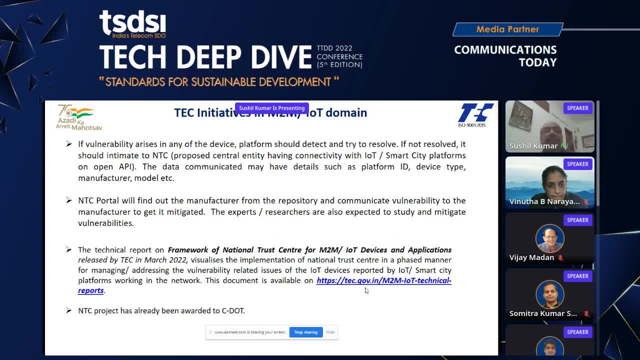 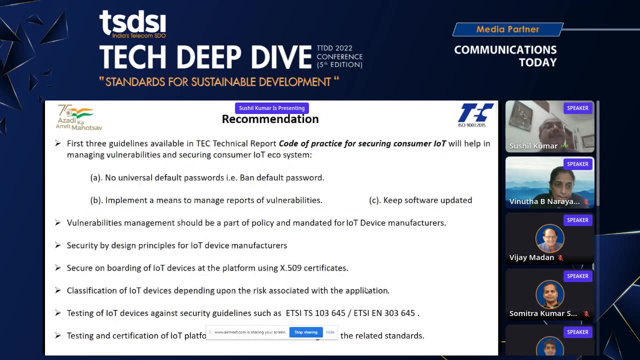 It will help for further research. So NTC framework, which was released by TEC in 2022. And we hope this implementation will be over in the next one year. Then, in my view, at least the first three guidelines of the TEC technical report. 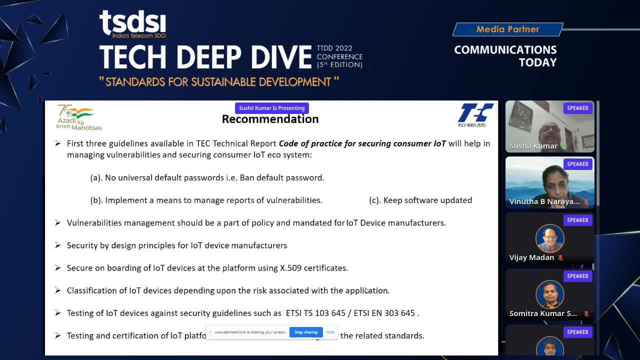 That is the code of practice for securing consumer IoT. It will help in managing vulnerabilities And securing consumer IoT ecosystem. Like no universal default password or banned default password. Second, the implementing means to manage report of vulnerabilities. And third, they keep software updated. 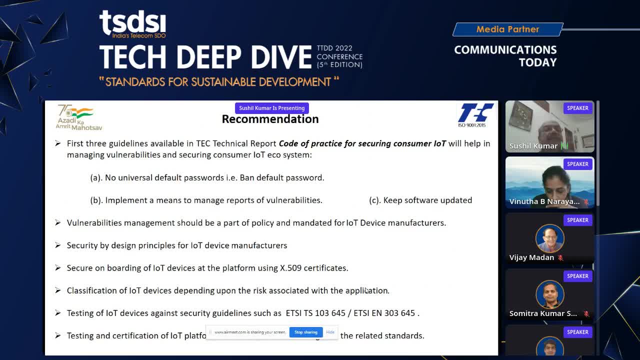 Like the online updation facilities could be available to the manufacturers, And manufacturers would also have the arrangement to implement the means of manage reports of vulnerabilities. And these three items should be the part of the policy And these are required to be mandated. Vulnerability management should be a part of policy and mandated for IoT device manufacturers or the importers. 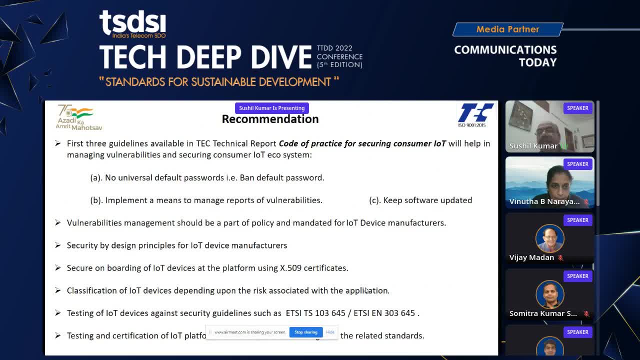 Security by design principles for IoT device manufacturers. These guidelines are expected to come by December. The secure onboarding of IoT devices at the platform using X.509 certificates. Classification of IoT devices depending upon the risk associated with the applications, Like the Singapore, Germany and the Finland. 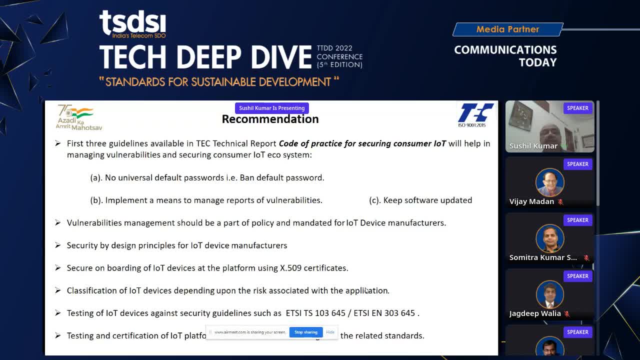 They have done this. It is also in the process of providing this IoT device labeling scheme. Testing of IoT devices against security guidelines- As you see, 103645.. And testing and certification of IoT platform, Because most of the IoT platforms are proprietary. 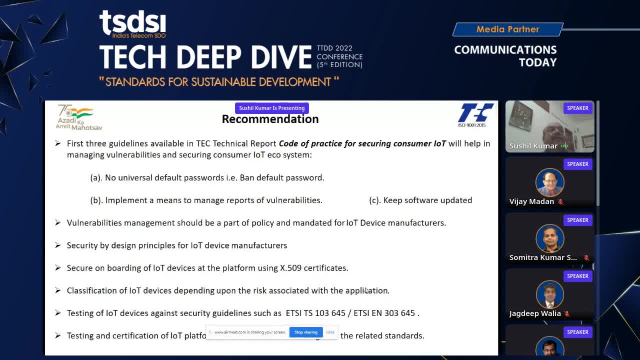 They are non-standard space And whether the security arrangements are security features are being built in or not, Nobody knows. So the IoT platform, The IoT platforms, as well as the 5G core, are required to be tested against these specifications. Related specifications. 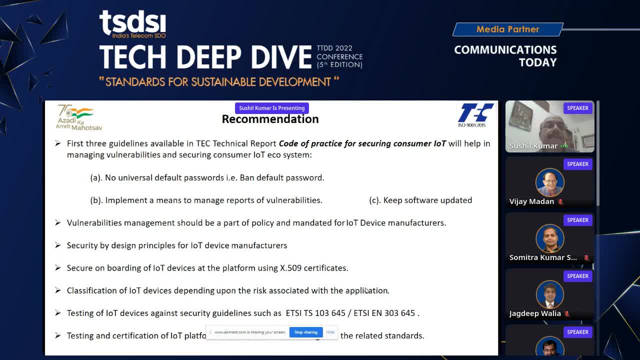 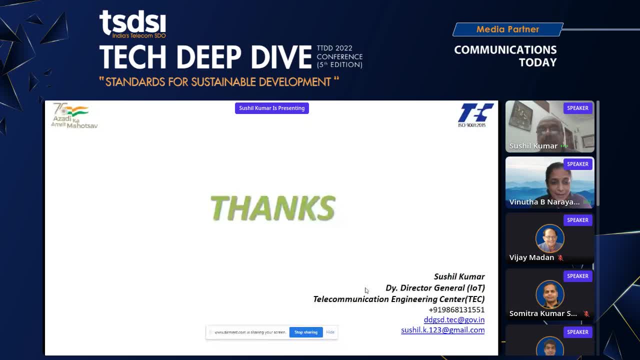 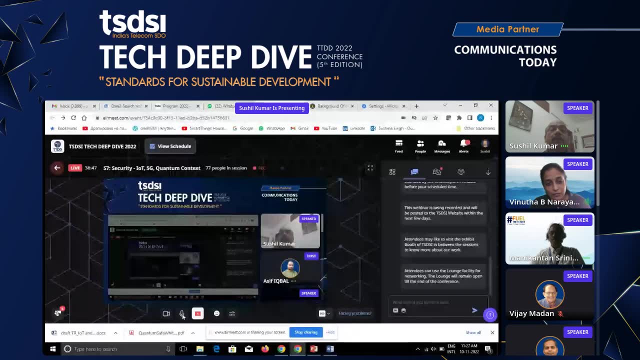 So these are the points from my side, Thank you. Thank you very much. Thank you, Mr Sushil Kumar, for the wonderful session Of getting to awareness, Aware of the challenges that can be in the IoT side, And it is not just that. 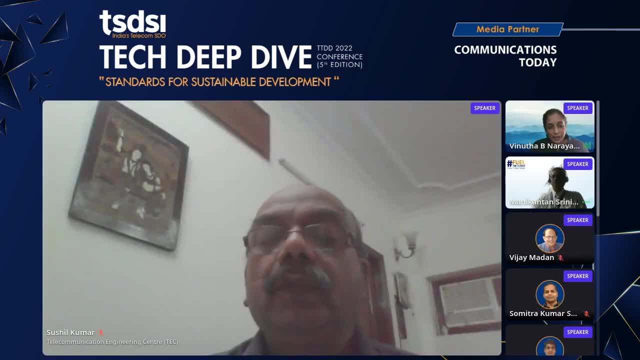 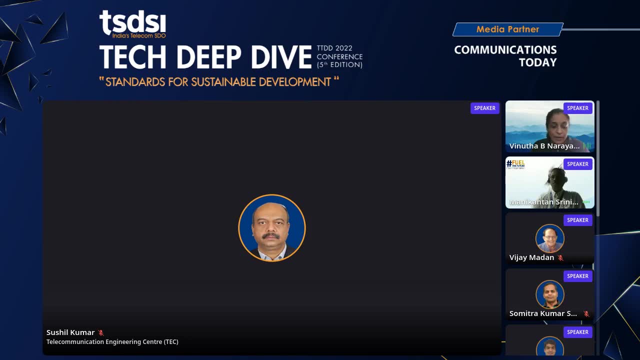 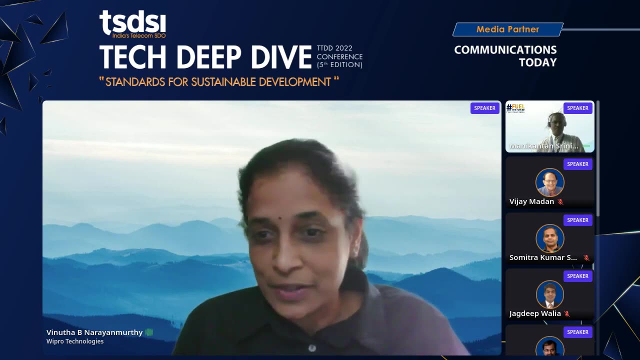 The guidelines and how we can also ensure that we can take care of these issues With various guidelines And maybe initially it can be voluntary for people to adhere to these guidelines And later on we could make it mandatory. Thank you for the wonderful session. 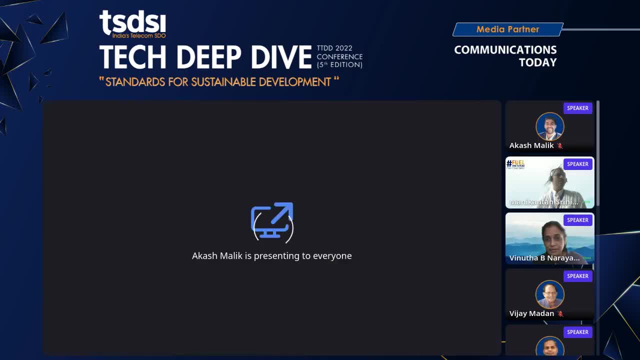 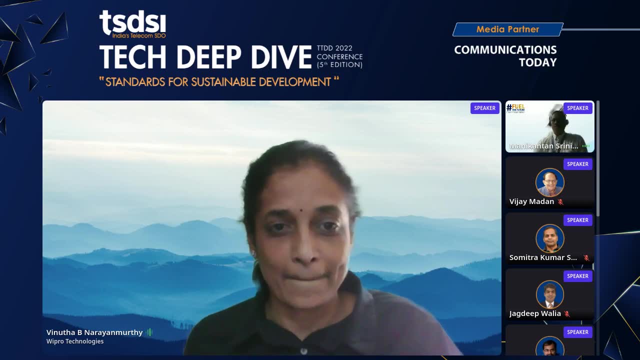 Are there any questions here That we have to flash or something? Sorry, Do we move to the next session? We have questions. If you would like, we can take them now or at the end of the session. Yeah, Maybe we could take them now. 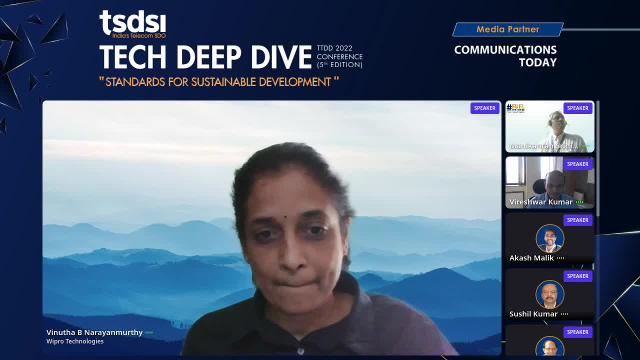 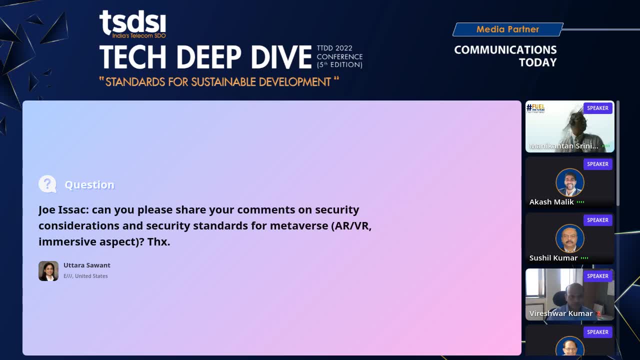 Okay, Yeah, We should take them now. Yeah, Okay, Thank you, the first question is on the screen. uh, so it's for the for mr joe. uh, can you please share your comments on security considerations and security standards for metaverse? they are, we are immersive. 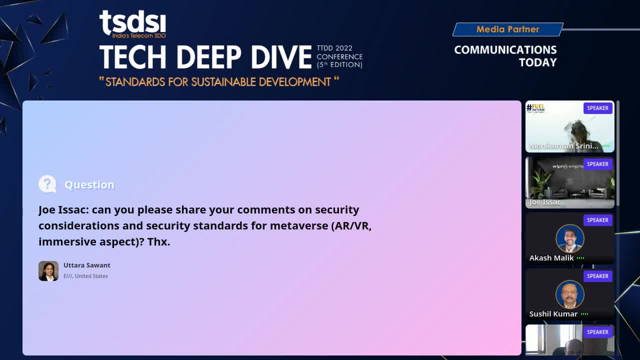 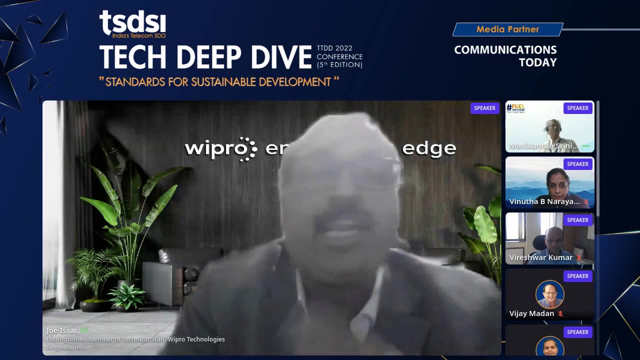 aspect. but do i answer now or should we answer now? yes, joe is okay. i think this is going to be one big area which i said on the radio, on the radio access side, which is going to make this very complicated one, uh, from a perspective that, um, the random networks are going to open out more. 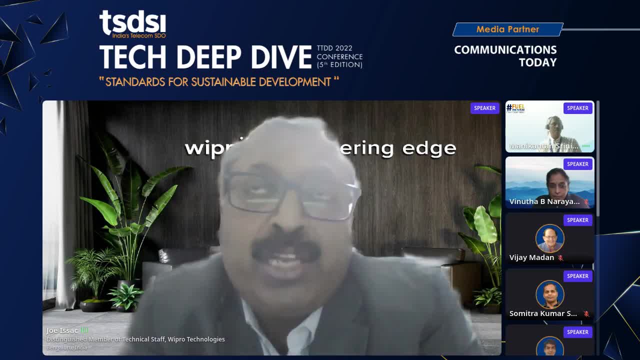 of these protocols. i think most of the applications, the new knowledge applications, have secure hashing mechanisms within the protocol, within the application, which can make it slightly more uh, contextualized from a security perspective. i think within the protocols also there's some moments of hovering on the protocol on the security packet sniffing. 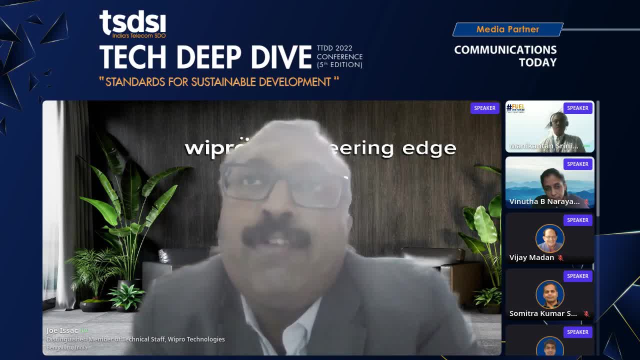 packet management is also in place, so there is some kind of thing already available. i think the place where i think we're going to have this problem is when you try to have all of these onto one common portal and have that transferred out. there we may face some problems, but otherwise 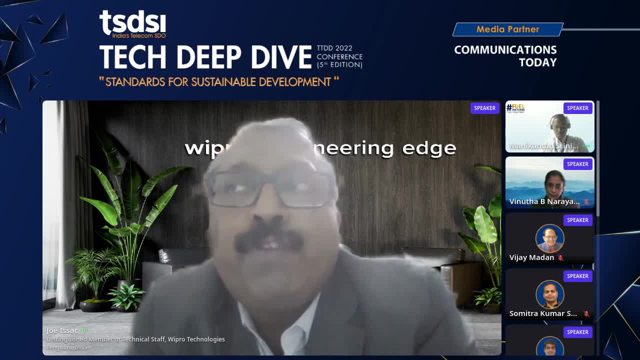 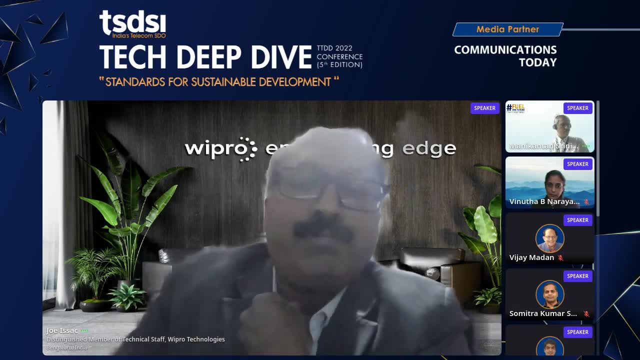 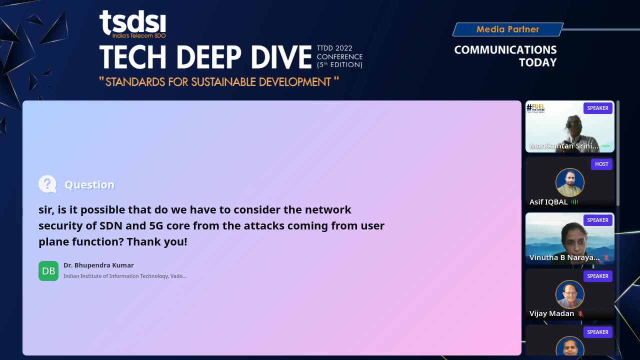 i think, uh, there will be challenges in the initial part, but i i feel that um, the existing uh security mechanisms are good enough to actually manage it. next question on that screen: yeah, i think um very valid question, um, if you look at the whole of the um the security when. 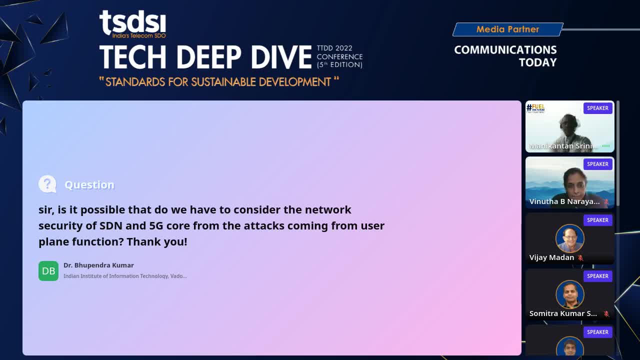 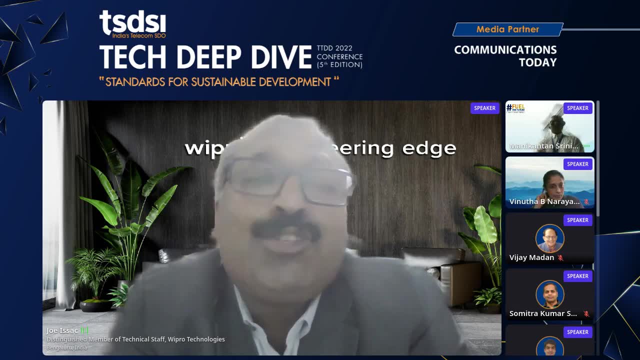 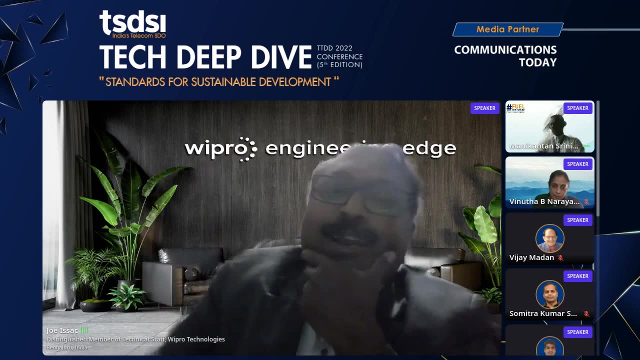 it comes not only from sdn and 5g packet core. it starts from the nfvi area itself, from the moment you are virtualizing the uh, the physical storage, to virtual and from there to having the virtual switches. i think from there the journey starts. um, it's a little little. 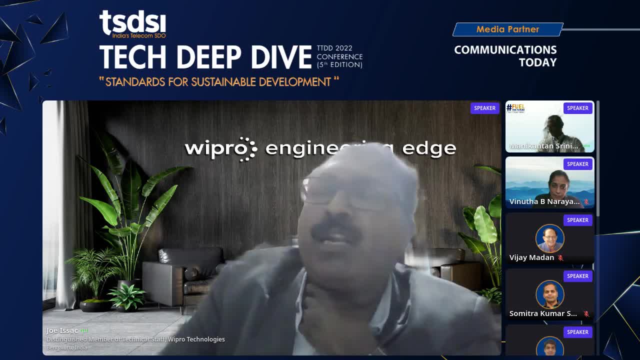 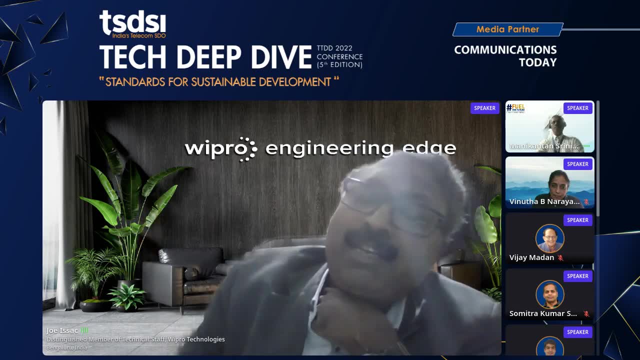 complicated. i think we have. we have, there are frameworks today available to secure that part of it. when it comes to the use of plane, i think, um, it's a little, it's a little, um, um little little serious matter, because you have a lot of these uh uh slipping going on between the, between the. 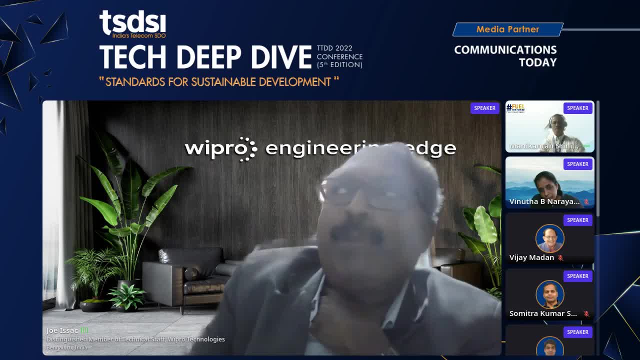 control plane and the user plane, but just the user plane. you don't know more. you don't have very much it gets. you can manage it. but the transition between off packets, between the control panel, user plane, is a little tedious. i think what i would suggest is that you would put up a virtual uh firewall there with an id is. 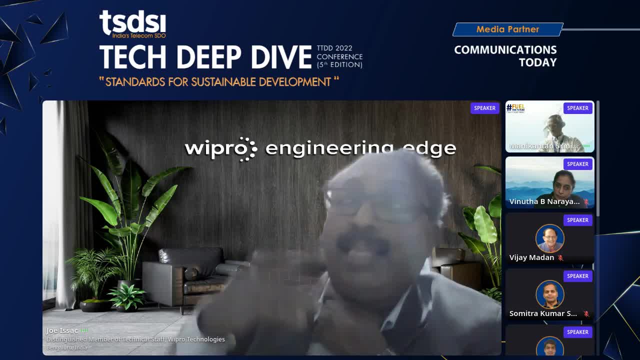 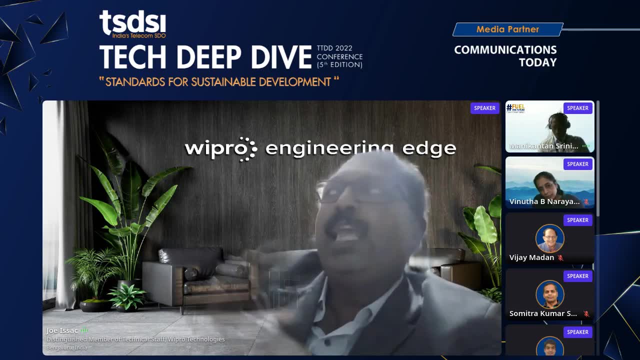 integrated and if you can orchestrate the application, the respective application, through the firewall, then there is a way to handle it on all nfva in sd networks. if you can orchestrate the application through the firewall, it takes out most of most of these issues. then you can manage it and 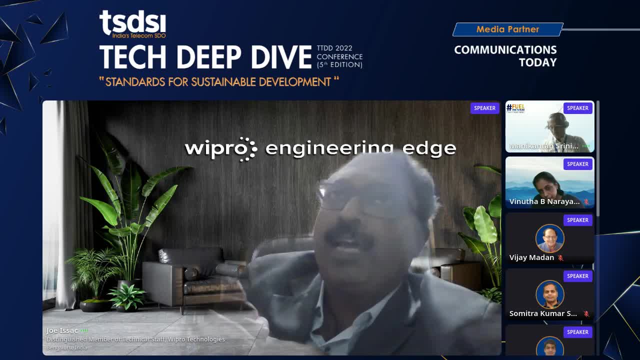 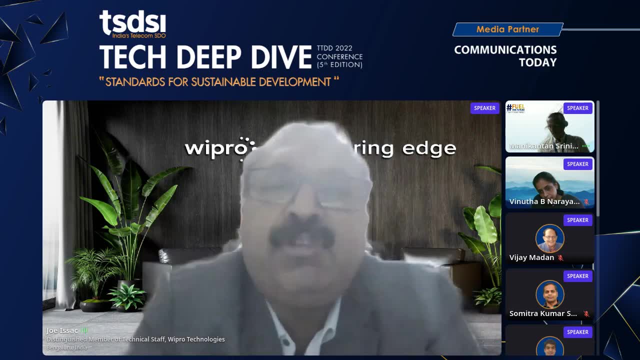 these issues. but if you were not to orchestrate the application through the firewall but leave it to the respective operators to handle it. it gets a little critical because one poc we did for the government of malaysia where we tried both, and i think the ones which applications which 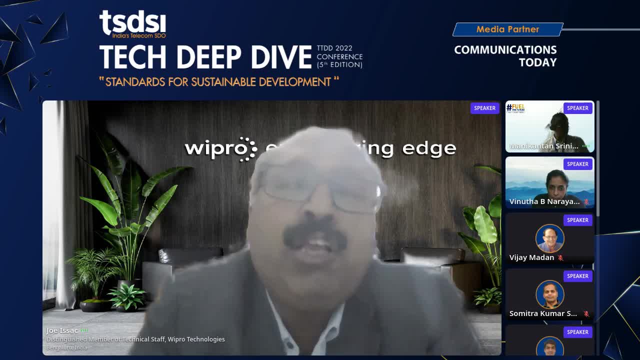 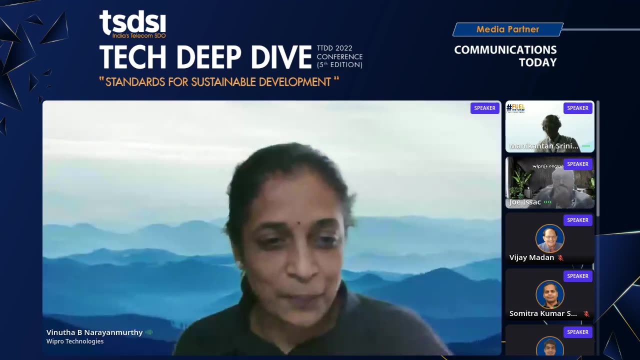 were triggered through the firewall or which were launched. the firewall were more effective than than having a mid firewall place there. okay, uh, thank you, joe, i hope, uh, this is very interesting insight, joe. thank you, i think. uh, with the sake of time, we move on to the next session. 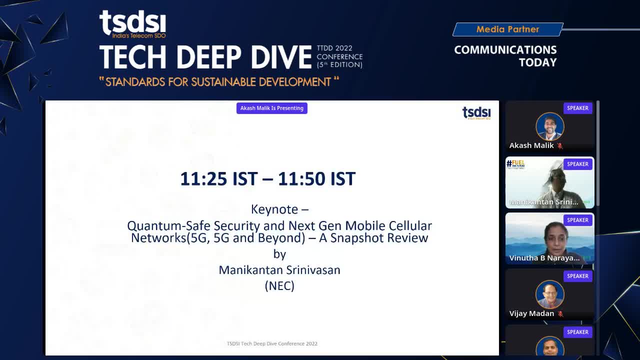 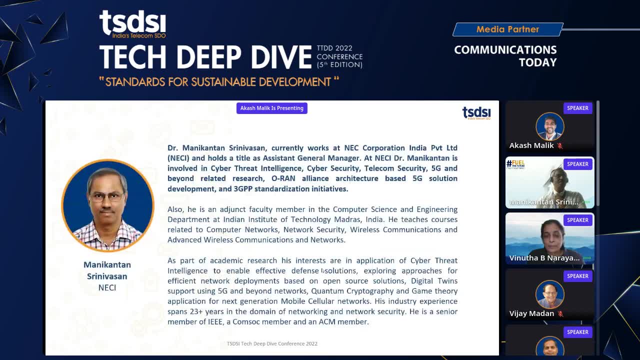 yeah, uh. the next session is by dr manikantan srinivasan. thank you, dr manikantan, for agreeing for this session. a brief introduction about dr manikantan is um. he currently works at the nec corporation india private limited and he holds the title of 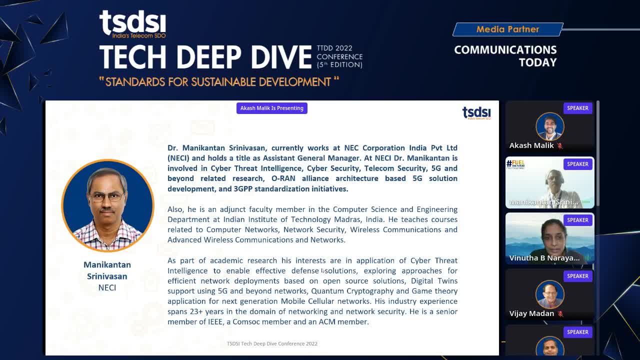 assistant general manager at nece, dr manikantan, is involved in cyber security intelligence, cyber security threat, telecom security, 5g and beyond related research over an alliance architecture based on 5g solution development and the 3g pp standard initiatives. over to you, dr manikantan, for your session. thank you, hi. thank you, ma'am. thank you so much uh. 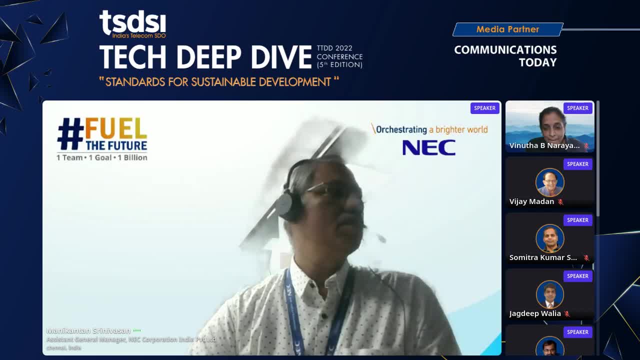 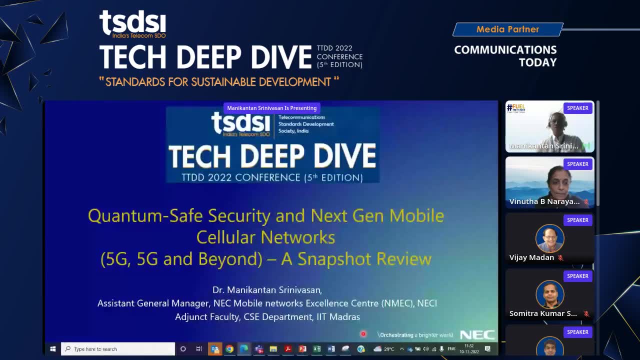 let me just share my screen. uh, in a minute i hope my screen is visible. shared screen. yes, yes, okay. uh, good morning and uh, warm welcome to everyone who is listening into this conference. i thank the chair and all the other speakers, mr joe and mr social kumar, and panel members. uh, it's certainly an honor, as mr uh social said to. 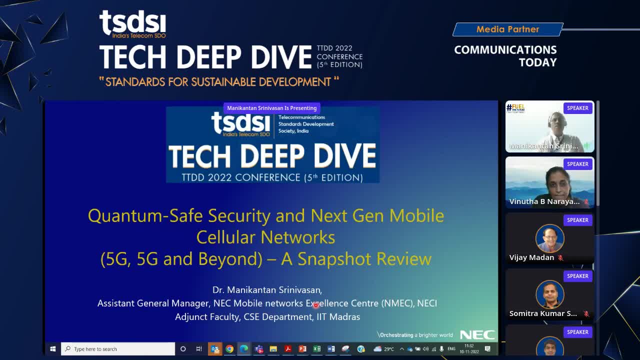 be here, uh uh, to share this floor and to share some insights to the larger audience in this uh short time in which to cover a large set of uh information. i'll try my best and i hope this will be just teasers or pointers that will help you to dive further in and get the details. so my uh talk. 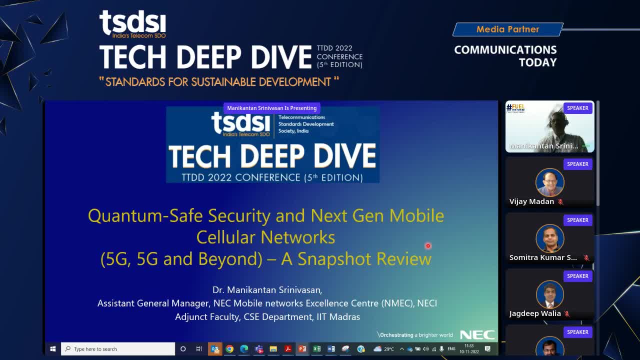 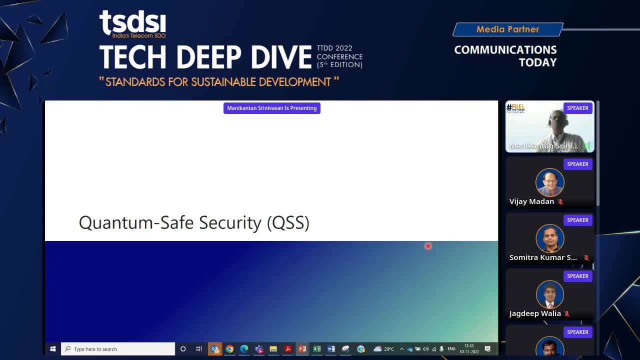 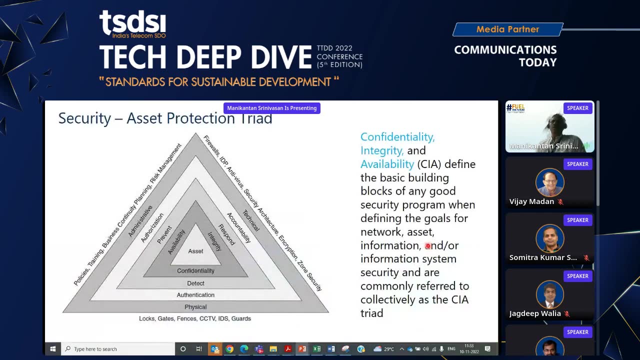 is going to be on the quantum side of the security part of it. That is related with respect to the telecom world. I have made here no assumption on the background of the audience, So I hope the steps that I take you through will help. On the very first slide we talked about security. 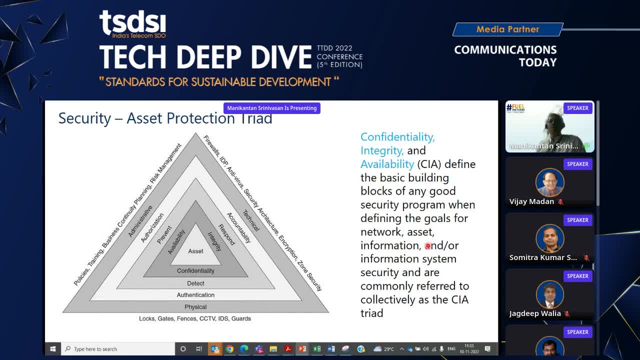 And why is it pretty much mandatory or required From a security. we protect an asset. Asset means it is a data. This data could be like a secret design that we make for our product or for our country, or even our own data, which is in the bank. 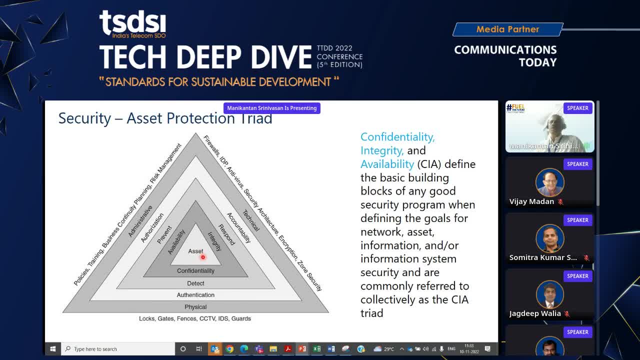 So this asset needs to be protected, which means and then it should not be changed and it should be available. So when it is protected from unauthorized access, it is basically to ensure the confidentiality Value does not get changed. is the integrity part of it? 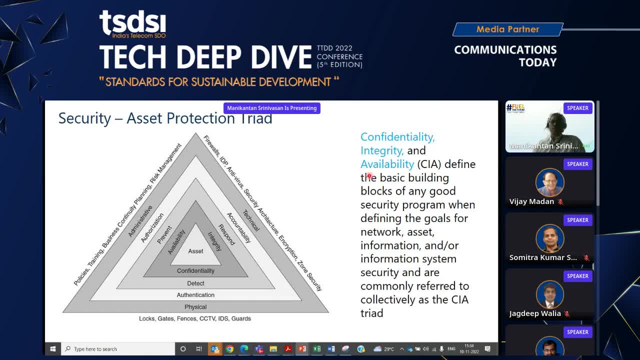 and then made available to you whenever it is needed. So this Three are the pillars of a basic security which has various ways in which it needs to be protected and applied. Here I want to highlight on two aspects: basically, this encryption related part, and then 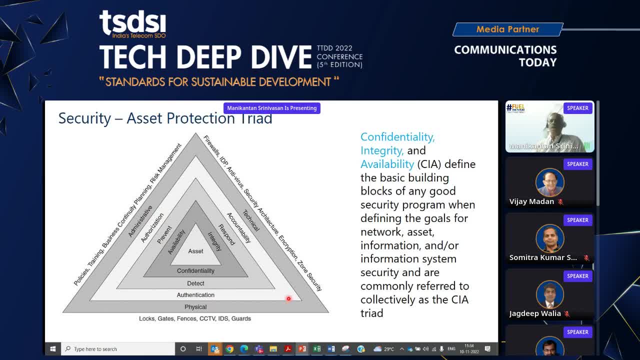 this, authentication, authorization, which are the core components of the cryptographic algorithms that I'm going to talk about in the subsequent slides. So please note. so we are going to talk more deal with respect to encryptions, decryptions and the cryptographic algorithms. 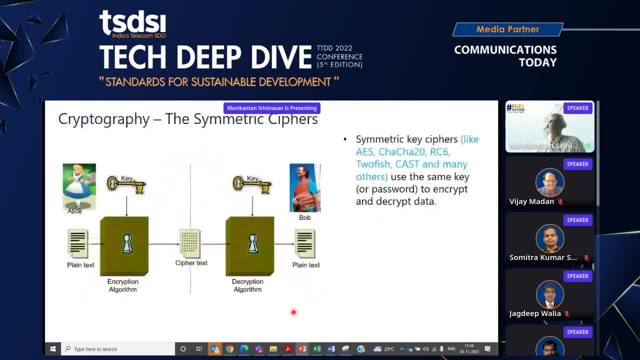 So this is a general slide Now moving further to the next one. Now, data is data can be in rest, which means where it is stored or the data moves, Like what was said by Isaac said it could be in the user plane of the 5G network. 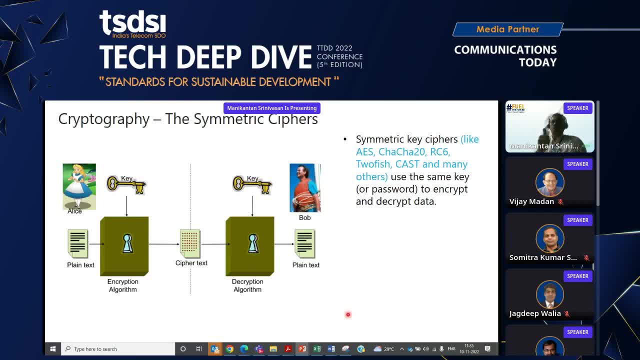 When the data flows also, it needs to be secured. One way to secure it, when the data flows at rest or in motion- is by using a symmetric encryption algorithm, And there are various symmetric encryption algorithms today. So what is symmetric encryption algorithm? 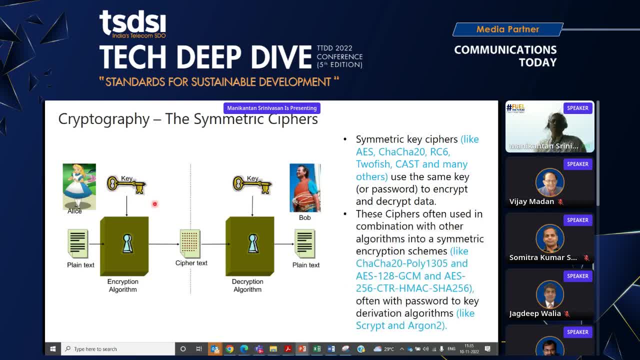 A sender and receiver both use the same encryption key and the encryption algorithm to handle their communication. Sender sends the plaintext encrypted using a key. It becomes an encrypted text. Let's see. and the receiver uses the same key. runs through the decryption algorithm. 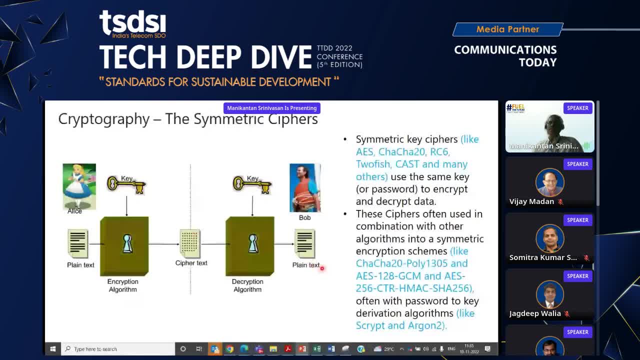 and gets back the plain test. This is an efficient way, especially when the amount of data to be sent is very, very large. So symmetric cipher is. most of the communications are done using symmetric cipher, So, but, if you observe, both of them must have this common key. 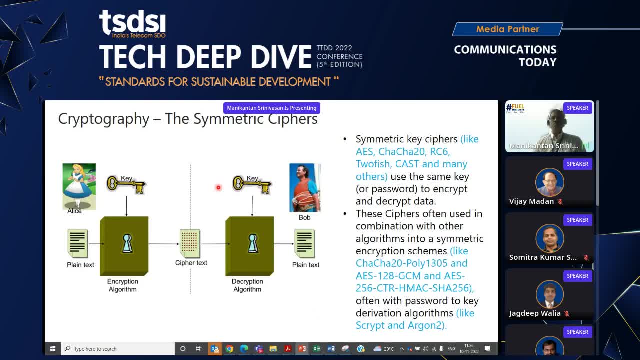 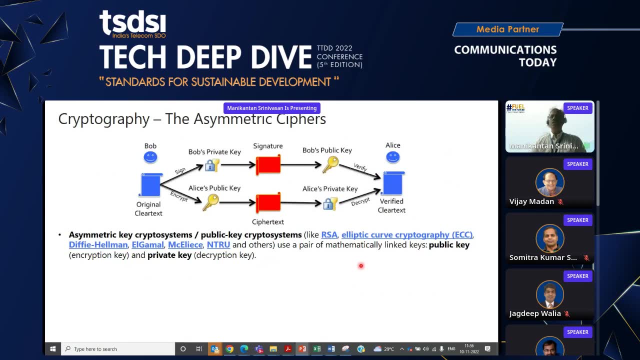 This is the fundamental challenge in the symmetric algorithms, where both sides should have this key, only known to them, and no one else should know. So this is one of the challenge, and this challenge is actually solved by this asymmetric ciphers, which was initially started by the RSA. 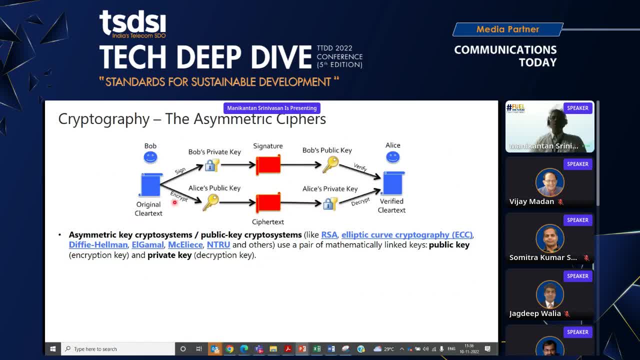 Rivest, Shamir and Alderman. So in asymmetric cipher or public key cryptography there are each member has two keys, So there is a private key and there is a public key. So and Alice and Bob, when they want to send the data. 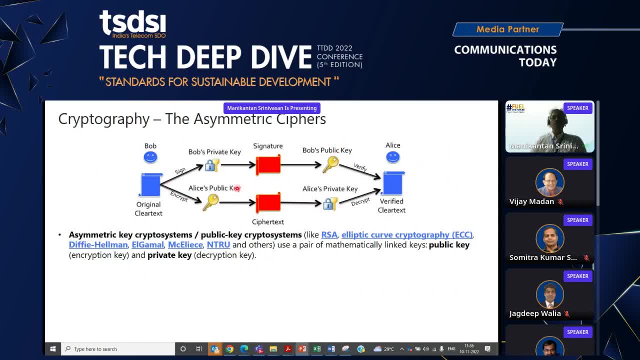 when Bob is to send data to Alice, he will use the public key of Alice to encrypt the data And for to make Alice really know that it was Bob who sends this data, he will sign it with his private key. So please note, we use both private key and public key. 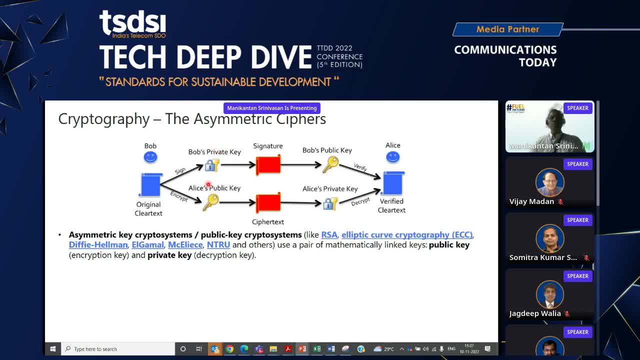 with respect to encryption, The private key is used typically for signatures. Public key is used for sending of this data, So asymmetric ciphers overcame the fundamental problem that is faced in the symmetric encryption algorithms of everyone knowing well in ahead the common key. 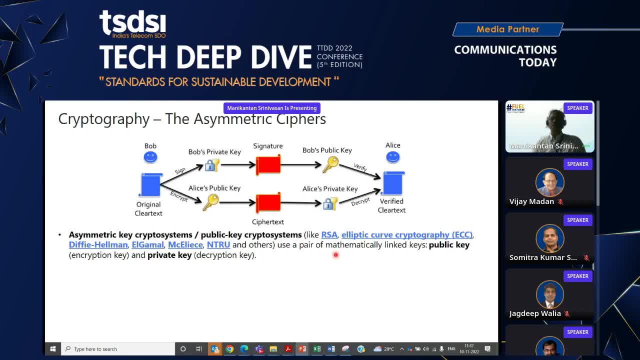 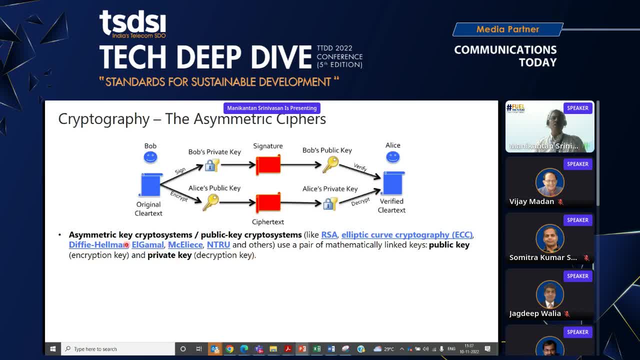 So this is. we have various cryptographic algorithms on this, such as RSA, ECC, L-Gamma, like that, And establishment of this key is done by algorithms such as Divi-Hellman to help with that. So now, as I had explained, 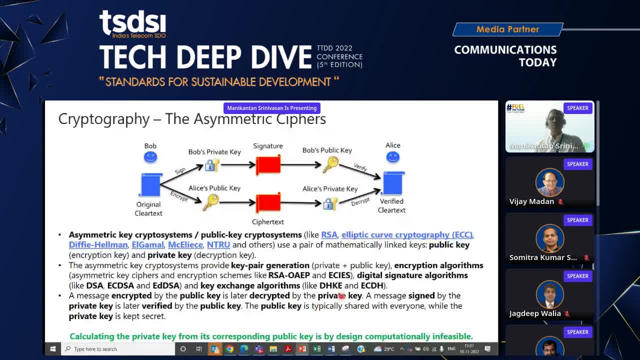 the one of the fundamental feature, one of the fundamental feature that brings strength to this public key infrastructure: are the public key based cryptographic algorithms. are the public key based cryptographic algorithms. are the public key based cryptographic algorithms. So the concept of cryptographic today is based on a mathematical concept. 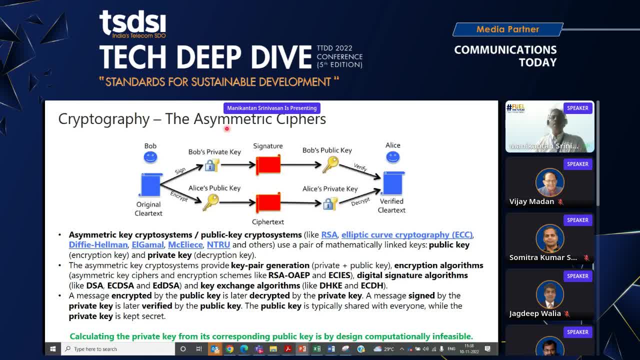 which says that one cannot figure out a private key only when they know the public key. It hangs on a mathematical concept called computationally infeasible using the classical computers. okay, So this is a key, or the very basic part. Moving to the next slide, 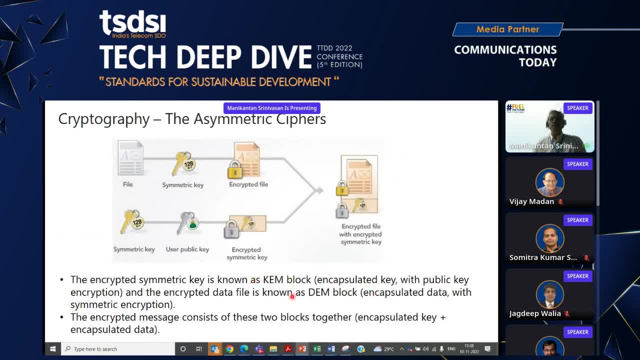 just a couple of key terminologies. just a couple of key terminologies. There is a key encryption, that is, the data that has been encapsulated. This is the key encapsulated mode and data encapsulated mode, Whenever a data has to go from a sender to receiver. 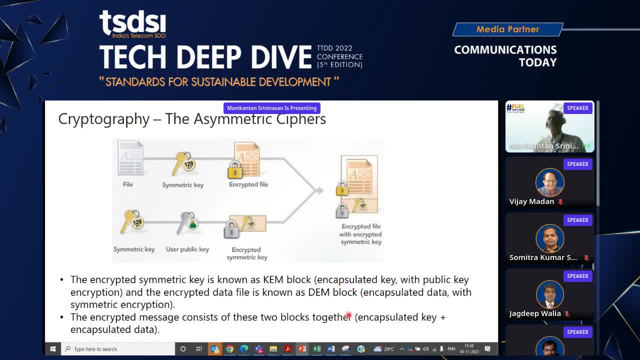 we have these two terminologies. I bring this as a reference because we'll be referring to it later. Sometimes, before we exchange the data, we will agree upon the symmetric key- that towards what the key kind of helps, And you can have it per session key to handle it. 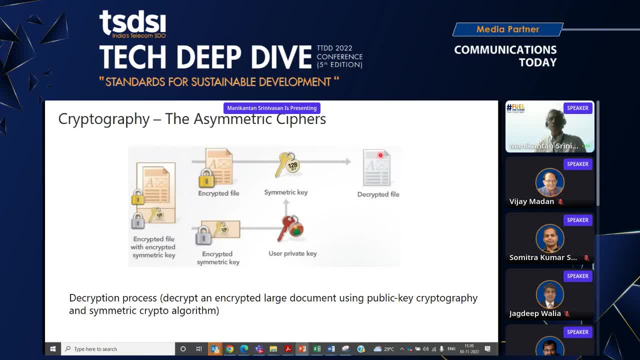 And when you receive the data and how do you decipher it. sometimes, along with the data, you can send a very specific key that you have used to encrypt, which has would have been encrypted using the public key. So the receiver, using the private key, can take this symmetric key. 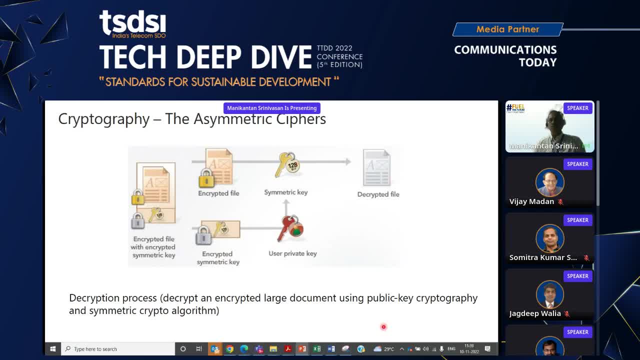 and decrypt the encrypted data and to proceed with it. This is what is being used everywhere today in complete deployment And please note, I emphasize: this has been successful today because the computational intensity challenge is based on classical computers. Now we enter the phase of quantum computation. 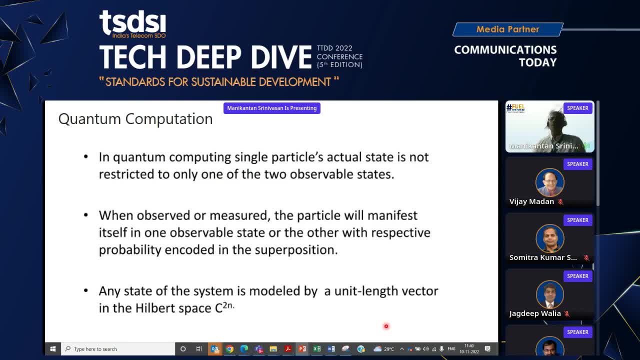 And this started somewhere in the early 90s. So we are now covering a field that has been covered close to three decades, When Feynman indicated that we can use quantum computing and create computers. the primary benefit is the power of computation significantly increases because of this concept of qubit. 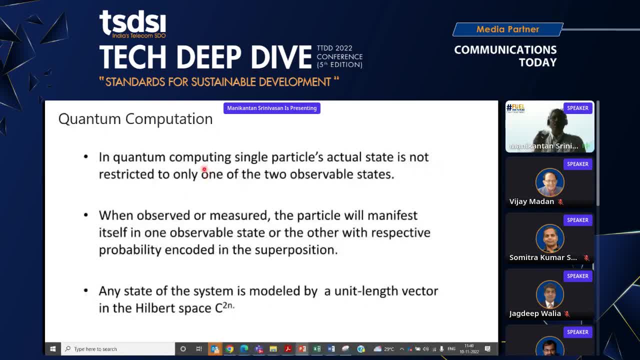 In a classical computer we have digital digit or the bit, binary digit or bit with zeros and ones, Whereas here, in the quantum state, here we have the qubit. the qubit which could be a photon or it could be an ionized, an ion in a particular state. 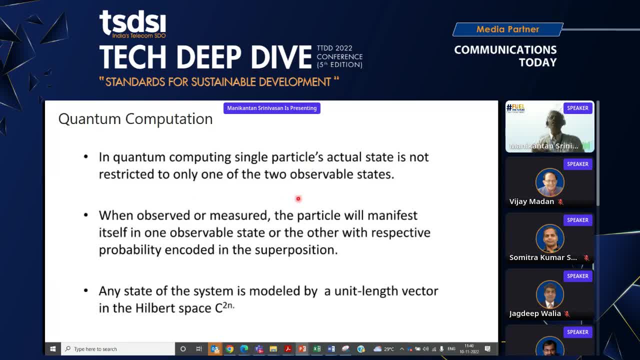 We can various ways you can derive it. It can be in any of the two observable states. OK, so ideally it can have two values and probabilistically you can get either a zero or one. So this the way In which the information held by a qubit for single qubit, you have two values and I have two qubits, then I have to power to four values and then I have three qubits. 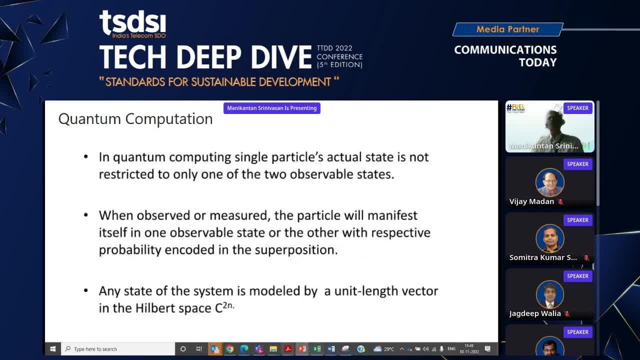 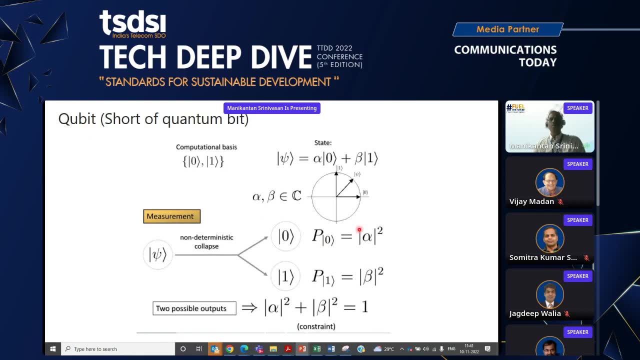 I can have to power eight. So basically, when I have many number of qubits, my amount of space or the amount of options in which I could have the values and becomes very large. So qubit, short form for quantum bit, which can be either in the state of zero or one. 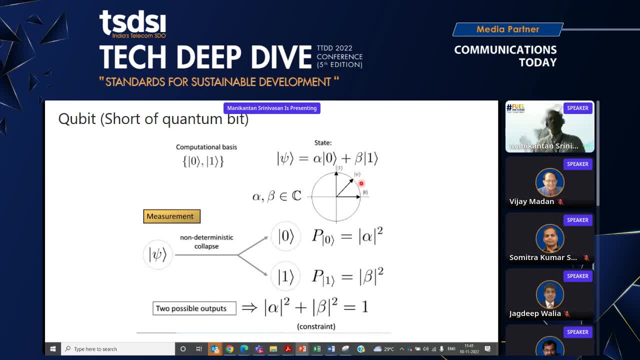 It's basically, you can consider this a photon or a part of light, light particle photon which is in a revolution, which is in a waveform, or as a particle. It could be spinning in around the Z axis, It could be pointing upward or in the down. 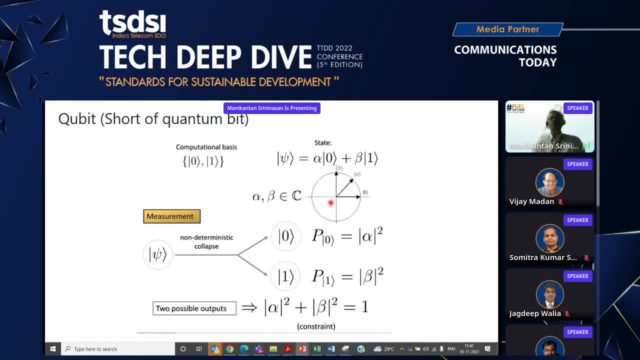 And when you make a measurement, We can figure out whether it is pointing up, which could be like a zero, or pointing in the other direction, which could be one, and it will be zero with a probability of alpha square and with one with a probability of beta square. 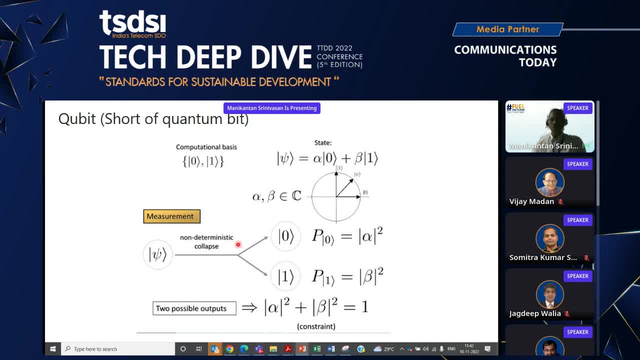 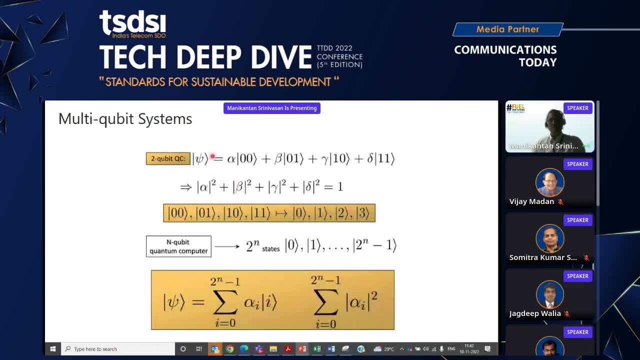 Some of their probability equals one. This is for a single qubit. We can have multi qubit systems. The first one is example where there are two qubits, Which means the qubit one in a value zero and the qubit two also value zero. 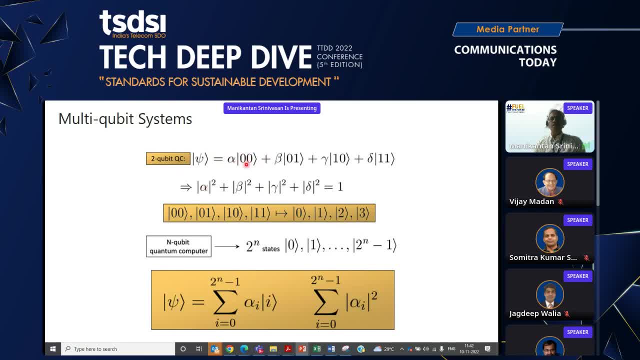 The overall with a probability alpha squared. in this state, with alpha squared Similarly, you have other combination: Some of all probabilities becomes one and you have a n qubit computer you could create Now when quantum computing was identified. It then gave rise to quantum computing. 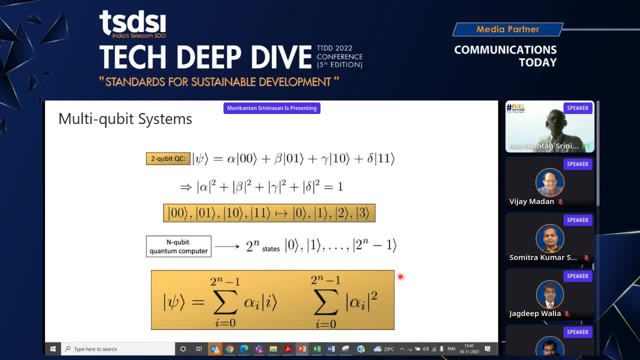 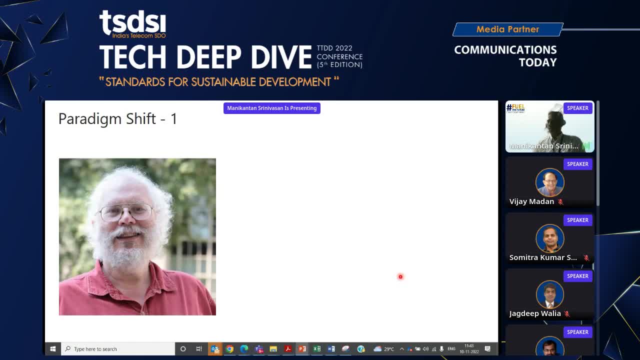 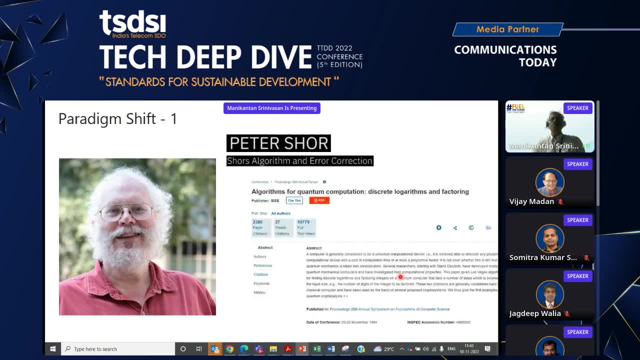 The first one is by Peter Scharr. So Peter Scharr came up and saying that there can be an effective way to factorize a given number. If you remember, I initially emphasized the public key. cryptography was based on a mathematical concept, or the computationally intensive, to find the divisor of a large number. 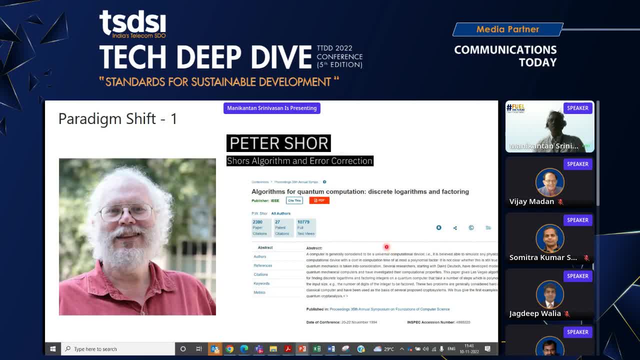 Peter Schardt in 1994 showed that we can in a very short time find the divisors of a large number. This brings in the breaking of our public key infrastructure or a PKC mechanism. So Peter Schardt, he is one of the quantum algorithm from Peter Schardt is the fundamental. 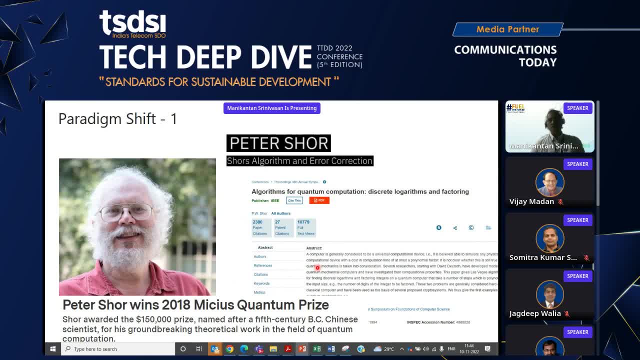 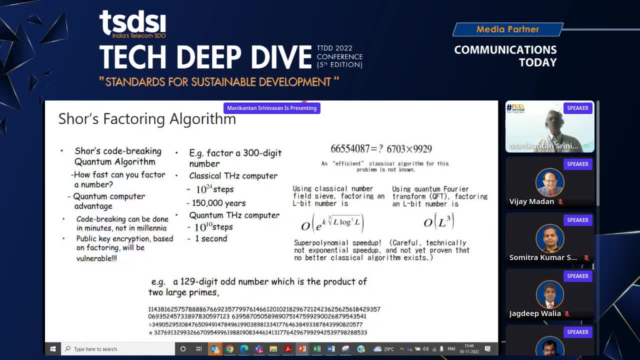 change. So this breaks the asymmetric cryptographic mechanism that you have been dealing with, Another fundamental. so this slide- sorry, before going to that, this slide which should give you a sense of it: For example, I can have two large prime numbers whose product is an another. 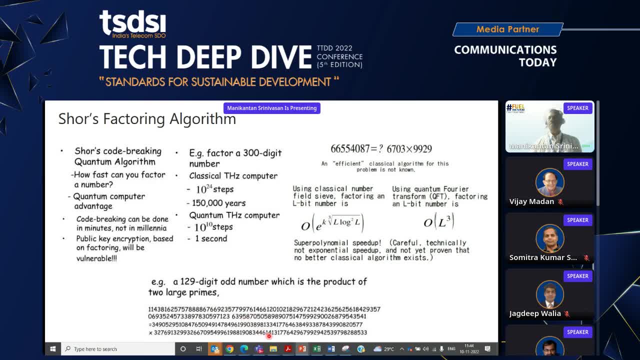 number. So this is a number of the quantum algorithm. So this is a number of the quantum algorithm. So this is a number of the quantum algorithm. So this is a number of the quantum large prime number. These prime numbers are the ones that form part of the RSA algorithm. 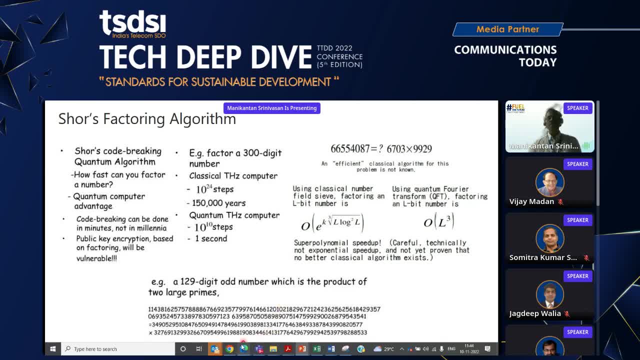 to generate my private and public keys. Now, even if I have a 300 digit number like this- now this is a 129 digit number. We have a 300 digit number In a classical computer. it will take 10 power, 24 steps, which is like, as shown here, 15,, 150,000 years, Whereas in a 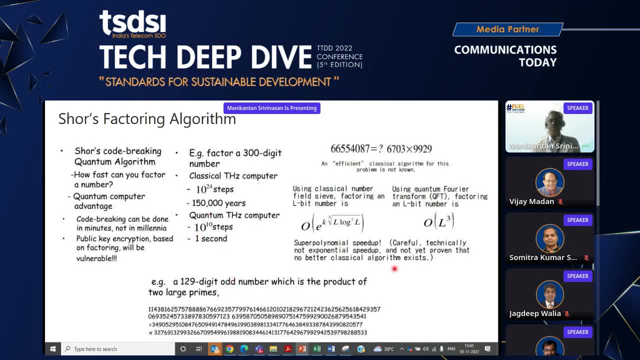 quantum computer, it could be done in one second. Basically, Peter Schardt's algorithm showed that, compared to a normal way in which you could factorize using his algorithm, which was in a super polynomial speed up, it could be achieved. So this puts us into the danger zone. 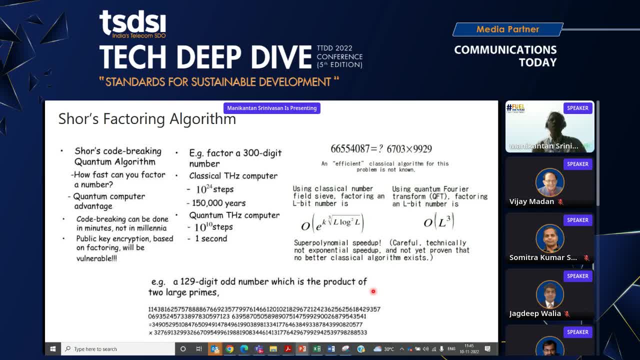 One question we can ask: do we have such a solution today? Actually, it's a solution that doesn't exist today. People are building large qubit quantum computers, but potentially it can be done. So if that computer could come in 2030, 2035, 2050,. 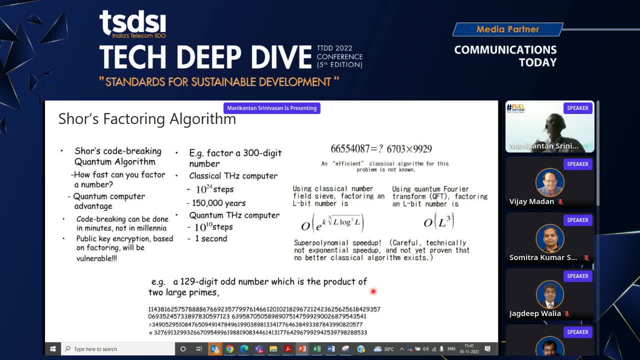 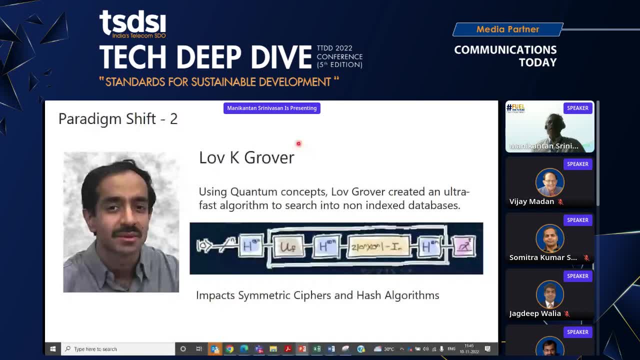 then all the public key based solution that we have created today are under danger. So the second paradigm shift, similar to that, is an algorithm derived or found by Lovegrove. Lovegrove, his algorithm, identified an effective way to find information in a large data set. 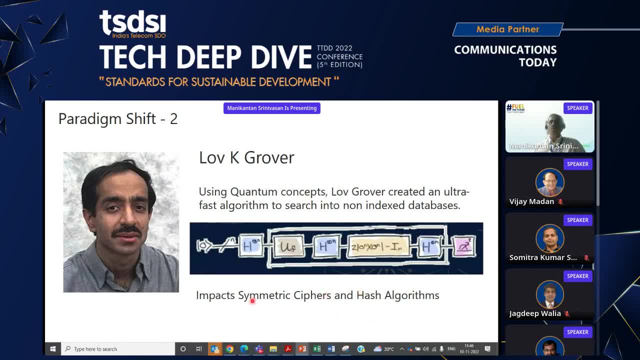 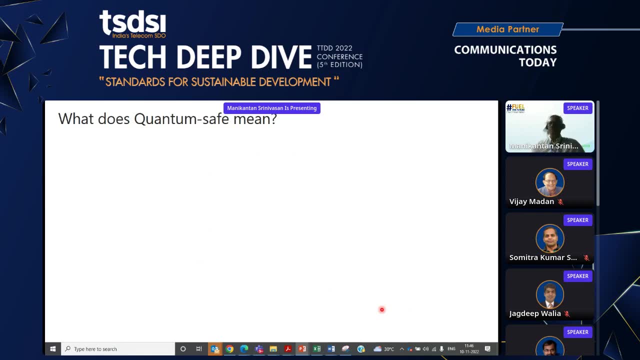 which is not necessarily be a structured data set. So his algorithm impacts symmetric ciphers and hash algorithms. So while Schardt's was on the asymmetric, Lovegrove's has an impact on symmetric and hash algorithms. So now we are forced to. 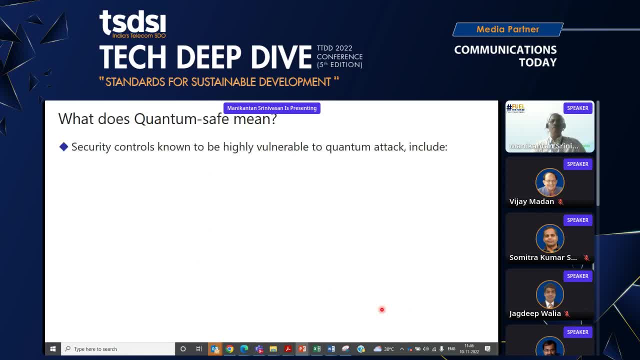 look for ciphers which are quantum safe, which means any of the security certificates like what was mentioned, and even, I'll be saying later, the newly evolving 5G on the networks, the current ongoing communication between the NFV elements, the network virtual function elements. nvnbnfs and vnfs are user authentication. This meetings, including virtual PSL functions, are bringing back emails. a message to님 on saber outside the Network As a result of игрomnf teacher at fastgather program xrm elements are being Compared with Virtual Function Family at wondering how to find information via internet. 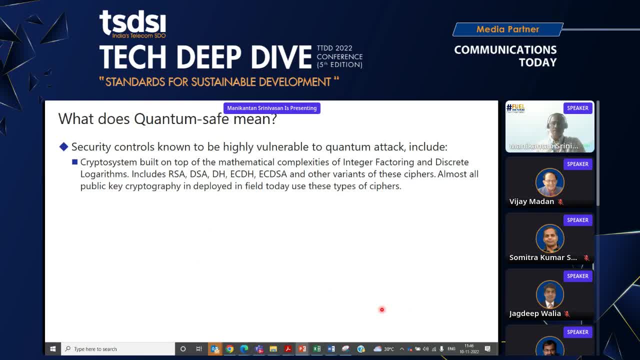 or user authentication is using public key and a private key. These are today vulnerable. One question you could ask: suppose if my exchange is done within today, it is no longer required tomorrow, which means if my confidentiality has to be for a long drawn. 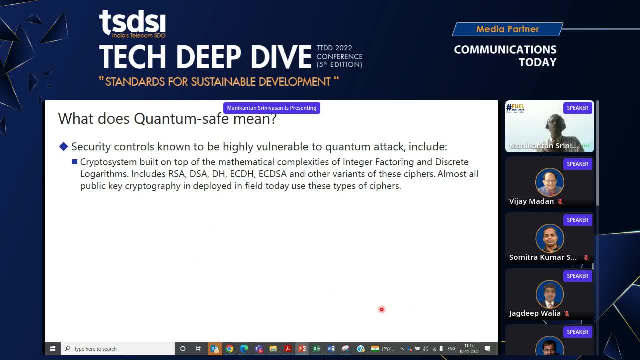 which means I have encrypted some information today which needs to be there for 50 years from now. then that needs to be protected. So that is also is what we are looking as a concern. So these algorithms that has been made using all this public. 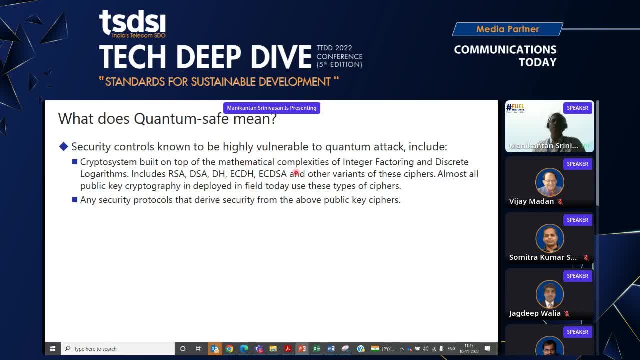 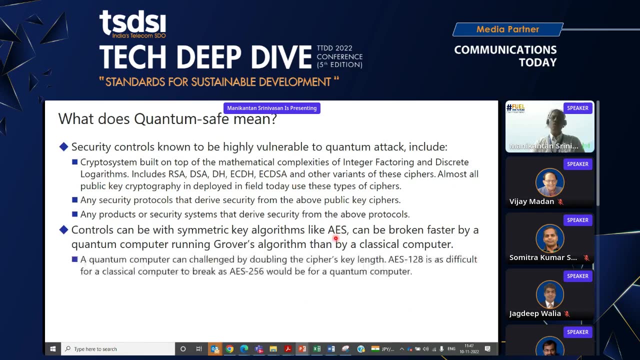 all this PKI, public key infrastructure or public key cryptographic base. they are under challenge today. Now it's not only that. as I said, a symmetric key such as AES can be broken by Grover's algorithm. Okay, But one thing is: the strength of the strength of the cipher is based on the size of the key. 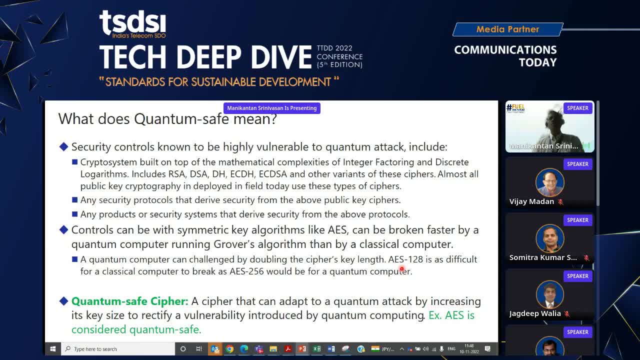 Simple example that you can see is in your house you can have a seven lever lock. Now if you make an eight lever lock, the lock is pretty strong. Similar here: if I have a key of size 128 bits, I double the key size. 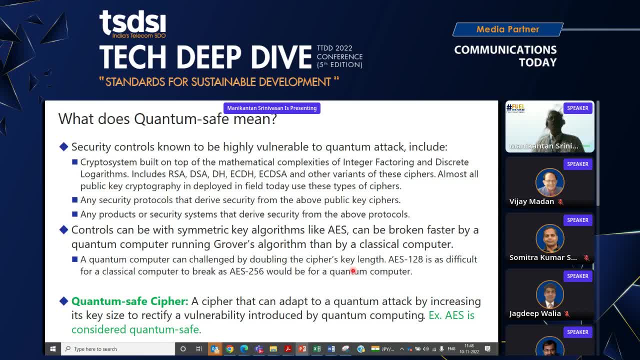 Your encryption is pretty strong, You can't guess kind of stuff. So basically, or a high level definition, quantum safe cipher is cipher, which means the encryption algorithm. A cipher is called quantum safe if it can adapt to a quantum attack. How it would adapt. 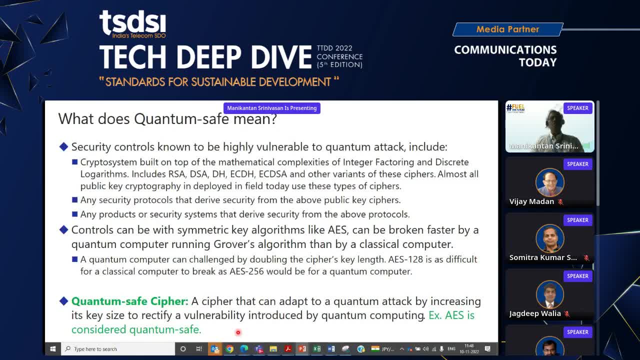 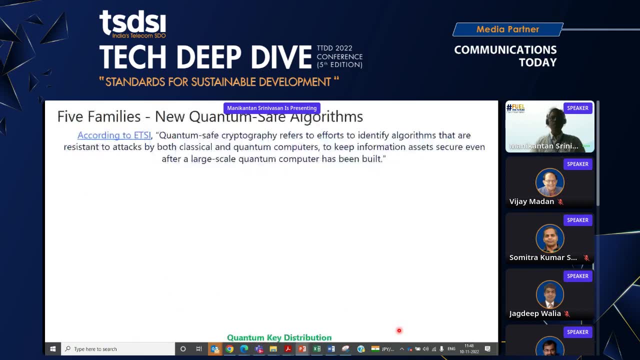 Adapt it by increasing its key size so that it can overcome the vulnerability which is introduced by the quantum computing. AES, as on date is AES 128, is considered quantum safe. It can be utilized So according to ETSI, ETSI, one of the standard SDOs. 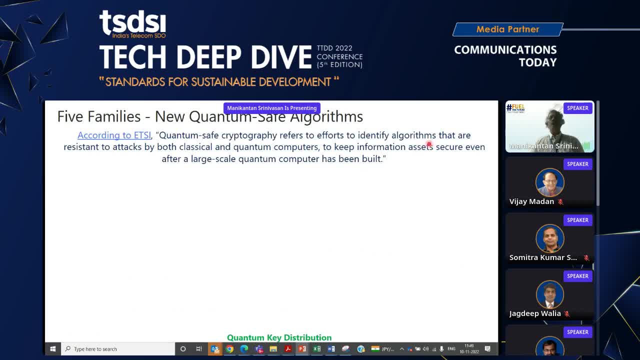 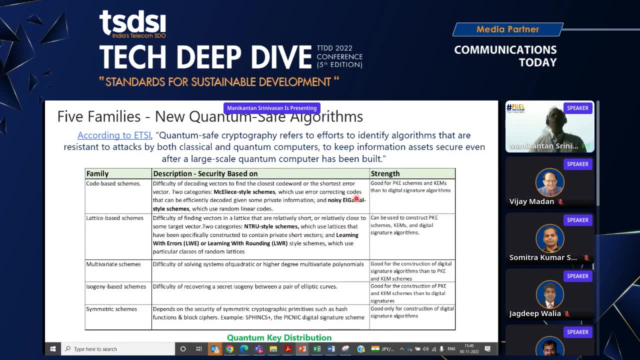 the quantum. safe cryptography means the efforts to resistant. We are trying to find algorithms which are resistant to attacks by both classical as well as quantum computers. Okay Now how are we doing it? once Peter Shor's algorithm woke all of us that public key cryptography is a challenge, 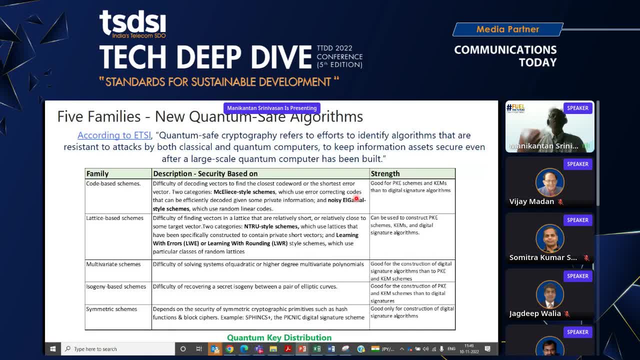 There were, there are, there are a set of families or ways in which we can derive the keys. The earlier one was mathematical challenge was leveraged. computationally problem was leveraged. Now we have other ways of deriving these particular keys. Yeah, one of them is code based schemes, where you have to find the closest to code word. 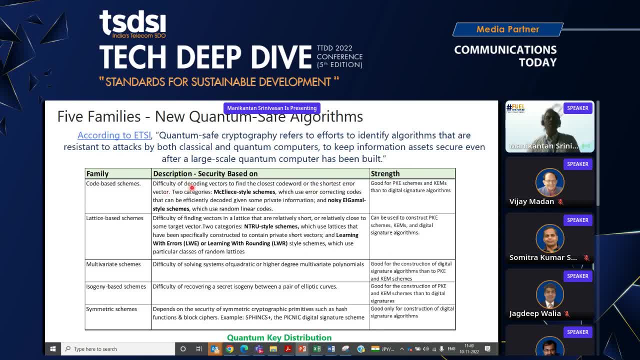 Or the shortest, the other vector. This is a challenge, So we are building where keys can be derived using code based schemes. Within that, there are two categories. This scheme is good for creating. you are the key, the both the data to be encrypted and then handle key encryption mode as well as your data encryption mode. 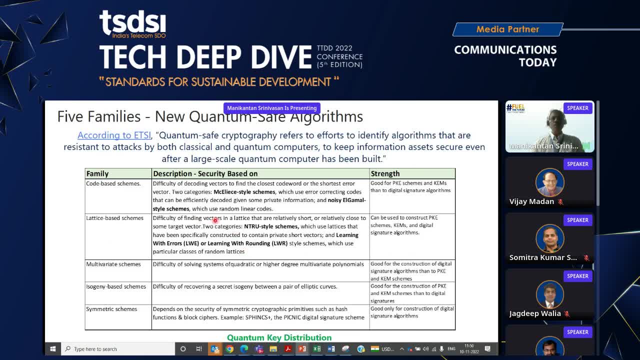 The other is lattice based. So in this lattice it is to Find the vector Which is in a enough in your space, to find the vector which is basically relatively short and close to your the size, some target vector. Again, there are two categories over here. 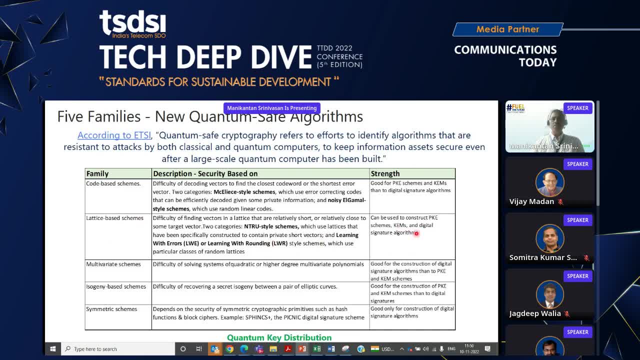 This lattice base can be used for both encryption, decryption related part, as well as for digital signatures. Then you have three others, which are multivariate schemes: isogeny, which is deriving from elliptic curve cryptography, And then, lastly, symmetric schemes. In addition to these five schemes, 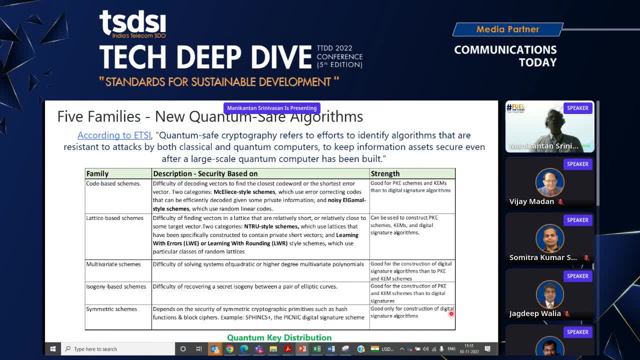 One can also share key using quantum key distribution: Q, K, D for short. So this is mean one of the ways where, using transmitting your photons, you can transmit your key from one side to the other sender to the receiver, Which is there. However, it has lots of challenges to create those transmitting. 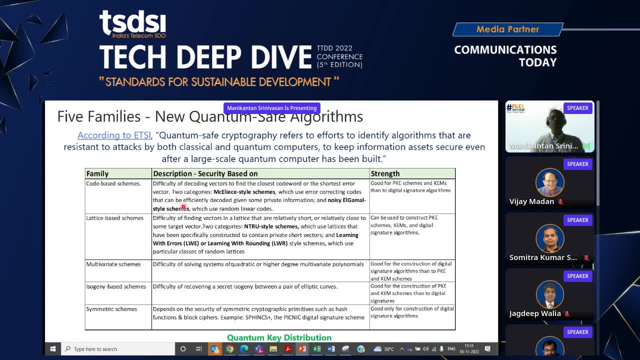 And receivers and to get the key. So, meanwhile, these five families based algorithms are work in progress, and I'm I'm talking about this because this is based on. this is where new cryptographic algorithms have been proposed to, And I ST. So Where are we today? 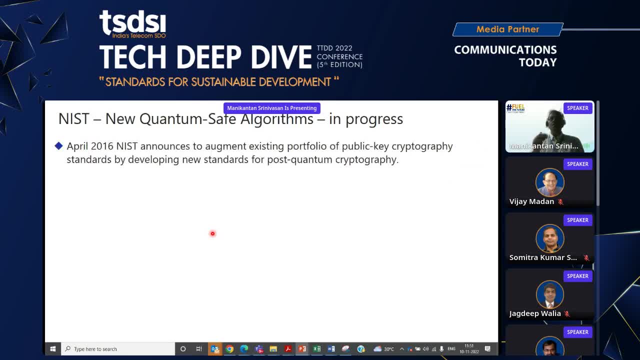 Once it was. once we found that the public in cryptography is in challenge, Then and I ST, Which is the standards body ensuring all safety, especially in the US- Unowns that they would want to identify new algorithms. Compare and yes, and similar to a yes. how can we replace other things? 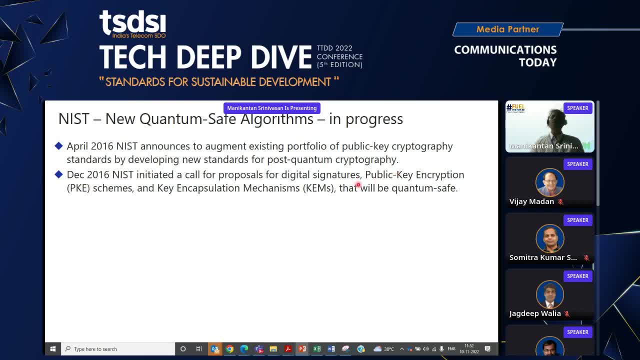 So in 2016, they call for proposals for digital signatures, as well as public key encryption schemes and then key encapsulation mechanisms that will be Quantum safe. So they are called for members to contribute, and in 2017 there were 69 contributions from across the globe. 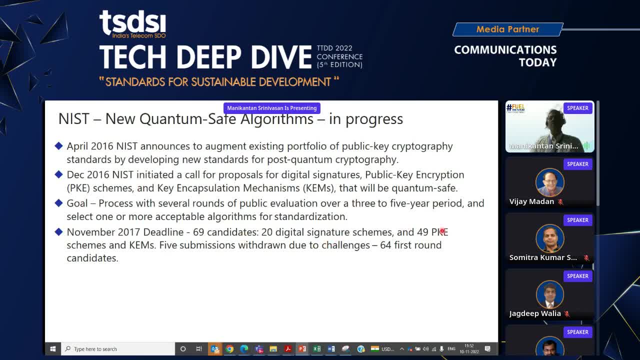 Out of which there was, 20 were for digital signatures and 49 for the public key encryption schemes, Immediately if I had challenges. so, end of the first round. there were 64 candidates. These 64 proposals Were analyzed and in 2019 and I ST. 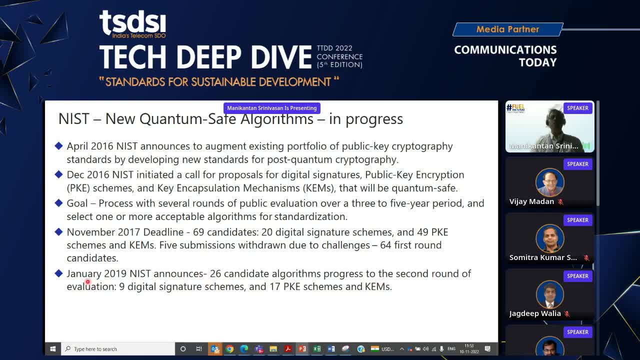 Unowns, 26 candidates are progressing to the second round of evaluation, out of which nine were digital signatures and 17 were PKE Schemes and KEM. Now, very recently, in the sense like July 2020, and the STS announced the 15 candidate algorithms, out of which seven finalists and eight alternate candidates exist, who among which will be? 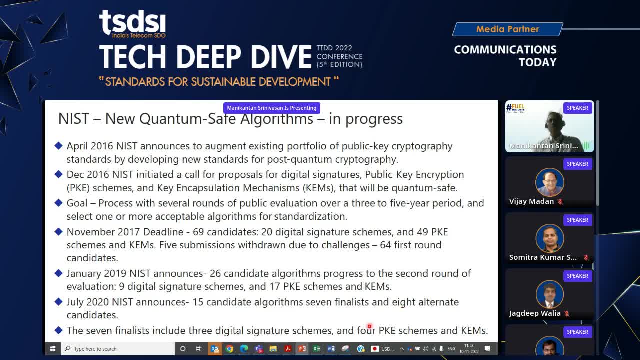 Identifying the final ones- The seven finalists- has three digital signature schemes and the public key encryption schemes. please note, when we use symmetric cryptography, it is pretty much helpful for faster encryption sending data, but to creating situations of non repudiation are you are the owner is typically not achieved in symmetric cryptography and public key cryptography helps in that particular manner. 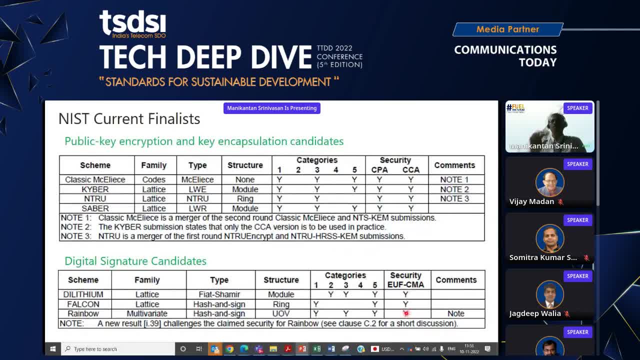 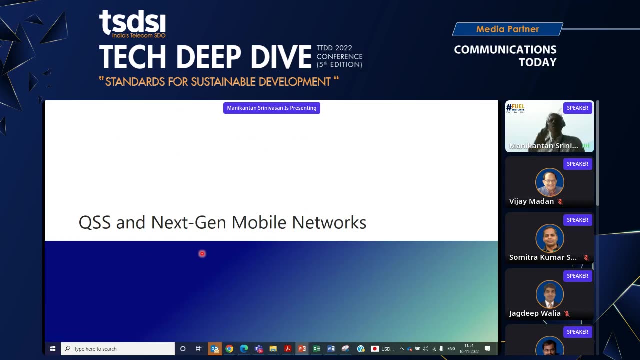 So in this slide I have brought you the highlight of what are all the candidates. if you notice here, this is the family that I talked about under the various code based, category, lattice, bit lattice based and multivariate based- the various schemes that are currently the candidates. okay, now I'm shifting gears, coming to our 5G mobile networks. 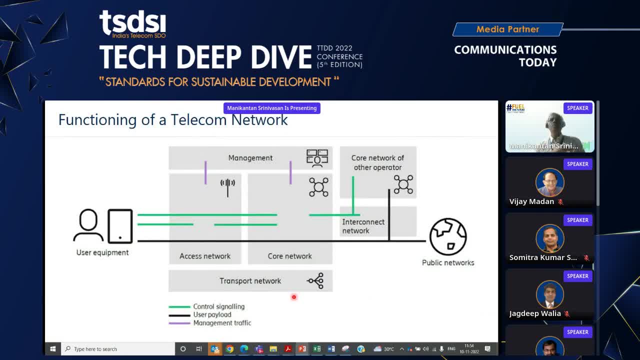 Just a Just a Just a quick view for people who even may not know about the this one. you, you have data going in. three broad planes are today, maybe four planes in five in 5G cellular network: your user plane, your control plane, your management plane, your synchronization plane, where time synchronization signals are sent in every plane. the data needs to be secure. the components that play, which has been expressed by both the 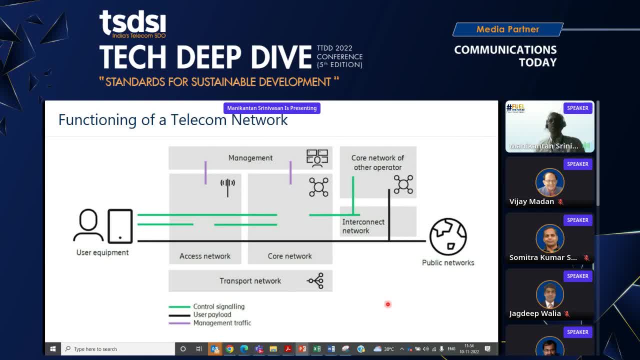 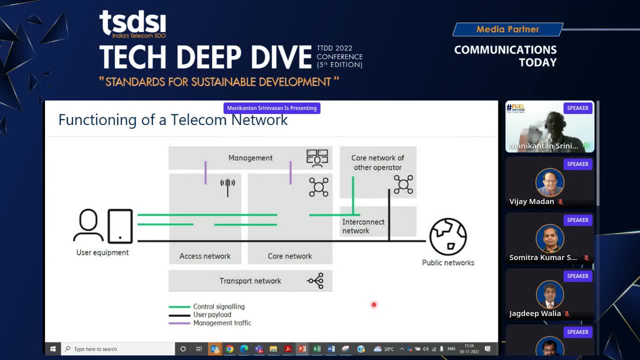 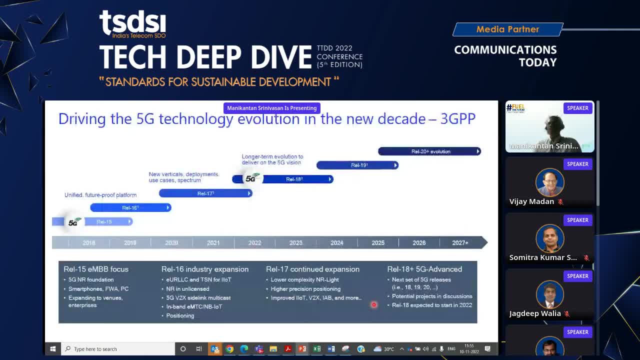 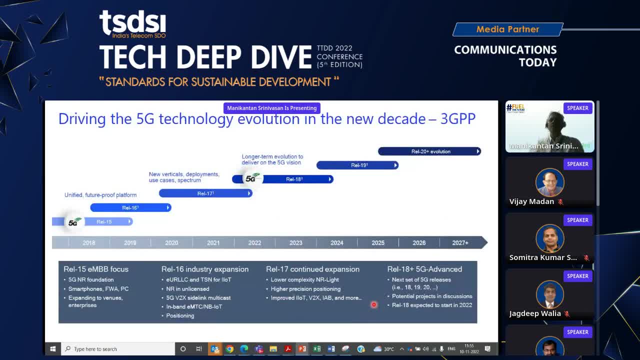 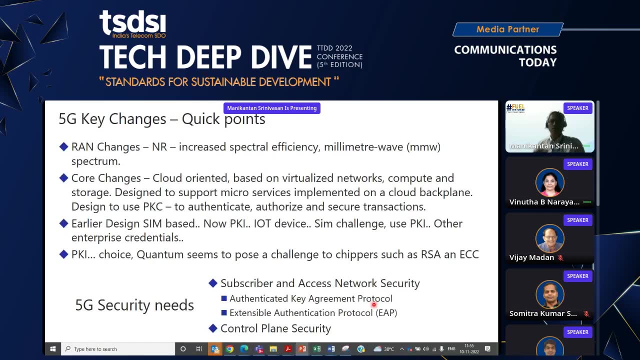 The components that play, which has been expressed by both the has been ensured that at every release, uh, things are being taken care. just this snapshot of 3g pps uh plan on the release in terms of what are the features that they are? yes, sorry, yeah, i think we'll have under five minutes, please, sure, yeah, thank you thanks. 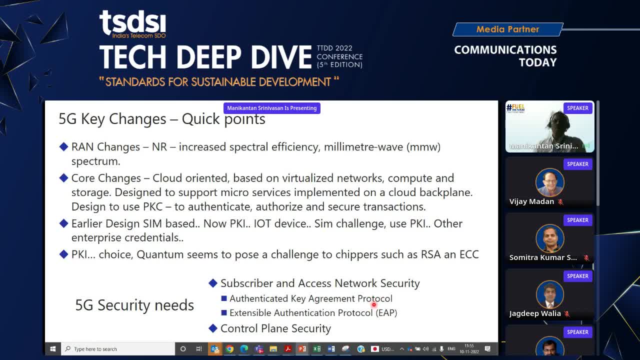 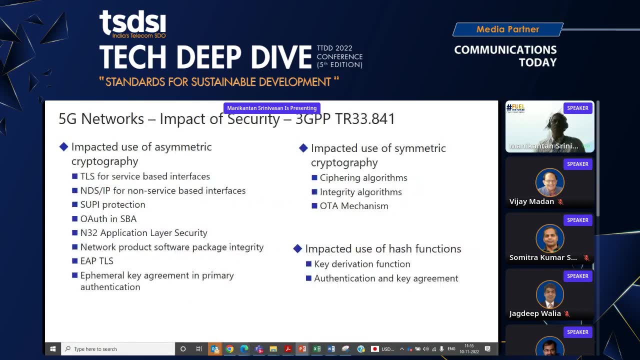 sure. so, uh, basically, uh, the we need. we have the challenges in terms of handling um, the subscriber and the network security access and ensuring that we have a key agreement, part of it. so 3gpp has done. how, uh this quantum impacts the security for the asymmetric? 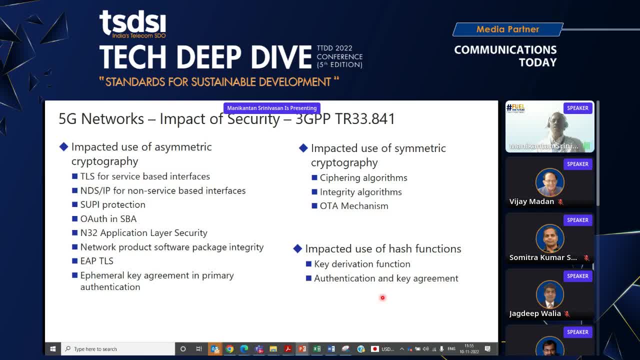 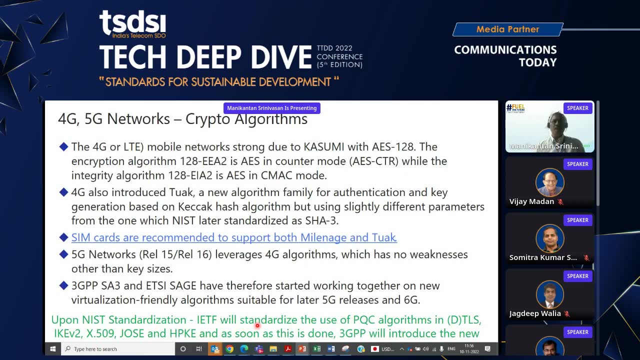 cryptographic and the symmetric cryptography and the hash functions. so this has been captured in the 3gpp technical report 33.841. now, uh, what is so? one people can ask. are we really in a concern today? maybe, uh, it's not as bad, as a 4g network has been, uh, pretty strong. there have been new, uh cryptographic algorithms has. 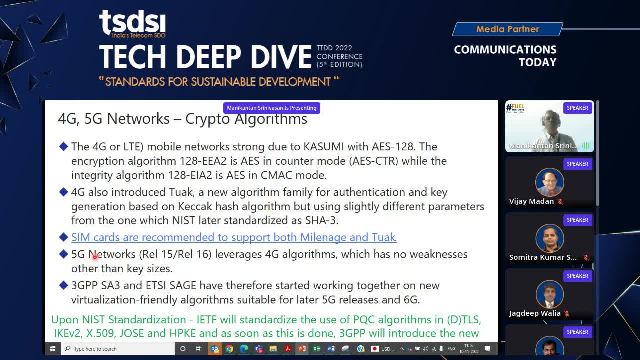 been put in place in 4g. the same is what has been used in 5g and 3gpp. sa3, which is a standards group, working along with its usage, are waiting for the nist finalization or to bring in the new nist finalization and the nist finalization and the new nist finalization and the new nist. 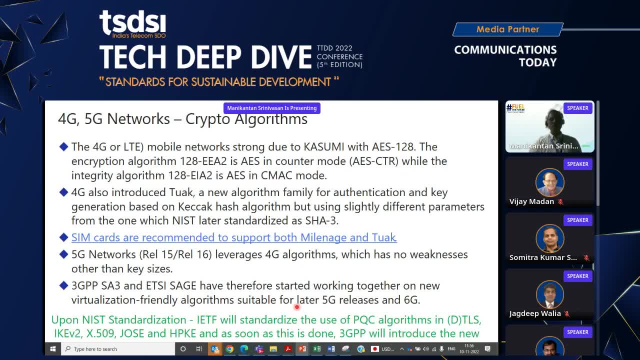 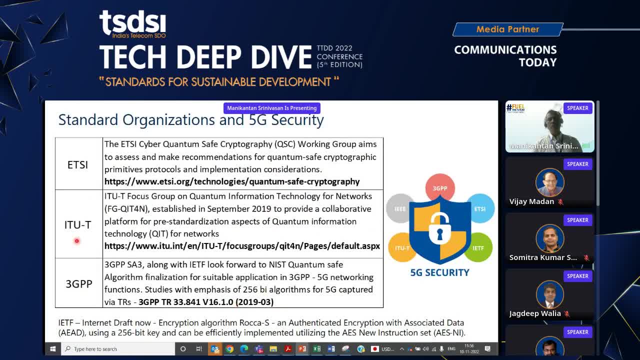 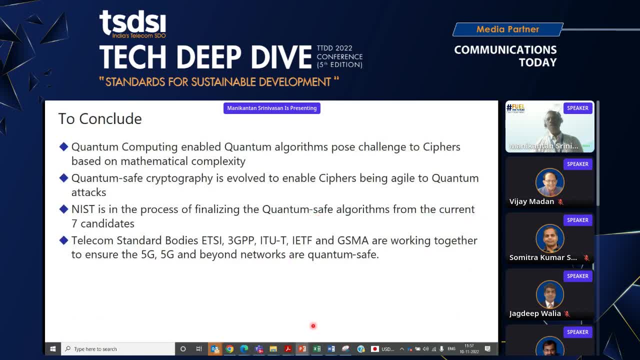 also how to transition is being done at itsy. it. ut has the standardization group to work on it and 3gpp taking care. so, to conclude, quantum compute has brought in a challenge that the cypher could be broken, and this quantum safe cryptography is. 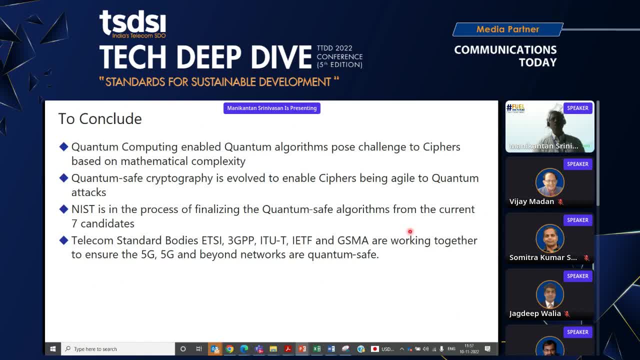 being evolved and cypher is being designed for that it could handle the quantum attacks. nist is in the process of finalizing the quantum safe algorithms and the telecom standard bodies are defining how you will migrate. also, they are waiting for the standardization and apply it. 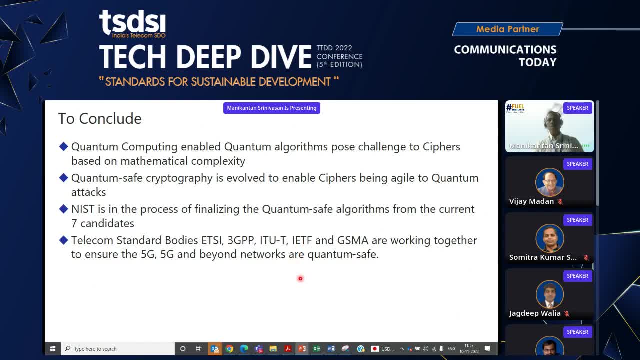 and bring it into the implementation. with this i conclude. i thanks for the time for this session provided and for your attention, thank you. thank you, dr manikantan, for taking us right from the basics of quantum computing to what has been done by the standards body and you know, uh, and how we can have a quantum safe world going forward. 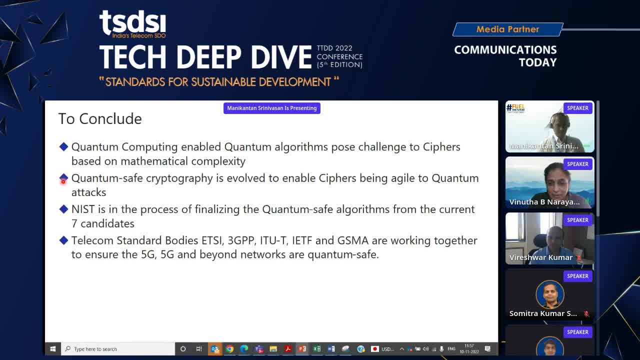 thank you. thanks a lot for taking time on this session, dr manikantan. so over to you, uh to for the next part of the session. yes, uh, thank you, vinita, and uh, thanks to all the three previous speakers who talked about 5g security, iot security and then. 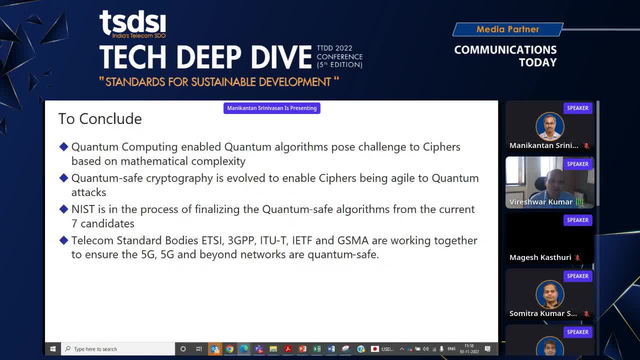 very nice, uh, talk about quantum computing and the impact of quantum computing on 5g. so thanks, uh everywhere. so now we have to look into the intersection of all these three aspects that we have been discussing, which is the 5g security, the iot security and the impact of 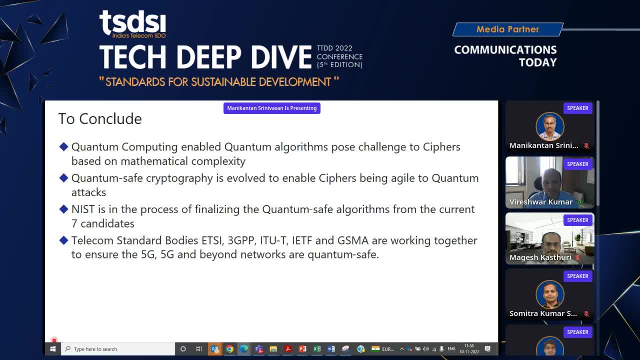 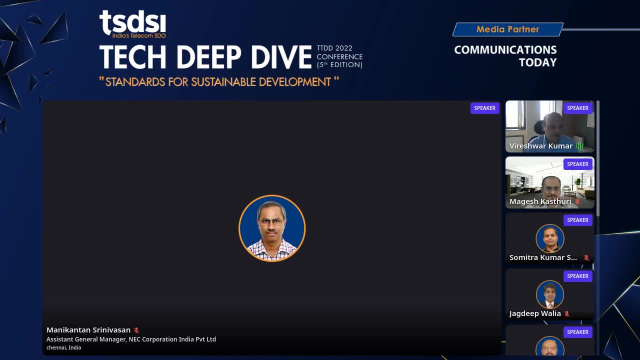 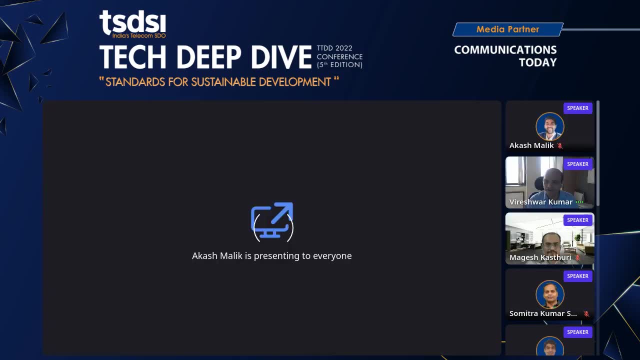 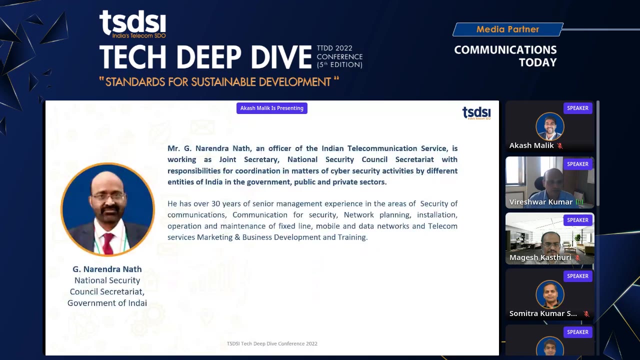 quantum on them. So therefore, the title of this panel discussion is the impact of quantum computing on 5G enabled IoT, and we have an excellent set of speakers in this panel discussion. I'm actually honored to be part of this panel discussion with some eminent panelists. So, yes, the first. 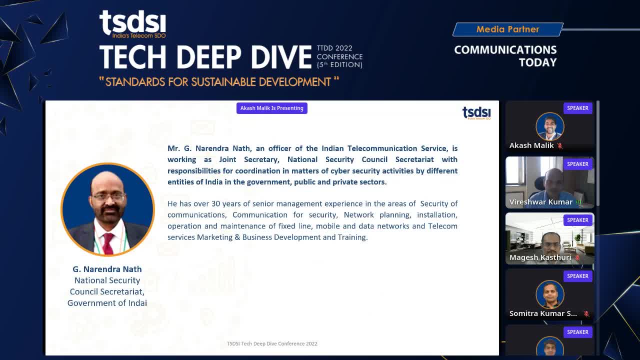 panelist needs no introductions: Mr G N Nath. he is an officer of the Indian Telecommunications Service. He is currently working as the Joint Secretary, National Security Council Secretariat, with responsibilities for coordination in matters of cybersecurity activities by different entities. 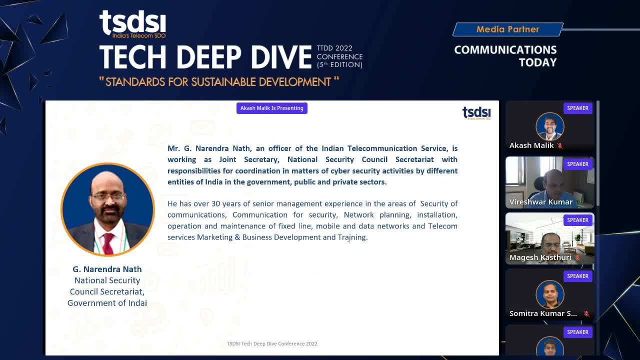 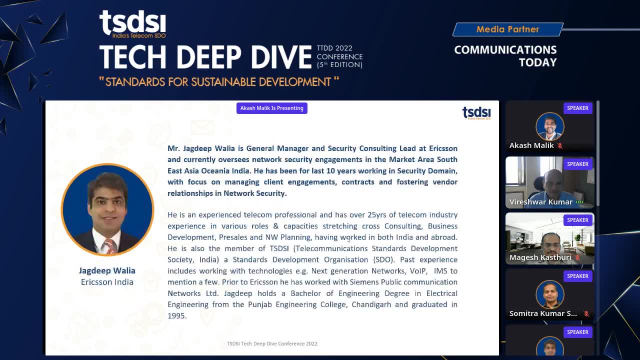 of India in the government, public and private sector. So thank you to Mr Nath for agreeing to be part of this panel. So our next panelist is Mr Jagdeep Walia. He is the General Manager and Security Consulting Lead at Ericsson and currently oversees network security engagements in the market area Southeast. 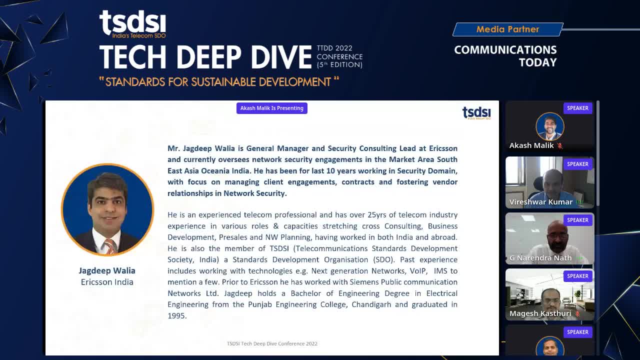 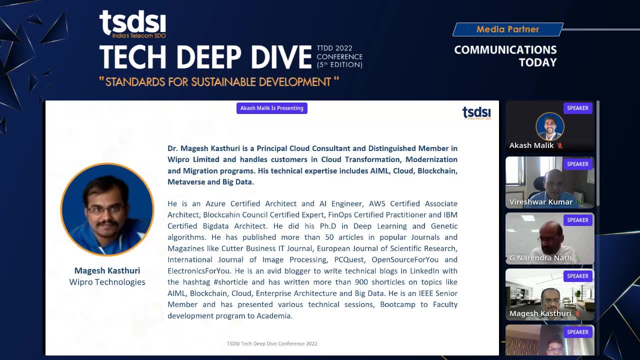 Asia, Oceanic, India. He has been for the last 10 years working in the security domain, with focus on managing client engagements, contracts and fostering vendor relationships in network security. Thank you, Mr Walia. Thank you, Mr G Nath. 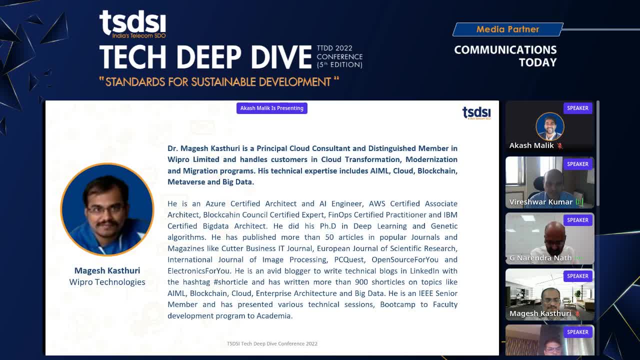 So the next panelist is Mr Mahesh Kasturi. He is a Principal Cloud Consultant and distinguished member in Bipro Limited and handles customers in cloud transformation, modernization and migration programs. This technical expertise includes AI, ML, Cloud, Blockchain, Metaverse. 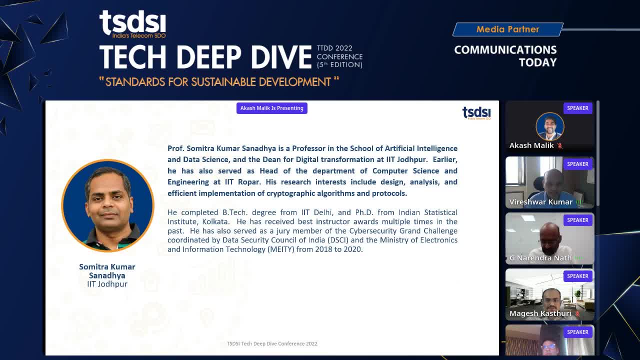 and big data. Thank you, Mr Kasturi, for being part of this panel. Our next speaker is from the academics, Professor Sumitra Kumar Sanadhyay. He is a professor in the School of Artificial Intelligence and Data Science and the Dean. 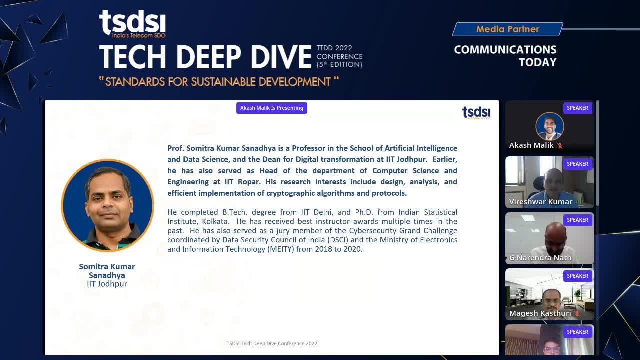 for Digital Transformation at IIT Jodhpur. Earlier, he has also served as the head of the Department of Computer Science and Engineering at IIT Roper. His research interests include design, analysis and efficient implementation of cryptographic algorithms and protocols, and he will talk about post-quantum crypto specifically in 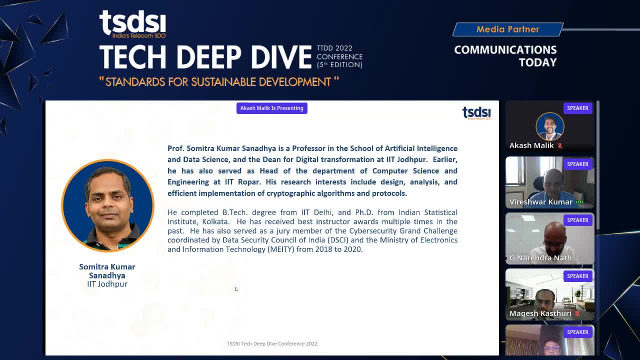 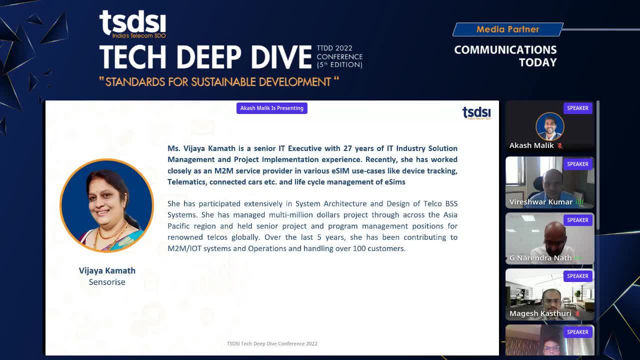 this panel today. So thank you, Mr Sanadhyay, for joining us. So last we have Ms Vijaya Kamatha. She is a senior IT executive with 27 years of IT industry solution management and project implementation experience. 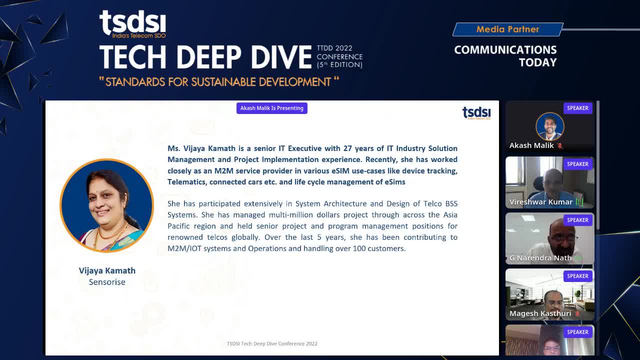 Recently, she has worked closely as an M2M service provider in various ESOs and IT projects. Thank you, Mr Sanadhyay. She also works on IT-related applications for VCs, eSIM use cases like device tracking. 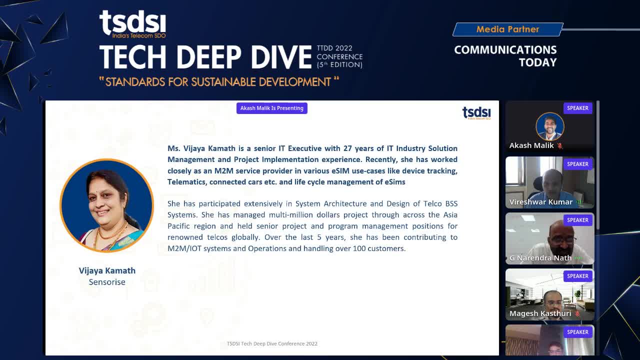 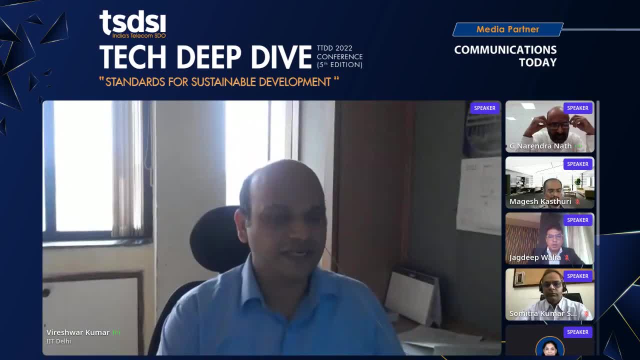 telematics, connected cars etc. and lifecycle management of eSIMs. So thank you, Ms Kamatha, for joining us. So I guess now we are in a stage where we could start discussing, so I should first go to Mr Nath. 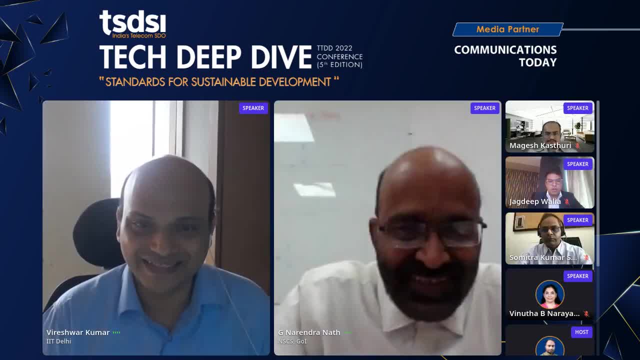 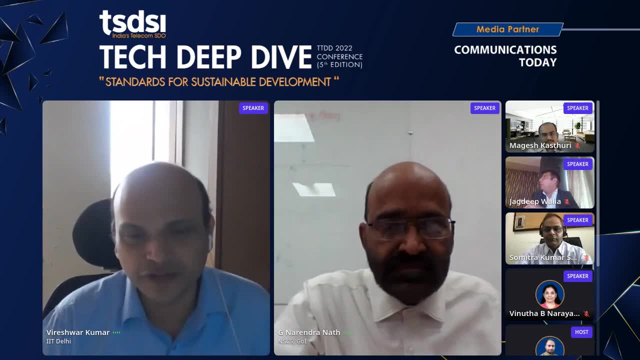 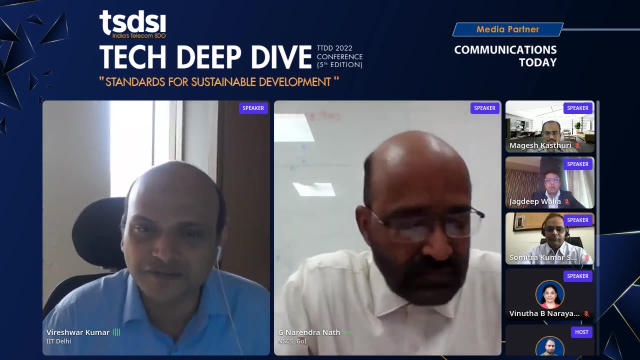 Mr Nath, welcome to the panel. Thank you very much. Yes, Thank you. Yeah, yeah, you are audible. Yeah. So, Mr Nath, I will start with you. So let me first start with the aspects of 5G security. only So, 5G will connect billions of devices with 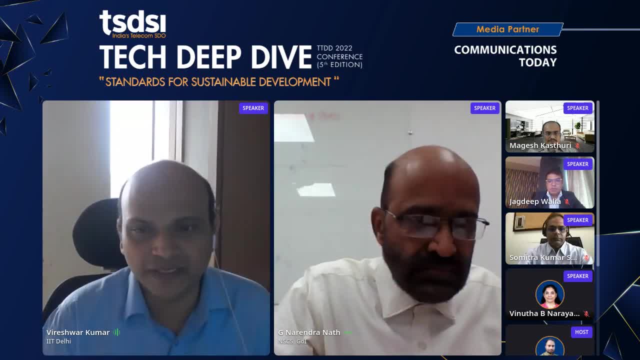 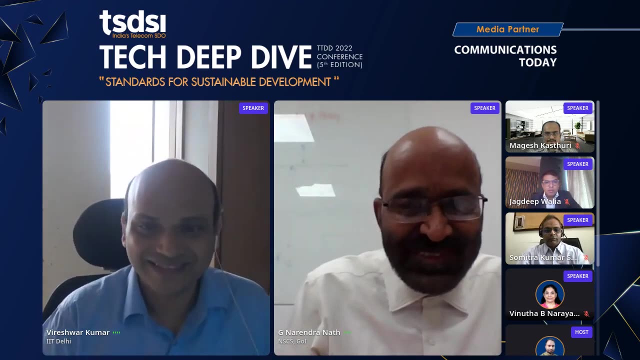 more than a billion people. So can you highlight some critical security challenges in making 5G networks robust against malicious threats? Yeah, thank you. I think you know people have been talking about 5G security for quite some time now, you know, and we tend to repeat. 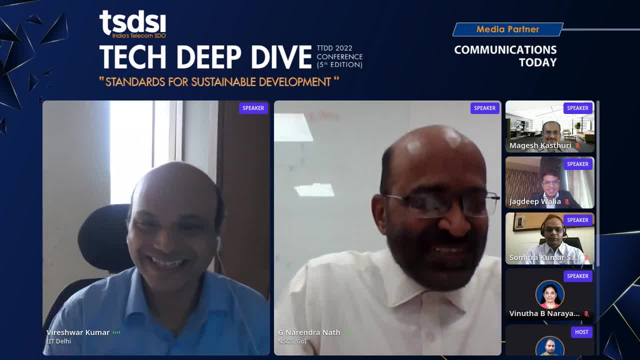 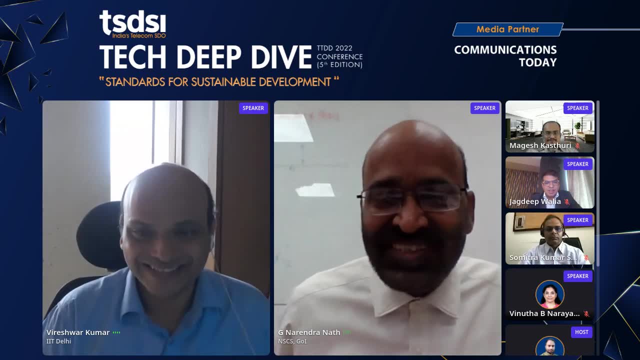 ourselves in various forms. So, from your perspective, what are the key challenges? It's not that you know- and somebody was mentioning that- So I was saying that you know- you just can't get fresh insights. You have a fresh audience, So you give the same insight to the new. 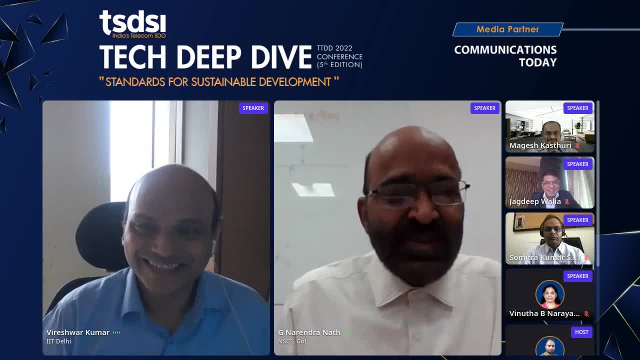 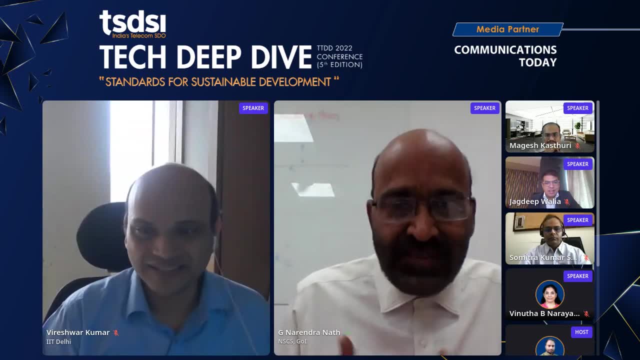 audience. So, but the problems remain. you know, whatever problems are there, you present it to and then we discuss about that. So I'd say, you know, we have a very eminent panel and a very highly technical panel which is there. I'll bring a perspective which 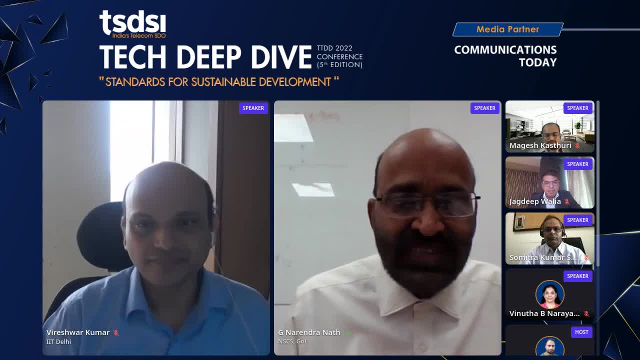 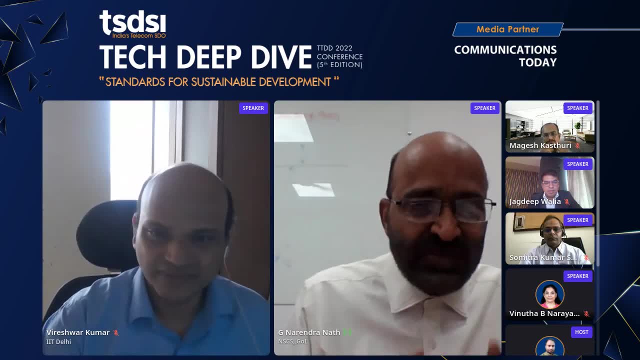 is from the National Security Council Secretariat perspective, about what it is. You know, one of the things what's coming up with 5G is. you know we have this five private networks that we're talking about. There are lots of private networks that you know we're talking. about. So you know, we have this: five private networks that we're talking about. There are lots of private networks that we're talking about. There are lots of private networks that we're talking about. There are lots of private networks that we're talking about. 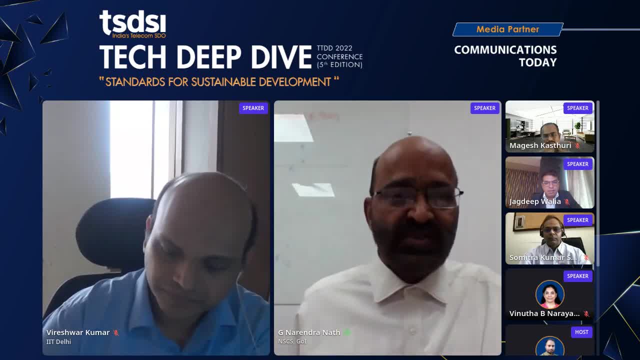 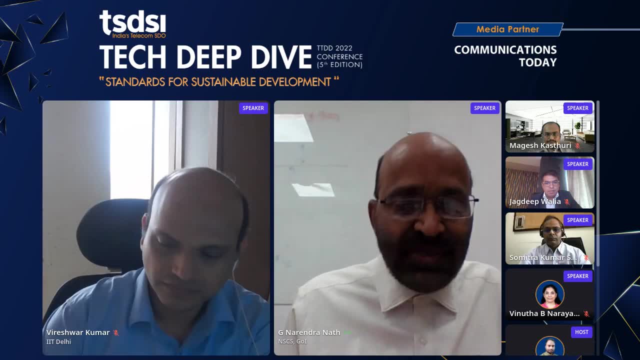 And we could also have, you know, smaller players who would come up with their own solutions and who would start deploying that. So that is one scenario that we would have. Then the other thing that we talk about is that, you know, 5G would have a lot of distributed 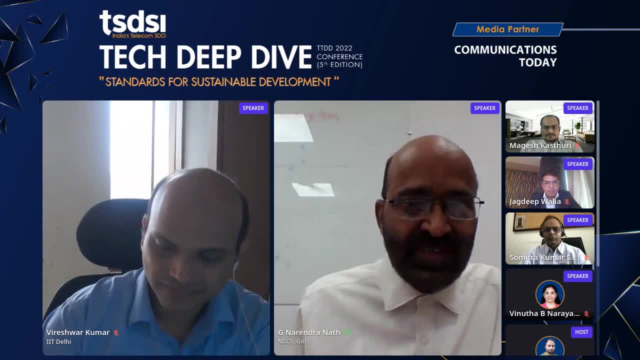 architecture with edge computes that is coming about, which is different from earlier 4G networks and other networks that we already had. Then we also talk of, you know, low latency applications, where you have remote surgery and mobility applications, which are coming up. We also talk of cloud security. So these are dimensions. They don't have to be. 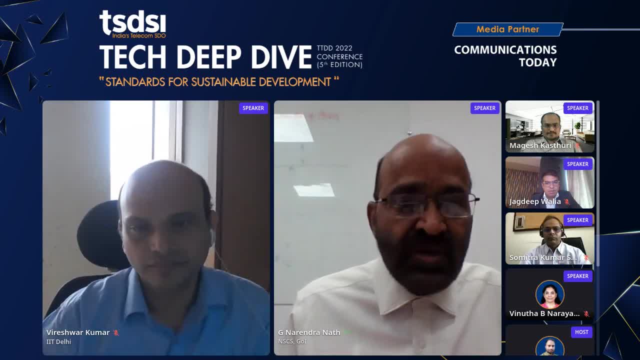 that keep coming up. And the other is, you know, IoT also. parallelly, IoT also is getting deployed, So you'll have lots of this data that's getting generated, And then we talk in terms of: you know, how do you protect the data, both at the edge and when it goes? 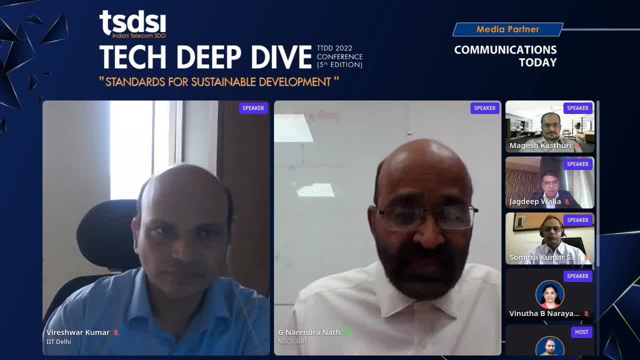 into the cloud in transit. That is one. The other thing- new phenomenon that will come over is data sharing and consent management. that will come about because we will start thinking about using this data for public good And then, you know, we start putting. 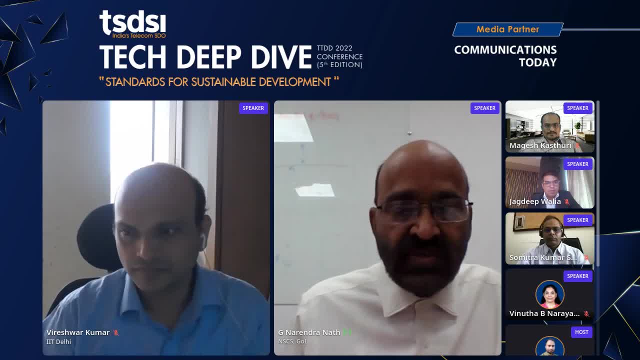 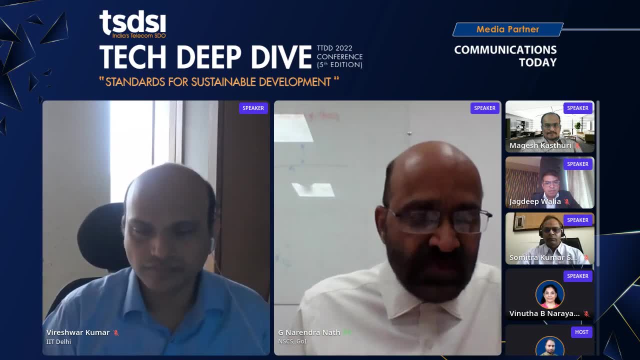 in place mechanisms for you know wherever the data is getting generated, how do we actually give it to people so that maybe, using AI tools and all, some new applications could be developed. So then you know there are security issues involved with that mechanism and all of that. Then we are also then a lot. 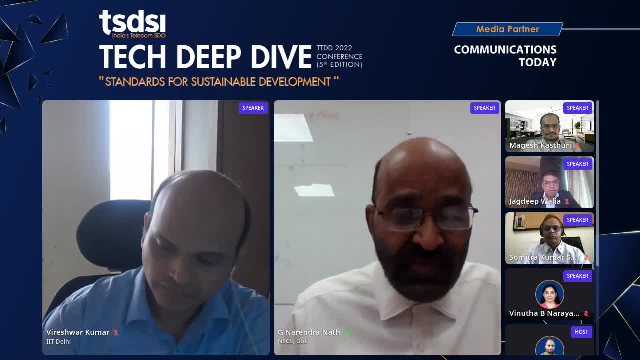 of stress now is on open radio access networks. So where we have- we are talking in terms of vendor diversity and posting vendor diversity, because there's been a consolidation that has happened traditionally in the telecom market And we have multiple players that were there in the 80s and 90s. We find that they're all consolidated into 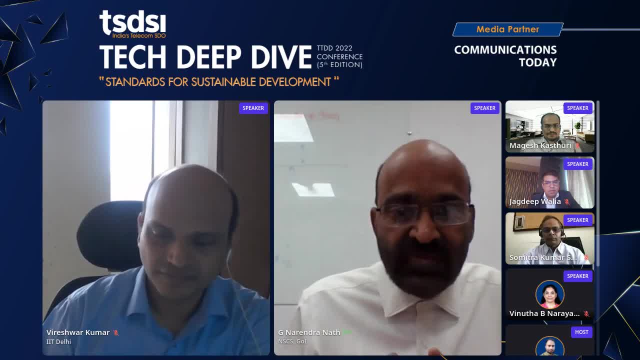 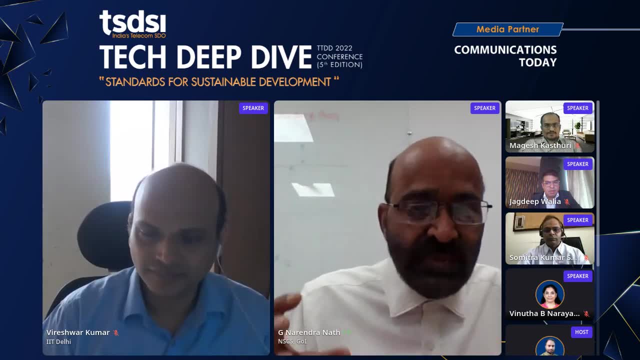 a few vendors now, And then we are thinking of now having vendor diversification again, And that's where the open radio access network comes. So when, where we are thinking of having smaller players coming with pieces of the architecture, then how do you ensure that? 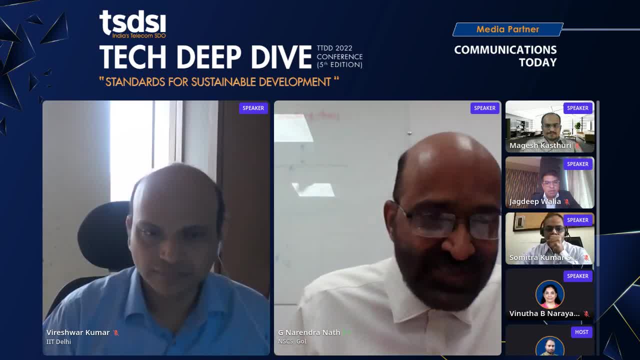 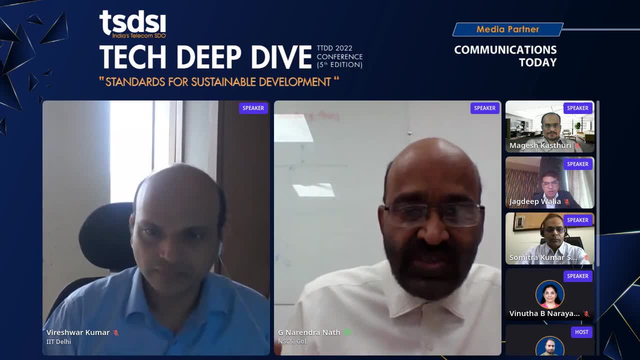 these companies which might not have robust practices within themselves. like you know, if you have a bigger company which is having robust practices, they would come up with secure products. How do you ensure the security of these pieces that are coming up and the challenge that the telecom service provider has to ensure that you know each? 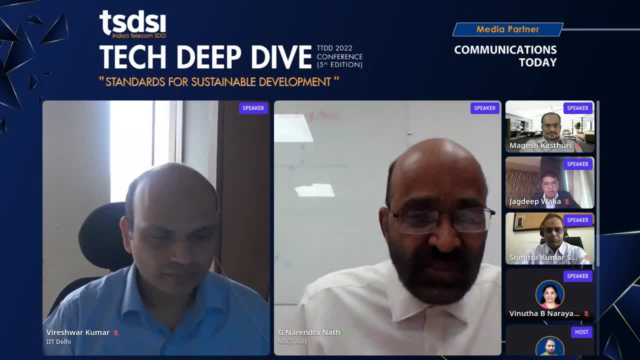 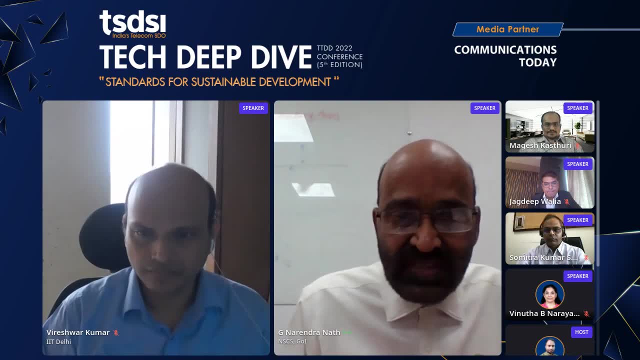 of these pieces is securely developed. How do you ensure that? So it means: what are the process that the company is following? Are there some you know standards for that, for evaluating the companies, the processes that they have and evaluating the products? 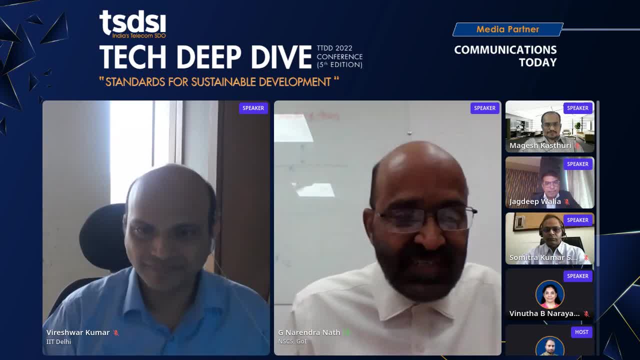 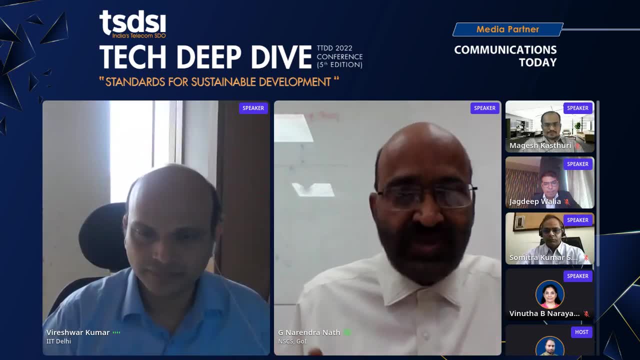 they have. So these are all multiple dimensions that are there and they're required to be addressed. Okay, So one is good is that you know, 3GPP is, you know, talking about security, and we have had some sessions. 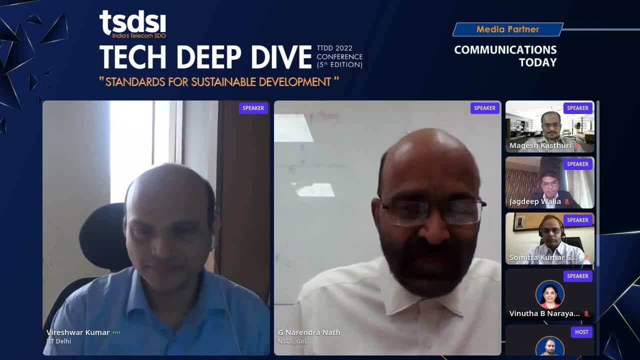 In this tech deep dive before we barged into this. I'm not, I mean, unfortunately I could not join in it earlier, but I am sure that you know those aspects were discussed, that technically you know what are these: at the, you know slicing or at the interfaces. 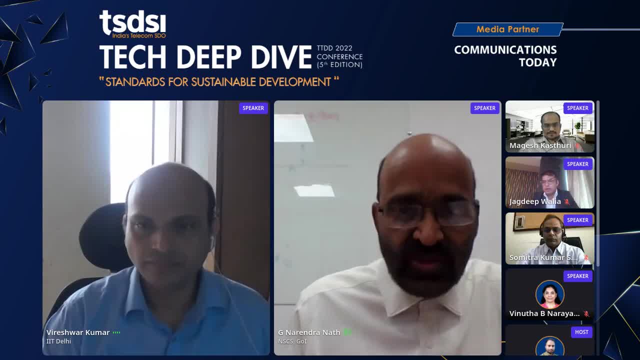 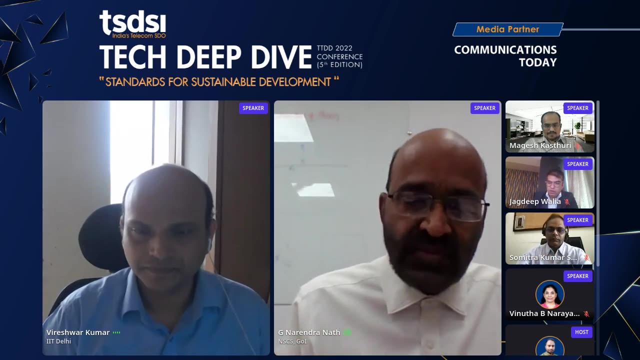 what are those thoughts that are going on to? and encryption was one thing that was being talked about last, So what technically that's going on? I just mentioned to this group and so that people are aware, I think where are we coming from. One of the things is we understood that, you know. 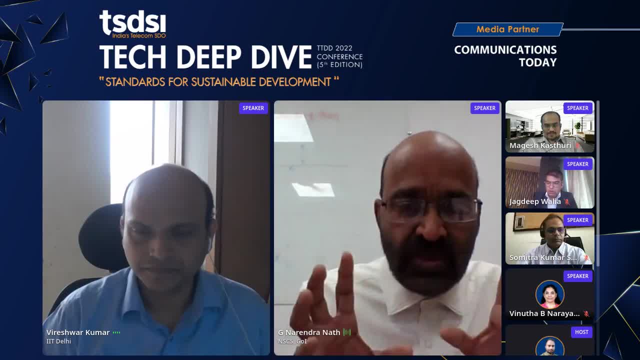 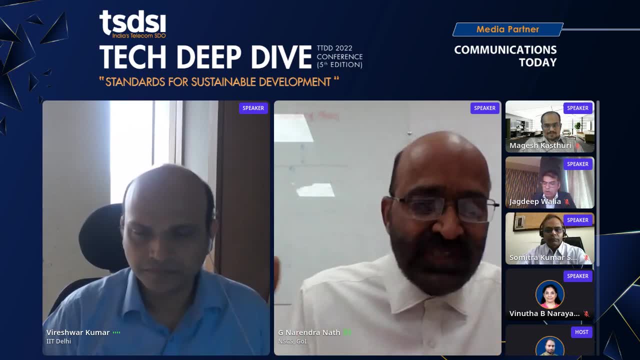 the 5G tech equipment or ecosystem has to be examined from, you know, our security requirements perspective. That's why we have been in touch with the National Center for Communication Security that's based in Bangalore. It's a unit of the Department of Telecom that they 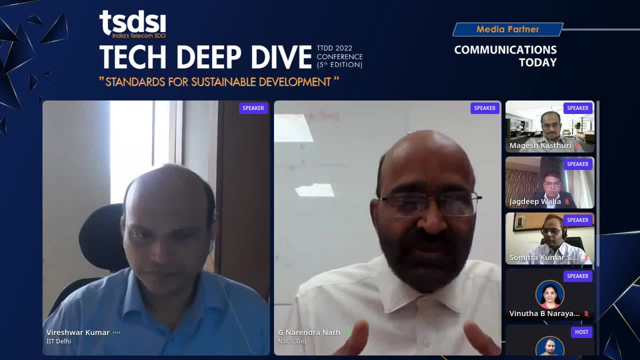 should work on this prospect, on this aspect of coming up with security requirements for 5G. i'm not when i talk network elements, not hardware software, but anything, it's a network elements. so they've been working and we have funded a project uh, along with triple iit, hyderabad, so i've been 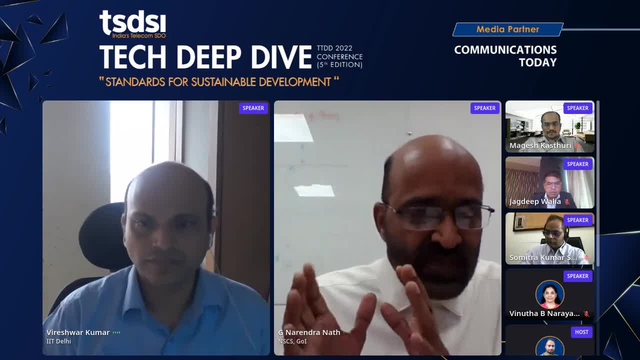 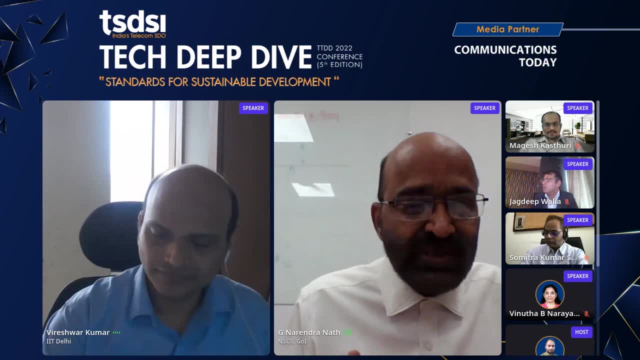 working on coming up with security requirements, 5g network elements. so that is one aspect. then we have also been, you know, actively trying to cultivate the industry and academia to come up with security requirements for iot devices also. it's very important you know that now currently. 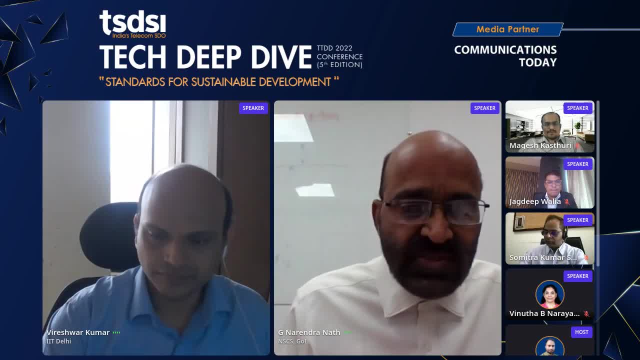 anybody can pick up a device without knowing if it's any security features. so coming with security requirements so that people know that i'm purchasing a secure iot device, so that's one, and we have funded a project. i'll not say that it's been a very success story up till now in 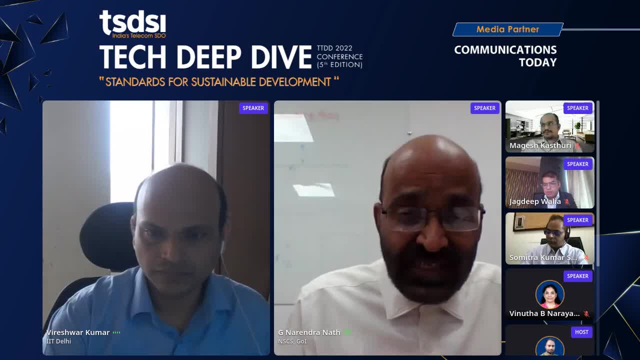 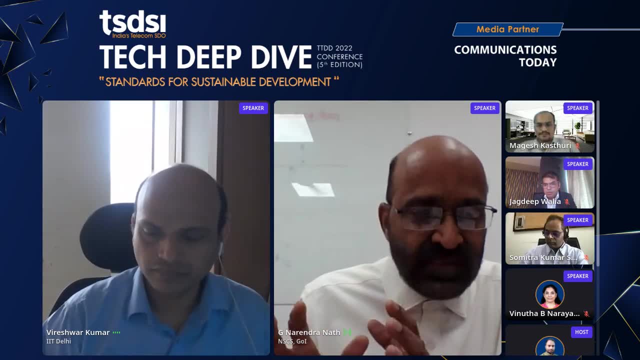 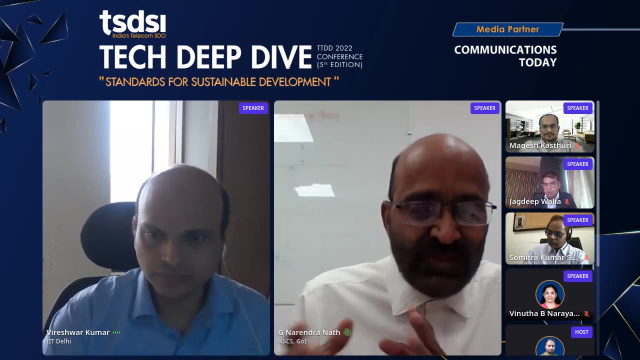 last one year we've been trying evaluating the work that's happened. but luckily, under the cyber physical systems of dst iit, bombay has been has a technology innovation hub. you know they have got they're working on the iota, so there we have been exchanging documents and we are trying to come up with some. there are rfps for 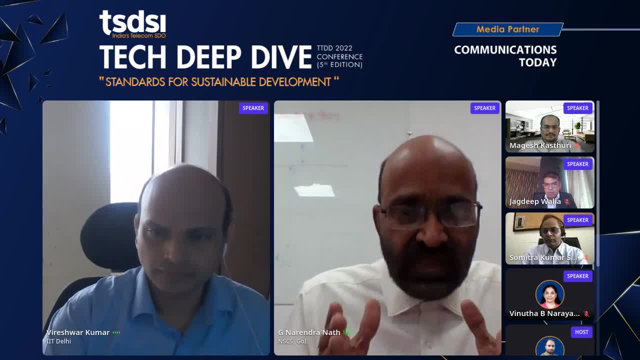 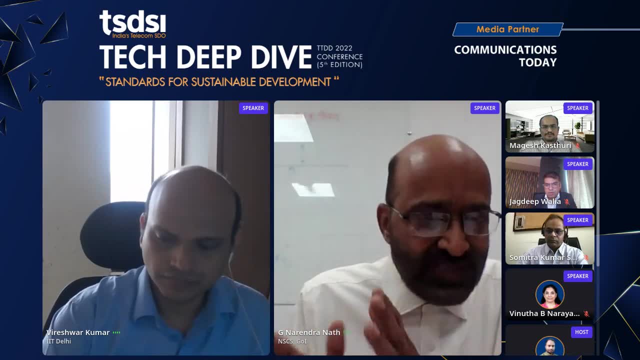 project proposals for iot security, where you know, one of the things that we're working on- security requirements for iot devices, maybe classification of devices- and that's one area that work. work is happening. the other area, and we are funding this, is the establishment of a national trust center. 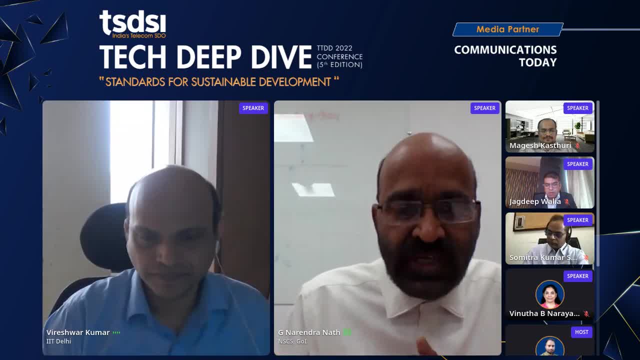 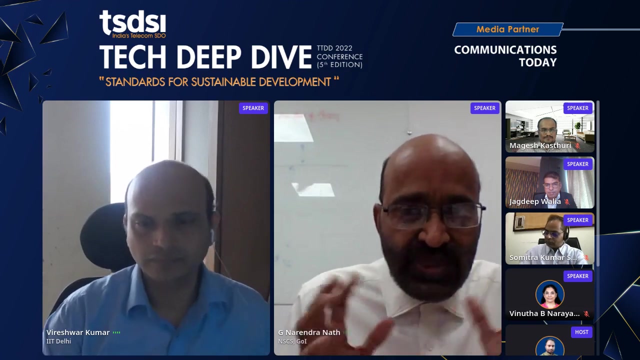 so we are funding cdot now. we have invited proposals- and cedar proposal has been approved- for coming up with establishment of a national trust center and that is especially for iot devices, registration of iot devices, certified iot devices service providers, iot service providers and vendors, device vendors. so that would be a mechanism for doing that. 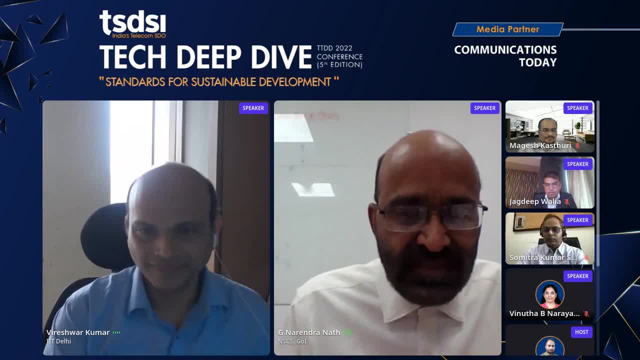 so these are some of the areas. i think when you start working in all of these areas, with active cooperation both from the academy and the industry, i think holistically, we would be able to manage to extend. you know the challenges that are coming up with all of this. you know one of the challenges. 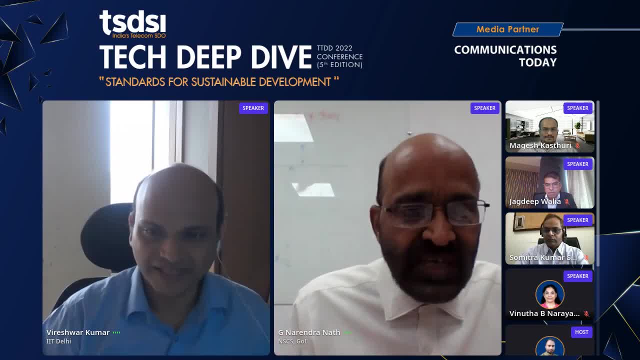 of course iot people talk of is updates and upgrades to all the devices. currently also. it's a challenge now: how does how does that happen? you know, how do you actually have a complete repository of what are the devices in place and whether all the devices have been updated or not? what is the 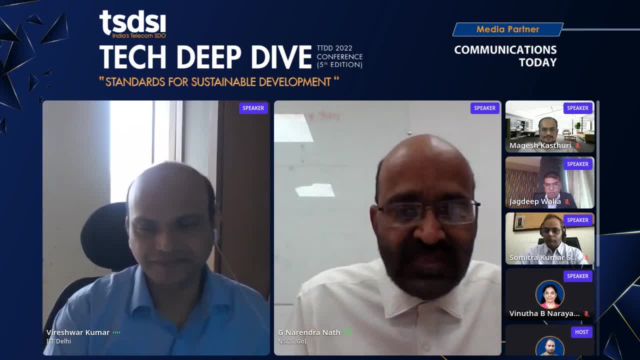 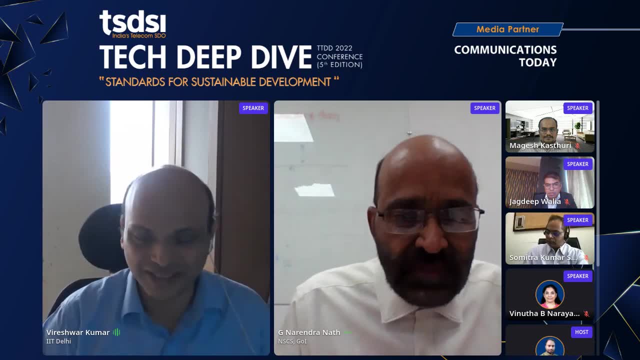 device. what are the updates that is required for that? you know, these are all challenges. i think it is a national trust center hopefully would help us in doing that. yeah, thank you very much for your remarks. so i think you highlighted the design security issues of 5g and then 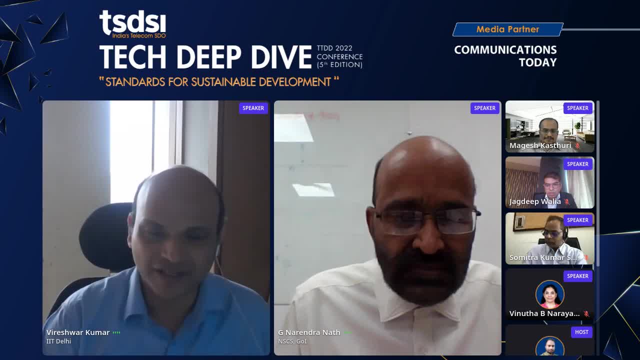 what security issues will come when you try to implement those designs in real world systems. i will come back to you about these different initiatives that government has taken to encourage the security ecosystem in india. but let me just go to mr valia and then. so mr valia, so can. 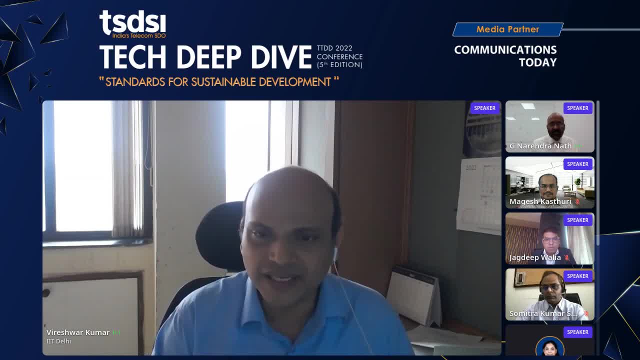 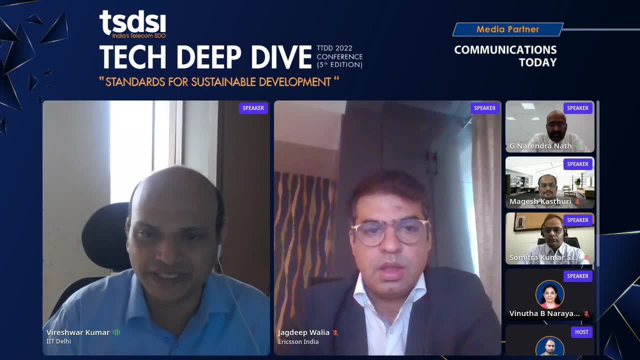 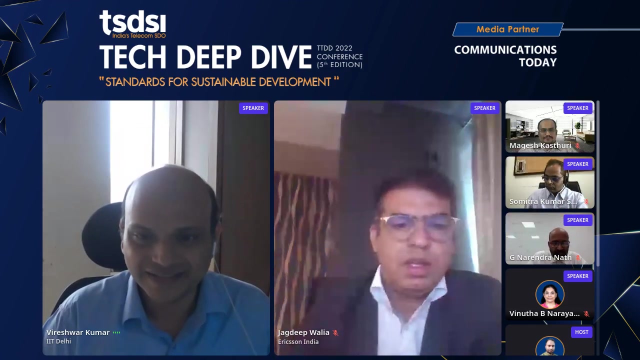 i highlight some key enhancements that have been introduced in 5g for ensuring that the 5g infrastructure is robust against the attacks that we have been discussing in this in this session. so, mr valia, please unmute yourself, can you hear me? yes, yes, please, thank you. thanks and thanks to. 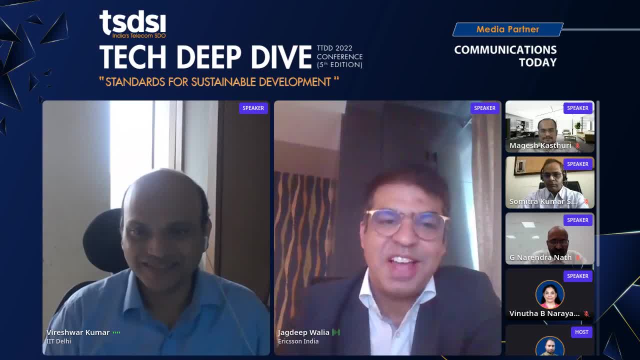 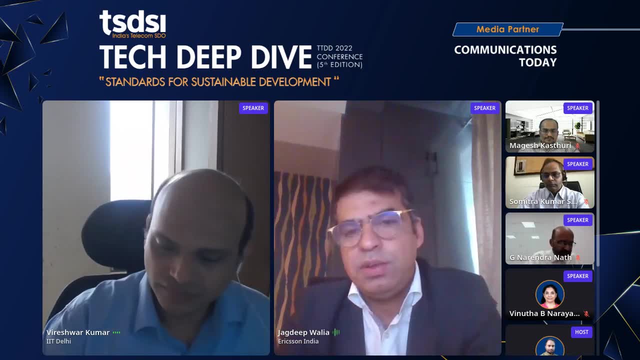 shreen, and then you know good insights into the challenges, and i think some of the key challenges that i- or i would say the challenge that he highlighted, i mean, which you were kind of referring to- was that you know to have security by design, to ensure that the 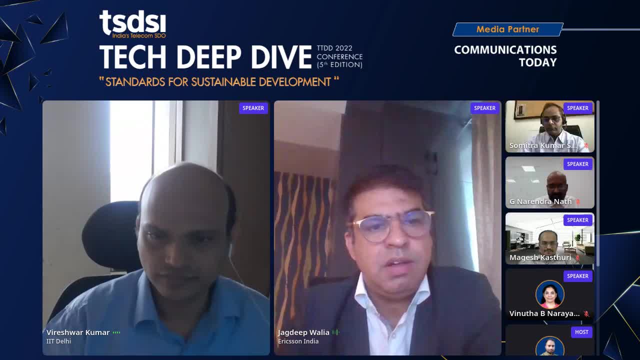 products have relevant security built in. and then, obviously, the other aspect comes in is the assurance, which is to ensure that when the operators are deploying, then they are confident that the relevant security capabilities have been implemented and they've been tested to ensure the- uh you know- proper functioning of those. 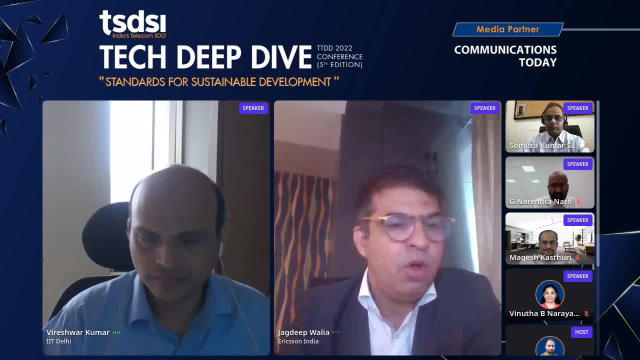 so those security controls or functions in the network and beyond that, uh, the, the, the, uh, you know 5g being used for different use cases. uh, one of them that being pointed out was, for example, from private networks. i mean, you know, and then you also have new concepts like edge coming up with with 5g. 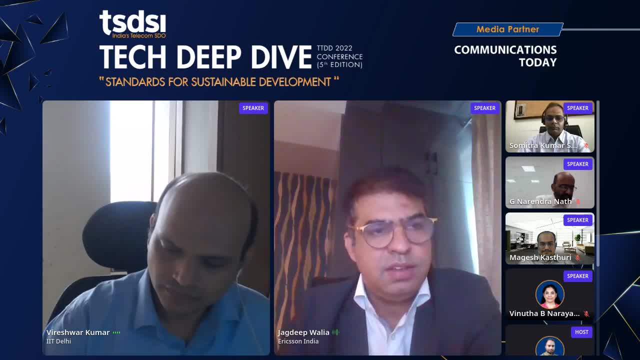 in terms of supporting, uh, let's say, ultra low latency use cases. so i would say the good thing 5g has been that that this generation, or you know, 3dp, started. when it started, standardization security was always a focus right from the start. so you can say that security by design has been. 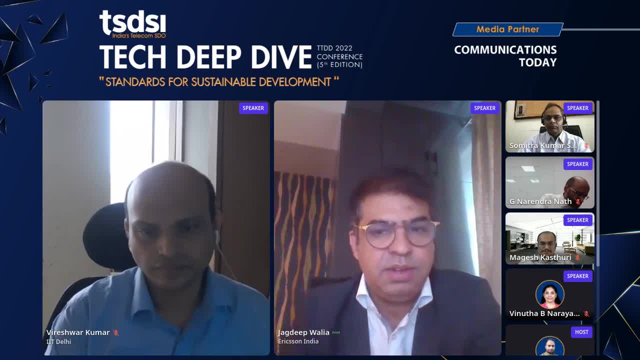 built into when it comes to, at least from a standardization perspective, when it comes to 5g. having said that, i would say that 5g, the, the, the. from a security perspective. it is basically using most of the 4g security and then it goes beyond and has several enhancements that are there. 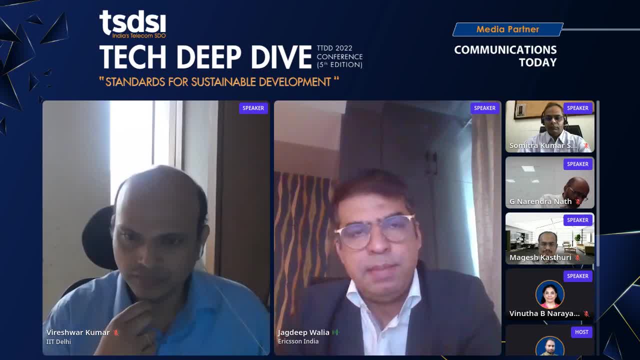 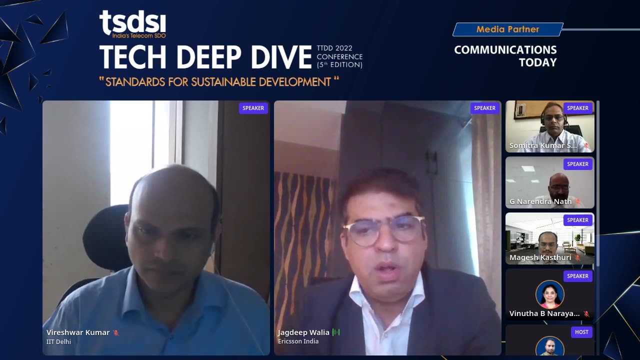 to address gaps in the previous generations. for example, we had issues with the, the mz being sent unencrypted over the radio interface. we had issues around the, the user plane integrity not being supported. we had issues of false base stations getting attached into the network and then there. 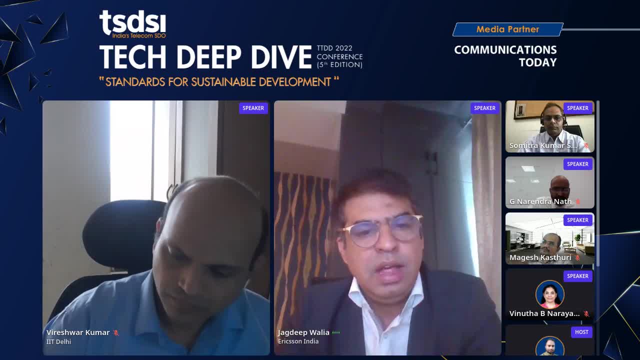 were also these legacy protocols like ss7 and and diameter when abilities that existed, so so these have been factored in by by 3dpp when they started to standardize 5g security. and also wanted to mention is that when they started to standard, they realized that 5g is. 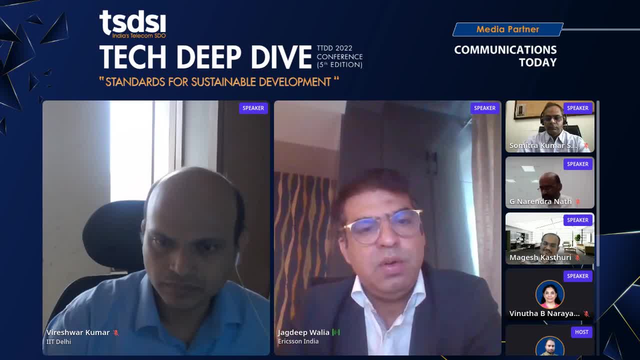 going to be used for multiple use cases which would have their own specific requirements. so how they addressed is that they divided uh, basically the standardization in phase one and phase two, where in phase one, which is referred to as r15, is where they define basic baseline security uh requirements. uh, mostly from examples like enhanced mobile broadband use case. 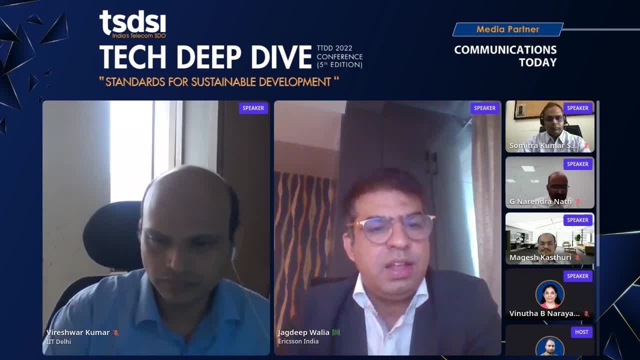 and then they also defined the security requirements for uh different other use cases. beyond that, in r16 and r17 they are defining uh security requirements for uh different other use cases. one of those as was private network, which is called as non-public networks, which has been 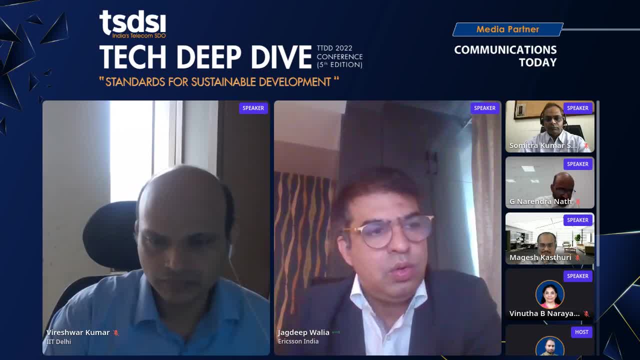 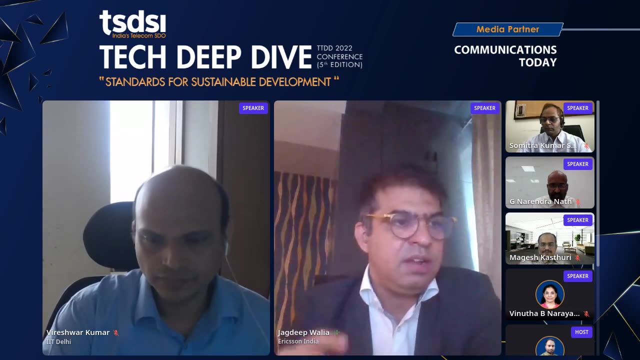 defined uh by 3gbp in r16 and then going forward in r17, and then also you have other use cases, for example, uh, uh, vehicular security i mean, or, or v2x kind of security that is being defined also uh in just to kind of give a- you know, a basic understanding that that's how the security 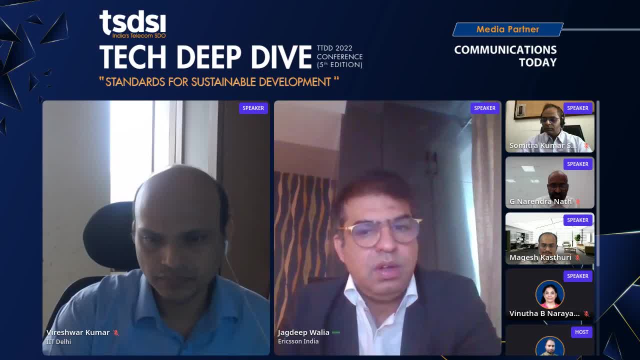 work has been uh taken up when it comes to 5g security. now, if we specifically look into the kind of enhancements that uh 5g has done, uh and and uh- here are some of those. i mean there are quite a few, i mean, so i'm just going to list out a few few of them. uh, and if we look from 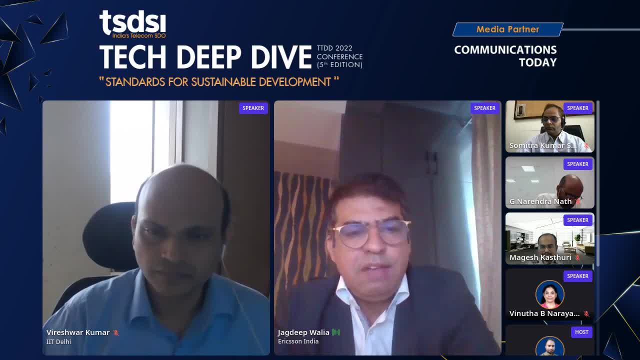 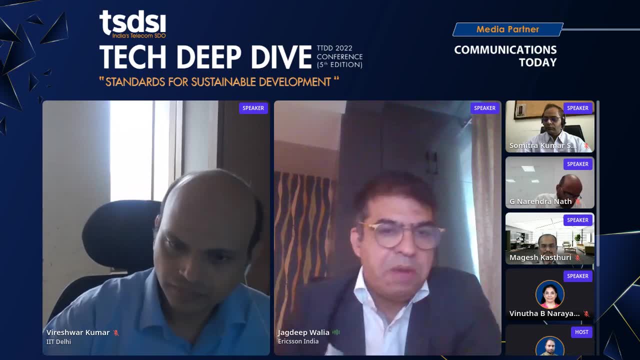 a subscriber authentication perspective. uh, you know, we have now uh authentication which is uh terminated in the home network uh, compared to previously where it was done in the visited network, wherein uh you know you could that that itself led to certain uh security uh gaps. uh. the other enhancement has been- since we see that 5g will be used for a lot of uh iot devices getting 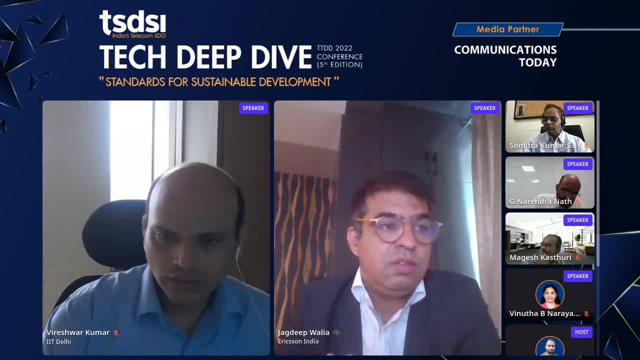 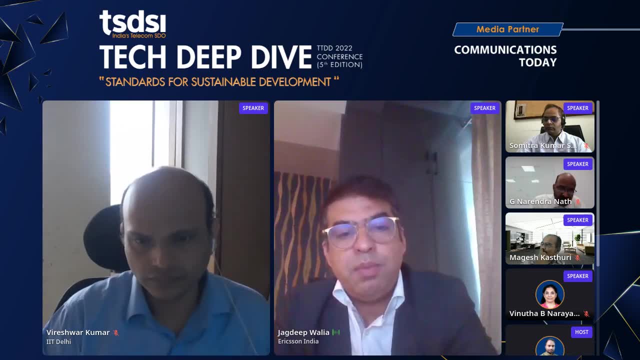 connected and id devices. if you look at some of the devices, the form factor is so small that you could not have sim cards being used. so that's where- uh, you know, we have support for non-sim card based authentication, which is useful for iot devices. 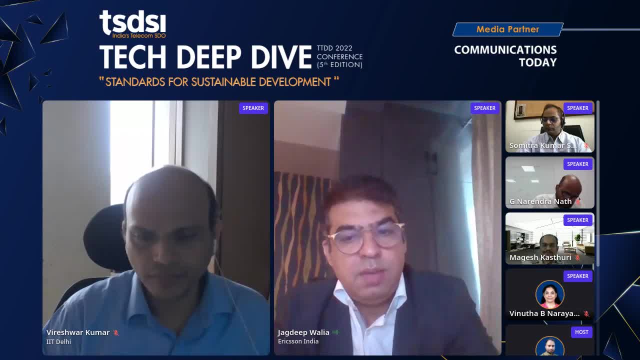 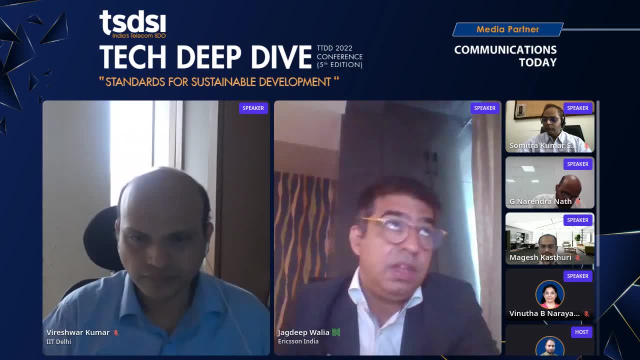 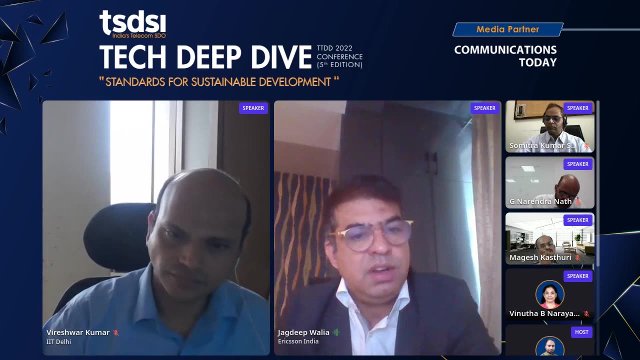 that has been introduced. the other area is subscriber privacy. that has been enhanced through introduction of mechanisms, uh for implementing, uh for encrypting imsi, uh and and and imsi is no longer uh used for paging, which again was leading to, in previous generation, uh to to certain uh, uh security, uh gaps which could be exploited. uh, then we'll. 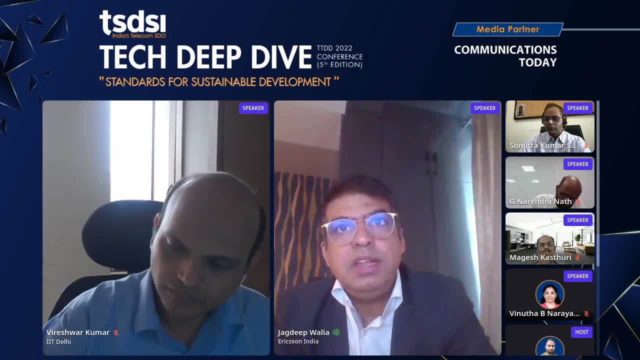 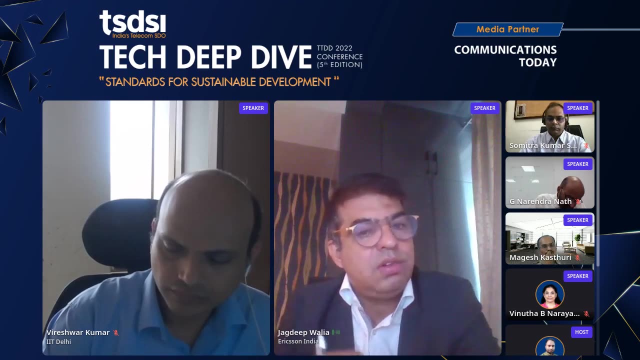 have, uh, you know from, from uh- vulnerabilities in the core which was related to, let's say, the legacy protocols like c7 and and and diameter. we now have a service-based architecture where we are using uh https, now and and and then. here also, we have a zero trust. uh, uh, that has been. 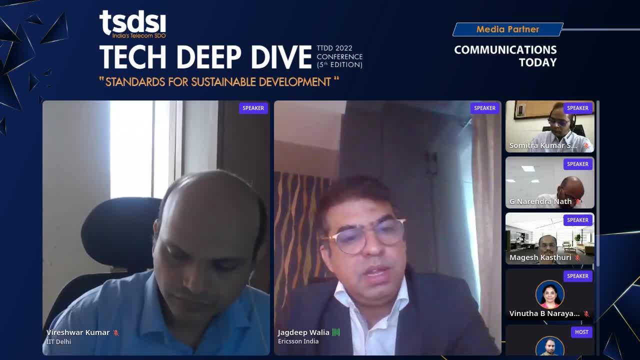 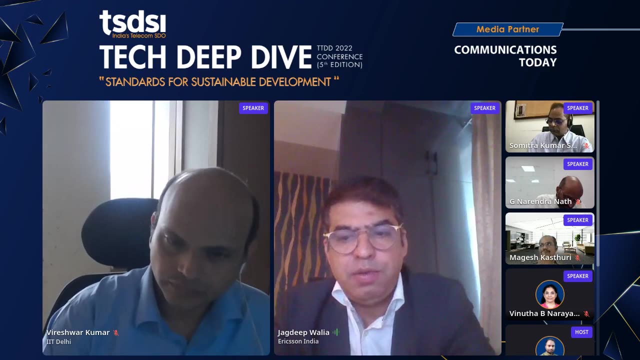 introduced wherein, you know, each network function, when communicating with other, has to authenticate and authorize so so we have concept like zero trust being already uh standby from a 5G core perspective. The other is from a perspective of roaming. We have roaming security. The whole concept of trust has changed. 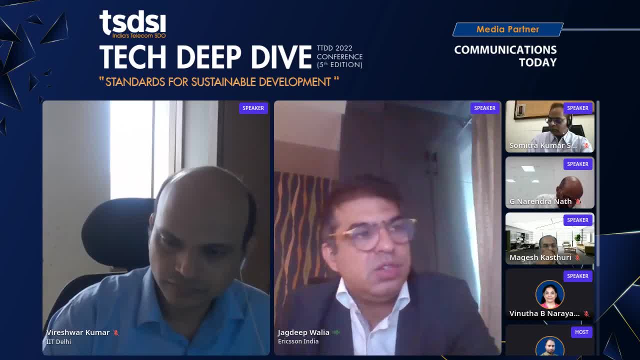 when it comes to 5G network In 4G or previous generations, we assumed that my roaming partner or interconnecting partner is trusted, but that is no longer the case, because- I mean specifically from a roaming perspective- there have been a lot of, let's say, 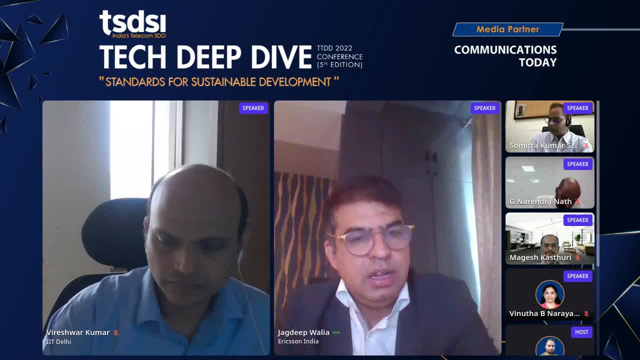 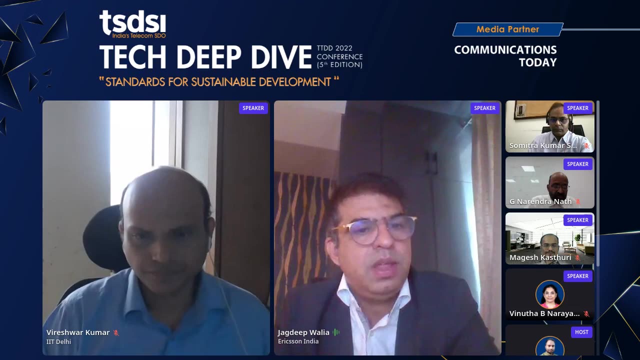 attacks that have been launched from the interconnected roaming partner networks. And that is where, in 5G now, we have roaming security that has been introduced, wherein you have an actual authentication or security that has been introduced both on the control plane and the user plane. 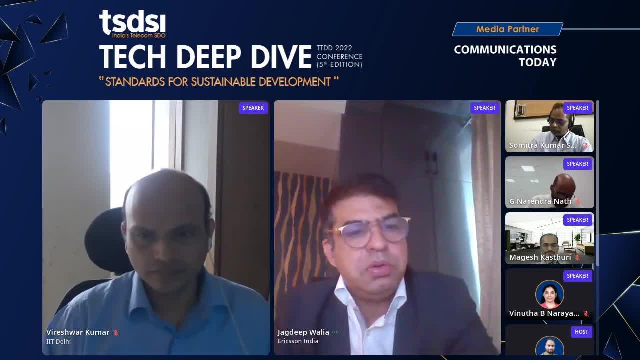 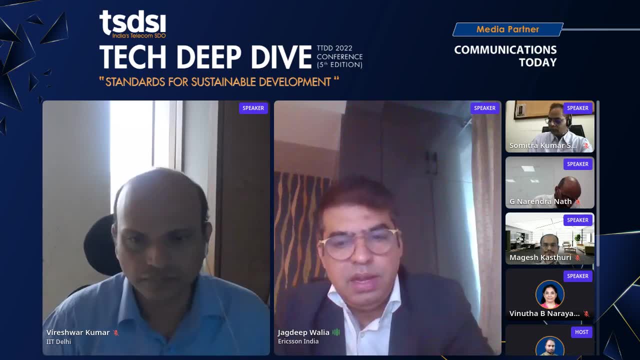 to ensure that you could kind of filter out any malicious traffic on the control plane or any attacks that are coming from the user plane. So that is from a roaming security perspective. Further, we have also integrated protection that has been introduced over the air interface. 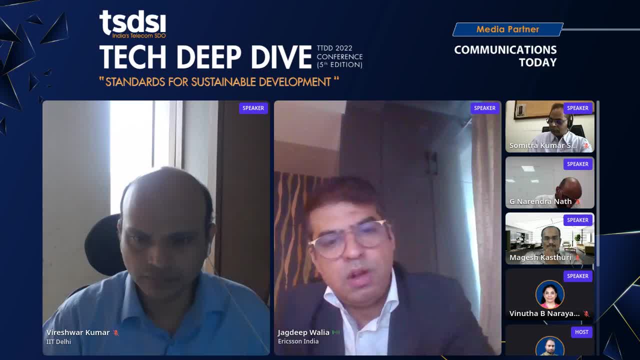 again, which is mandatory for the vendors, like us from Ericsson or whatever I mean to implement, but then it is optional for the operators. And lastly, you know, even the key hierarchy is longer informed, So you know, in 5G than in 4G. 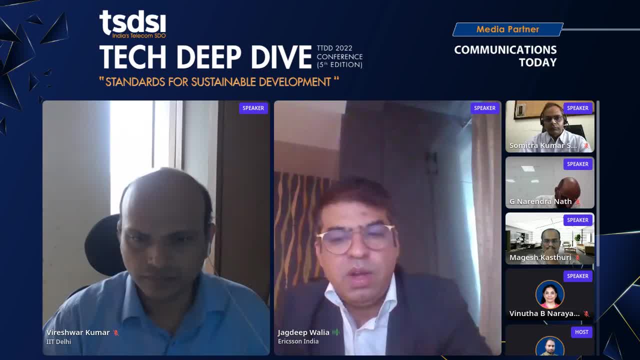 because, you know, in 5G we have introduction of two more intermediary keys which provide better separation and then security. Further, in the last I would say we also have four space station detection in 5G. that is supported. 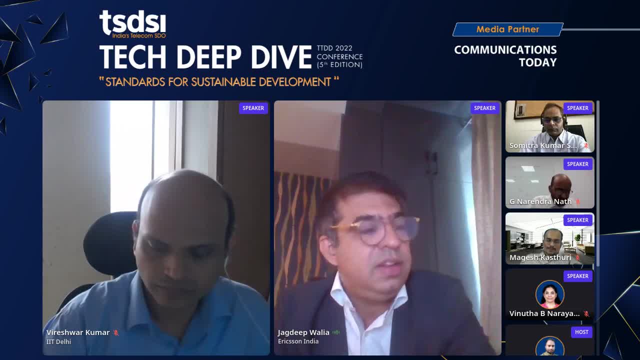 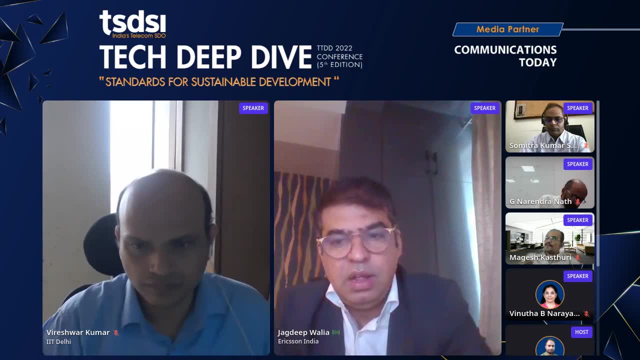 which was something that has been increasingly being seen in the networks around the world. So now, with 5G, you have a possibility to detect, of course, base stations or fake base stations that are connected. So therefore, I mean I would say that you know. 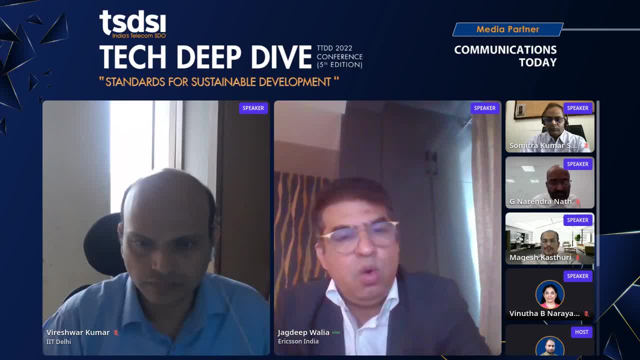 it's safe to say that 5G is the most secure G among all the mobile generations that we have seen so far, And the expectation is that, at least from a standards and implementation perspective, it is ensured that you have these capabilities implemented by design. 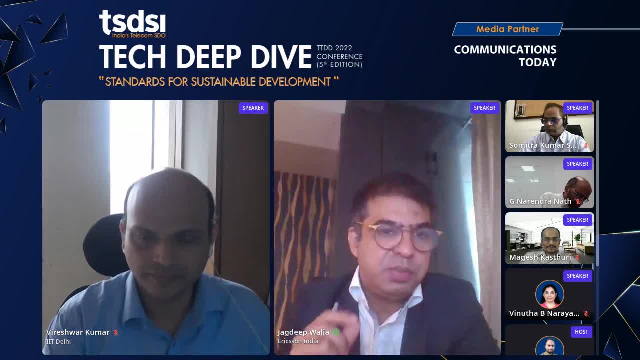 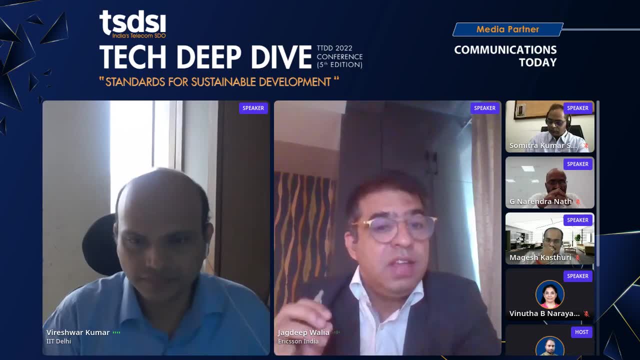 And that is one aspect which is in terms of, you know, look from a standards and perspective, I think, in case we need to ensure the security of 5G networks- for that matter, any networks I mean, you know. 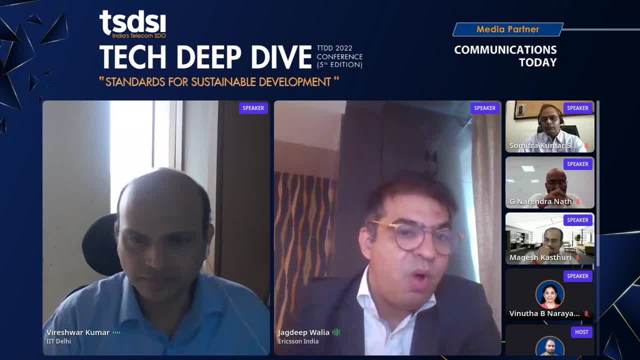 you have to go beyond just the standards and implementation. I think most important aspects are in terms of how these are implemented and how the networks are managed, monitored. I think that is another area which is beyond, I would say, 3GPP. 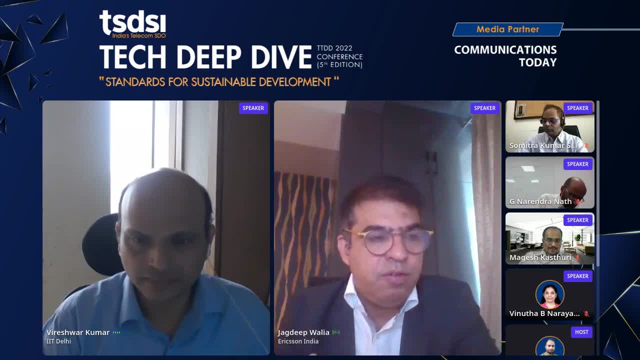 But then you know, then it comes in from a perspective of that. you know you need to be aware of what's ongoing in your network And that is where you need to have a strong security management policies and tools that needs to be implemented. 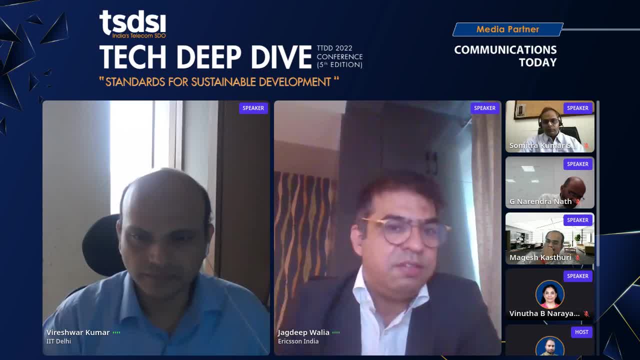 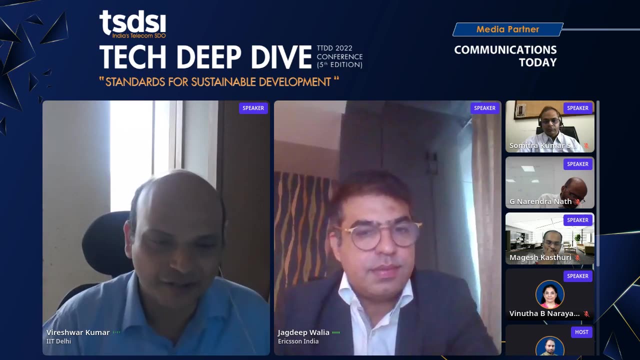 to ensure you know, end-to-end holistic 5G security. Yeah, Thank you, Mr Valia, for highlighting the key enhancements and pointing towards the security aspects that have been brought in 5G, especially related to the fake basis stations. 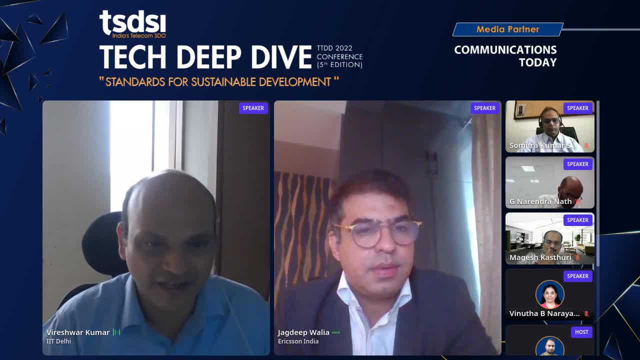 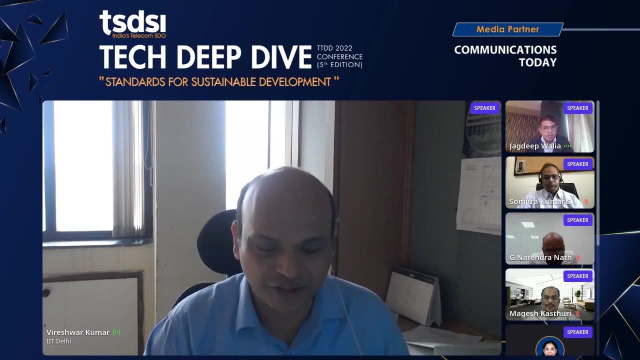 and NC encryption. These have been very closely followed in the academic community as well, So very thank you to you. So, now that we understand that 5G has put security at the forefront, now let's look into what the quantum will be like. 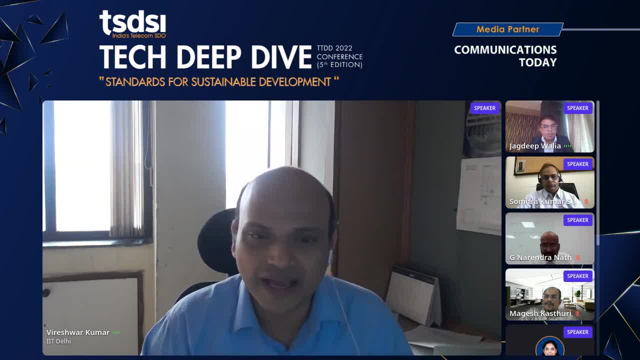 What quantum computers will bring into the picture. And there I would like to go to Professor Sanathya And I will ask him that we know that the quantum computers will open a Pandora box And Mr Manikarnikand. 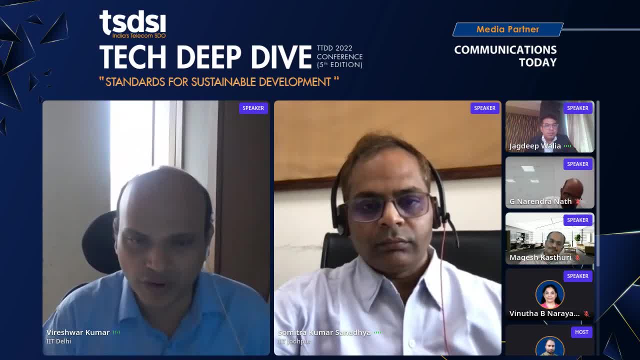 he talked about some aspects of quantum impact of quantum on 5G security, But can you also highlight the level of maturity of post-quantum cryptographic primitives and whether they are ready to be utilized in 5G networks in particular? Yeah, 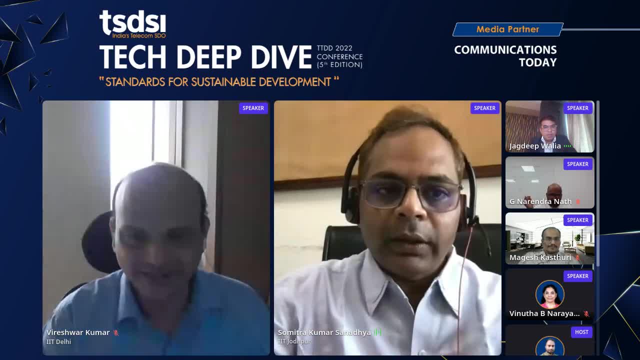 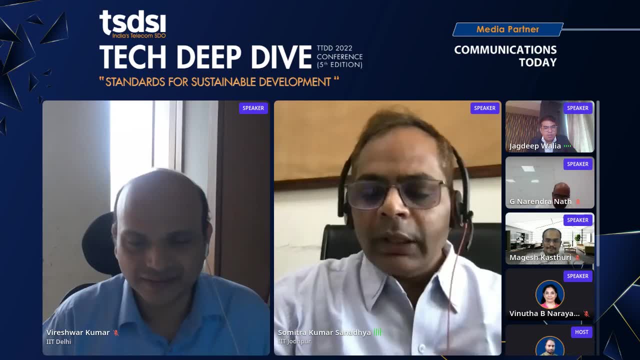 So thanks, Dr Riteshwar and TSDSI for this wonderful session of which I am privileged to be a part of. So, as Dr Manikarnikand was already mentioning, we know from the 90s. 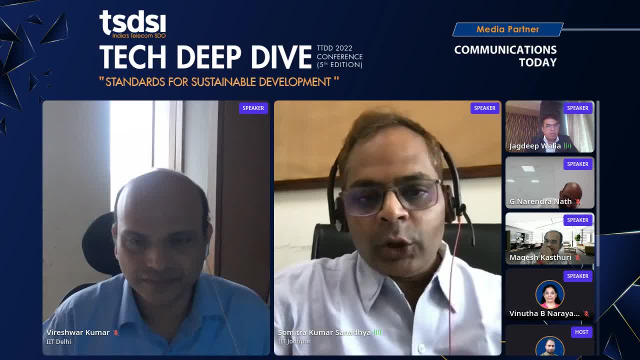 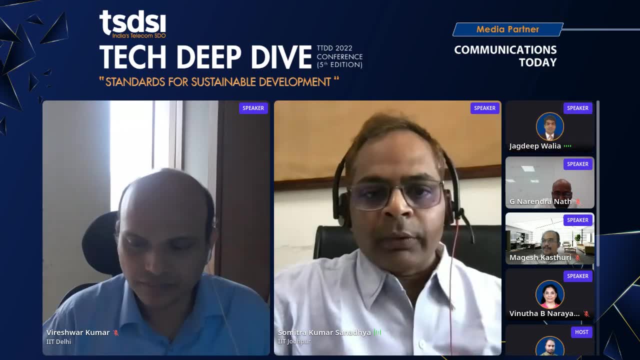 I mean to be precise 94 and 96, when Shor and Grover gave their algorithms. So Shor essentially told us that discrete log problem, on which we have a lot of current cryptographic algorithms based, will be broken in polynomial time. 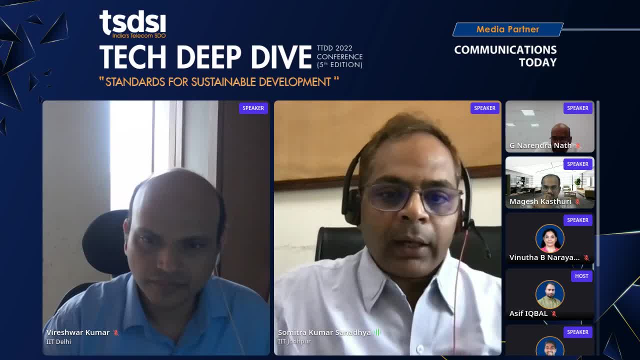 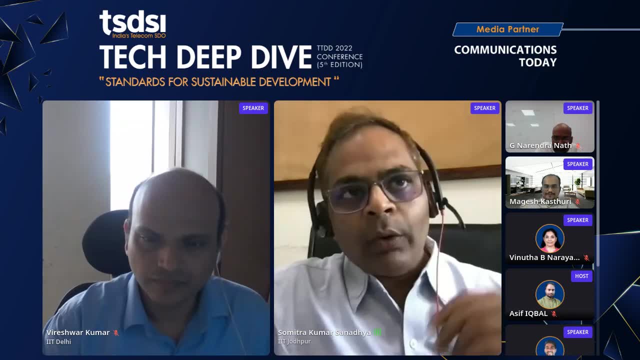 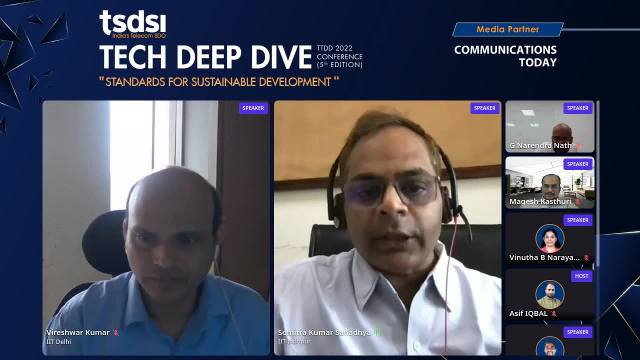 However, this is still in a sense theoretical attack, because we need a certain size of quantum computer to actually use that. Similarly, Grover talked about an attack which will essentially allow searching for an item in a much faster way than what we can imagine. 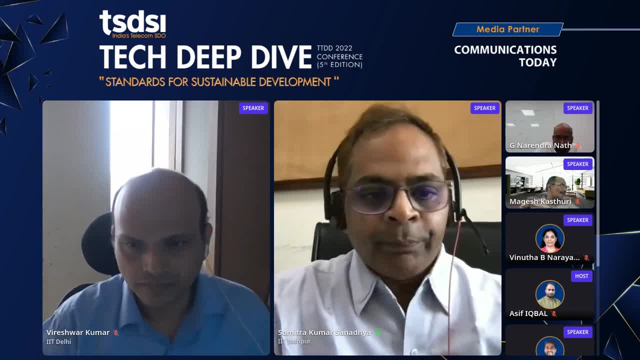 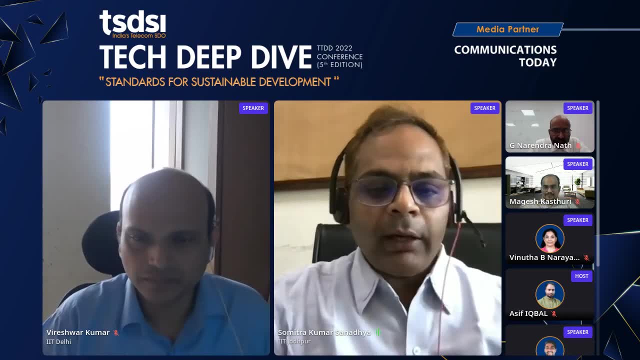 So think about a situation that I have where I have n things lying on ground and I want to find out a specific one with satisfying certain property. So maybe the best way is I keep looking one by one and I'll find it in essentially n trials. 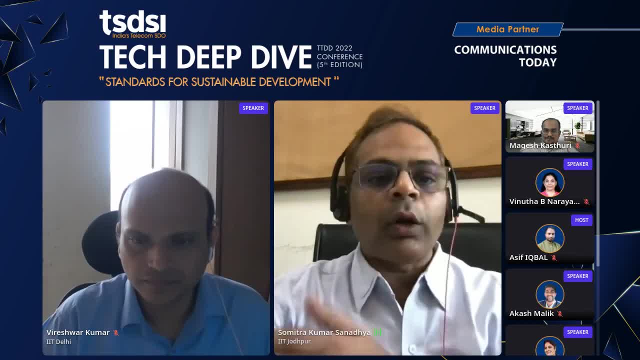 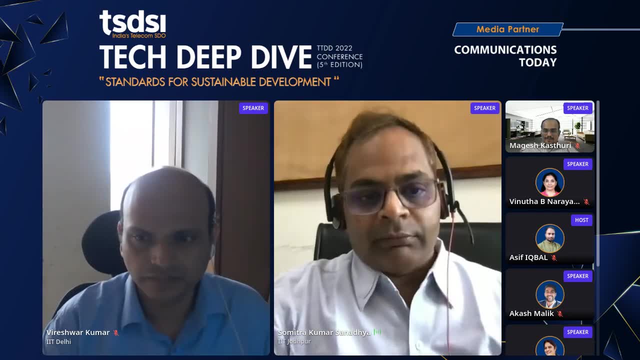 If there are n things, I'll need to search all of them. in the worst case, However, what Grover said is that this can be improved to something like square root n in quantum computers, with quantum computers And the implication of this attack. 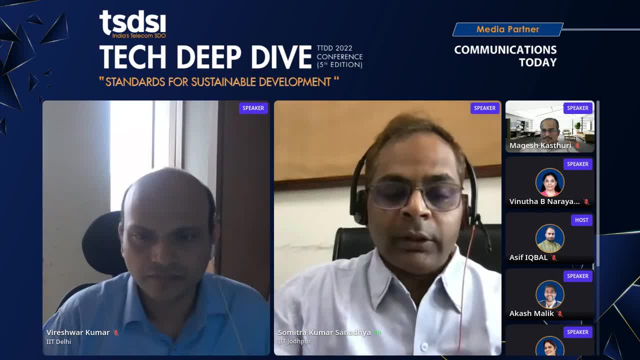 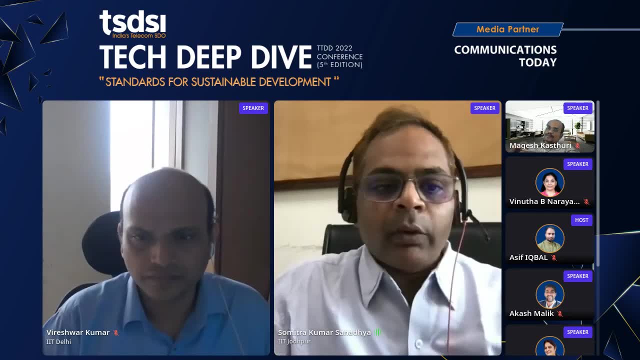 is that on symmetric key cryptographers it is possible to find n things lying on ground in symmetric key cryptography. when I use a 128-bit secret key, it will effectively become only 64-bit on quantum computers. So these are the two things that trouble us. 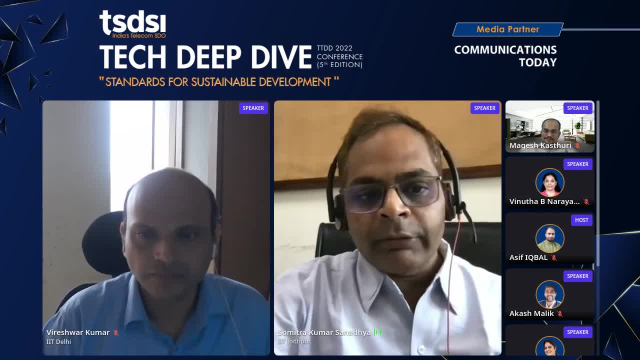 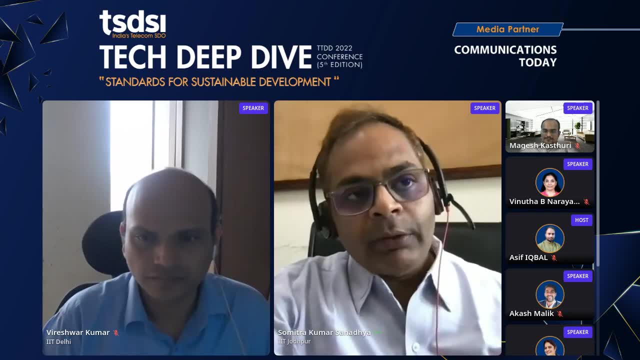 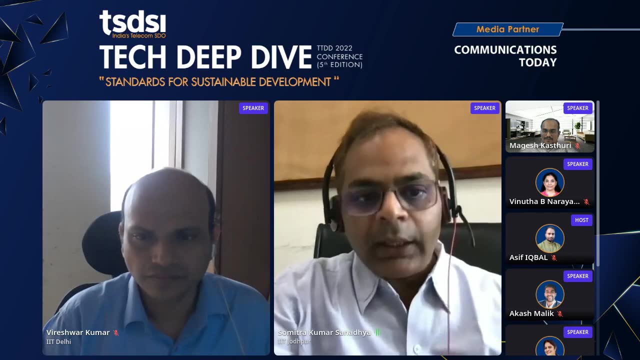 in cryptography: The Grover's attack, which will reduce the level of symmetric key security, and Shor, which will break discrete locks, and factorization, Which essentially means any cryptography which is being used currently will be gone. So the question now is: 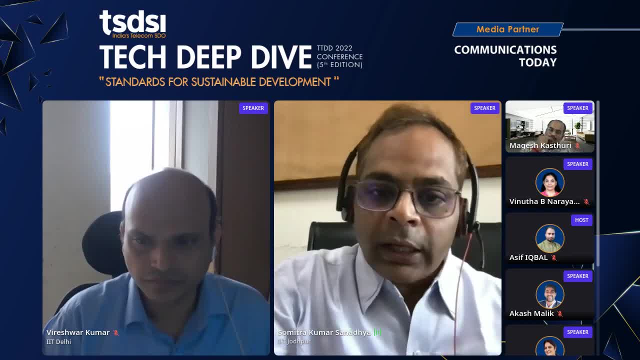 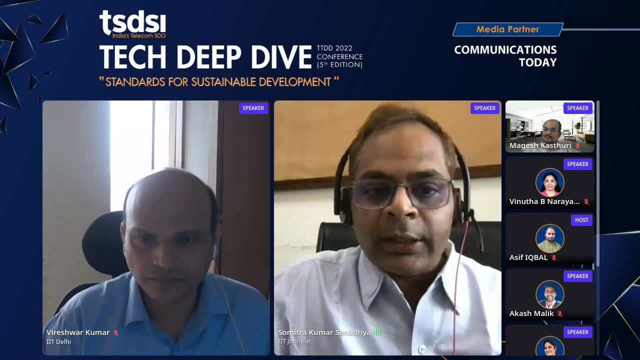 are we at a stage when we are already going to see a real-life break of these public key algorithms? So, fortunately for us, it does not seem that we have reached that stage yet. So if you look at the history of last few years, 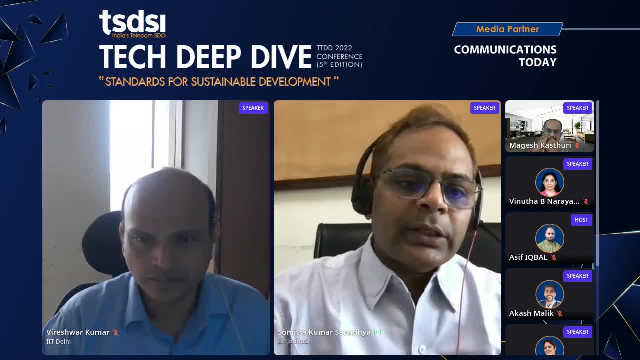 I mean Intel, IBM, Google, these big organizations have introduced quantum computers having something like, say, 49 qubits to say about 80 qubits, But we haven't even crossed say 100 or 150 qubits till today. 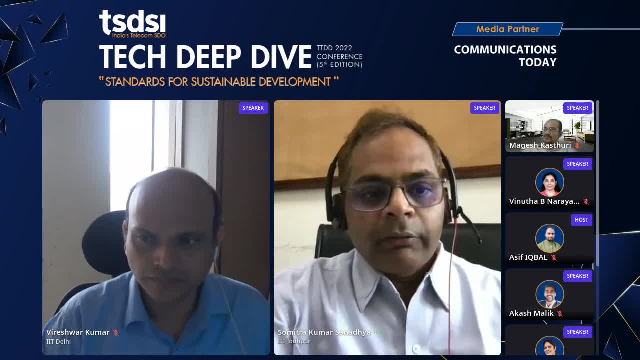 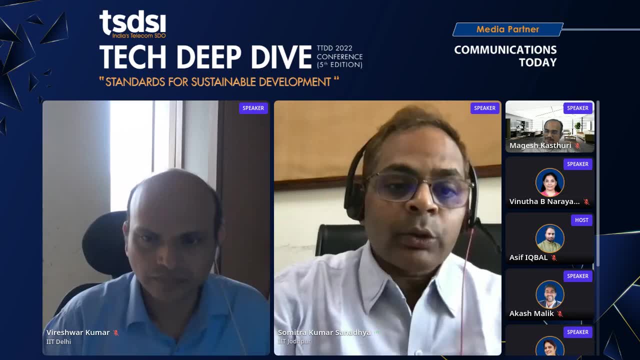 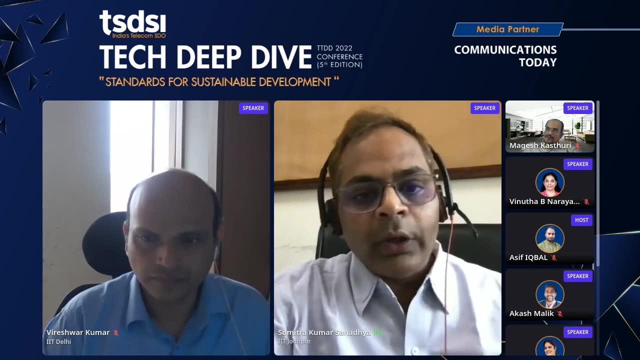 So, unless we cross a large barrier, we are not really threatening the security of public key cryptography, or even symmetric key cryptography is being used today, So fortunately, we are safe from that point of view. However, the way the research is going on, 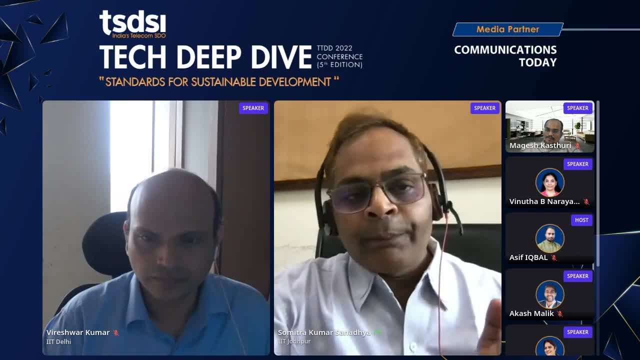 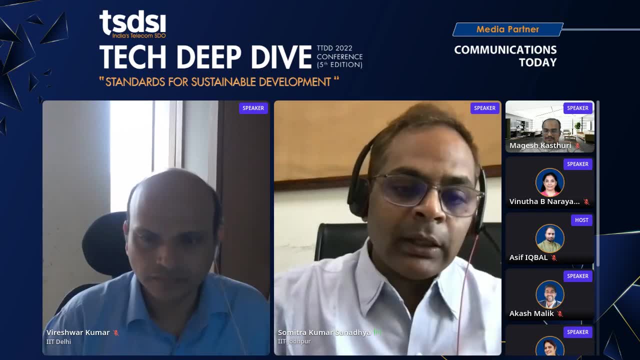 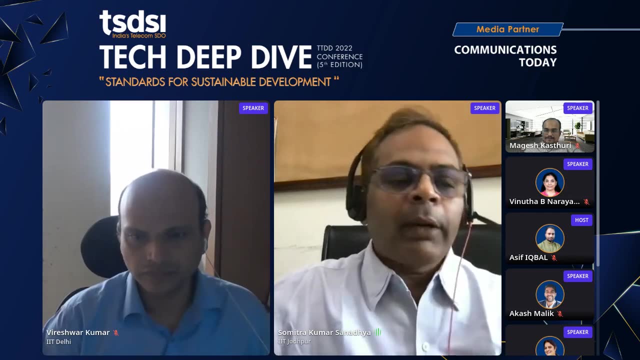 and the physicists are predicting that by 2023 or maybe 2030, we will have large-scale quantum computers And once they are in deployment, the cryptography which is being used will be broken. In fact, I would like to quote a comment. 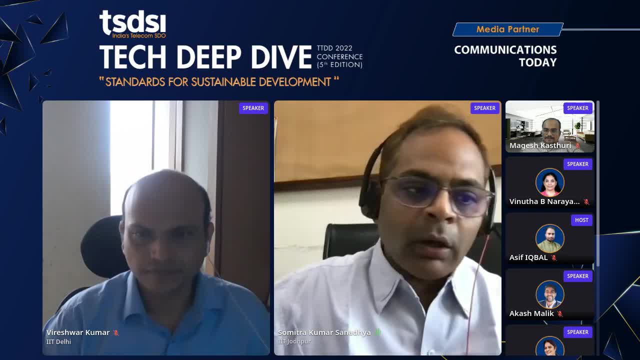 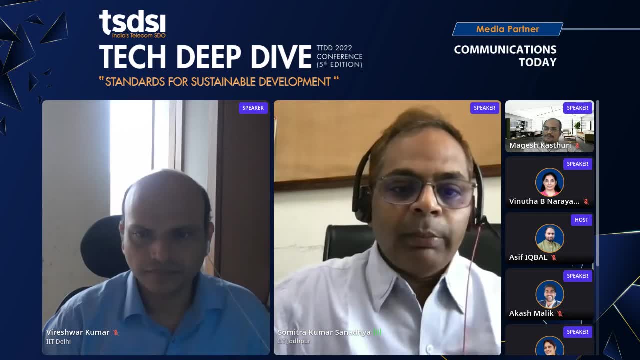 by Dr Michel Mosca, who mentioned in a famous talk that there is a 1 in 7 chance that one of the fundamental public key cryptography algorithms will be broken by 2026.. And there is a 1 in 2 chance- 50% chance. 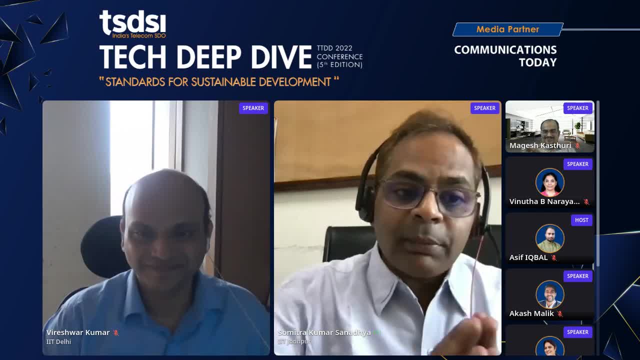 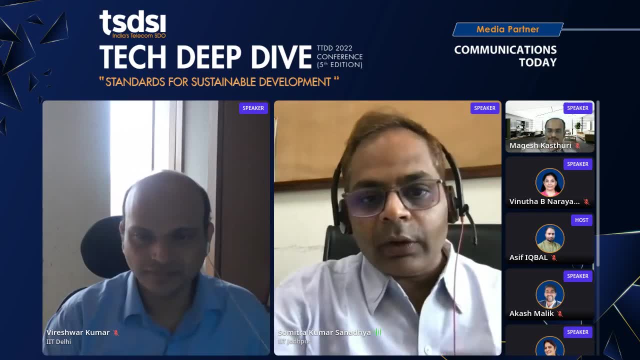 that one of these algorithms will be broken by 2031.. So this is the prediction we are looking at. In just next 10 years, we expect, with a more than 50% probability, that one of these algorithms, which is being deployed right now, 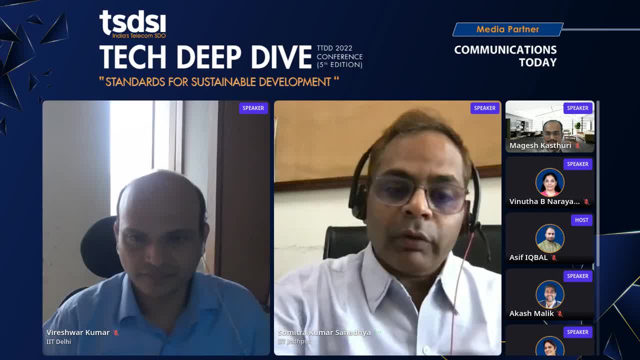 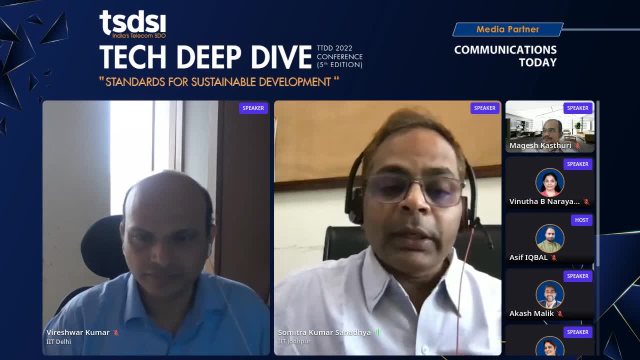 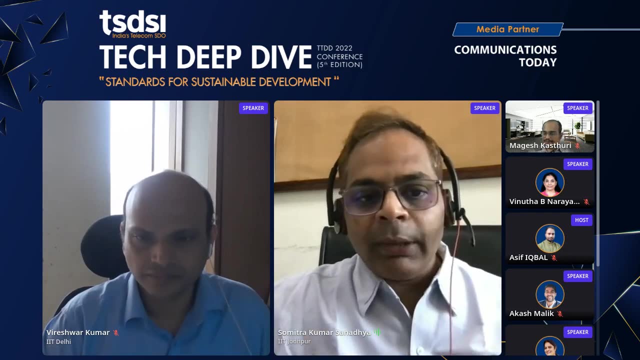 will be broken And think about algorithms or data which we want to keep secure for a longer time. So I still remember from my college days. India was participating in this comprehensive test-ban treaty negotiations, CTBT negotiations, Similar such treaties in which the government 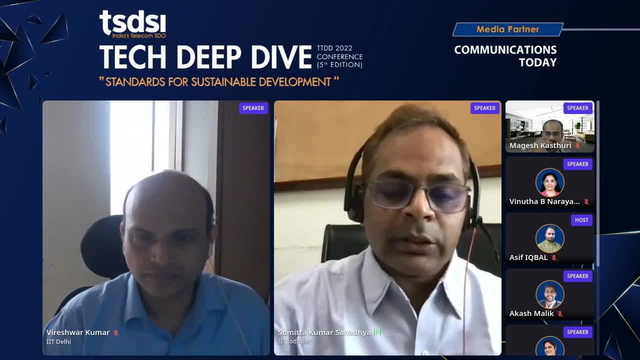 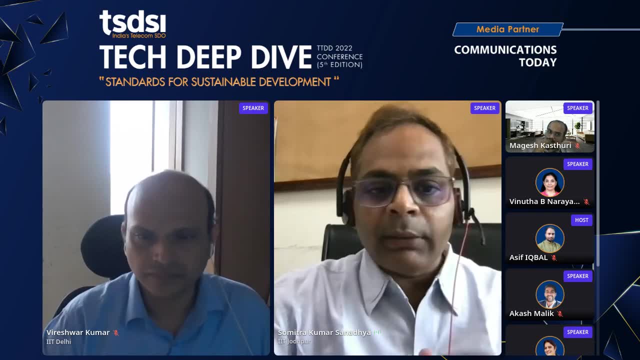 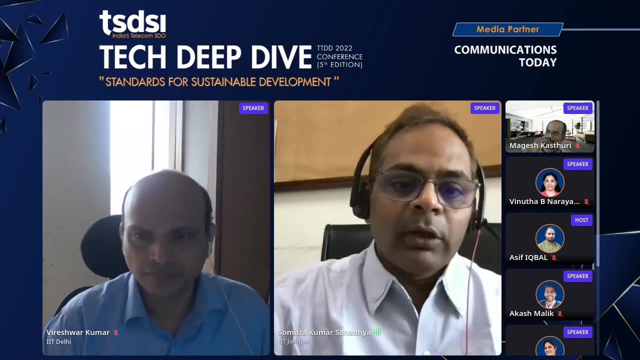 is making a certain policy decision. there are discussions happening between various organs of the government, and government would not like to reveal these secret discussions among other governments or within the government to public parties for maybe next 30 years, And that's why we have official secret acts and 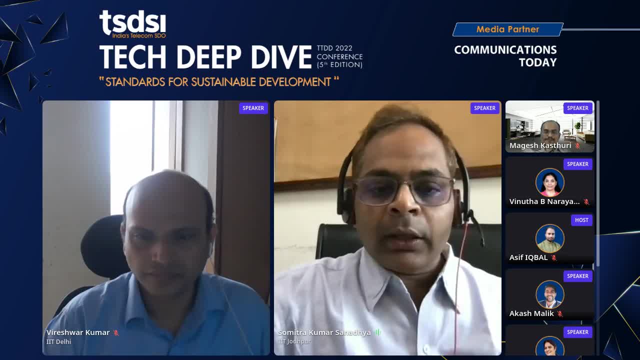 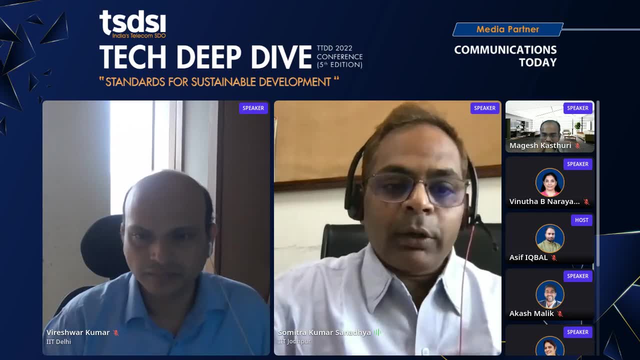 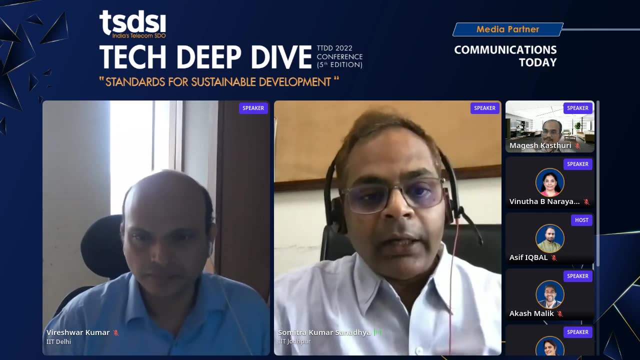 rules like that. So suppose we are expecting communication to be kept secure for, let's say, next 30 years And we are using the classical cryptography which is being deployed right now. It may be broken in next 10 years, So this is the time when we are already. 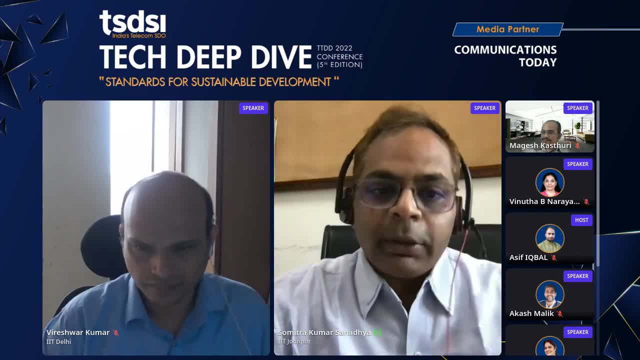 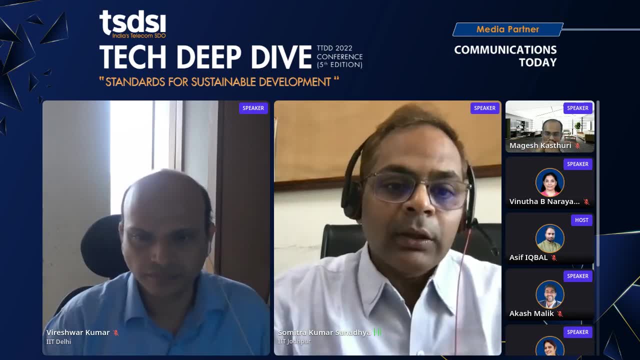 worried about- not right now, but in the coming few years- what is going to happen. So, although we have not been able to build quantum computers of that large size, which will practically threaten the security, they are already a threat for near future. And that's where comes the picture of 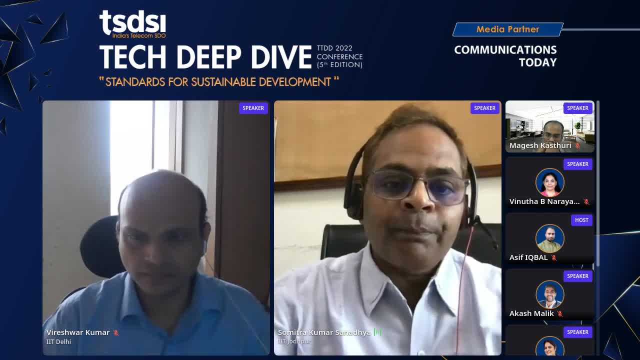 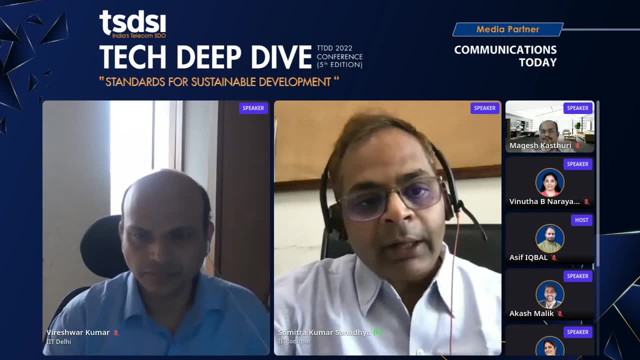 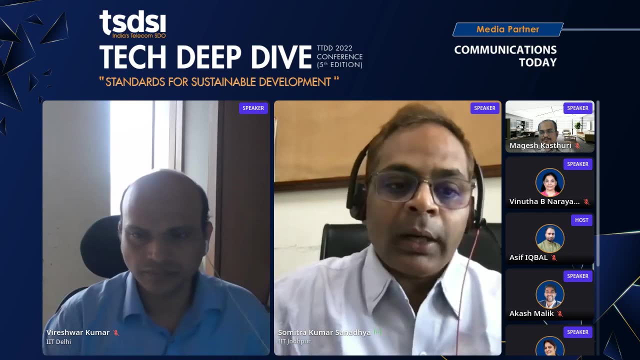 can we do something about it? I was already mentioning about the NIST algorithm development program for post quantum cryptography. Now, fortunately, mathematicians have identified a class of problems which will not be solvable very quickly, or, to be precise, in polynomial time, even when quantum computers come. 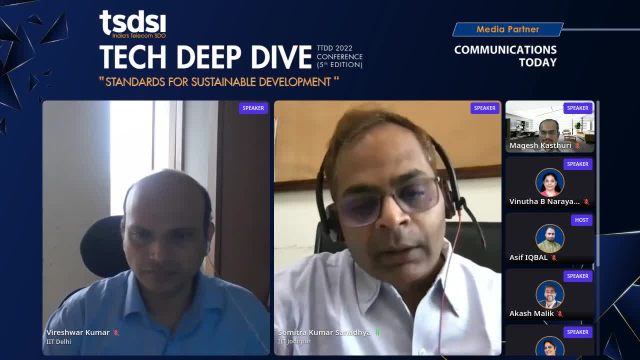 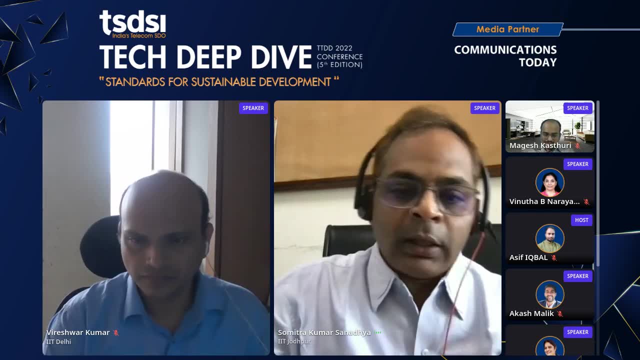 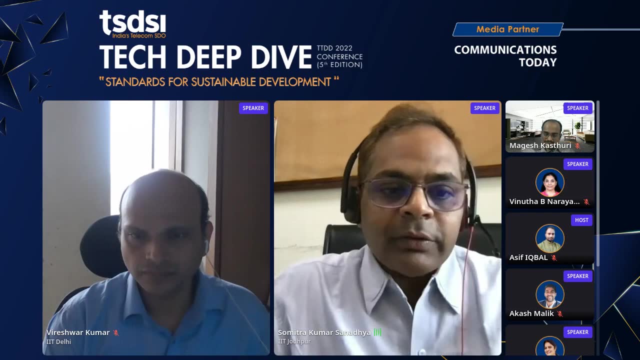 And these are problems which are hard, even for quantum computers- And basis these problems. we are now in a situation to design the algorithms. But again coming back to what Mr Valia and Mr Nath were mentioning in the beginning of this discussion, it is not enough to just think. 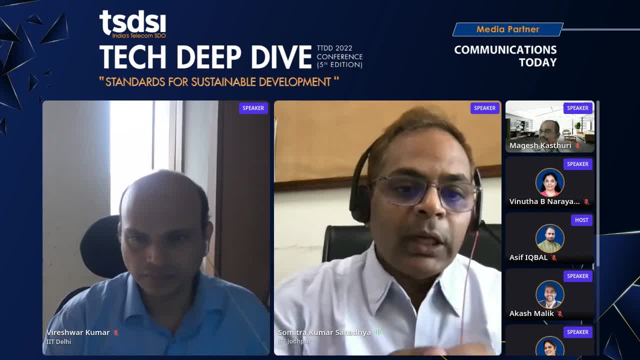 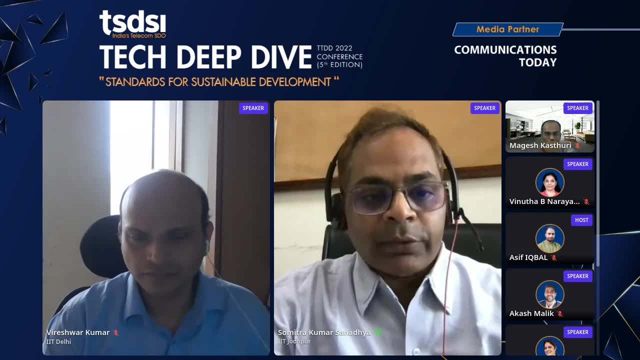 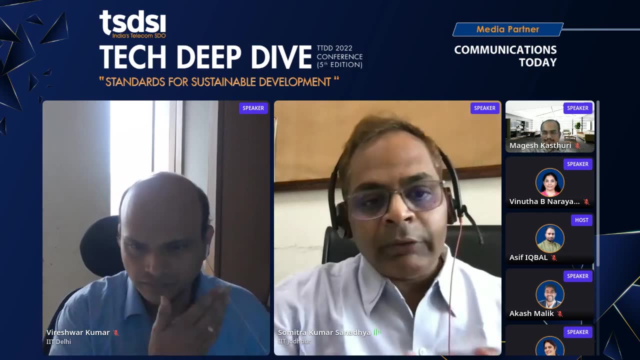 about a small tool. It needs to be deployed in a setup, And that deployment will only happen if there is a standard developed for these algorithms. You cannot just have any kind of parameter being chosen by different vendors, because then they will not be able to communicate. 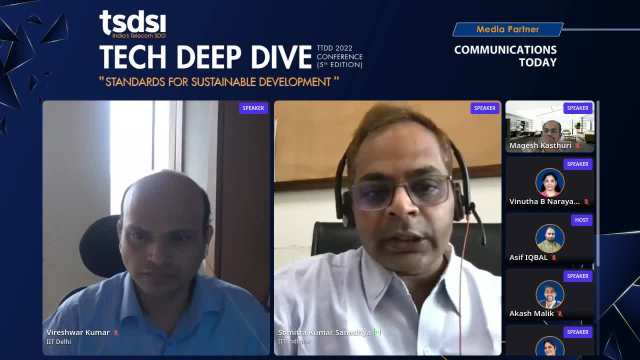 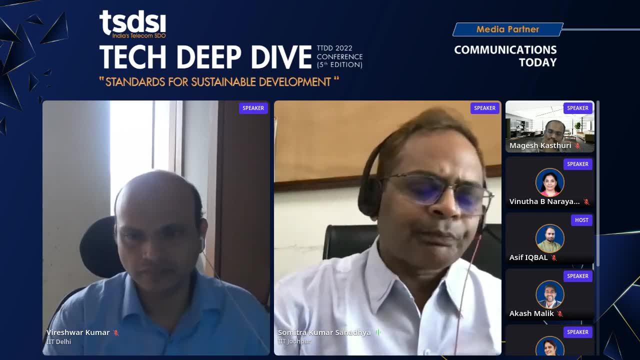 with each other. So this standardization process has started around 2016 and it is going on till today. NIST has already reached from level, so they initially started in December 2016 and they asked for candidate algorithms to be given to them. 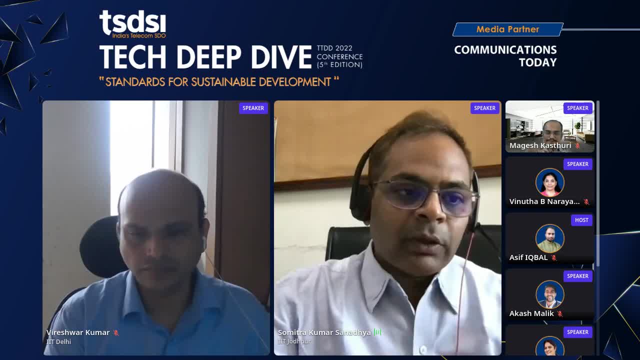 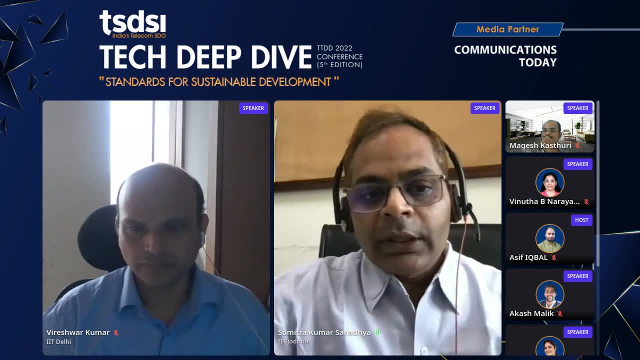 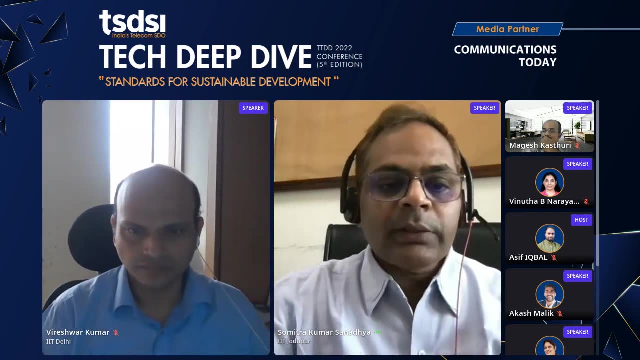 for public standardization And this process, first round, actually completed around December 2017, or may be November 2017, and there were 64 submissions of various kind of encryption algorithms: key exchange algorithms, signature algorithms. This is precisely what we need in today's world. And very quickly. there were attacks found on some of them. By attack I do not necessarily mean that, a practical break. What I am saying is that the security level is not what was claimed in the algorithm. So a lot of these algorithms were removed by NIST. 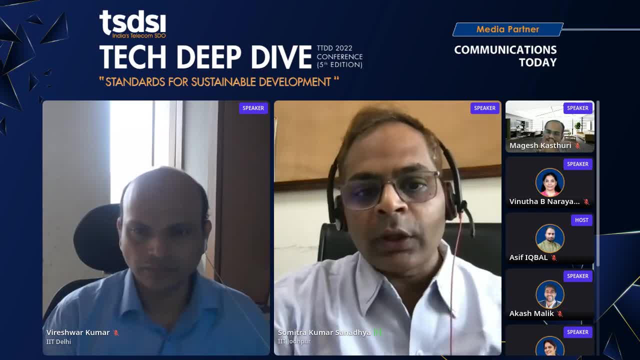 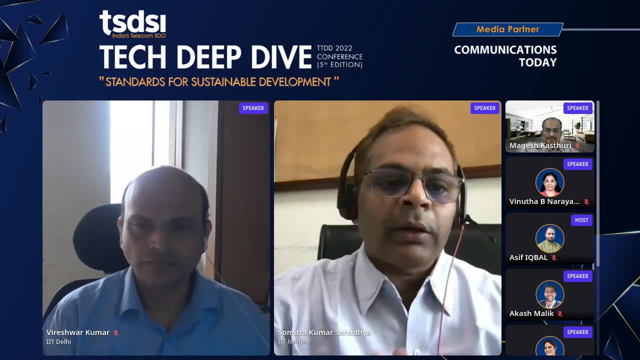 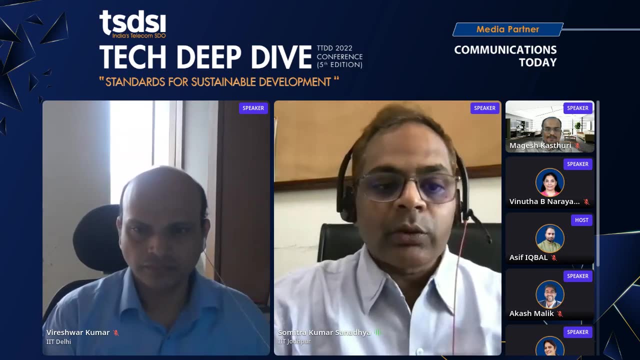 in this competition and then second round, third round and fourth round went on, and this year, few months ago, NIST announced seven final algorithms which are being considered for standardization and there are six alternate candidates for whom NIST wants further studies to be done. 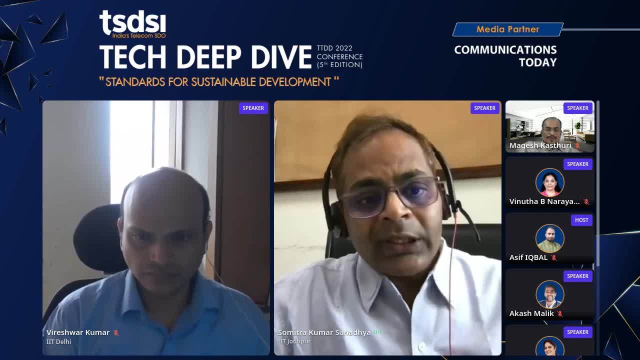 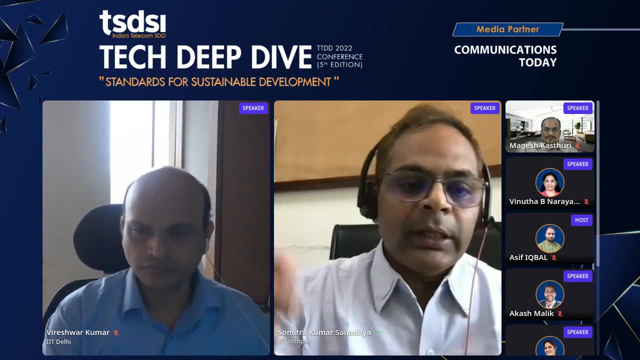 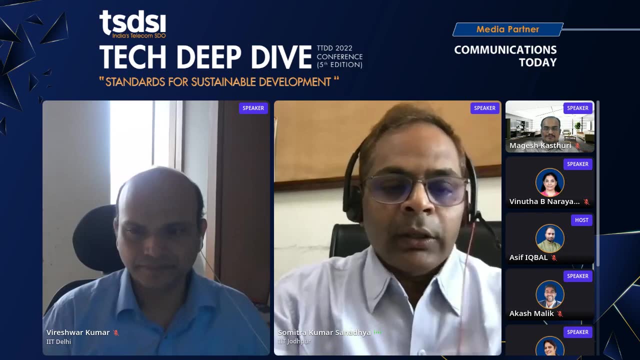 may potentially future standards. So this is the current state. However, we do not have these algorithms still in the final stage. NIST is believing that we will have these by 2023 and once the final standards are announced, deployment will start. 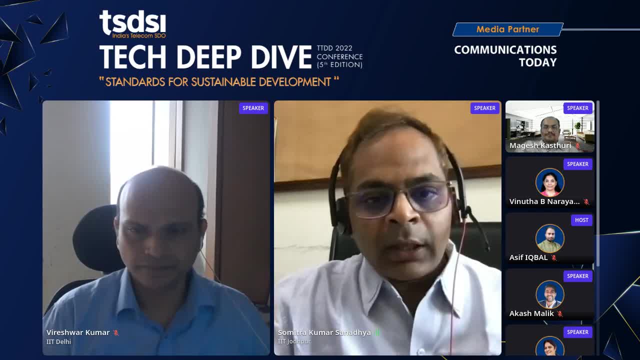 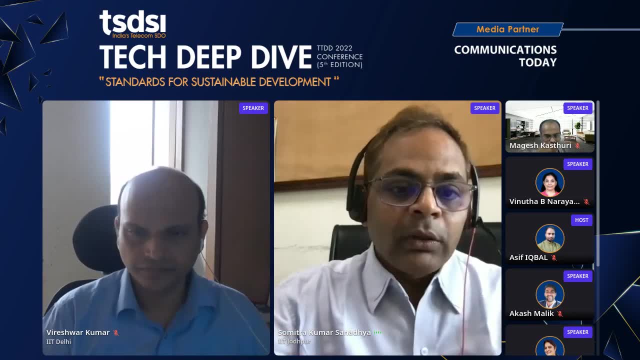 Again, deployment is not very easy. It is not like an academic algorithm which you take and implement. If you look at the history of attacks on public cryptographic algorithms, most of the attacks did not happen because the algorithm was weak. Most of them happened because there was 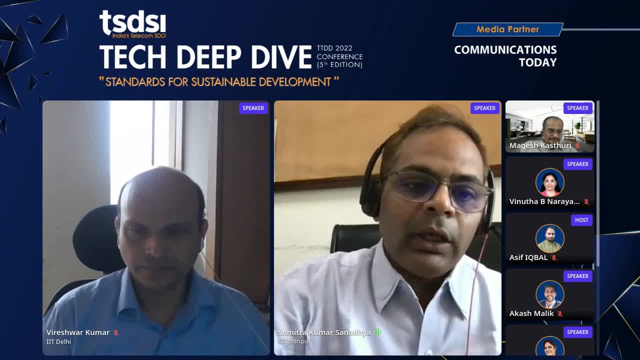 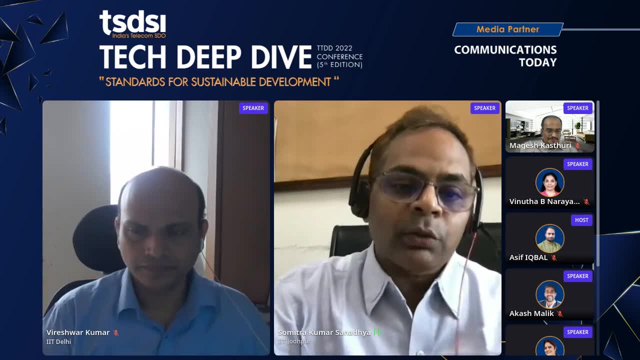 either implementation weakness or there was a weakness in one of the inputs which were coming, Most likely maybe. say, a true random number generator or a pseudo random number generator, which was not really so random, is expected And this led to a lot of attacks. So there can be many inputs. 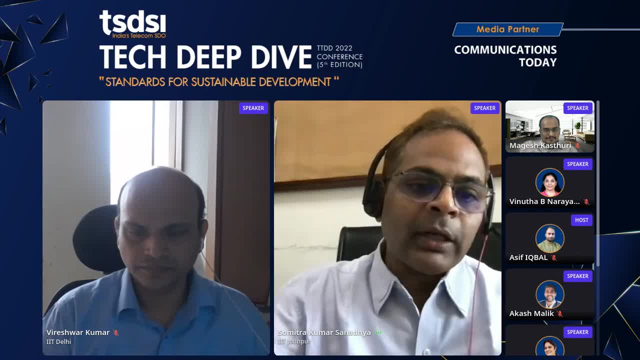 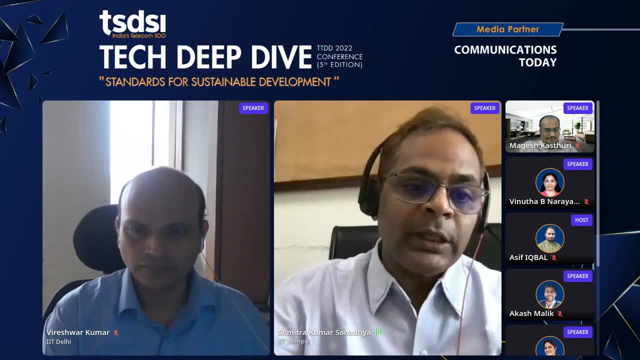 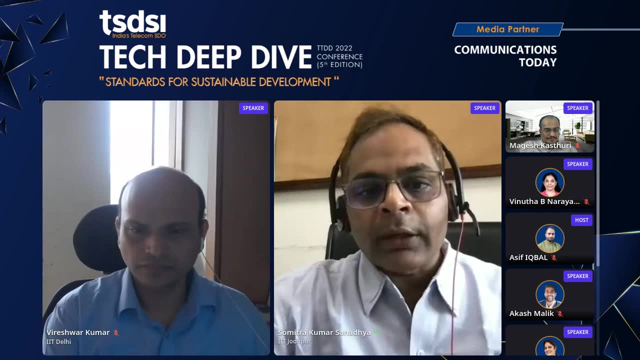 or many parameters which are playing a role in final implementation or deployment. So these are still being studied and this is where the current focus of researchers is and we hope that in next few years we would have matured and we will have deployment. So, as Dr Narendranath was already, 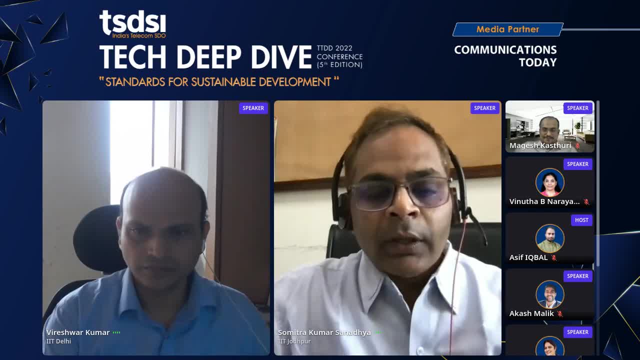 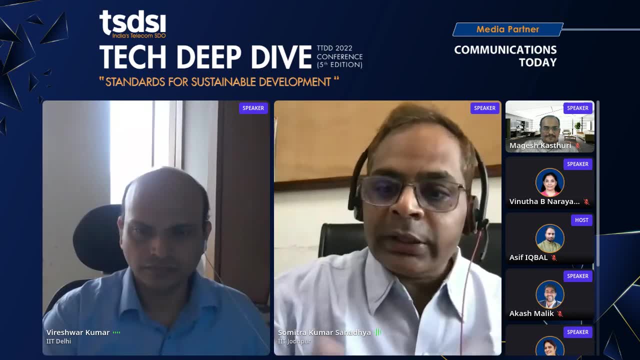 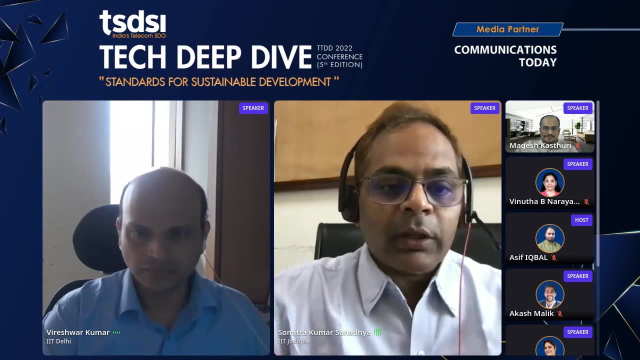 mentioning about CDOT as a trust center. it is actually very nice to see support of the NSCS and the great work being done by organizations like CDOT, which are actually taking a lead in the post quantum critical security. already They have begun to deploy some of these. 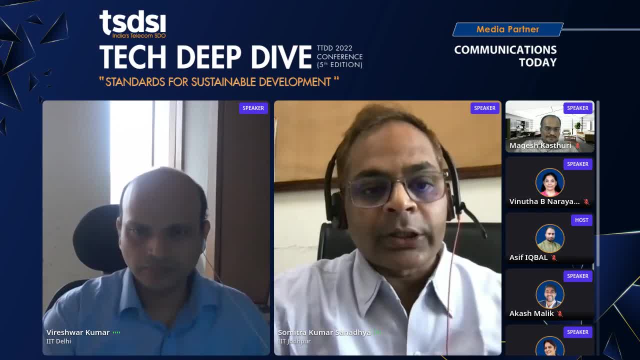 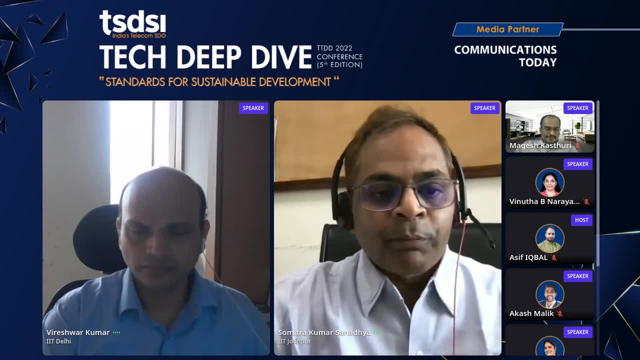 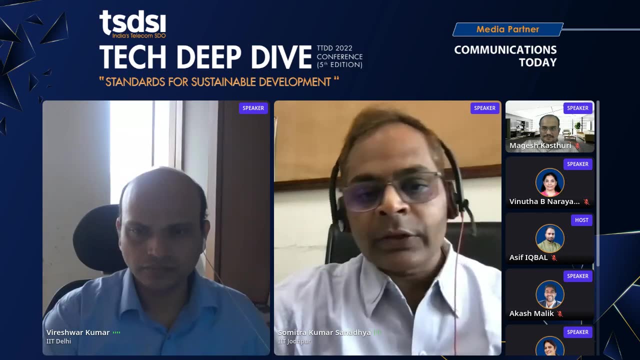 algorithms in a test case inside their products. So I am very, very hopeful and excited that maybe in less than say, five years we will start to see the deployment. The next question you talked about was whether it is feasible on, say, various kind of devices. 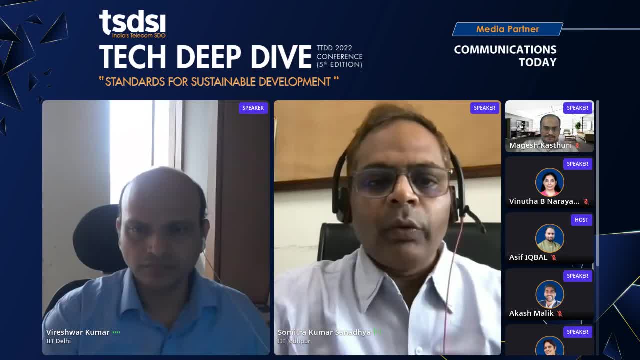 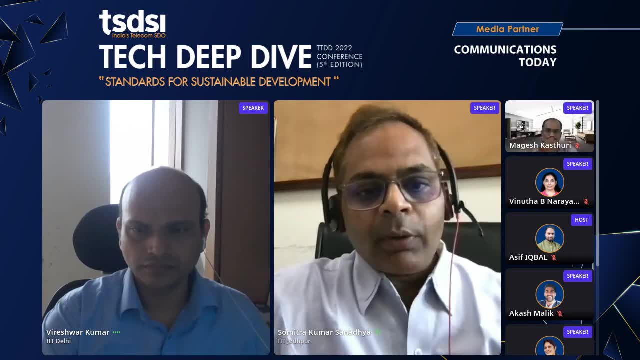 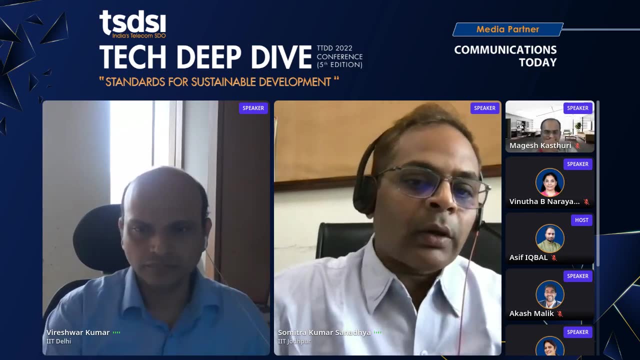 which are going to be in 5G. So most of these algorithms are based on essentially four kinds of problems. Either they are based on lattices, where certain problems are very hard to solve, even for quantum computers, or they are code based, or they are isogeny based. 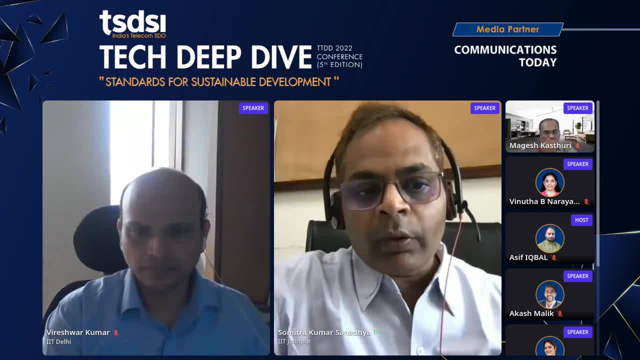 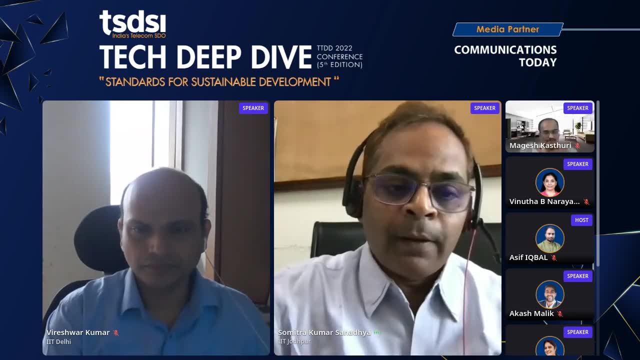 or hash based. So this is the four classes of problems on which post quantum critical algorithms are essentially, fundamentally based on. Most of the algorithms that we have studied are actually in these four classes. Now, lattices are still good to deploy, even on small devices. 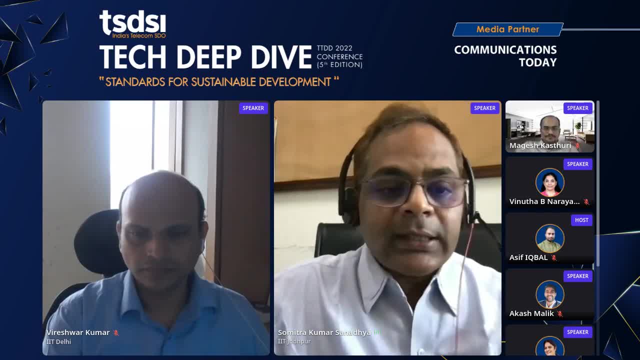 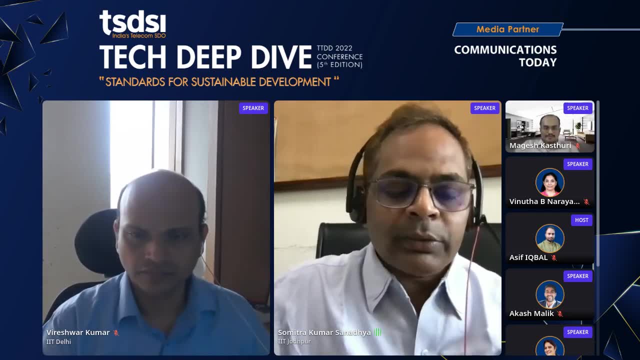 but some of these algorithms are so heavy in some sense The key sizes are something like, say, 10 kilobytes or 100 kilobytes, So you certainly cannot fit in these kind of algorithms in small devices, which are likely to be there. 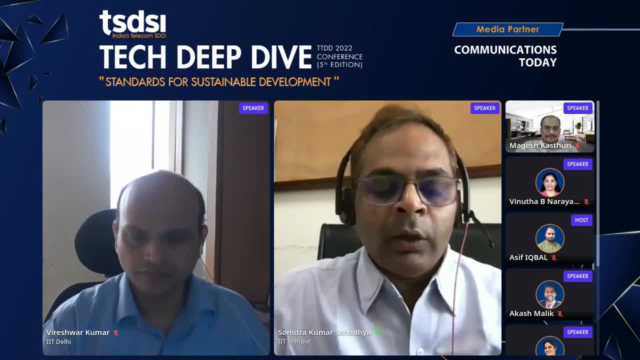 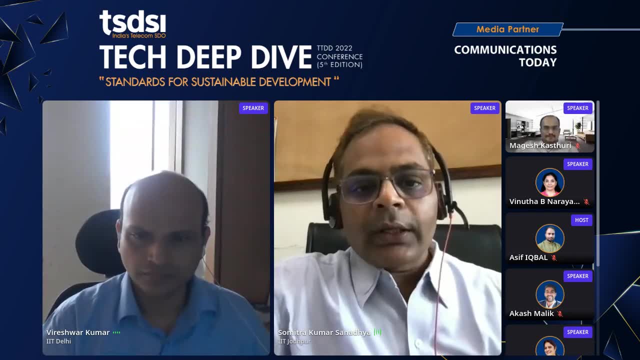 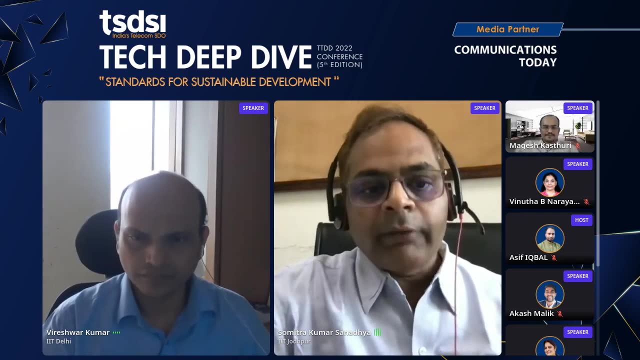 in 5G networks. So we are still looking at the final decision on the PQC algorithms, but it appears, as of today, that at least certain lattice based algorithms, or at least some variants of them, are still available, even for small devices, lightweight devices etc. 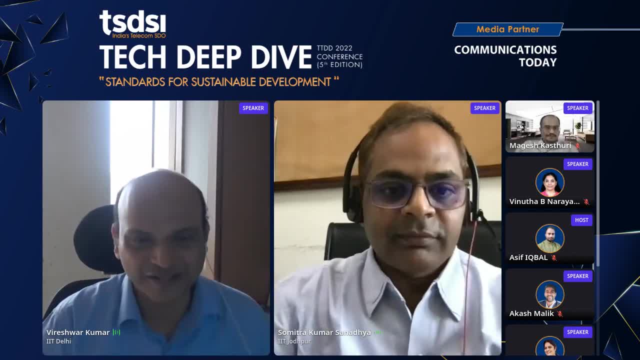 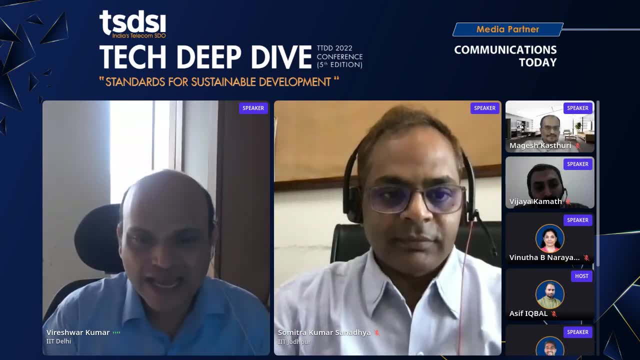 So this is what I would like to present at this moment. Thank you very much. Yeah, thank you, Professor Sanadhyay. Thanks for bringing out this aspect, that 5G will be the enabler for Internet of Things and even with the development. 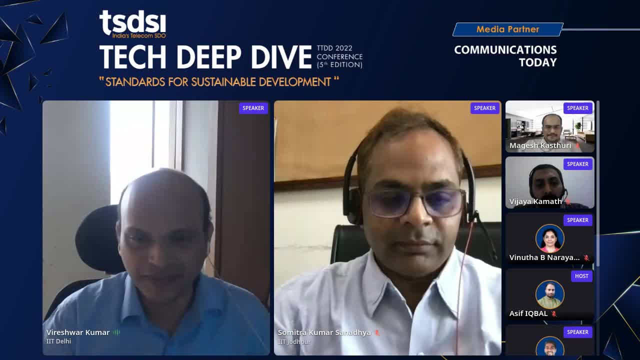 of the existing security mechanisms and the complementary quantum safe crypto systems. it is possible that many of those crypto systems may not be implementable on IoT devices, but that is true for our conventional crypto systems as well, and hopefully there will be some solutions there. So let me now 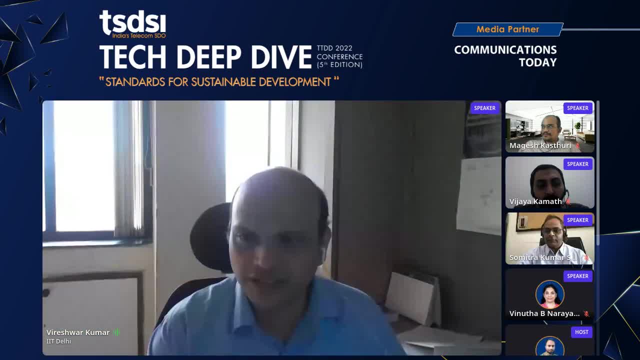 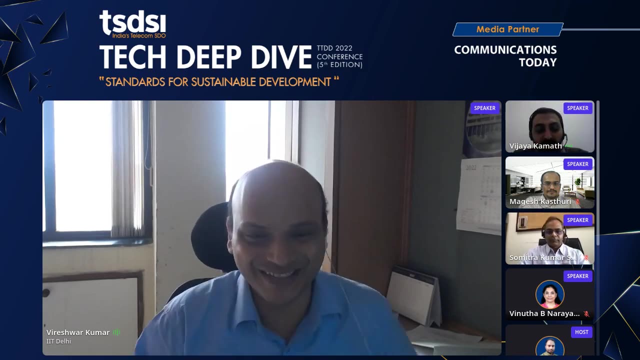 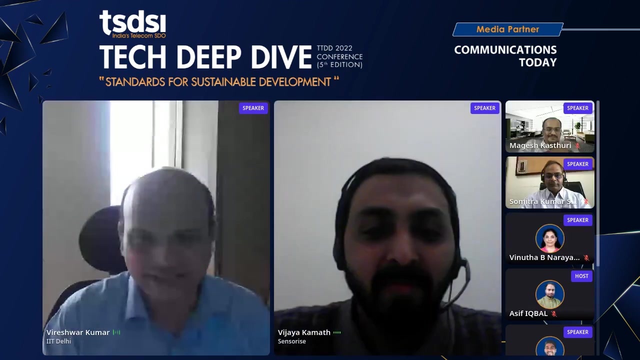 go to our another speaker, Mr Vijay Kamath. Mrs Vijay Kamath, Sir, I will be taking from her side. You can continue. I got confused there. Okay, so now we are at the stage in our panel discussion. 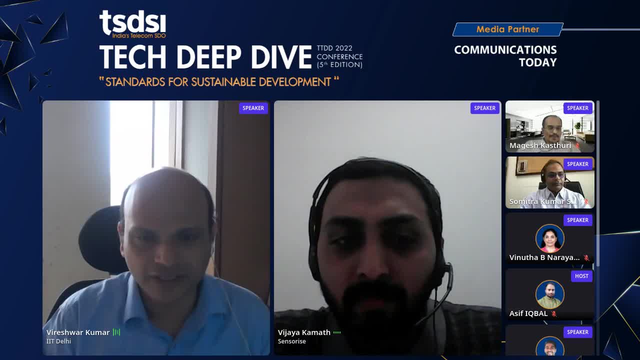 that we would like to understand the implications of quantum on IoT security. So can you please break down the IoT security aspects, how security is implemented in IoT and what are some of the requirements, and then what will be the role of quantum in that scenario? 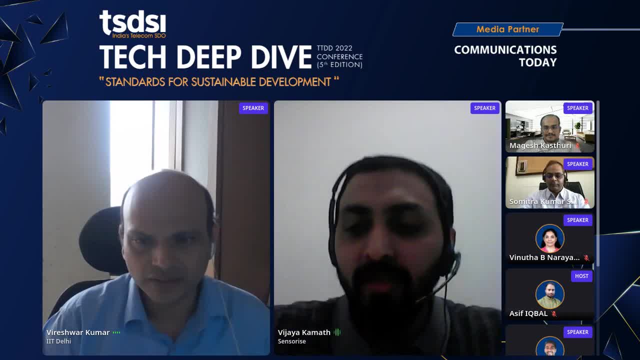 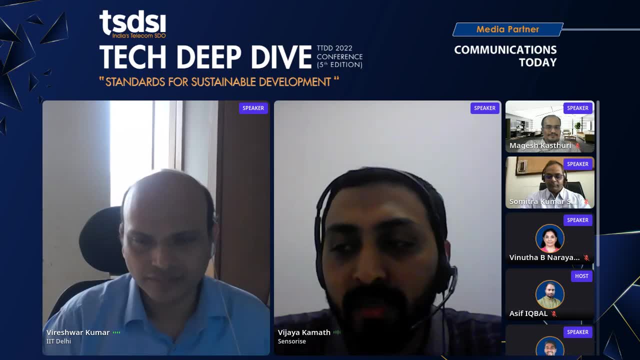 Right, sir, So majority like. if we talk about IoT, we have seen significant growth in numbers in IoT devices. From last year, it has grown to 18%. Now the total devices connected in the network is 14.4 billion, which will increase to almost double. 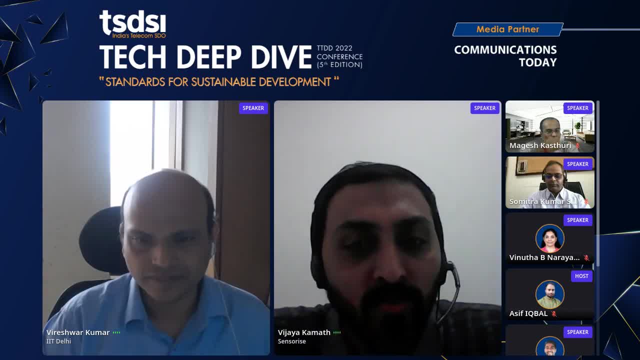 27 billion by 2025.. So definitely, as you mentioned, that it will have an impact and quantum will also have an impact on this. But, as rightly mentioned by Mr Walia, we are in 5G network, which is seeing the surge in the IoT. 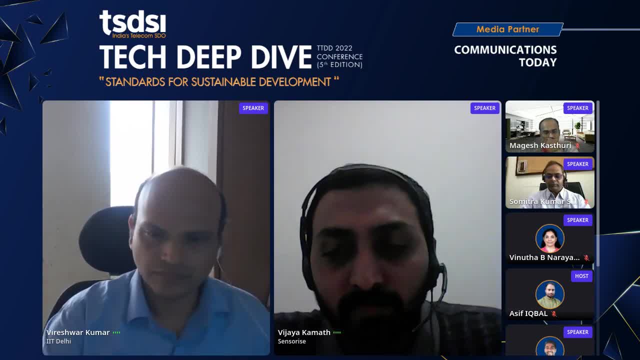 devices connected in the world. We, with 5G developments and the developments which have gone into the OS sided of the SIM card, where we have covered the previous 4G, 3G and 2G network deficiencies which were there, the security deficiencies which were there, into. 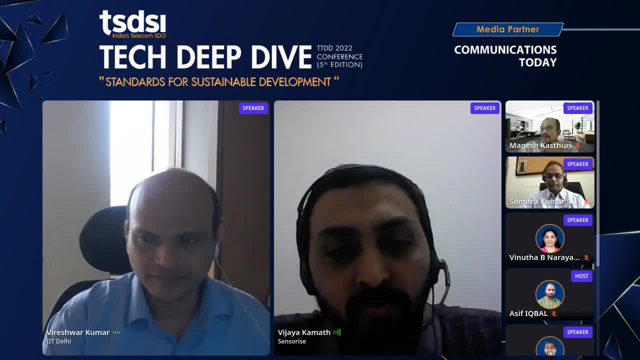 the 5G, The new authentication algorithm is introduced where IMSI is not being directly sent to the network. There are pretty much encryption which is developed across 5G, which will protect the devices from vulnerability, But this is towards the SIM card only and the network only. 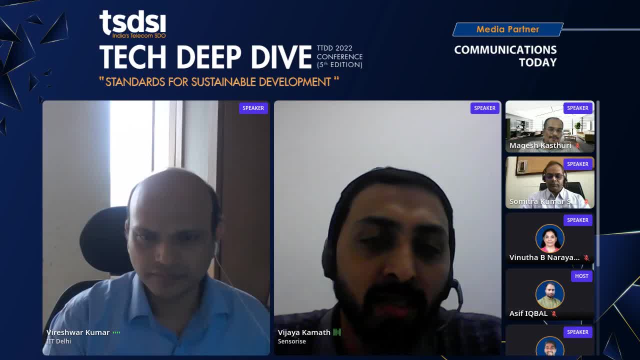 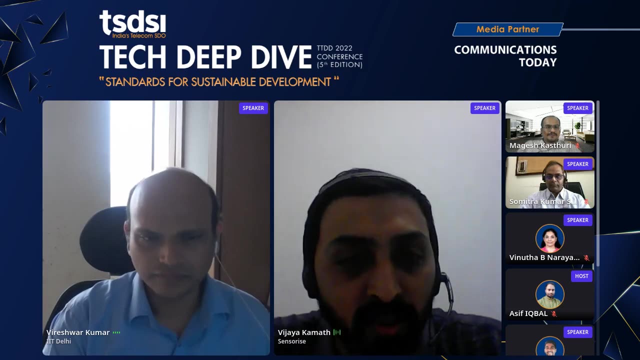 Yes, as correctly in the question mentioned, that IoT devices are still not protected and, as Mr Sushil Kumarji mentioned, that TEC is coming with the code of practice where they have highlighted 11 points to do the device certification and implementing the vulnerability in the 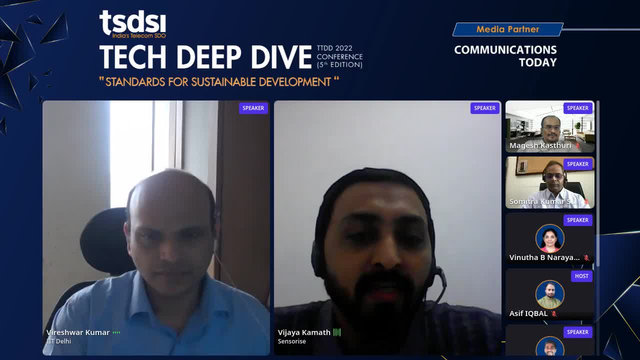 devices. So three. they have guided three points for the industry to take up forward, which is first: is password encrypted, the photo could be updated if we found vulnerability, and the device should be tested first before going out in the market. So countries are following. 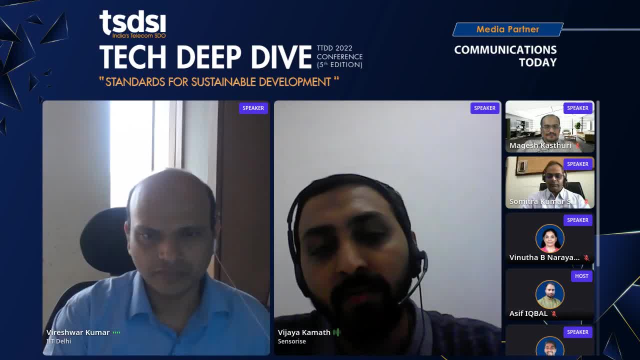 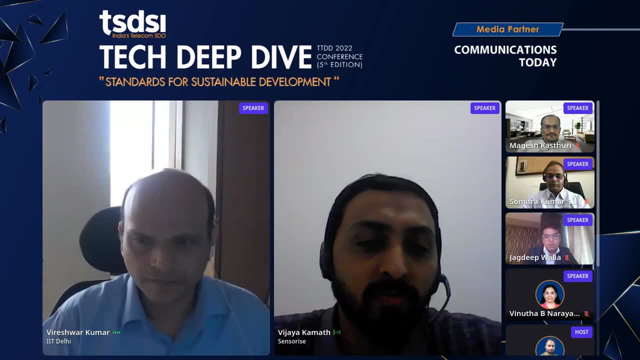 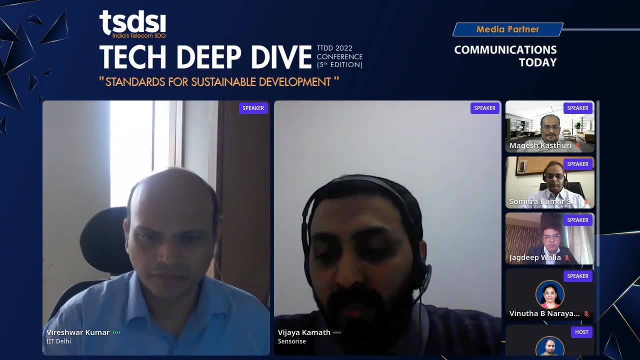 norms to certify the devices before we export, but definitely we should have when we import also and when we produce for India also. we should have some certification in line so that we could protect the threats in the IoT industry, as the numbers and the quantums are going on, Then 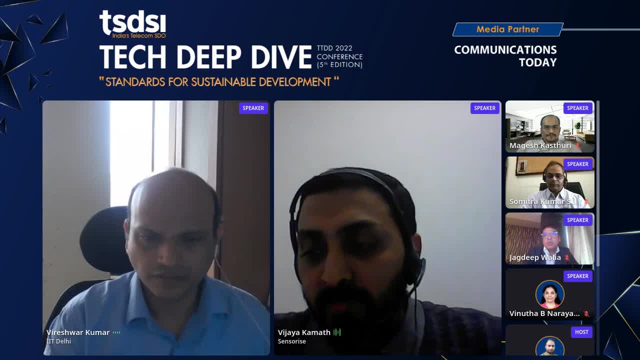 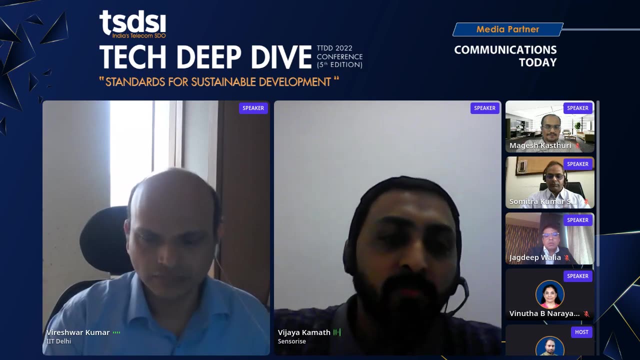 as Mr Walia mentioned, we have encryption methodology on the card, on the network. CF is there, Sufi is there and rest of the mechanisms are there. Then we can build multiple applications, either on the card and on the devices which could be. 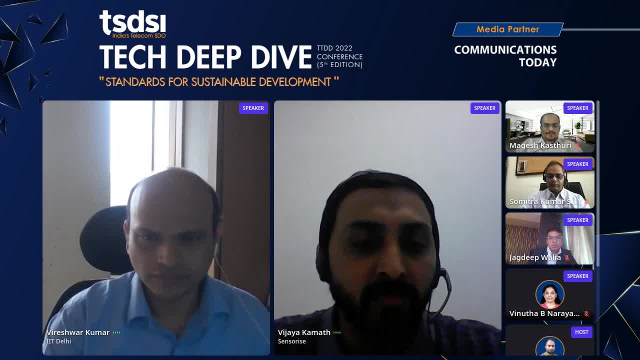 on AES minimum, AES 128, which is quantum effective right now, so we can have the applications encrypted, the data encrypted, using the technologies and we can move. we can somehow, till an extent, could avoid the issues, vulnerability issues. but yes, we should have some guidelines, the research work. 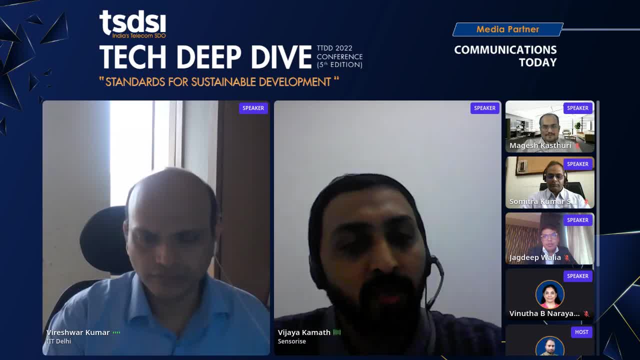 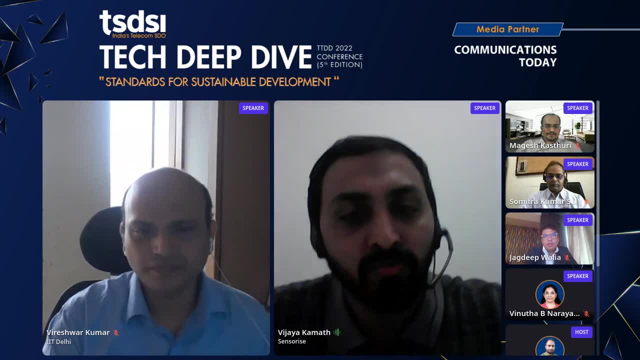 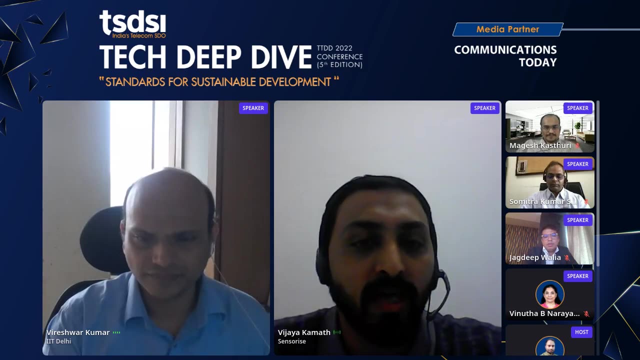 which is going on parallel in the institution, to adapt in the devices the IoT work structure, the application structure, so that all these issues could be avoided. So we have together, like GSMA has included iSafe, how the data could be encrypted. so people, the manufacturers, 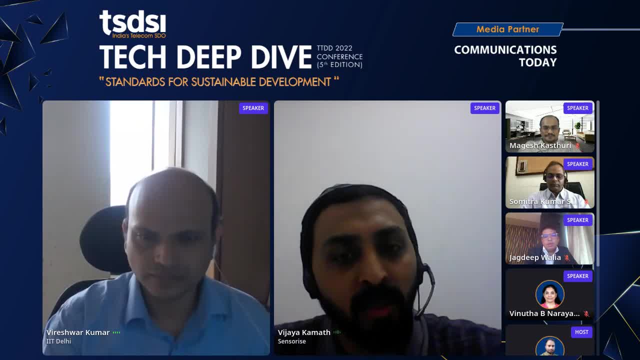 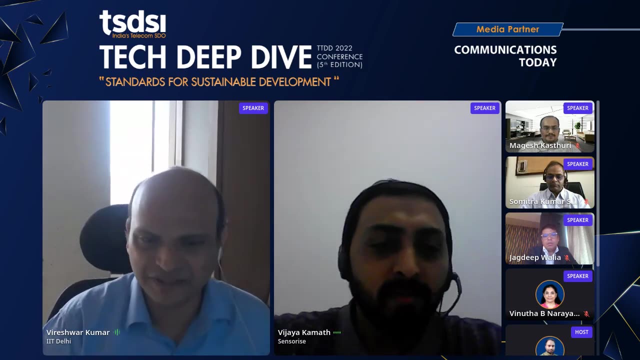 the device side and the sim card side should start adopting those standards and specification for better utilization of the already existing standards and the and the security which is there on the ground. Thank you for bringing that perspective to us. I guess at this point we should. 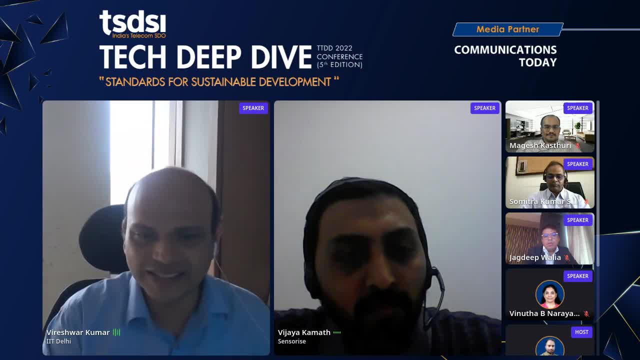 try to see what are some of the industry initiatives in this domain of enabling security in this discussion about 5G and IoT that we are looking at. So I will go to Mr Kasturi, So could you please tell us about some key initiatives? 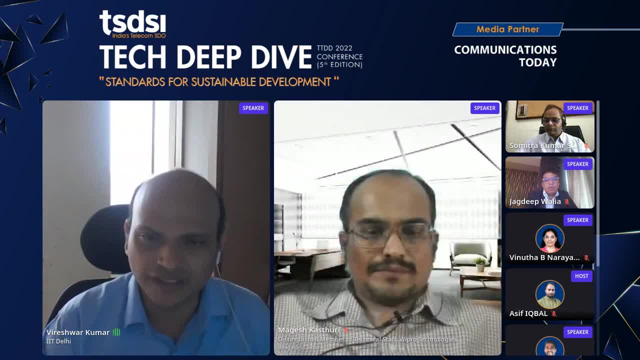 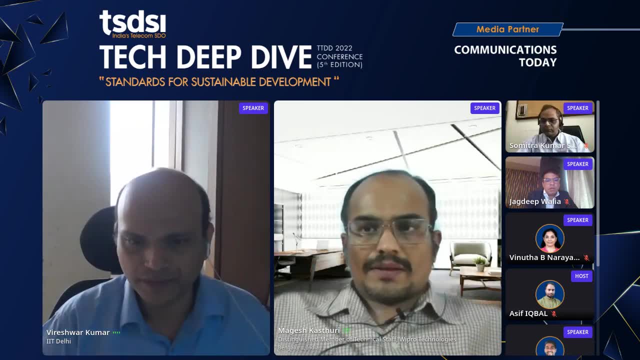 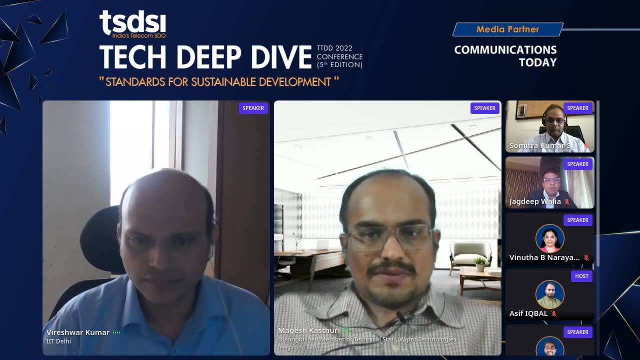 that have been taken by the industry for resolving some of the security issues, especially in the IoT domain? Yeah, thank you. Thanks for inviting me for this panel discussion, So let me give you a brief answer to this question about some of the IoT related. 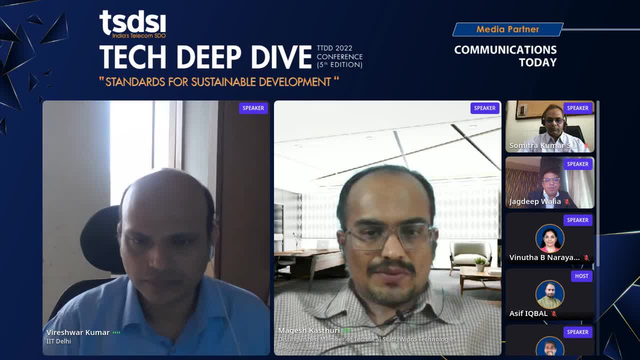 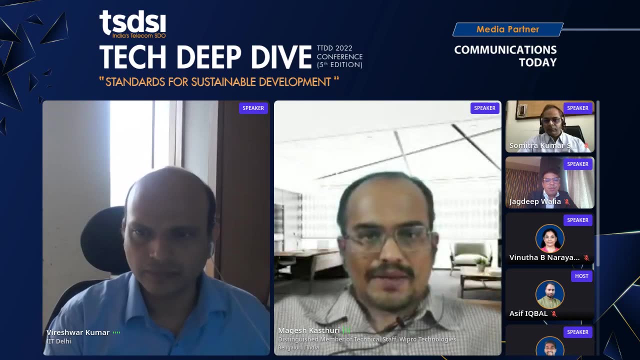 threats. So I would like to quote two reports: one from BlackBerry, BlackBerry Trend Report 2022, which talks about top 10 security threat issues, and in that, one of the major issues that they have highlighted is the IoT security issues, be it application level IoT security issue, or 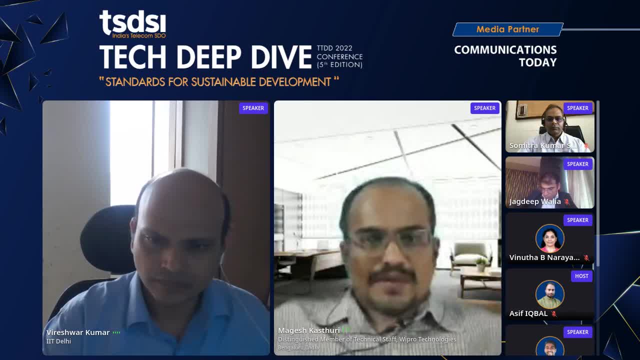 the network and infrastructure level issue. I will be explaining that in detail. The second one is from Singapore Computer Society, where they have published a trend report about cybersecurity- top 5 cybersecurity issues- and they have quoted IoT security threats in terms of how each client 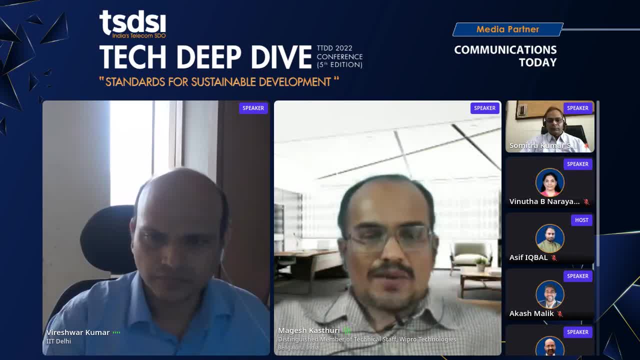 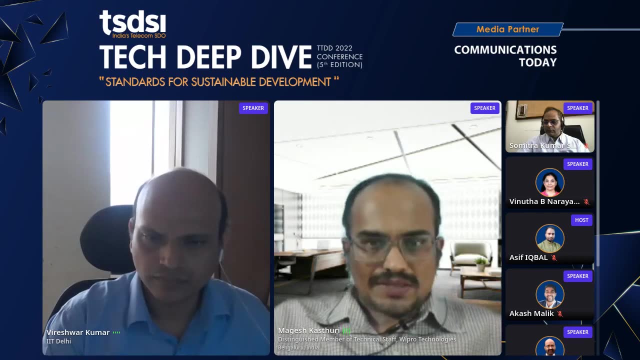 is having unprotected data or how unsecured storage services being used by third party in the IoT ecosystem. So they have quoted that as a key issue, as one of the top 5 issue with respect to cybersecurity. So, quoting these two references, you can understand. 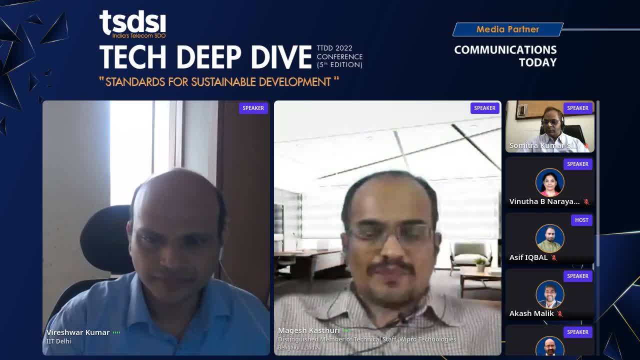 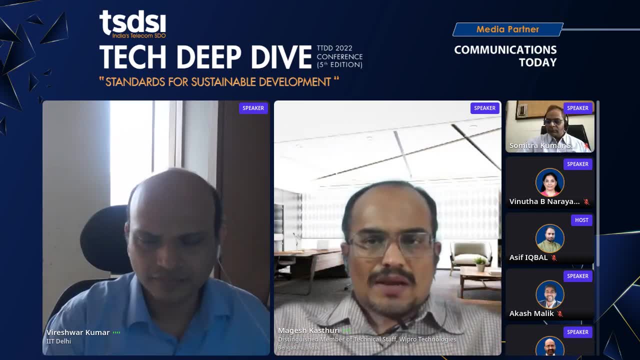 that the importance and the emphasis on IoT challenges. So when I take IoT security issues, I can look into that into four different stages of security issues. One at the infrastructure level, which is at the physical device, and physical infrastructure level It could be on the edge client. 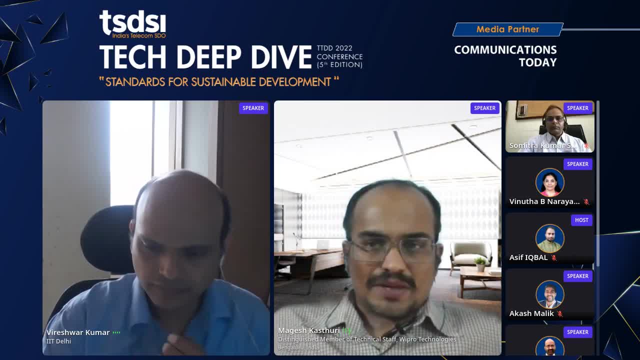 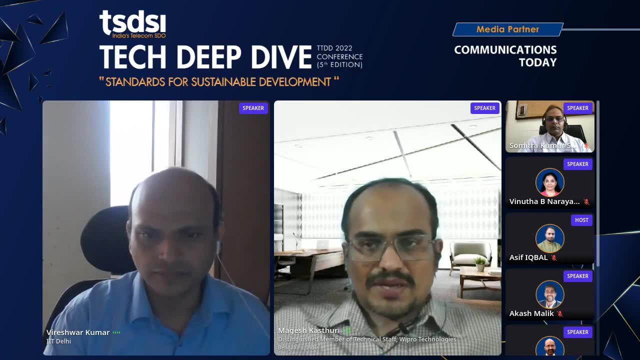 or it could be on the IoT devices, be it a smart watch or an IP camera or whatever it may be, but physically on the device level, which is the infrastructure level, IoT security issues. The second level could be on the platform level security issues where it will be, for example. 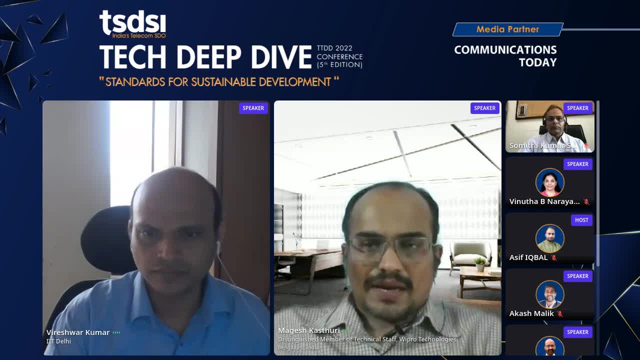 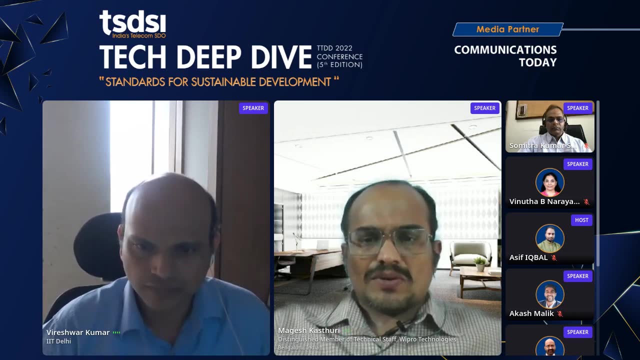 on the edge or on the gateway where it collects the data and sent it to the cloud services. So at the platform level there could be security threat issue that you need to address. The third level could be on the communication or the network level. So how? 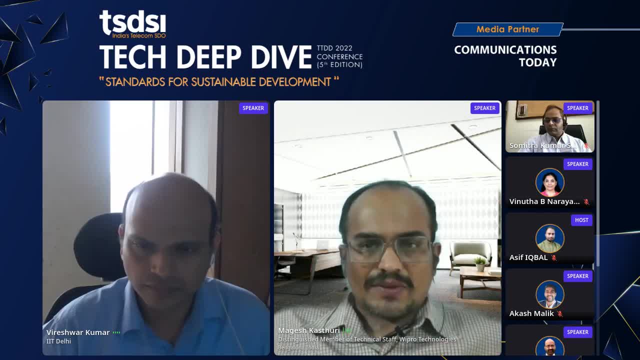 you are using the network protocol, or how you are using a secure channel or an unsecured communication channel to connect with your IoT services, edge gateway and cloud together. So how this is unprotected and how to handle it better, Whether you need to use 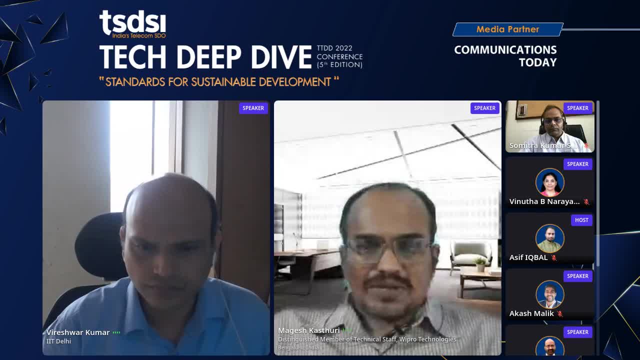 data encryption mechanism when you are transporting, like data in motion, data address kind of ways that you need to take to protect the data during network communication. That is one part of it. The fourth level, or the fourth stage, is at the application level. So if you take a 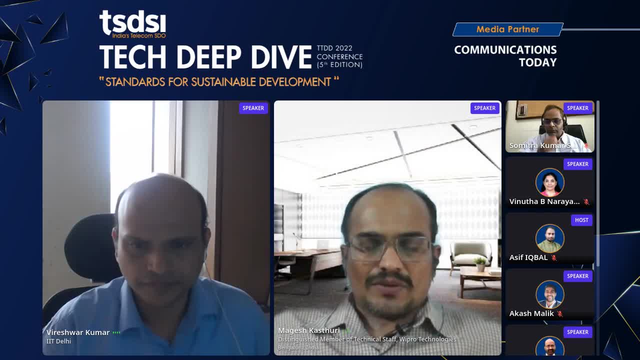 complete IoT ecosystem together. it could be from your organization level IoT services that you will be using, and also you will be using some third party legacy services and third party IoT services from external vendors, where you are already using data for a longer time, So some of them lack security updates. 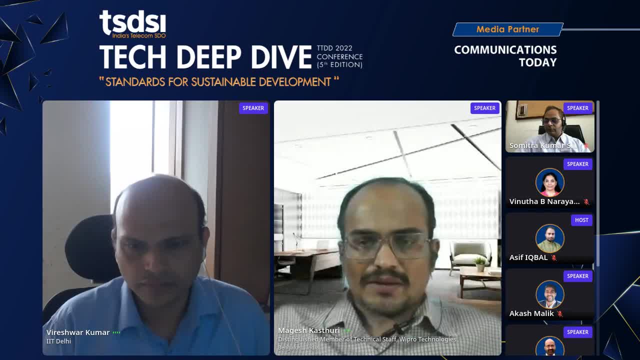 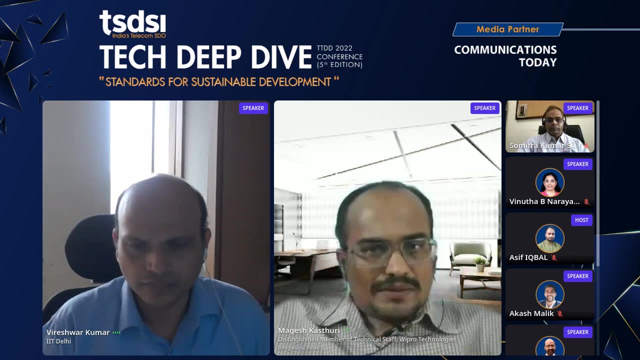 maybe patching would not be done, or they are not very clear about the role based access that needs to be given, So it could be potentially unprotected. So in that, in your ecosystem, if you are bringing that services also, then definitely it will have a security threat. 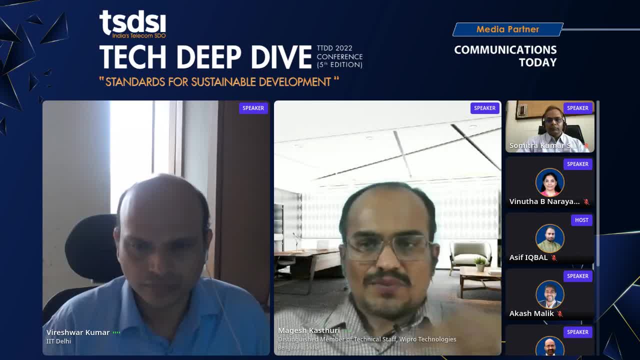 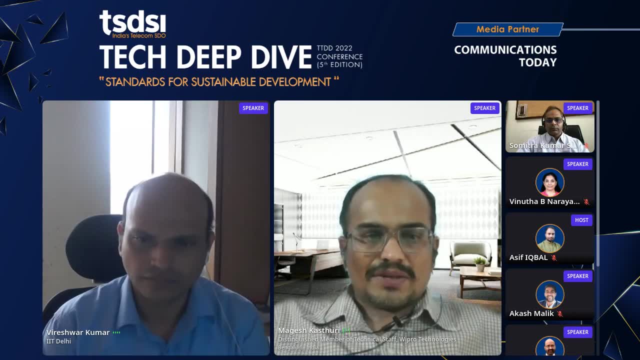 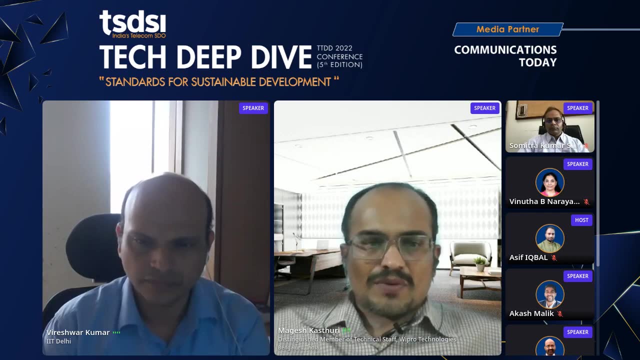 to the overall IoT architecture. So these four levels of issues needs to be addressed and that's where the emphasis goes on in the security challenges. Some of the examples which I want to give here about potential security issues could be like privacy, data privacy, like after the GDPR, and 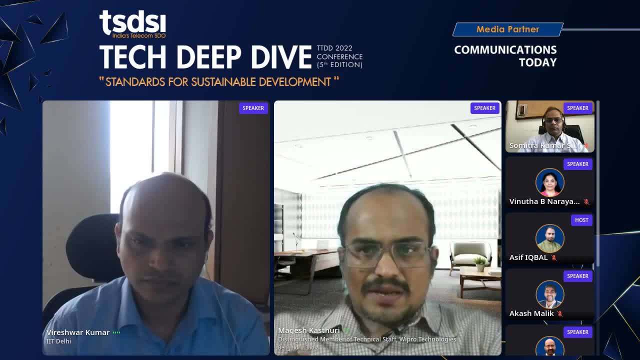 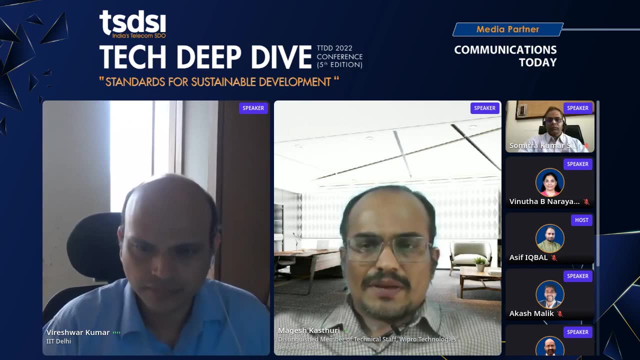 PIA comes into picture, where data privacy and how your private data being handled in a public domain need to be protected. There are various legacy IoT applications where, literally, this PIA or GDPR was not handled and they are enforced to do that because data privacy is at most. 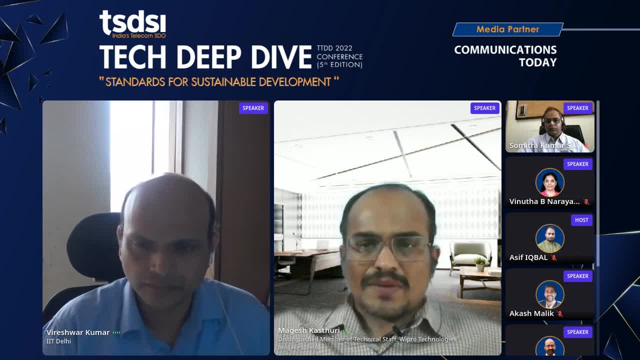 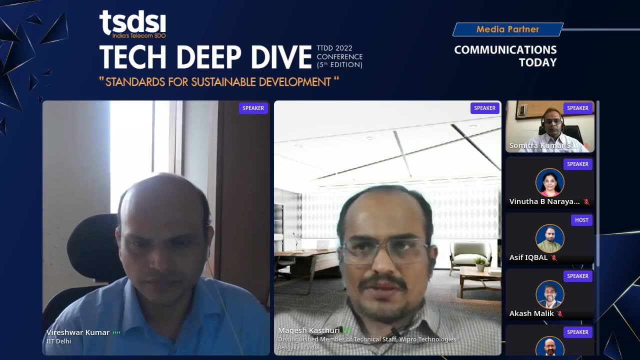 important and in a public IoT system, you should not have unprotected data, having your private data being there. So that is one of the important things that needs to be addressed. Second, how your data storage and data transfer being done with both the network communication as well as the storage services. 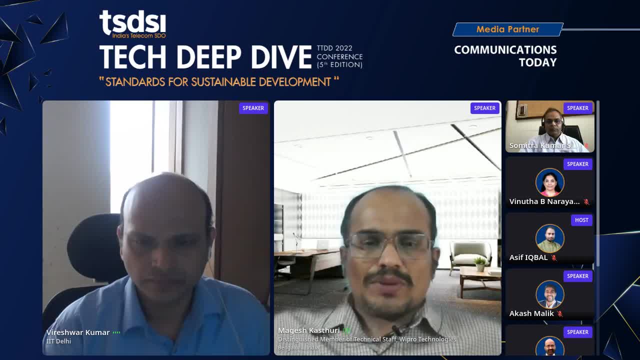 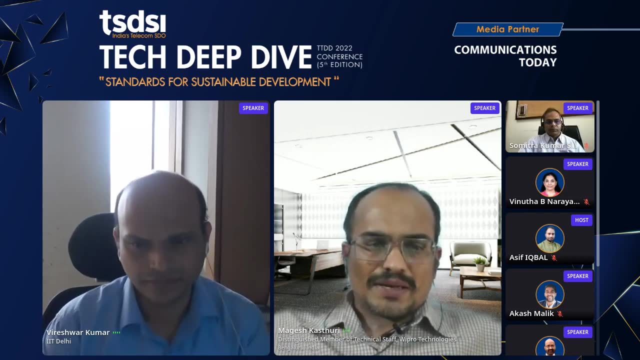 that you are using in the cloud and in the edge. So how they have to be protected, how you have to use an intelligent security mechanism to handle the storage service to be protected, as well as the network communication to be protected. This needs to be addressed. 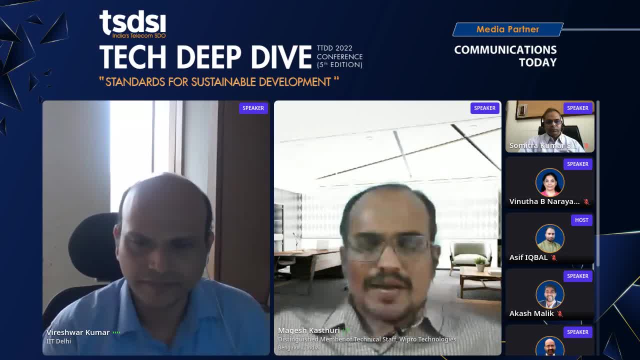 The next one is how you are having a kind of autonomous facility or an auto healing facility to the entire physical infrastructure services. So if there is some potential threat, how to recover on its own and how to make itself self-equipped, make the system and services to. 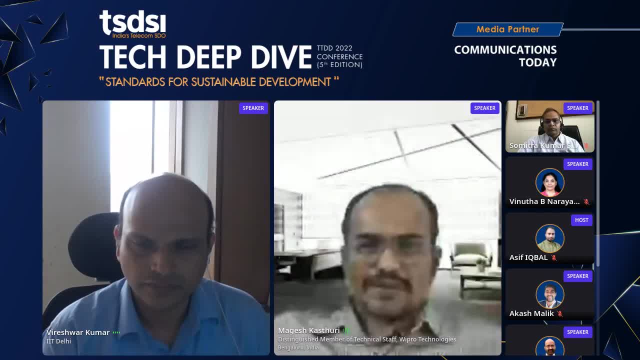 equip itself to be self-secure, to handle it in a better way, needs to be addressed So that you will have a modernized ecosystem in your IoT architecture. at the same time, you are addressing your long-term problem on automatically managing, preventing and monitoring, reporting your 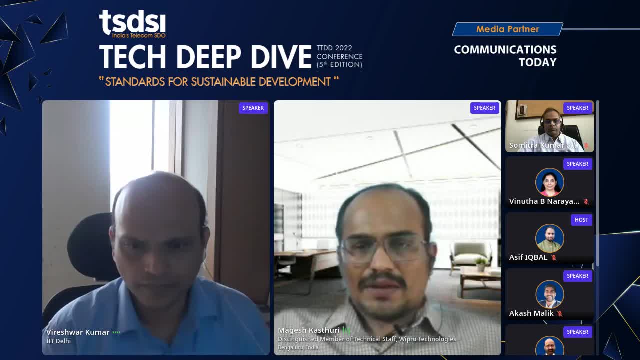 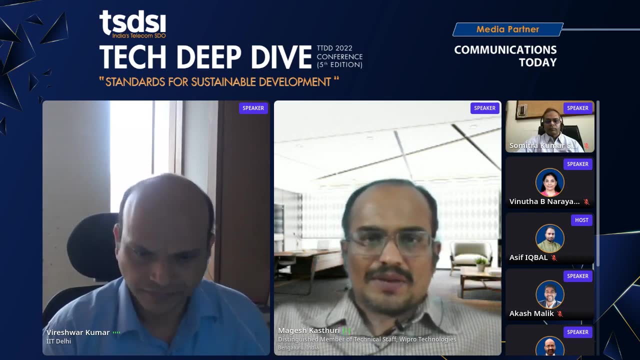 security issues upfront and that will help for the team on the ground to understand the criticality and act upon if needed manually, or pre-program the services to enable the security features automatically. So this is a brief view that I want to give about IoT security in terms 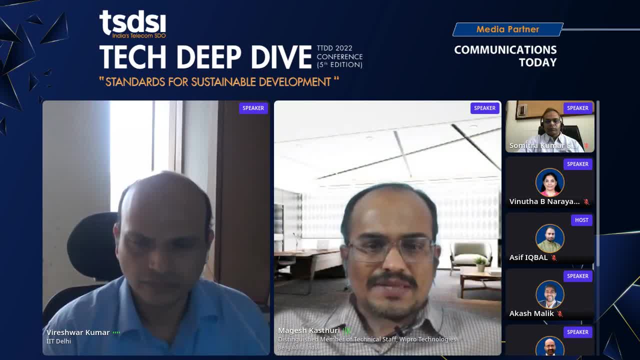 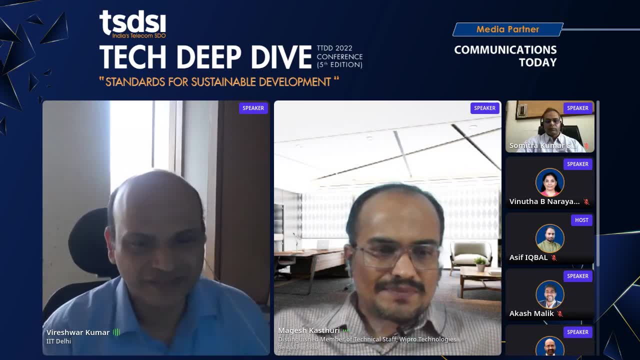 of the key principles in terms of the key challenges and the stages that you need to look into: the IoT security. Thanks Back to you, Veerish, Thank you. Thank you for giving us that perspective, So I guess now I will go ahead and go. 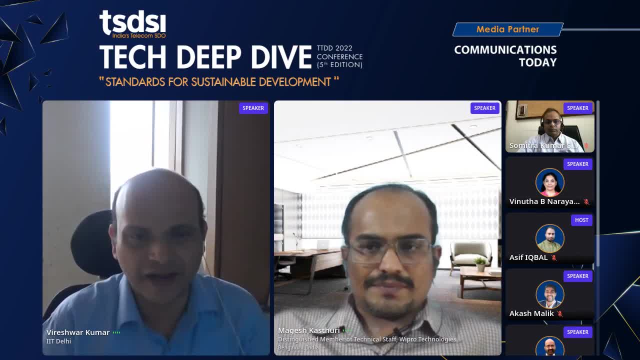 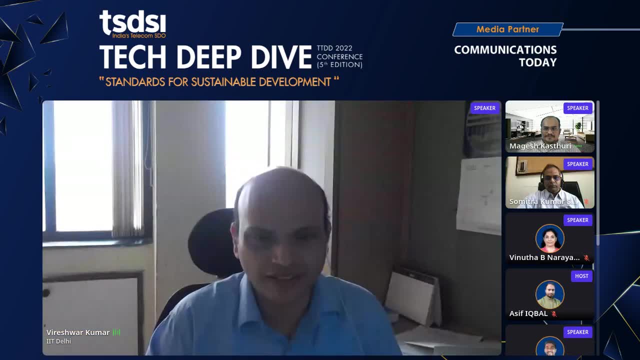 to each of the panelists for their remarks after hearing the different aspects. So let me go to Mr Nath first. So, Mr Nath, you heard what 3GPP is working towards, what the industry is focusing on and what kind of 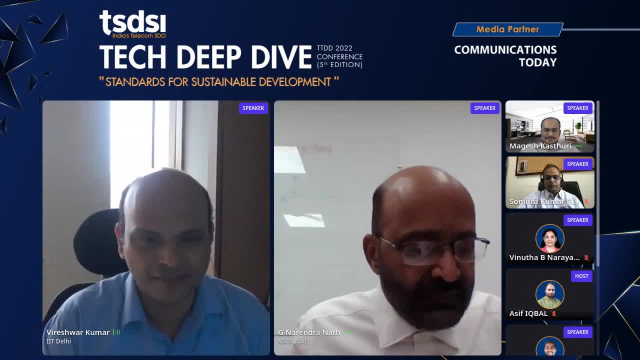 maturity level that we have in terms of quantum computing. So now I would like to quickly ask you for a brief comment on should we look into- are we also looking into- some India-specific needs? So we are definitely working on these challenges on a global scale. 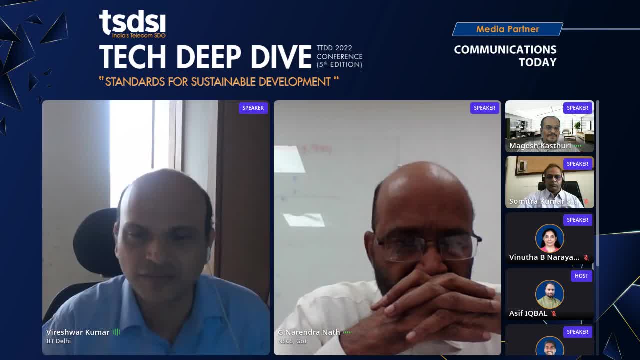 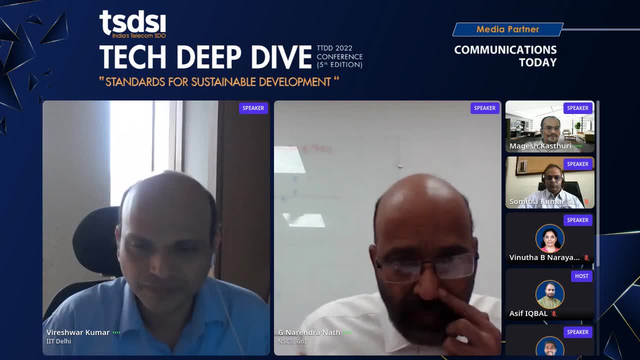 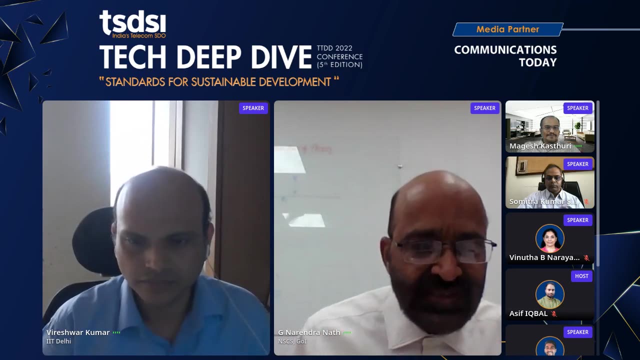 but are there some India-specific challenges that we should also look at? Yeah, I think one of the things is what all the points pointed out by the panelists that we have got. As it's been pointed out, 5G is more secure than the earlier. 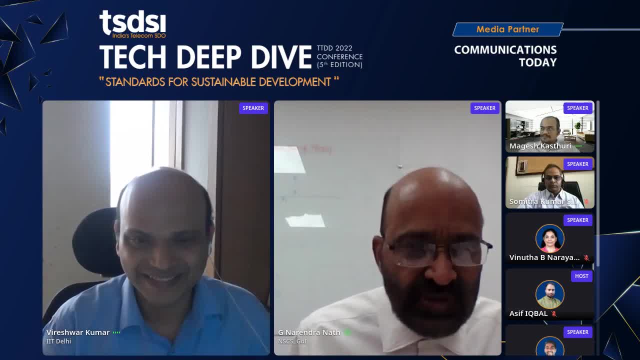 generations of that and because there's an understanding that has come about And one important point that was brought out is that zero trust is something that's been implemented across. That's very important, And there are also multiple enhancements that Mr Wali had. 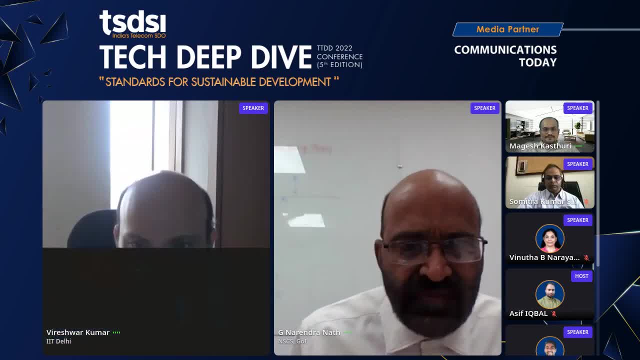 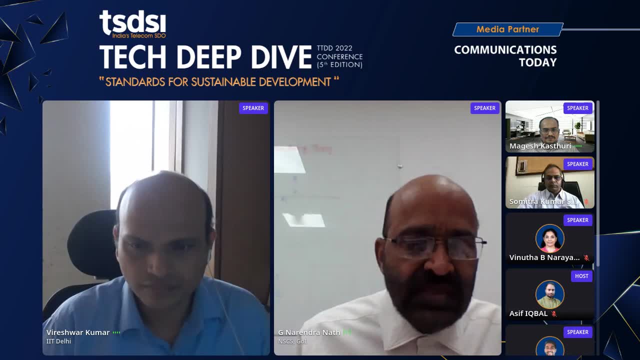 pointed out. that is there. If you look at India-specific, one of the concerns that we had is one is having standards and developing products as per standards. But then there is also an element of trust that we talk about. Let's see from where do these? 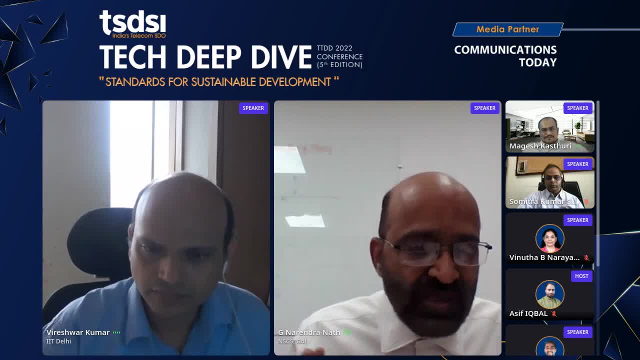 products come from. So standards are important. Then it's important that you certify test against that and then see that they are conforming to the standards and they're putting them in place, And that is one level of assurance that you get. 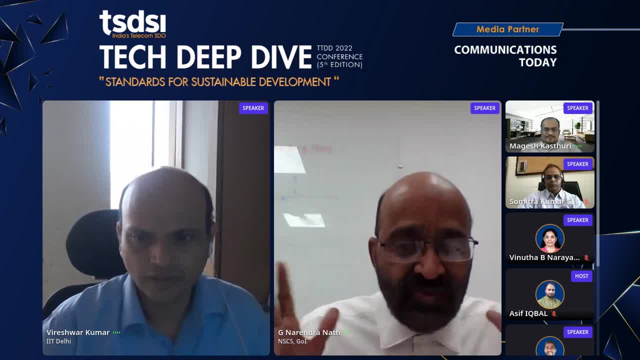 And that's a very important component of assurance, because there's a lot of thought that goes in from different members. But then we also found that bulk of equipment comes from outside sources, And how do you ensure trust of the equipment that comes in in terms of the intent that is there? 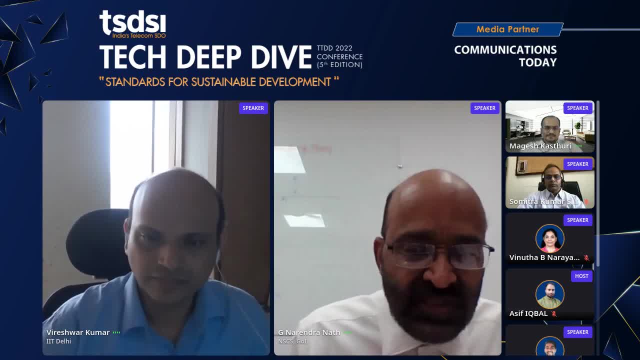 That's where we came up with this national security for telecom systems, telecom services, where we have asked that we are also looking at the sources from where this equipment is coming from. So you could say that it's an India-specific solution that we are trying to address. the 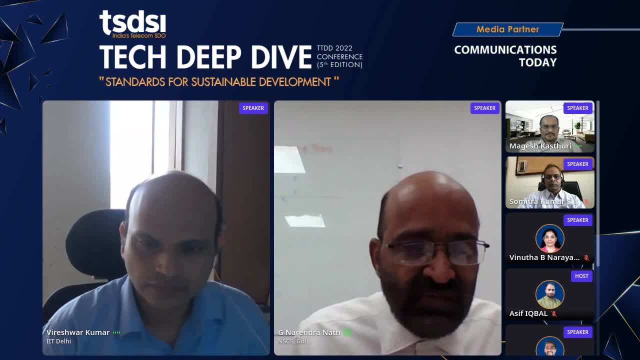 problem, without actually going and saying, you know, going for a negative list, coming up with a positive list, of saying that this company we have evaluated based on certain parameters, to say that this is, as a company, a trusted source from where the products would come And as a 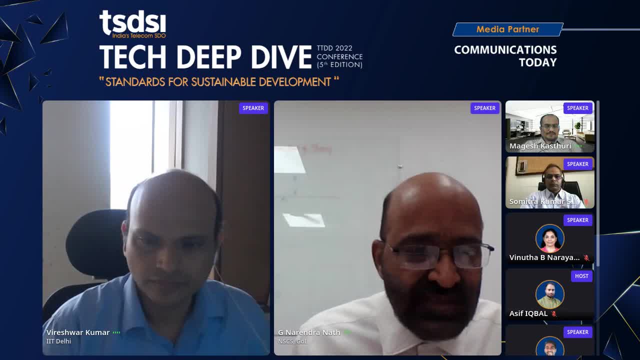 company- these are components from this- are trusted, Not specifically looking at standards, which is a different dimension, but looking at other processes in place, that you know, governance principles, that they have The type of people who are there where it is based and 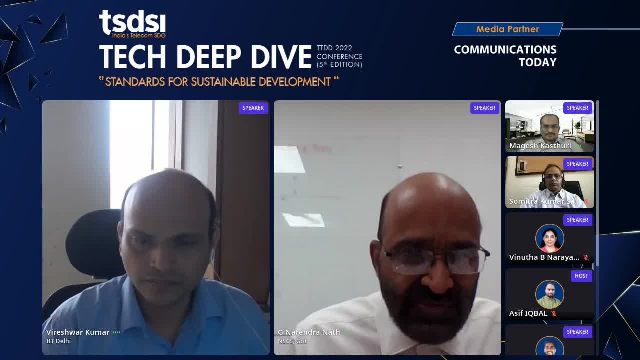 internal processes that they have. So that is one thing that we have added here, And I think some of the other countries also looking at the system that we have put in place to see if that could be replicated in their countries. Of course it's a very elaborate exercise. 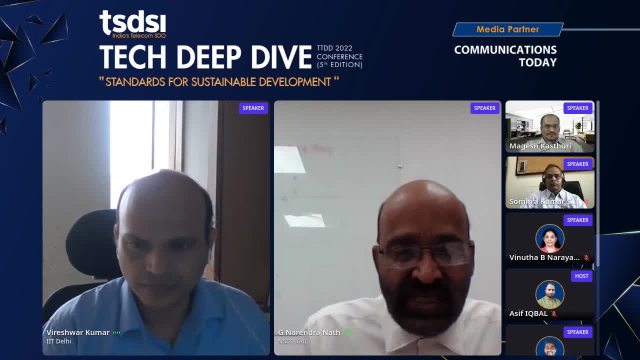 involved exercise, but that's something because of the criticality and the multidimensional 5G deployments, multistakeholder 5G deployments that are happening, that we felt that they should also be part of this whole security exercise. Yeah, that is very important. 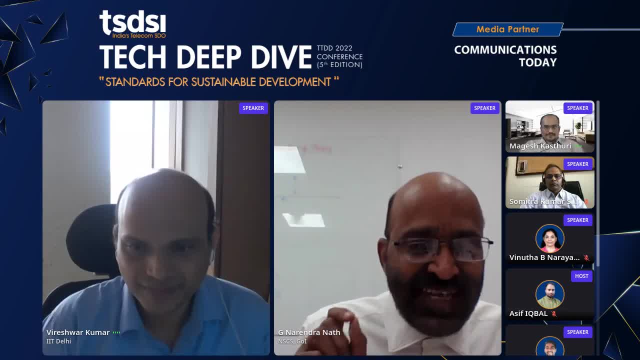 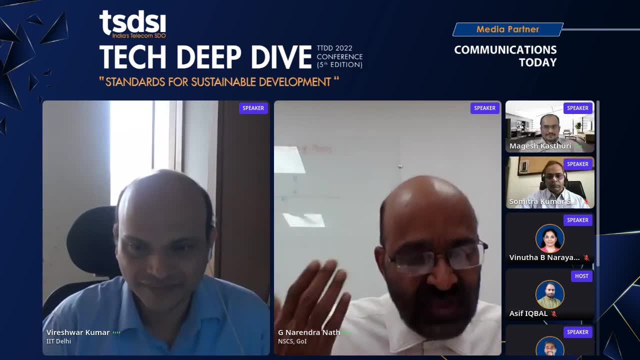 to note that. Yeah, here is. the challenge is that: how do you ensure the security of the supply chains? We are doing some exercise, I think, but there is still some work to be done to actually work to find out how do you really ensure a robust supply chain. 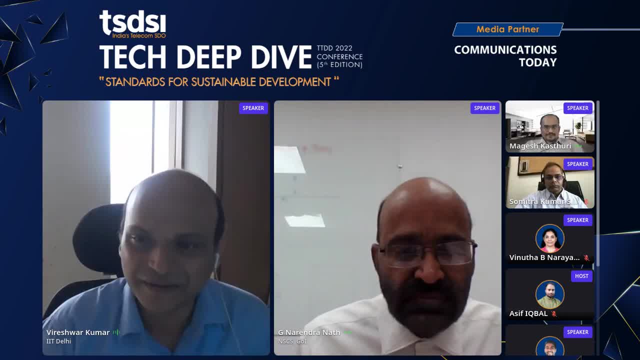 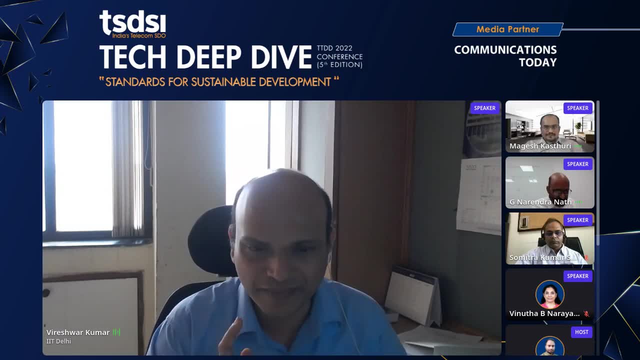 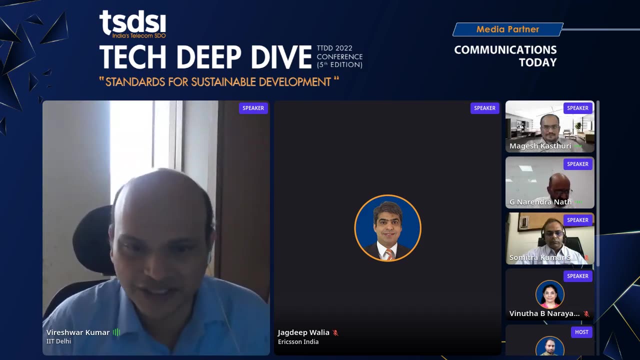 Yes, yeah, Thank you for your comments, Thanks. So let me go to Mr Walia and take a quick comment about so can you just highlight one major contribution that India is doing in the 3GPP domain in terms of 5G security? 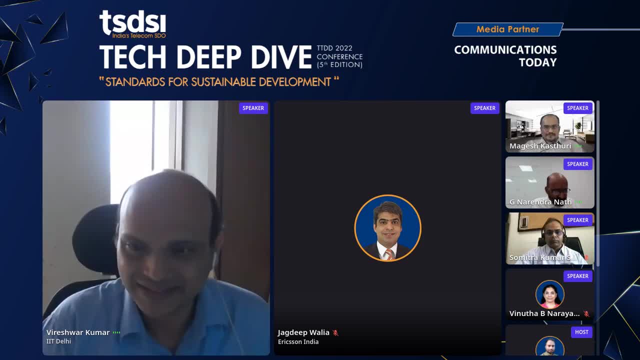 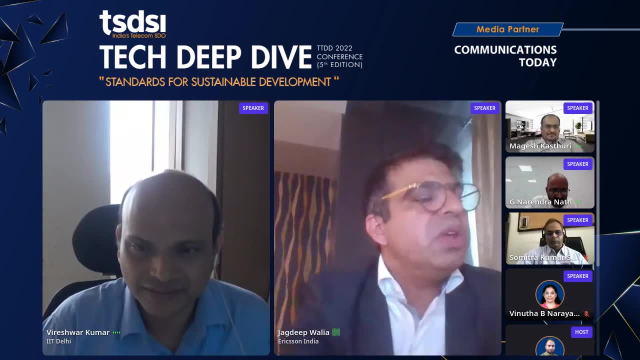 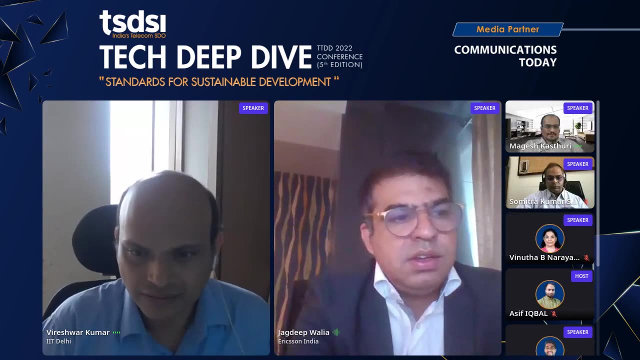 Mr Walia, I would say I mean, I think what we have, at least from a India perspective, I think we are getting involved with the 3GPP standardization process and there is more and more interaction that is happening. 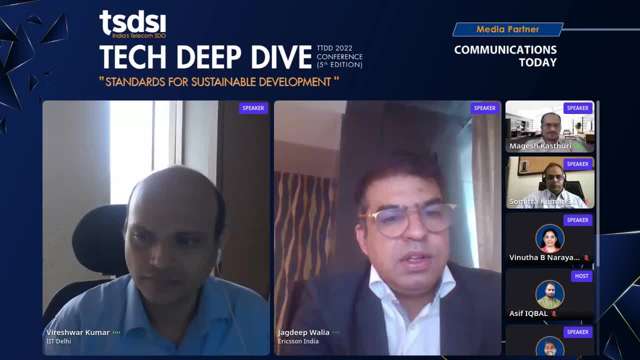 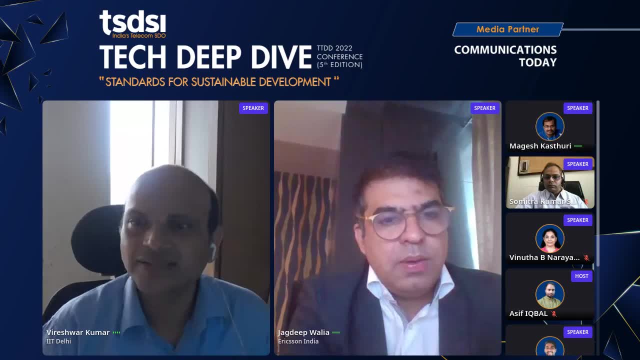 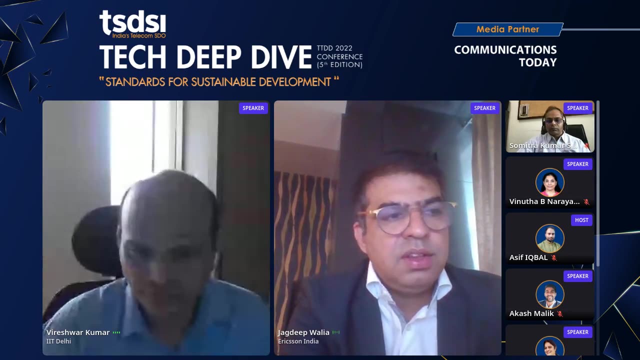 I think this is something that we have started, so it is hard to say, okay, specifically, we have what we have brought out towards 3GPP. so I would say it is hard to say, but then the thing is that this is: 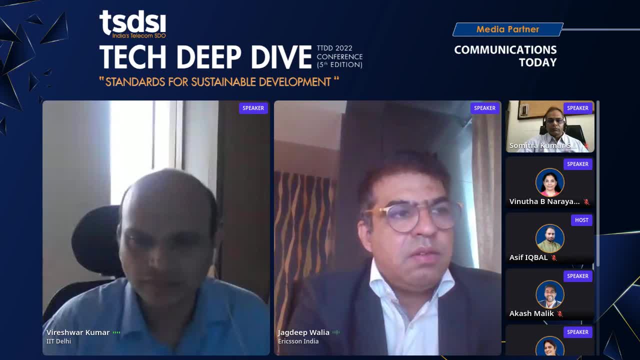 something that has just started, wherein, from an India perspective, we are taking more and more kind of getting involved with 3GPP and, as we go forward, we would see that these India specific requirements are then also included as part of overall 3GPP standardization process. 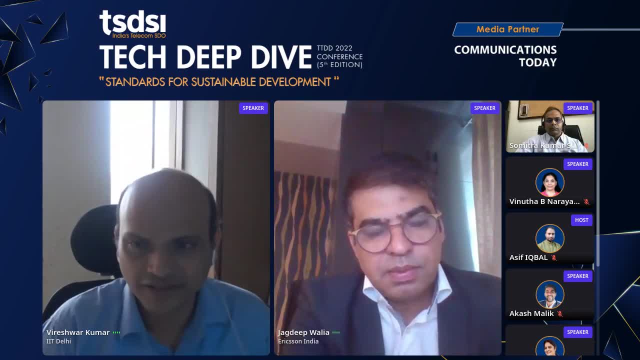 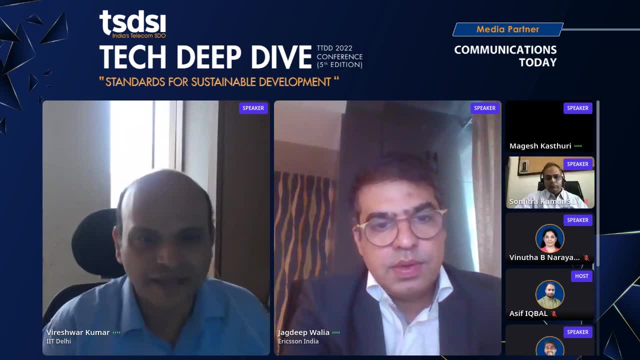 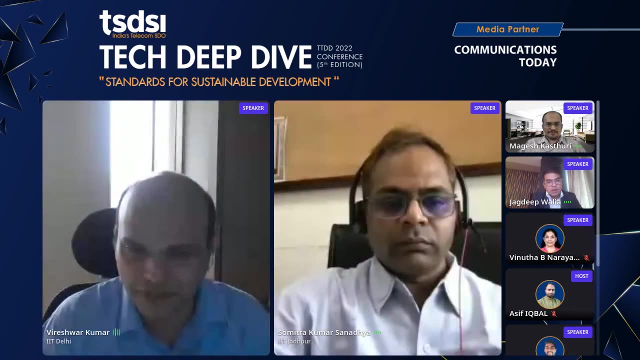 That is what I would like to comment in brief. Okay, yeah, thank you very much. So I will also quickly go to Dr Sanathya. So, Dr Sanathya, so are there any fundamental challenges in post-quantum cryptography? 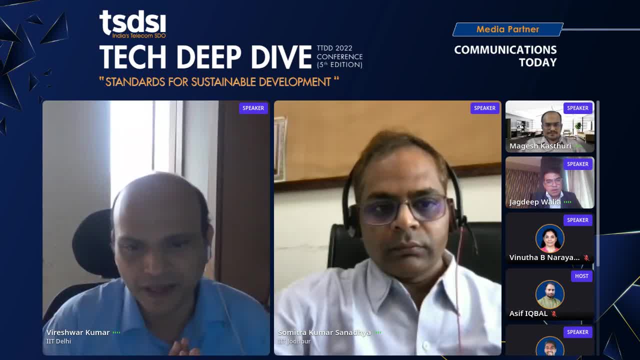 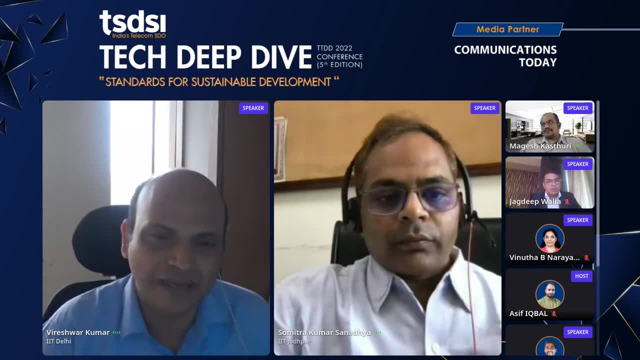 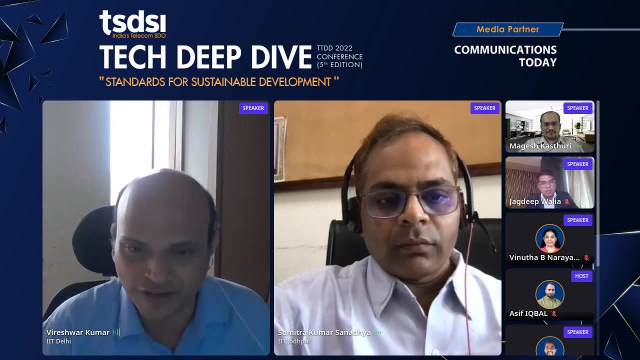 with respect to implementing them on IoT devices. So can you just highlight one quick challenge that the participants in this panel discussion, or the people who are listening to them and interested in quantum, can take forward and work on that? Yeah, so one of the issues that we already 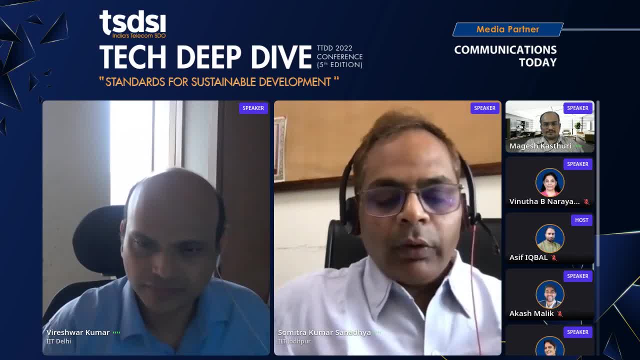 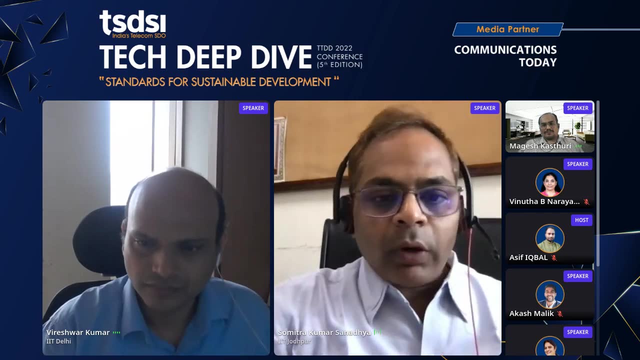 discussed was the parameter sizes. If you are looking for even, say, 128-bit security, the parameter sizes are very, very large, even for small devices, lightweight devices. So this is a very big challenge and that's where we will have to not use. just these PQC algorithms, but we will also need symmetric algorithms which essentially, will be attackable by Grover's algorithm. So, essentially, if you want to achieve, say, for an IoT device security level of 80 bits, we will be using 160-bit security. 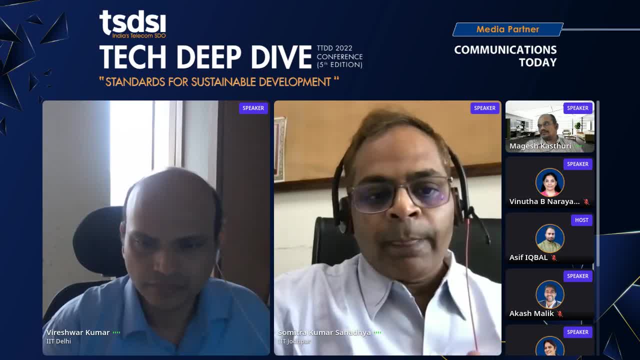 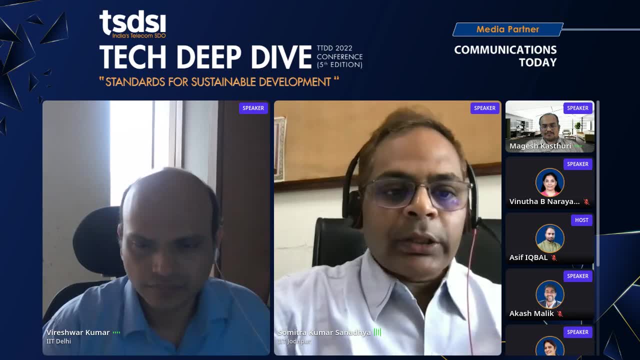 algorithms and probably they can be very, very fast. Fortunately, we have another line of algorithms in this direction which is standardized in the NIST competition on lightweight cryptography, or LWC. So LWC is something that we can work on and this is something. 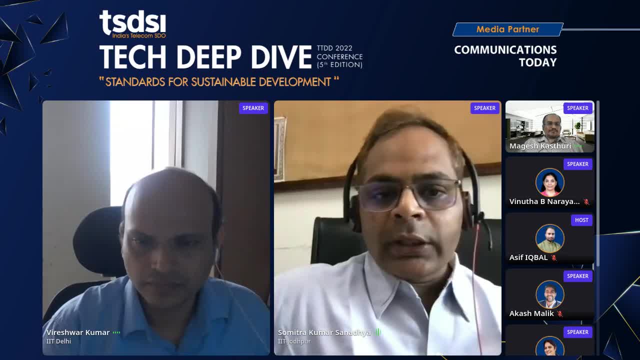 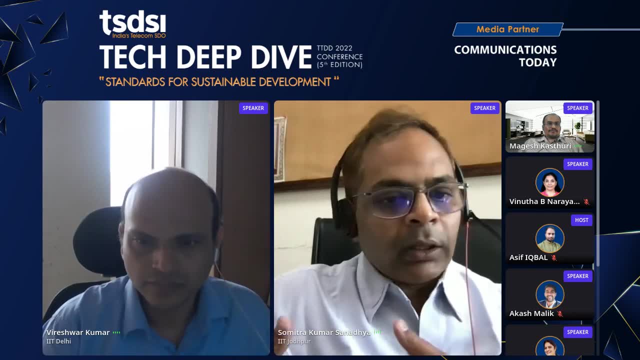 that, again, I would like to highlight. As a country, we are not focusing enough on studying these kind of algorithms. there are very few groups in the country who are working in these and, being from academia, I would at least like to argue about closer collaboration between academia. 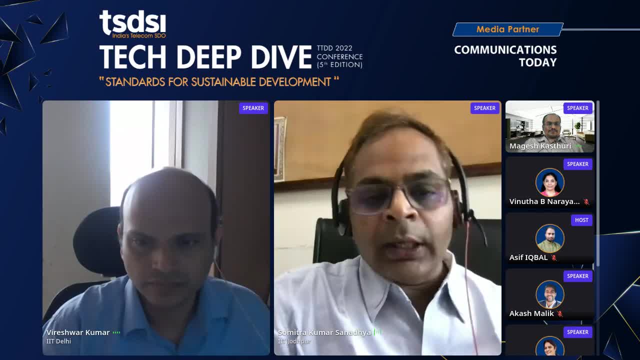 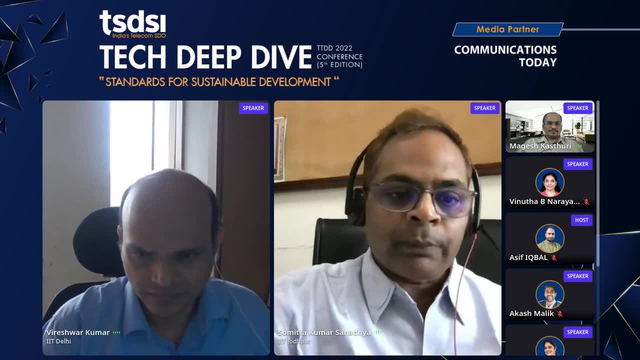 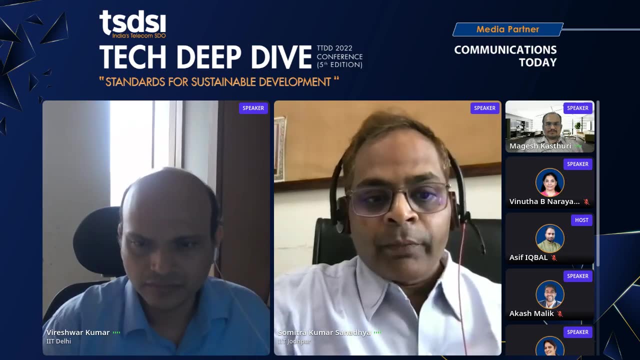 and industry, which unfortunately hasn't happened too much in India. So hopefully that is something we learn and probably invest more on it in future, and not necessarily in terms of the government support. Government support is actually very, very good in many, many situations. 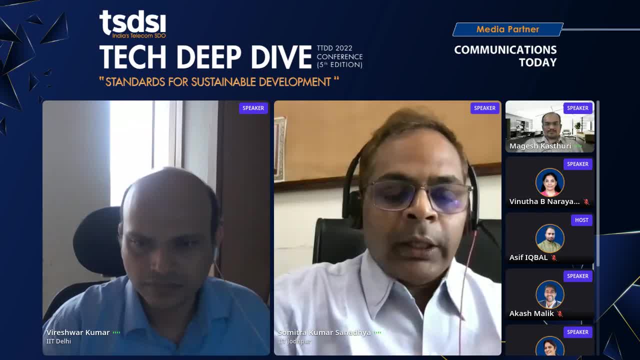 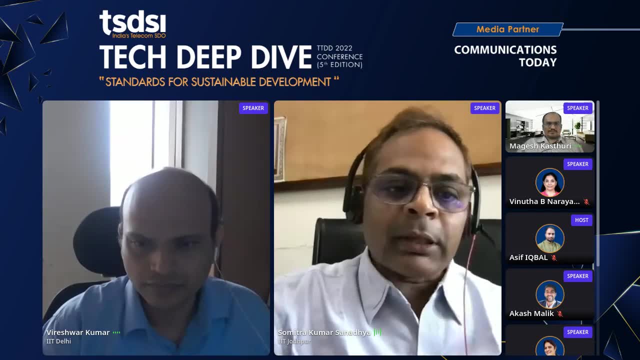 I would say that if somebody writes a good proposal, it is highly likely that it will be funded from one of the government agencies. My problem is actually the industry is not coming up to that same extent, And because industry is not coming, we are not in a situation. 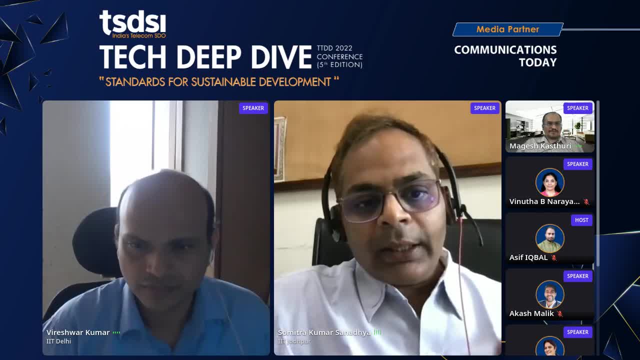 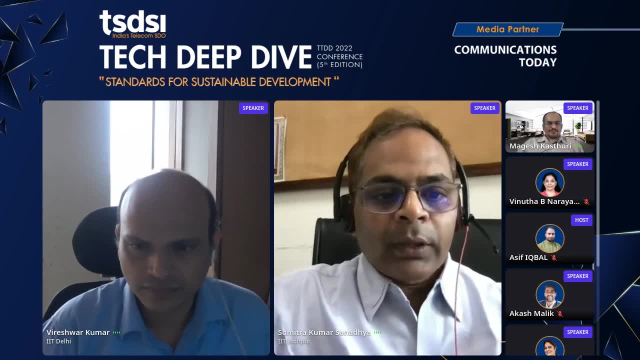 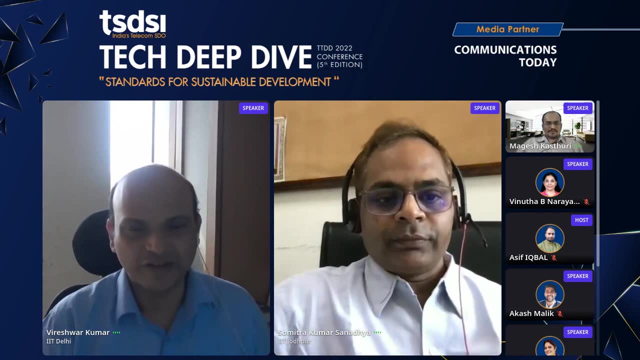 where we can think about deploying algorithms. So probably that deployment and more study of practical attacks, which cannot really be done purely by academia, is where we are lacking terribly, and hopefully this is an area in which we will do further work. Thank you, As a young member of academia. 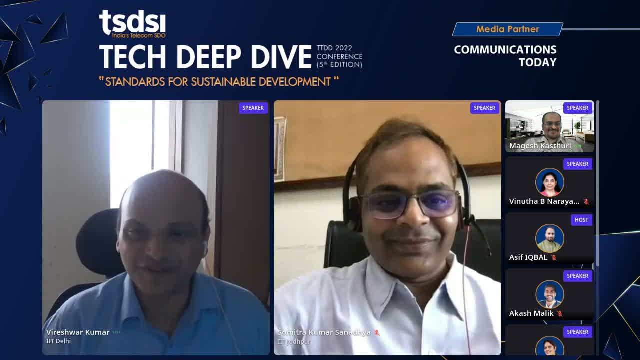 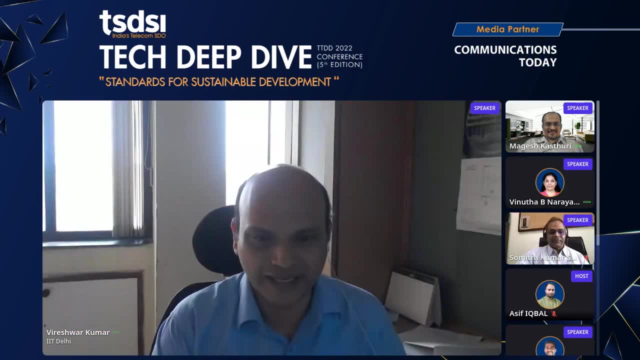 I also hope that whatever you are suggesting becomes true, Thank you, So I guess we are out of time now. I would like to again thank you, all the panelists, for giving their views and highlighting the key issues that we have been looking into in the domain of 5G security. 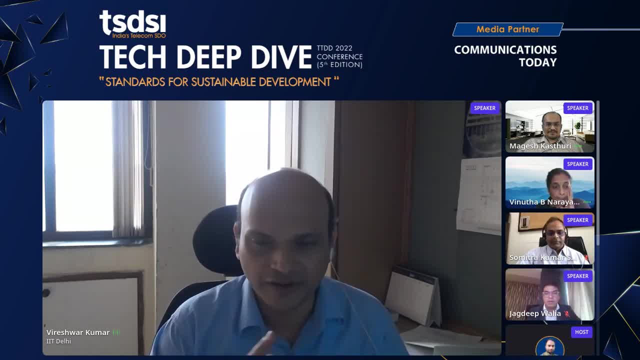 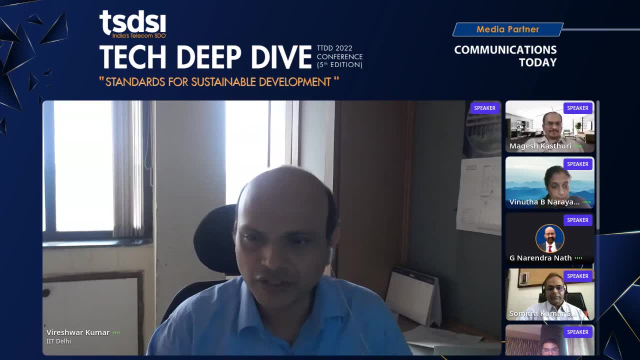 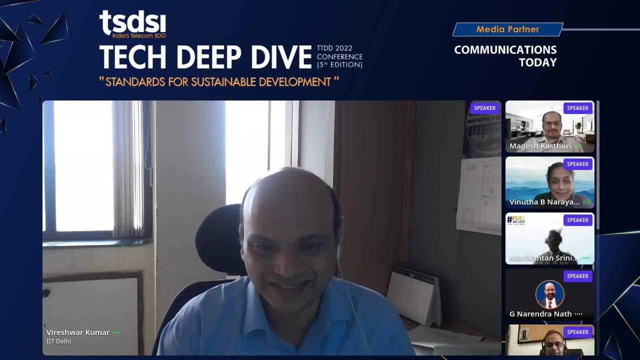 IoT security and the impact of quantum on 5G enabled Internet of Things. So thanks again to everyone. So I would like to go back to Vinuta to give a few concluding remarks and then close the session. Thanks, Thank you all to each of the panelists. 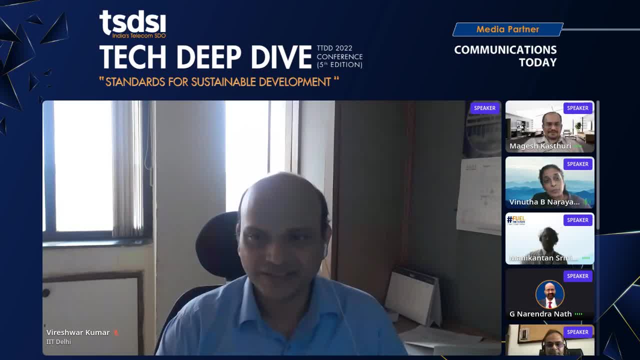 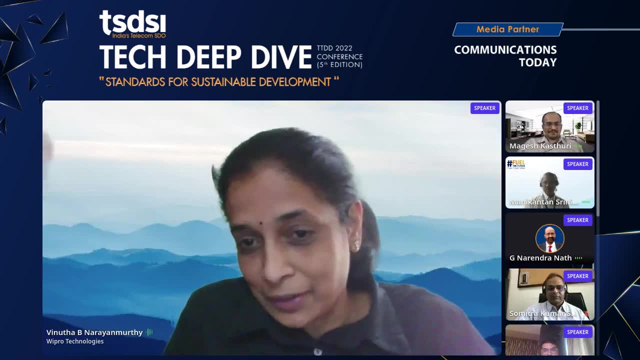 for such a wonderful session where we talked about right from what's happening in 5G to make it far more secure, to the challenges to how industry and academia- everybody should collaborate together. To just end the final note, I mean across the complete session we live in. 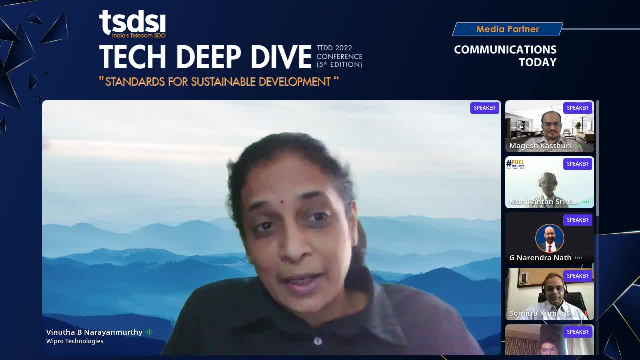 a world where we have multi-vendor virtualization, 5G enabled, IoT world. It has a set of security challenges. Quantum computers has further added to these challenges, But with methods such as design audits, security testing of networks as a daily affair.